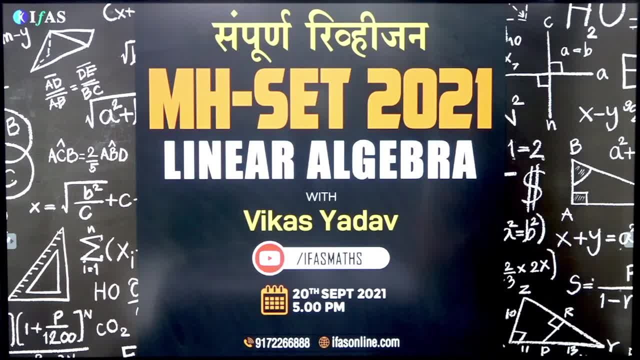 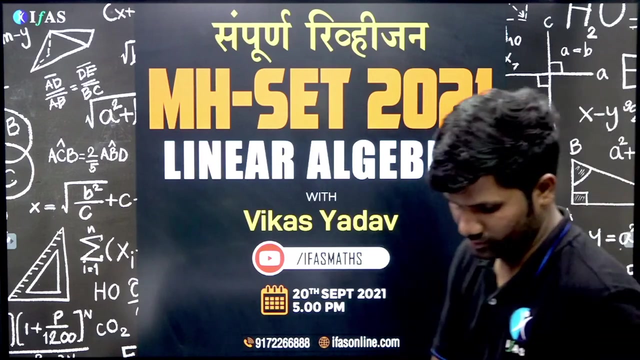 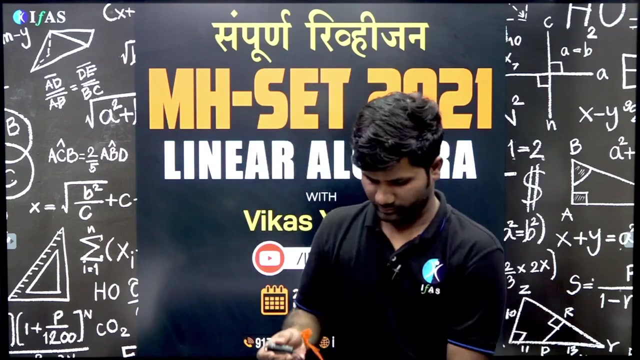 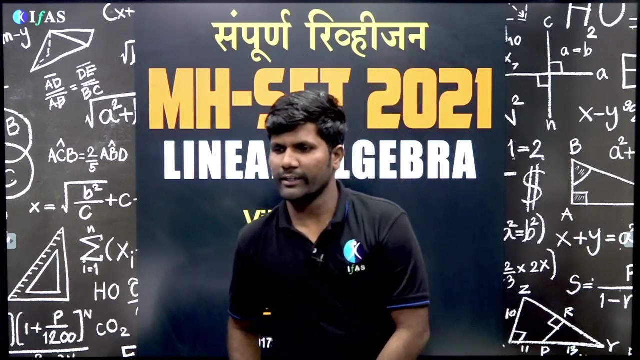 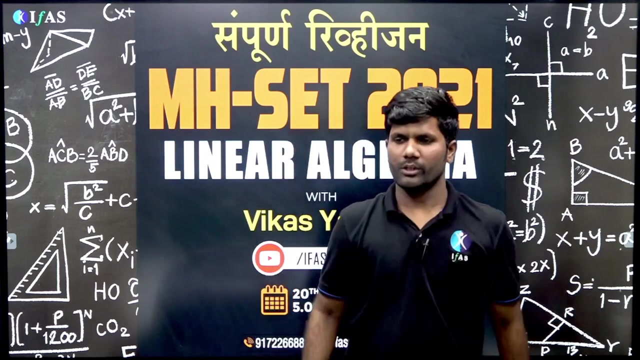 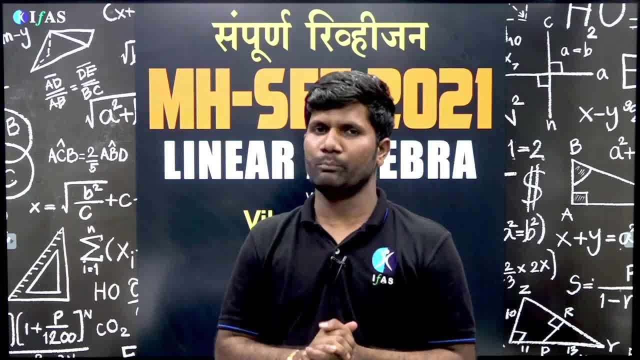 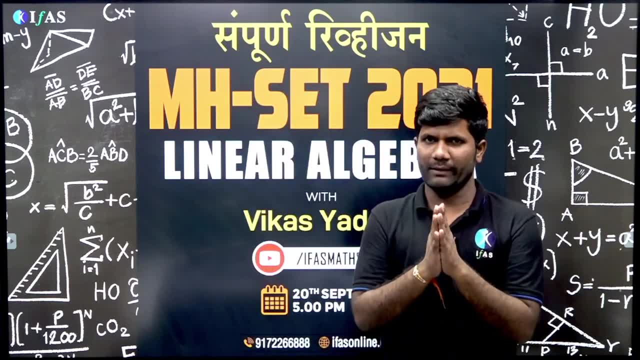 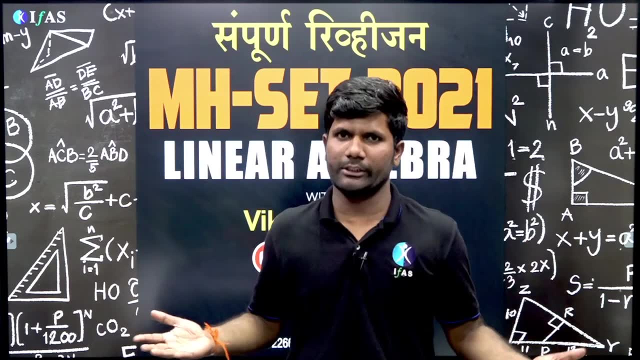 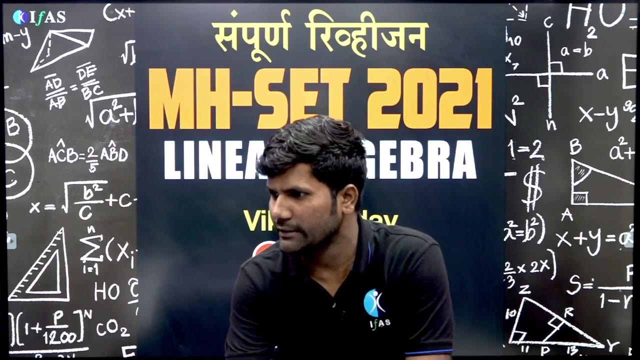 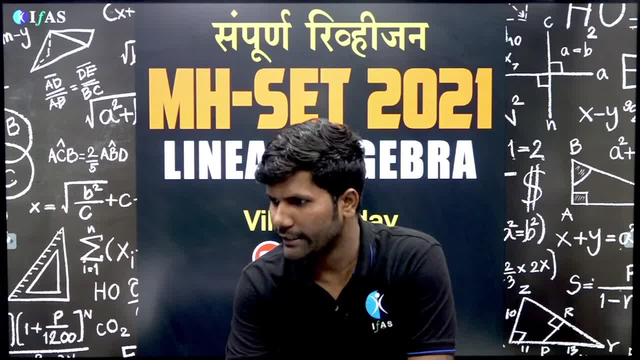 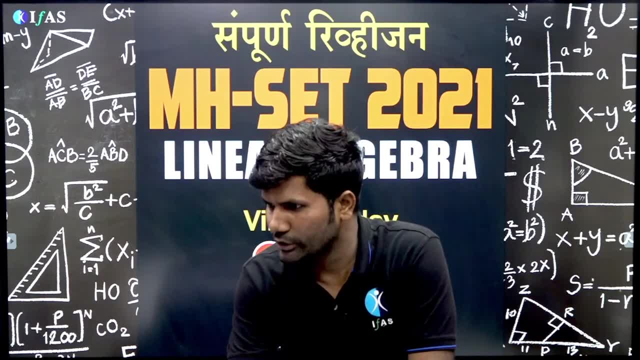 Thank you, Thank you. Thank you, Taslima Sekh. So good evening everyone. Lalita Pawar, Jyoti Dhiman Vivek, Rohit Kia Vaisnavi, Lalita Dilip. 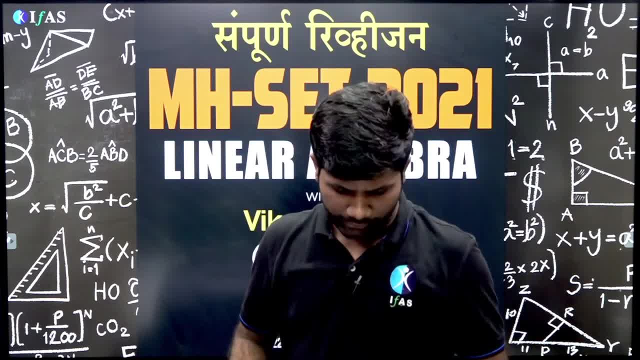 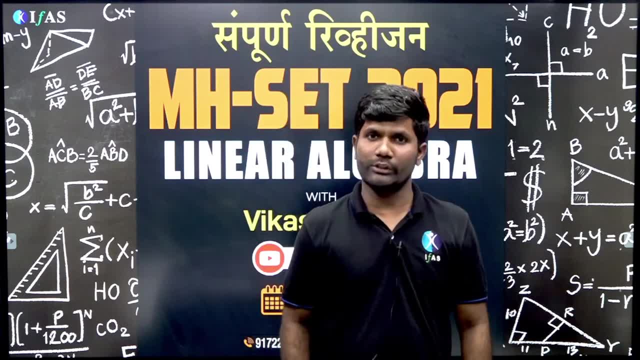 So good evening to all of you. So welcome to our online platform, So we hope that you will be fine. So what are we going to do in today's session? In today's session, we will solve some questions. 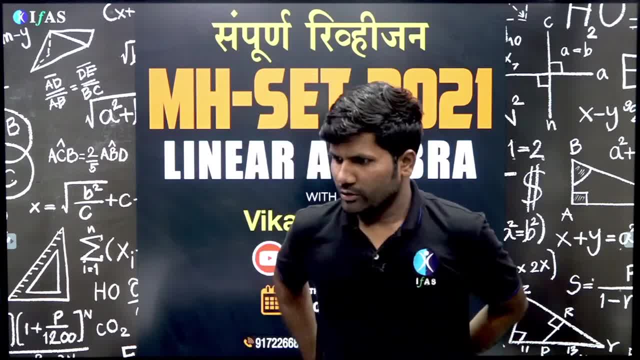 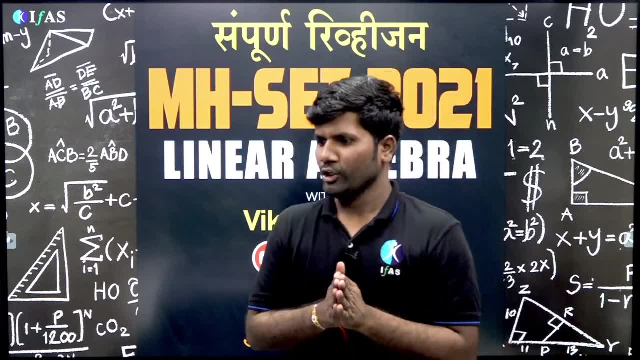 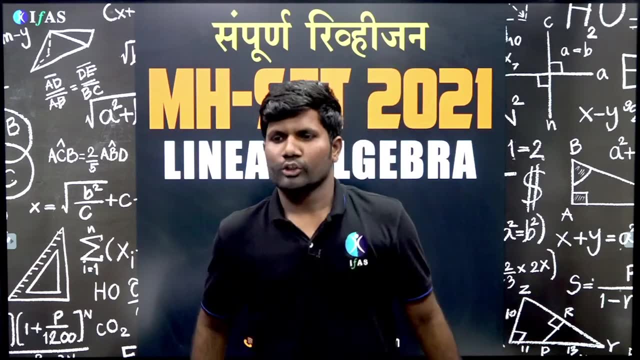 There are 25-30 questions. Okay, Good evening, Subham Malik. So let's start today's session. So if you are new to our channel, then what you have to do is subscribe to the channel. You have to turn on the notification bell. 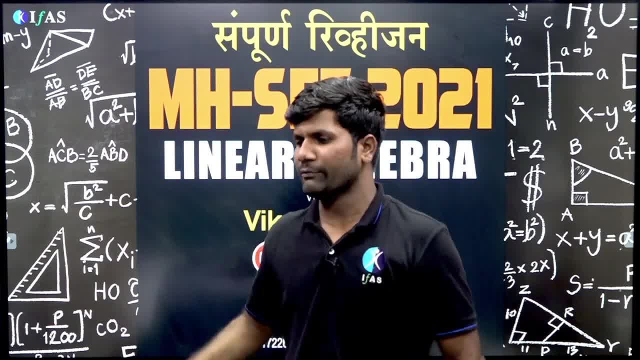 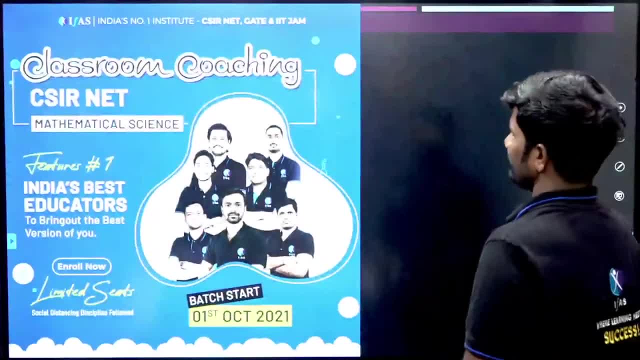 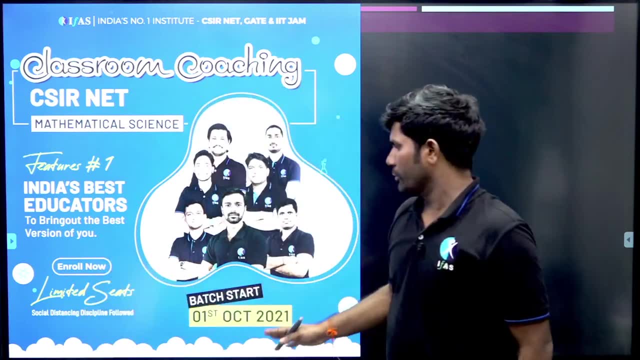 If you have not liked the video yet, then like it once, and then we will continue. Okay, Okay, So let's go to the next slide. So now we are moving from online to offline. Our offline Classroom coaching. From 1st October, a batch is starting. 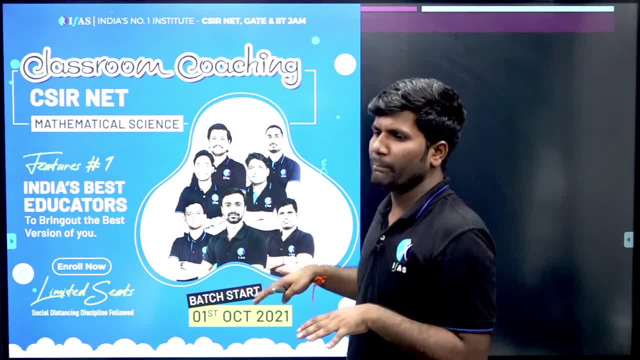 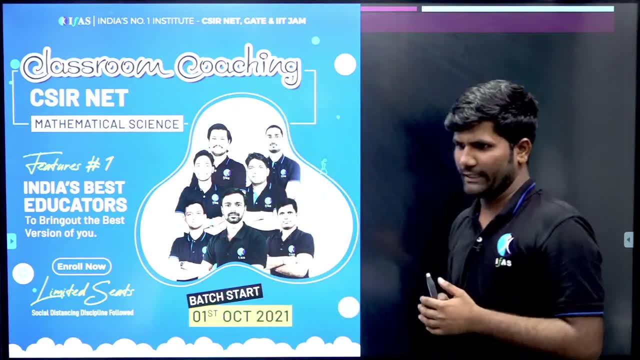 If you are preparing for CSRNet And our batch has started in Pune So you can join us offline, You can clear all your doubts there. Okay, Let's go. So our new batch is starting- Offline batch. Since when? 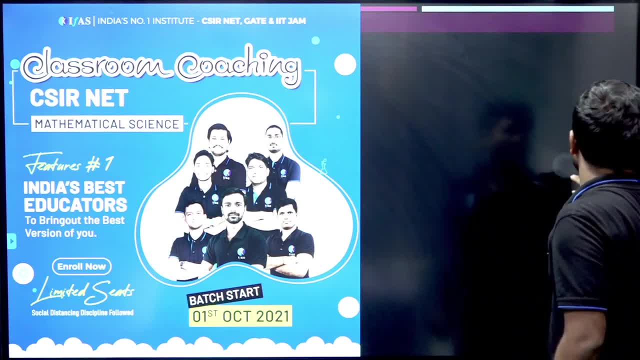 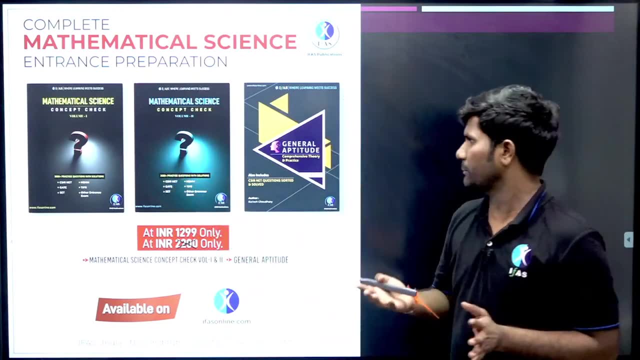 From 1st October: From 1st October for CSRNet And this is our book: Mathematical science, Two concepts: One is where there was a thousand plus questions And this is the book of the aptitude And those who had ordered. they have started getting dispatched from today. 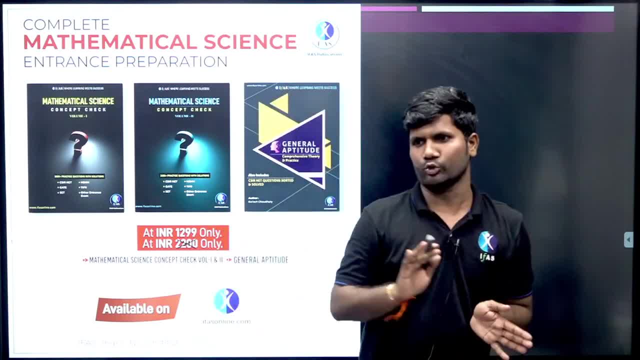 So in 4-5 days they will reach your house. Okay, So from today they are being dispatched from our side. Let's go. And you can get these three books only on 1299.. For this, you have to visit our official website. 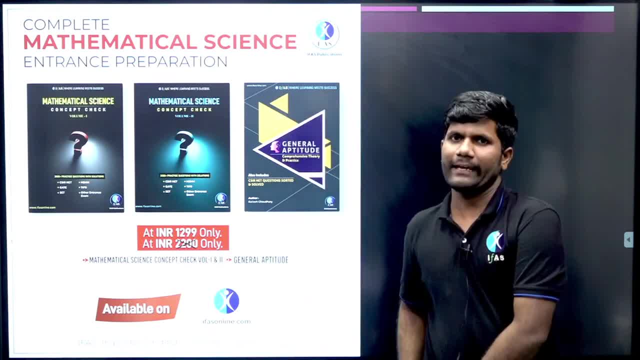 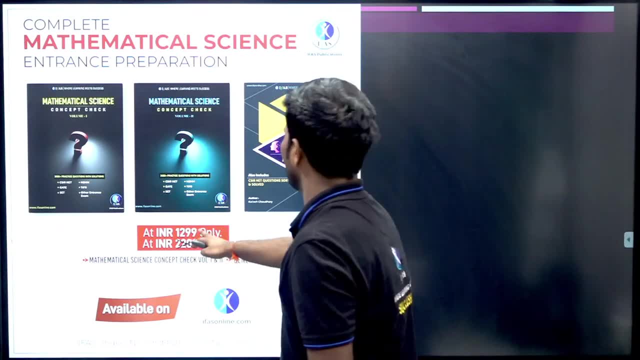 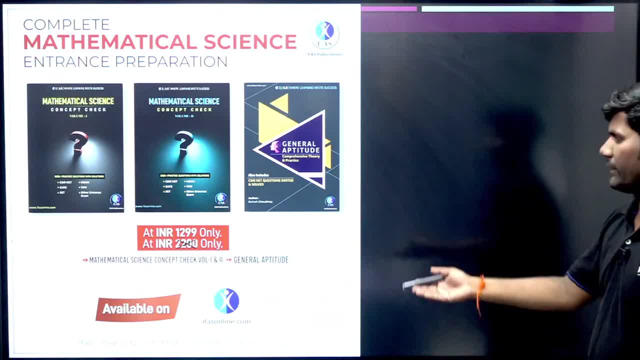 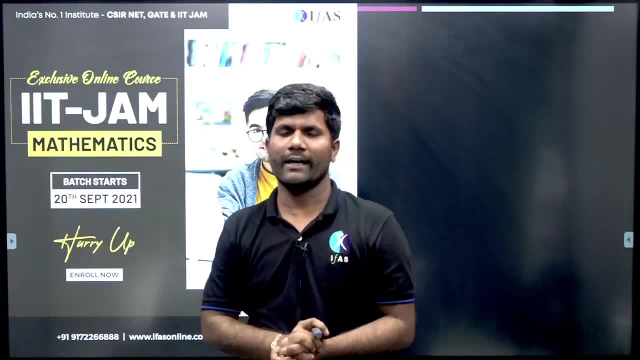 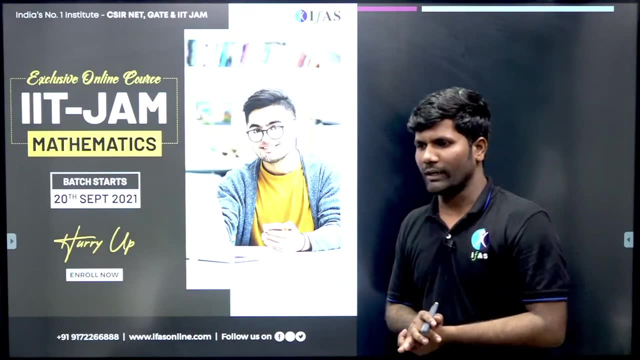 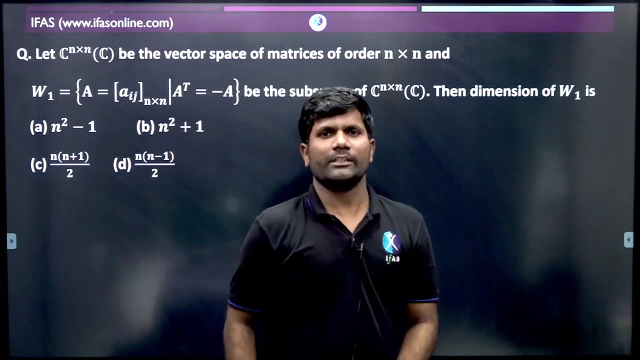 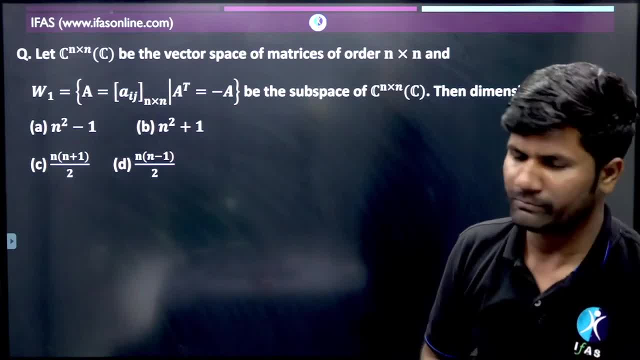 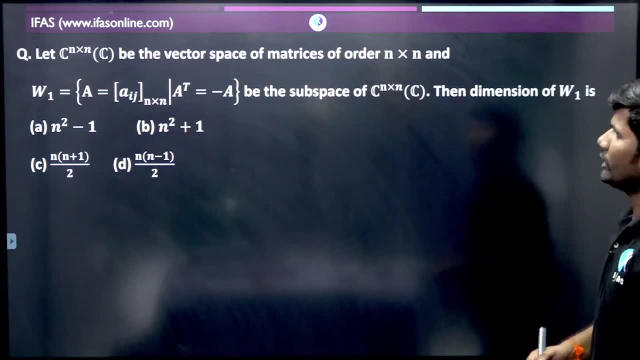 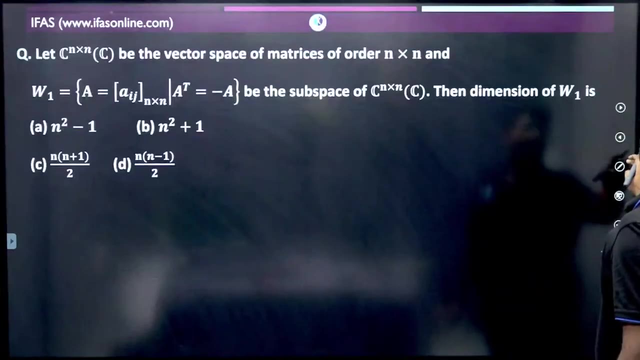 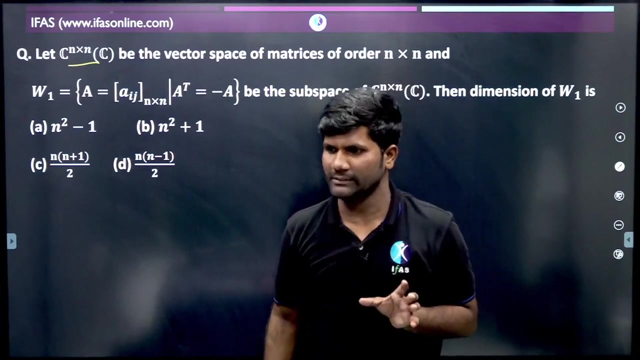 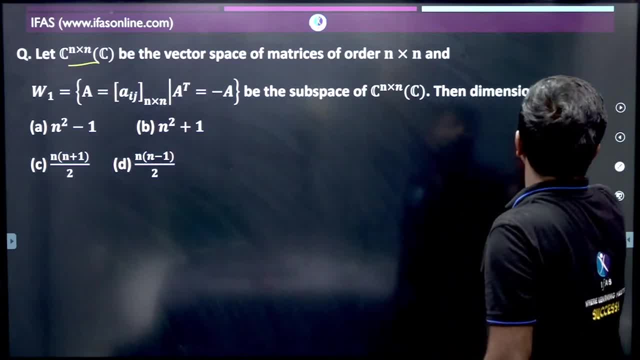 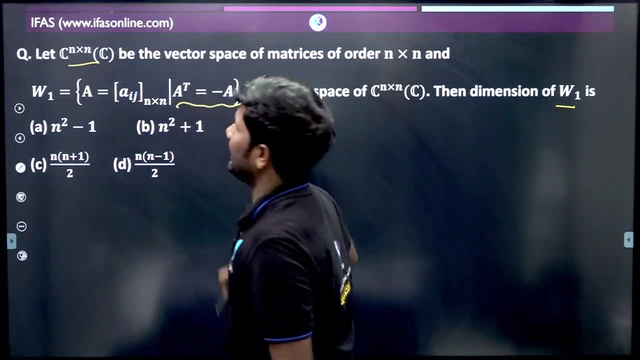 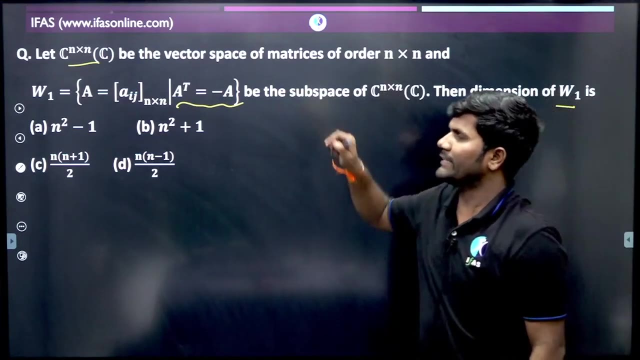 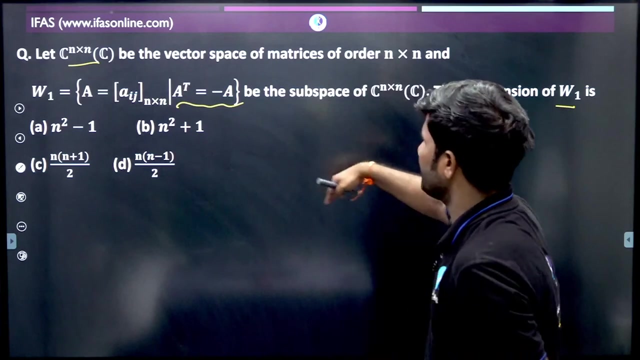 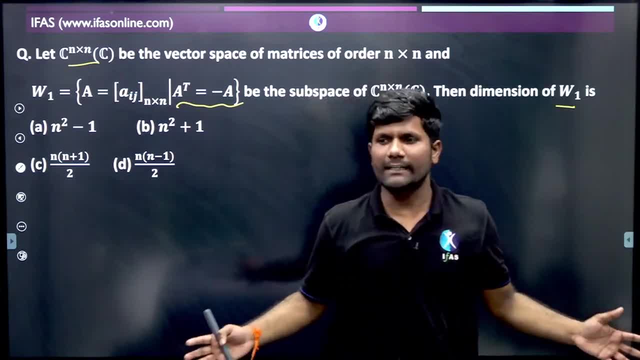 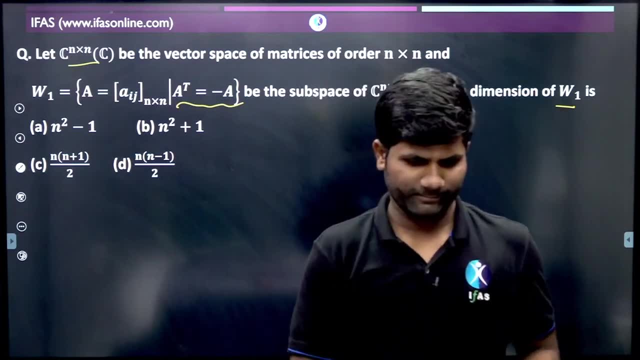 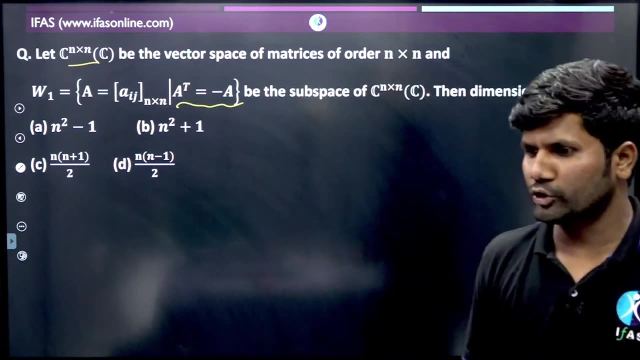 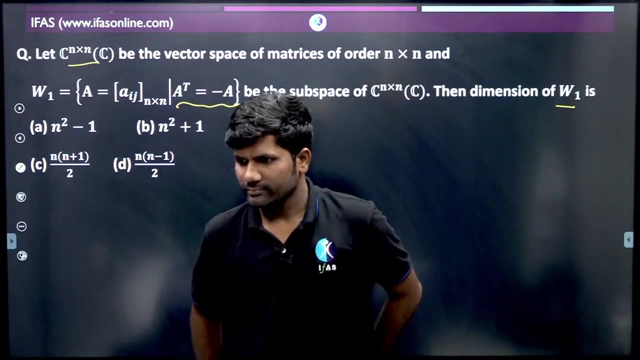 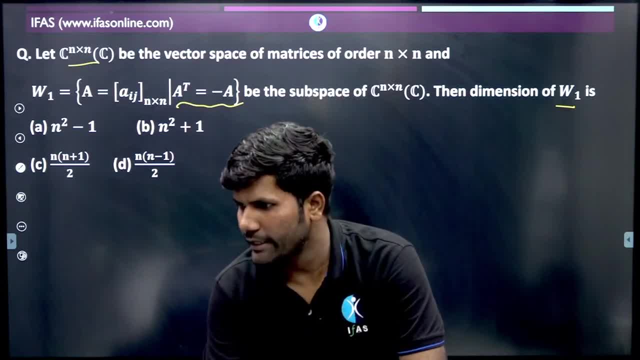 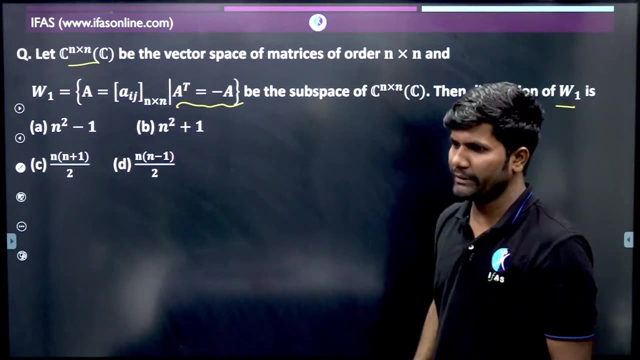 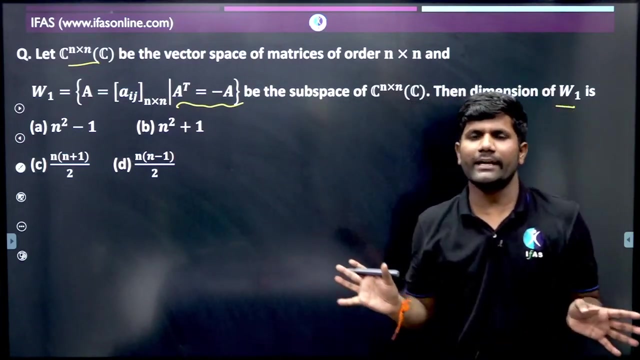 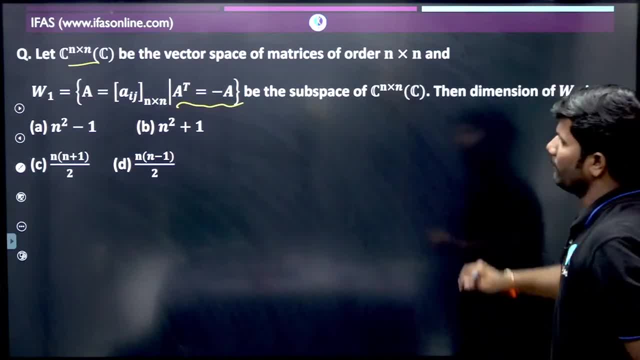 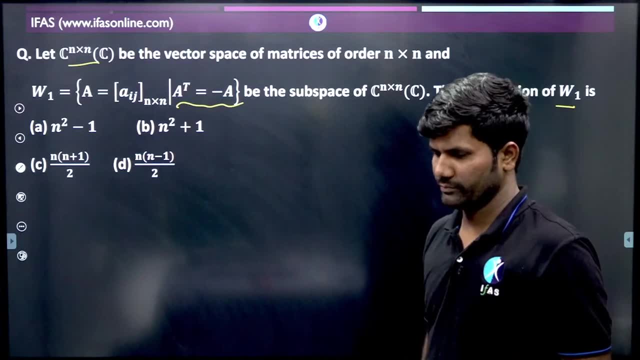 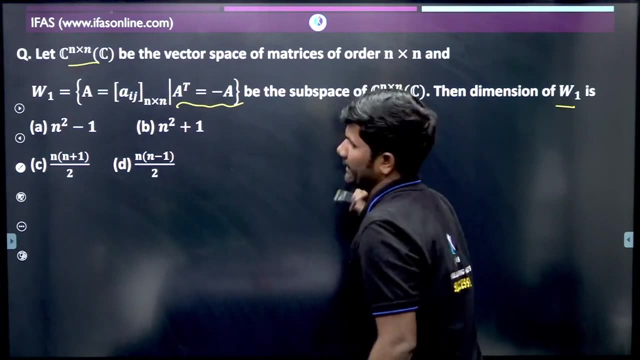 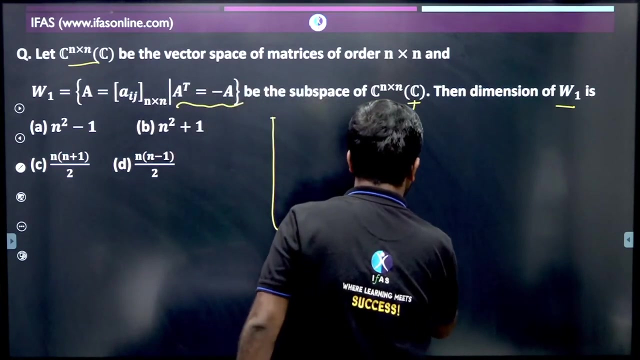 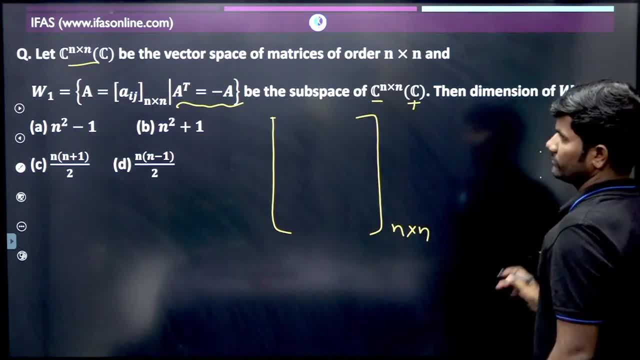 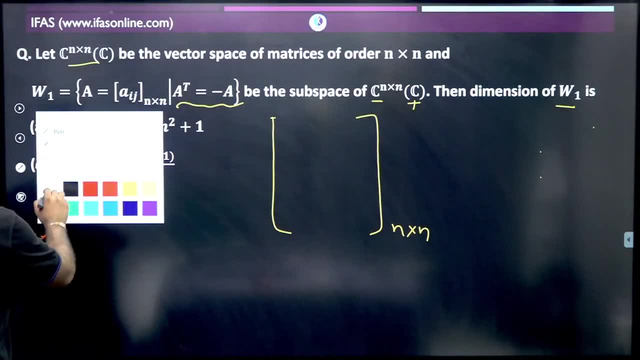 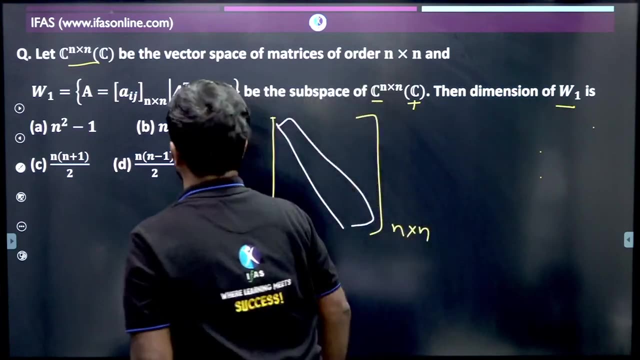 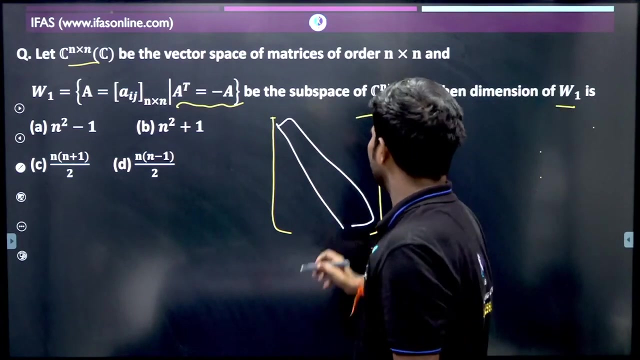 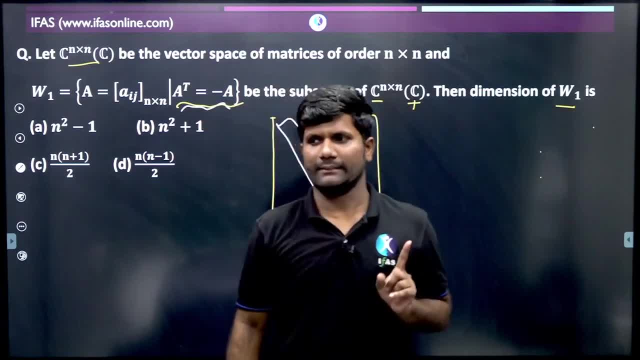 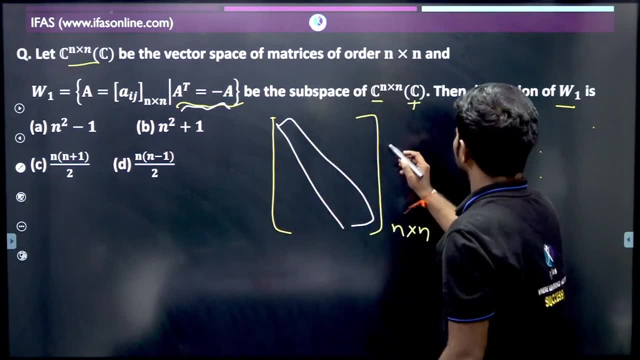 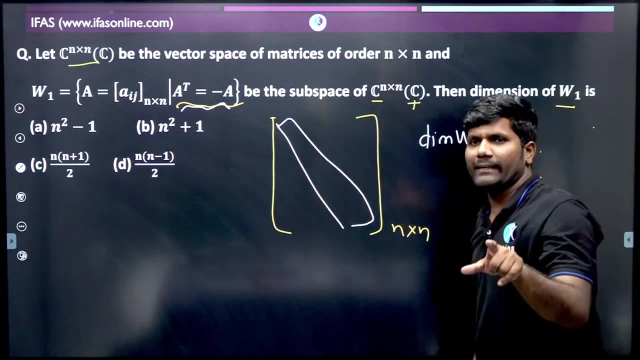 because this is a skew symmetric matrix. if it is a skew symmetric matrix, then its diagonal elements are zero. if I want to find the dimension of w1, then how many elements are there in this matrix? so in this matrix total is n square element, but in diagonal there is zero. so we remove the diagonal. 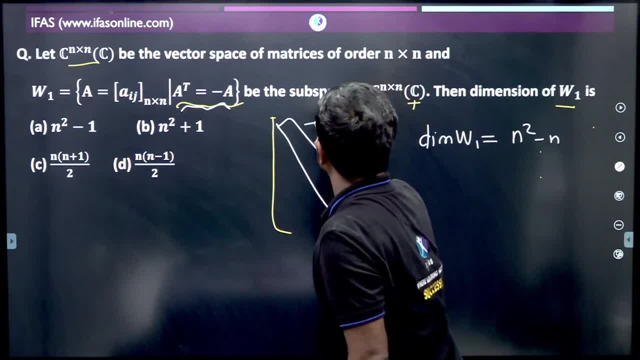 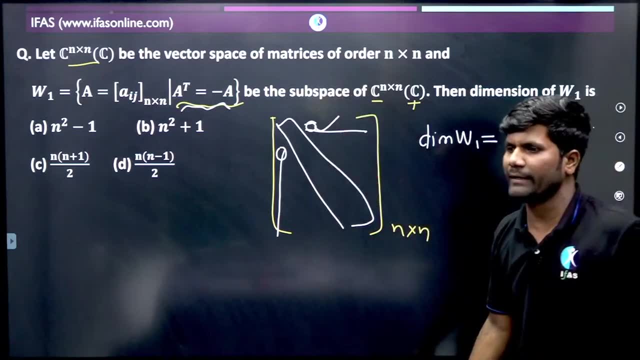 n square minus n. now, the element which will be here minus time will be here. also means: if I generate it by itself, then it will be generated by itself. if the first row is made, then the first column will be made by itself. this means n square minus. 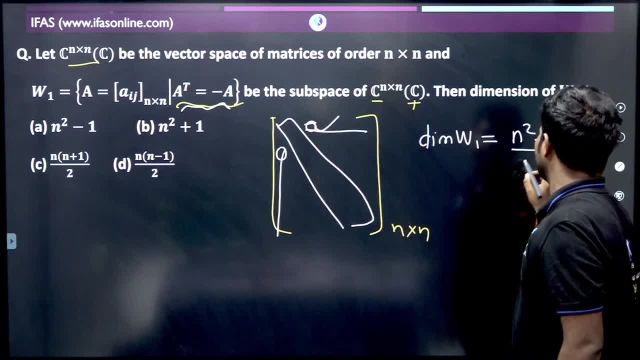 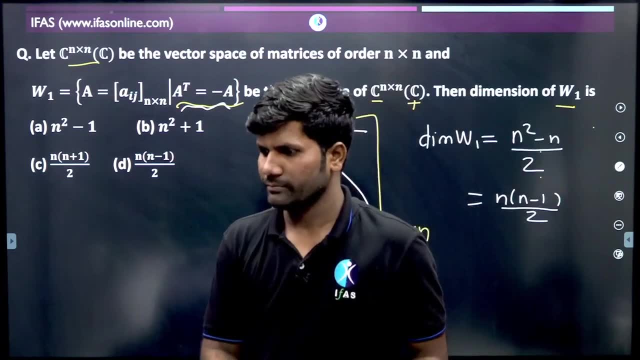 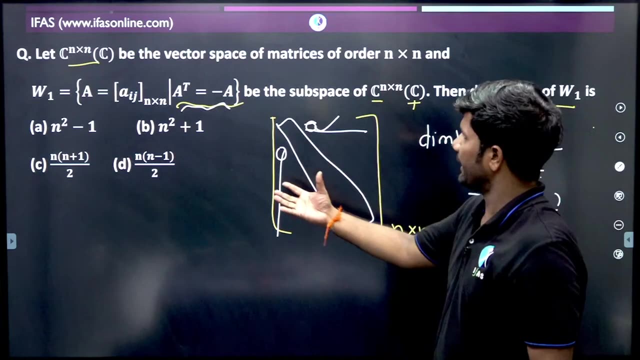 so how many total elements were there? now each element is repeated twice, so divide by 2. so if you write this, then what will happen? n n minus 1 by 2. so this will be the correct answer. ok, so what will be the correct answer? so here for this question, we will get the correct answer. 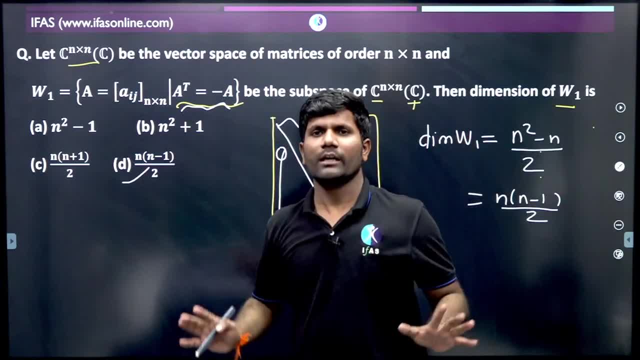 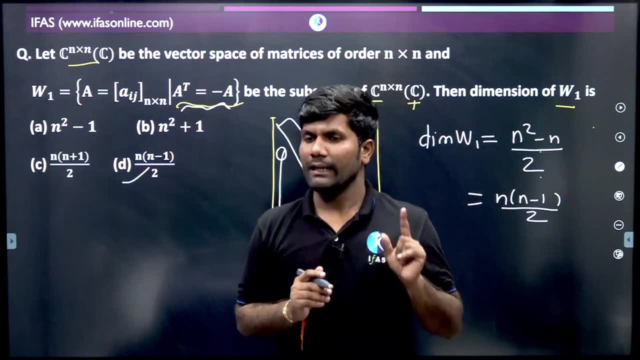 option D. is it clear till here? does everyone understand? does anyone have any doubt? what is the correct answer? Pooja patee lei said: ok, very good, Pooja. what did the rest of the people get? is it clear to everyone once you comment, so that I move ahead? 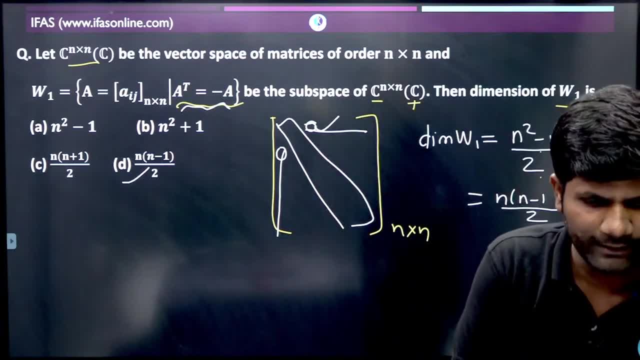 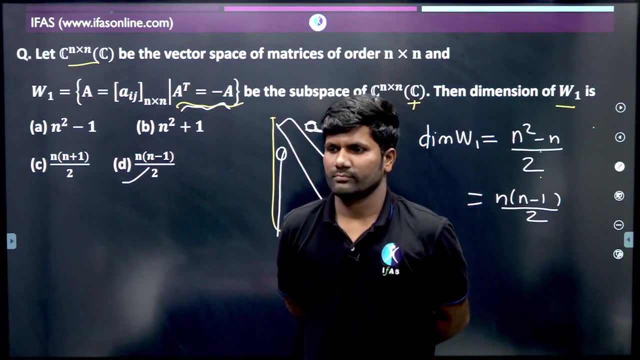 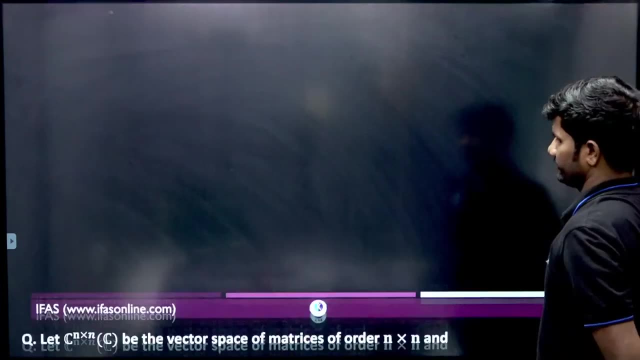 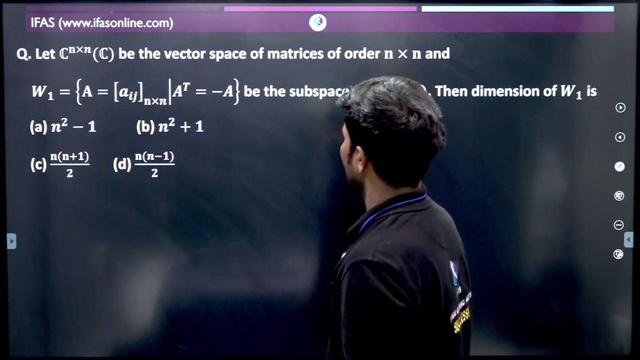 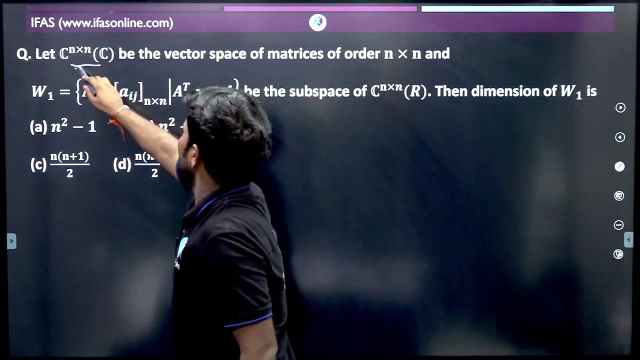 on the next question. please comment fast once. let's come to the next question. so here again we have been given a question. Now what will be the correct answer for this? What is given here? Same matrix, same vector, space is given C, n cross n over C. 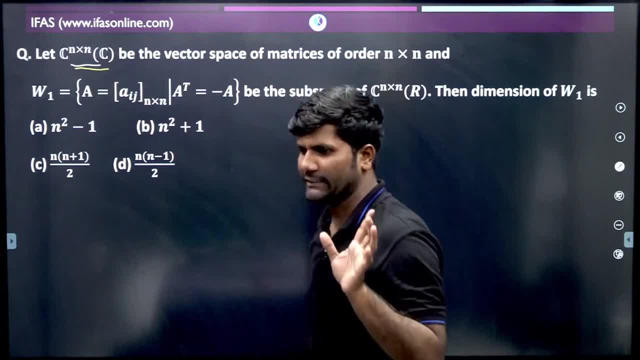 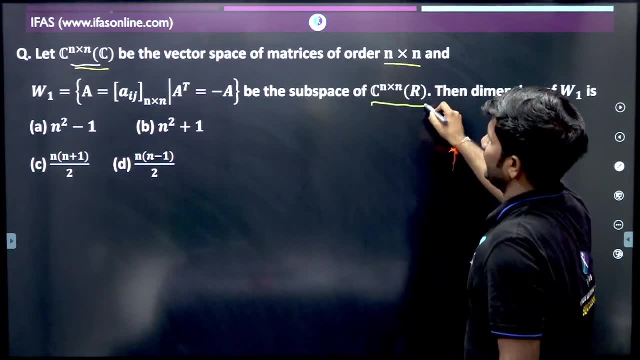 Means set of all n cross n matrices whose entries are complex numbers. Now, what is given to us after that? W1 has given a subspace. we have been asked. It is given over R. What do you think? What will be its dimension? 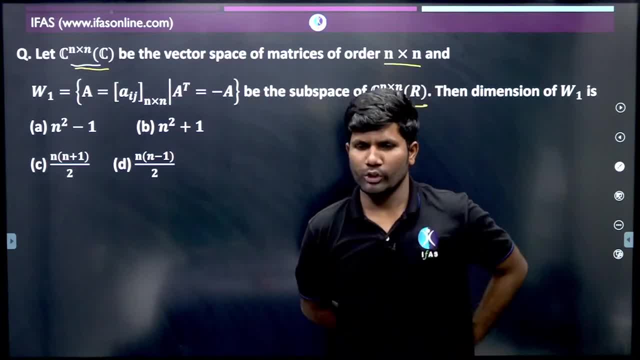 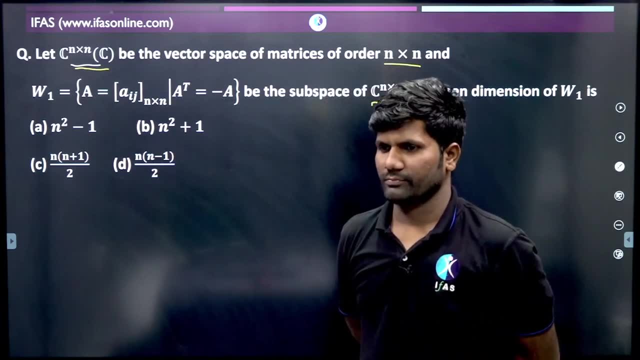 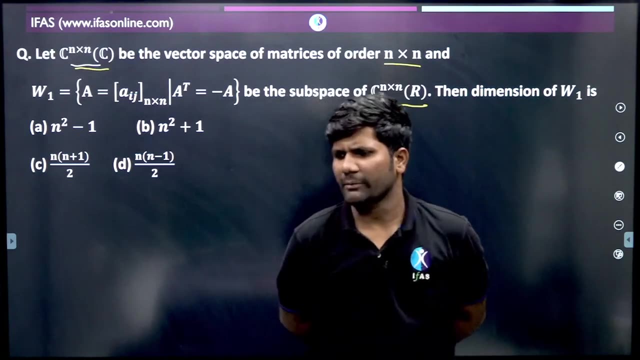 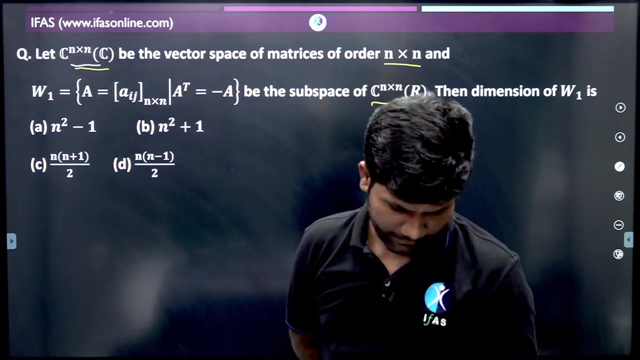 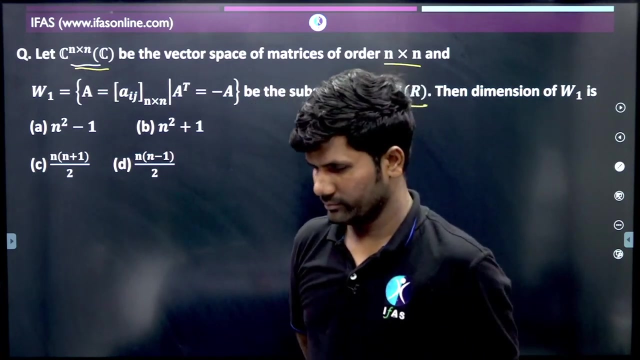 Good morning Nandita. So quickly solve it and tell us what will be the answer. What do you think? It will take 1-2 months to find the answer. So others tell us what is the answer. Sajnima A is saying: Mathematica A is saying: 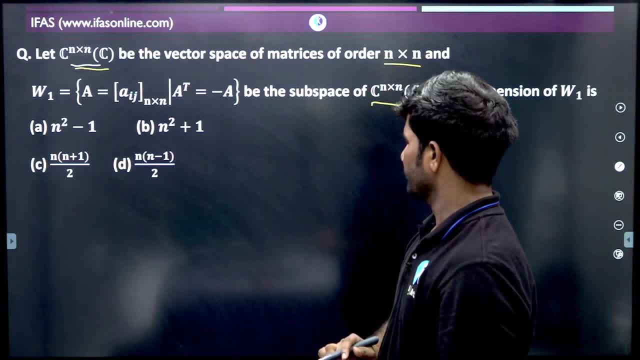 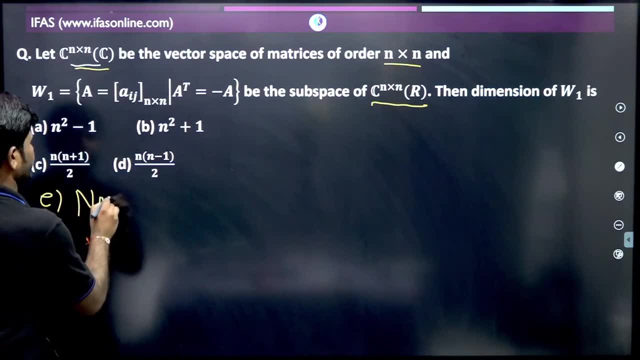 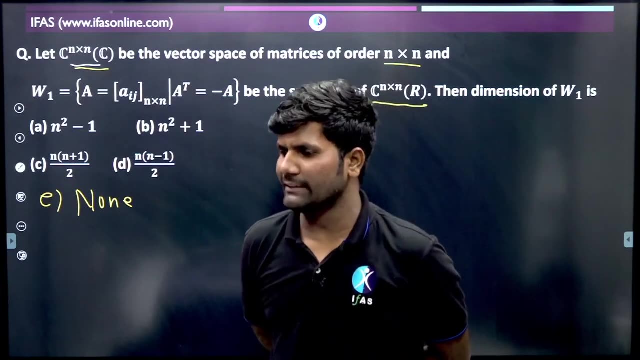 Bharati Nagpal is saying n square minus n. So add one more option here: None of the above. Add one more option here- D none. Now tell us what will be its answer. Ok, So now solve it and tell us what is the answer. See here. 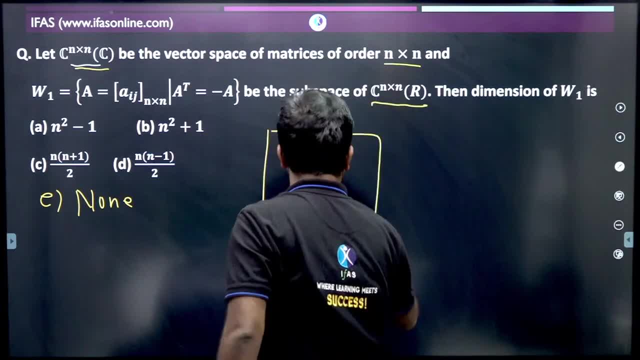 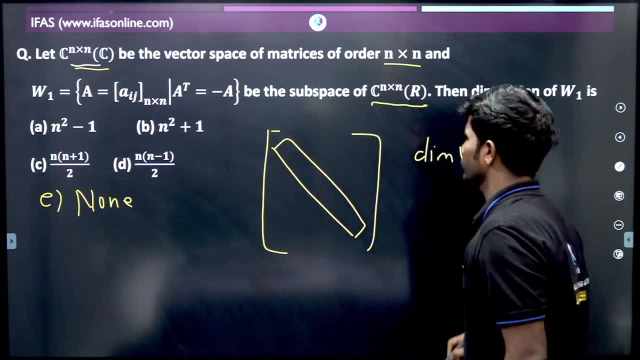 First thing, the same situation is here, Here. What is the diagonal? It is zero. So if I want to find the dimension, So if I want to find the dimension of W, Total element is n square. But what is the diagonal there? It is zero. 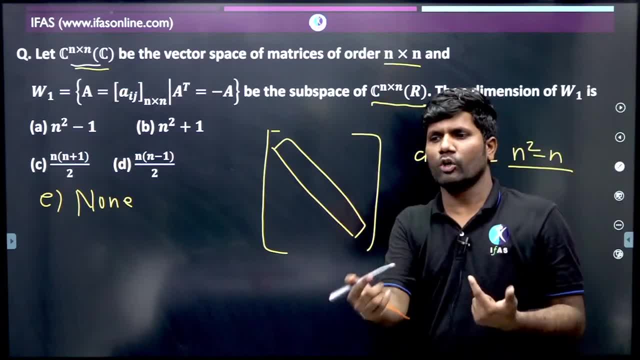 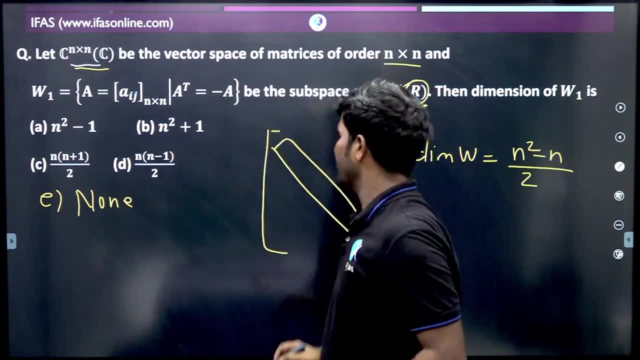 So what did I do? I removed the diagonal Rest. each element is repeated twice, Divided by 2. But here over R is given What is the dimension of C over R? It is 2 Means to generate one element. here It will take two elements of R. 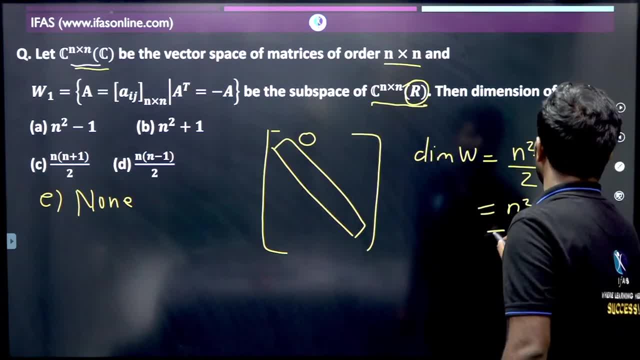 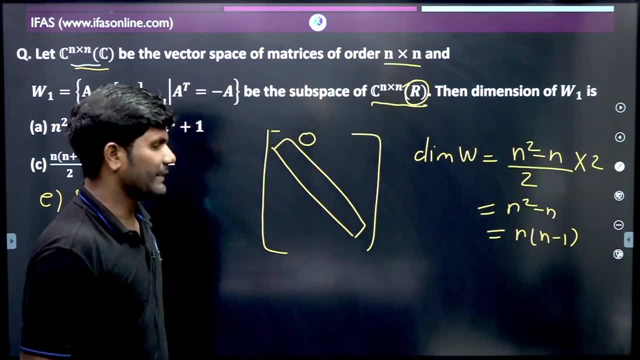 So multiply by 2, So what will you get here? N square minus n. So what will you get? N minus 1. So what will be the correct answer here? So solve it and tell us what is the correct answer. 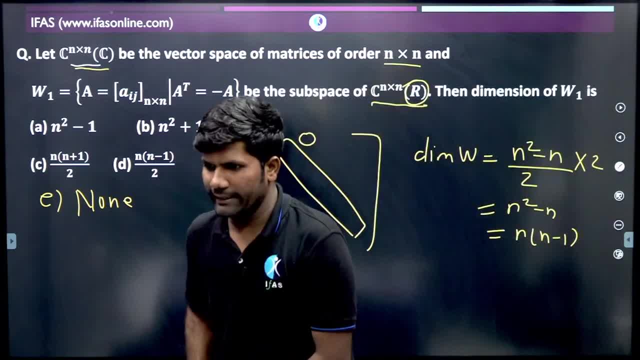 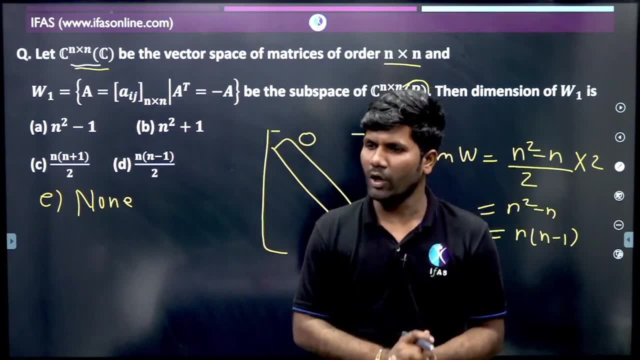 All students. What do you think? Ganesh E. Sheetal E. Phulkit B, Gokatto, None Ok. Bharti E- Ok, very good, So you have given the right answer. The correct answer will be D. Now let's come. If it is clear till here. 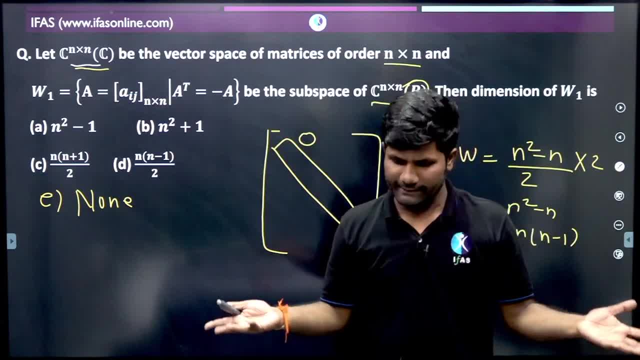 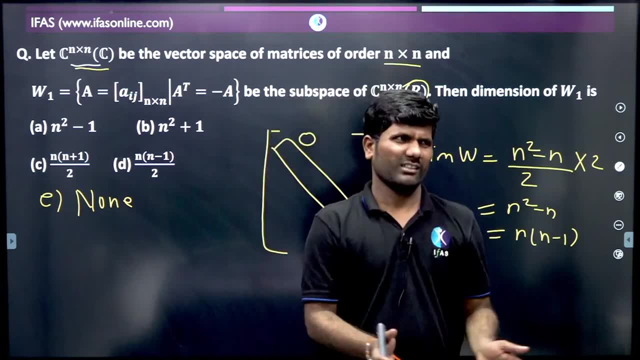 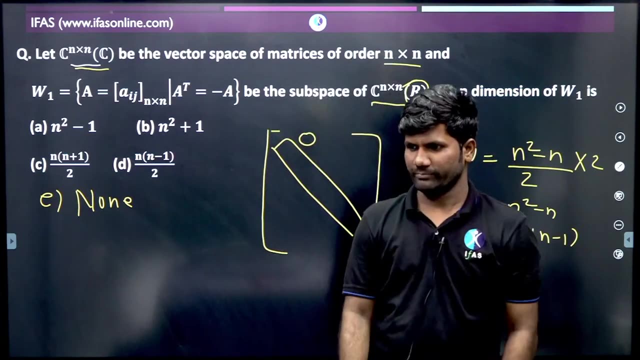 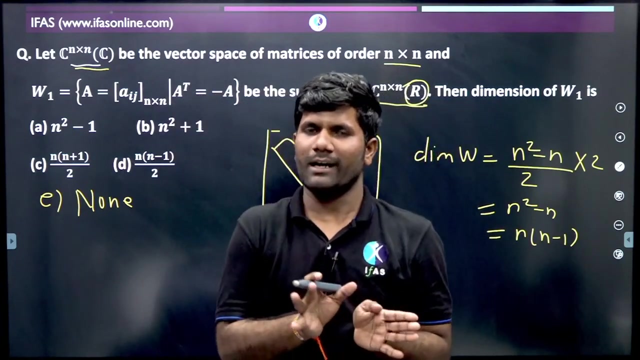 So once you comment, So let's move ahead. The next question is waiting for you. Ok, The same. It will run till about 2.5-2.5. Ok, Until the questions are over. MSSET is an exam of Maharashtra SET. MSSET means Maharashtra SET. 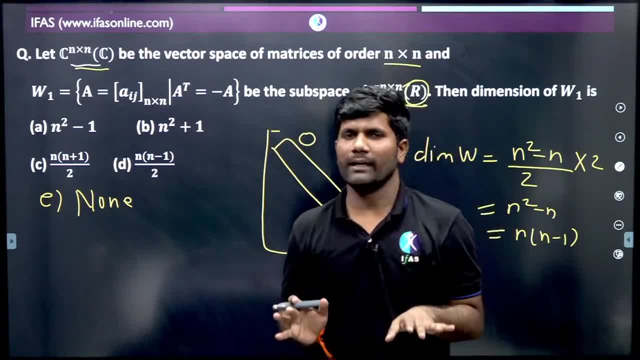 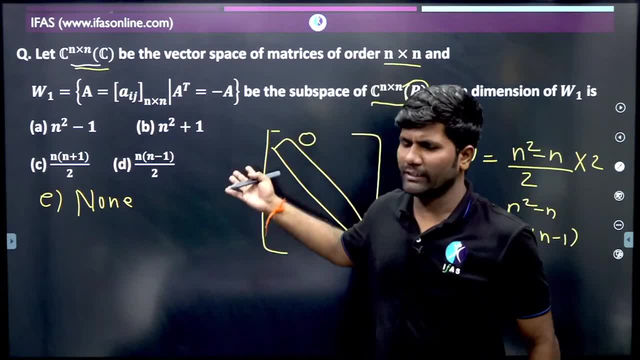 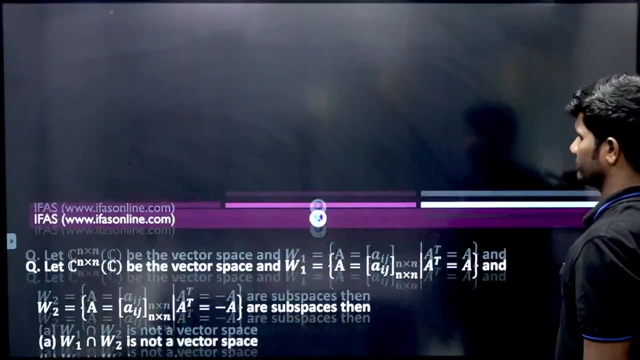 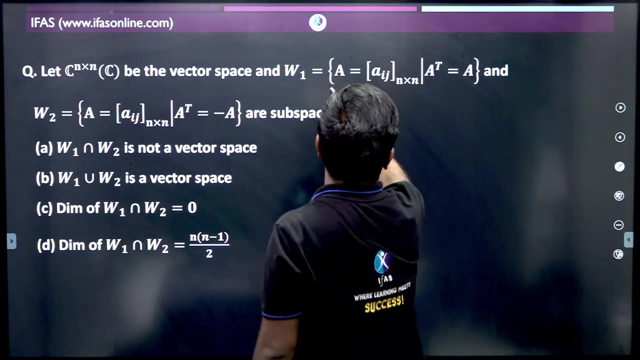 State eligibility test is done. It is passed. People become assistant professor in Maharashtra. Ok, Linear Algebra is asked everywhere. Let's come to the next slide Now, what have we been given here? Let C and C be the vector space. What is given in W1?? 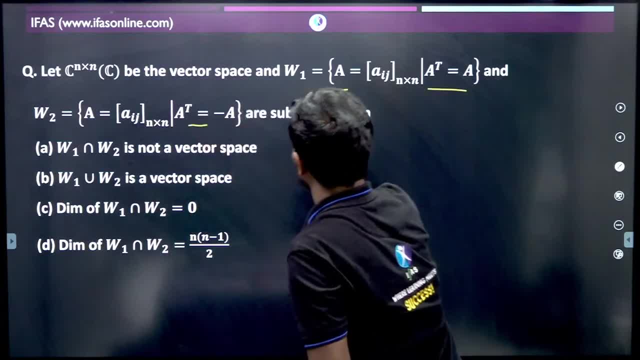 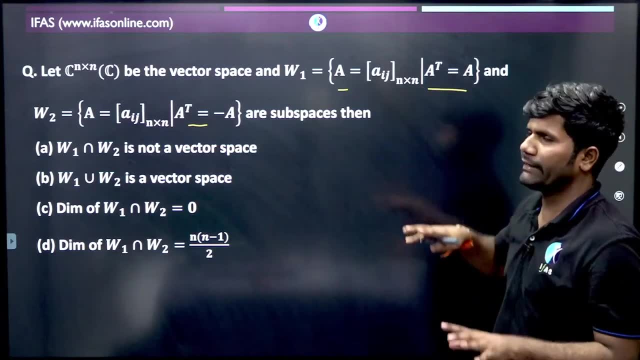 SET of all symmetric matrices And, in W2, SET of all skew symmetric matrices. Now tell us Which option will be correct among these. So the first option is: Their intersection is not a vector space. Option B is, given that Their union is a vector space. Option C is, given that 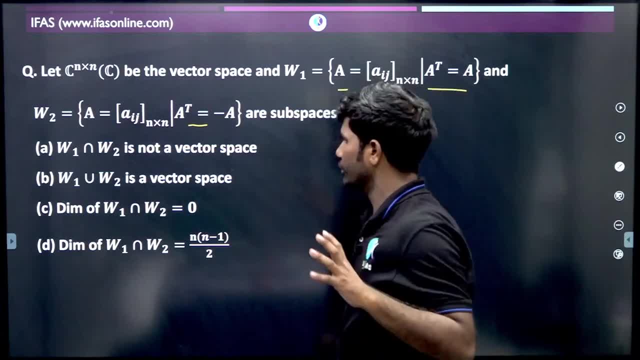 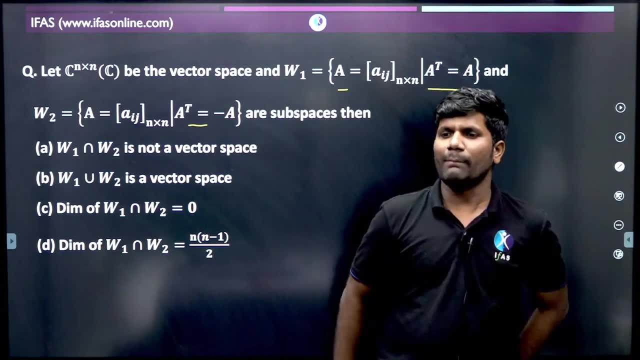 Dimension of W1, intersection W2 is equal to 0. And last option is: Dimension of W1, intersection W2 is equal to n, n-1 by 2. Now you have to tell What will be correct among these. So you guys scroll and tell. 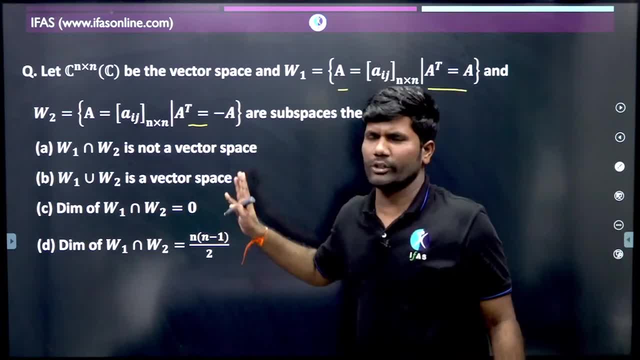 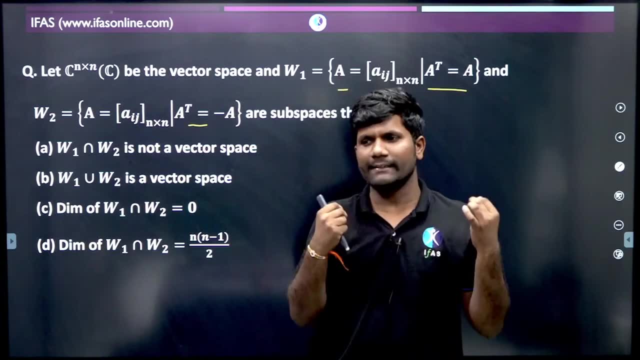 What will be? Just check once. See W1 and W2. both are subspace. So what is the hint for you? If W1 is a subspace, W2 is a subspace, Then their intersection will always be, But it is not necessary that there is a union. 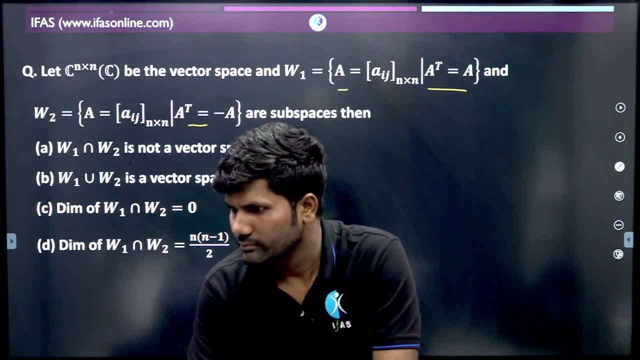 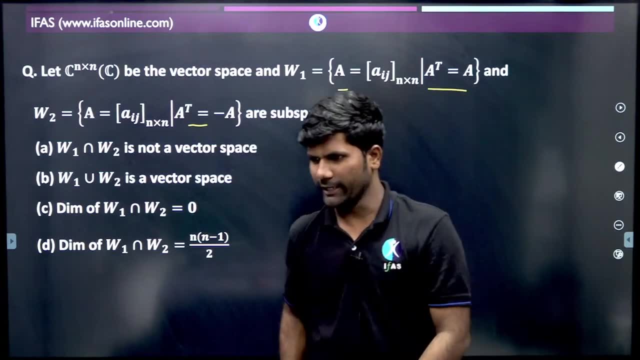 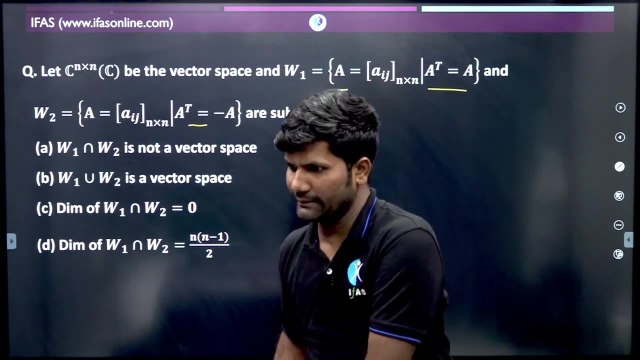 Okay, Keep this thing in mind. Yes, it is done. State people only give Okay. That too, if MSC is passed Or if MSC is in the second year. Okay, What did the rest of you get? Jyoti Dhimansi Smita. 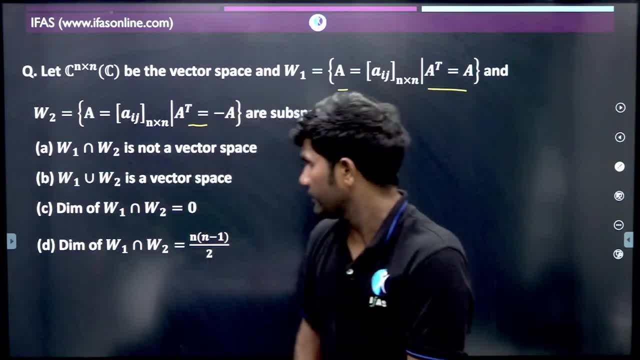 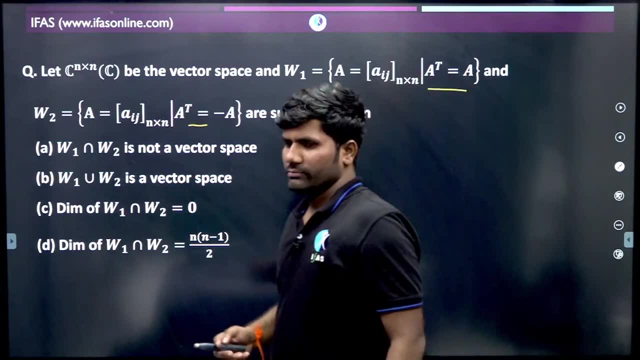 C Vivek Priyadarshi, C Seetal Jamdade, C Okay. Almost everyone is saying C Okay. Tell me one thing: We have done a result. What does the result say? If W1 and W2 are subspace, Then their union is not necessary. 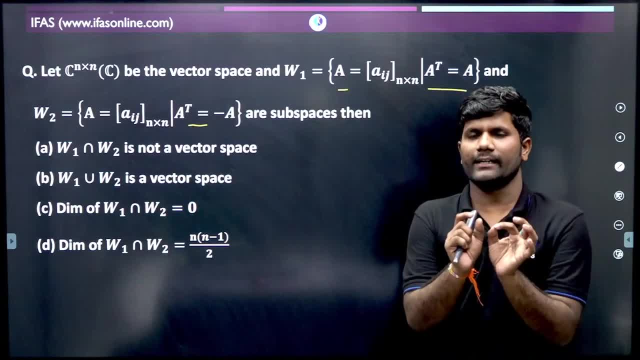 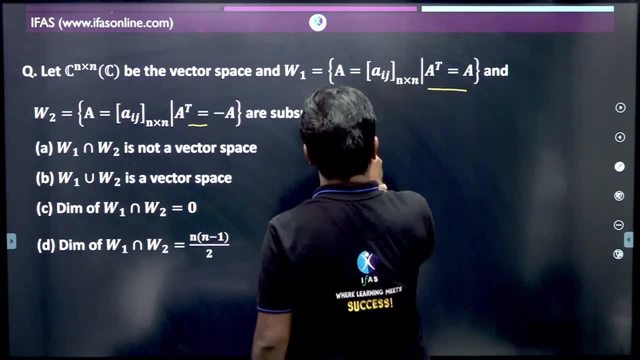 But intersection is always a subspace. Okay, So here you can write a note. What does the note say? So write down note. Note says here: First note: If W1 And W2 Is Subspaces Of V, So write down note. Note says here: 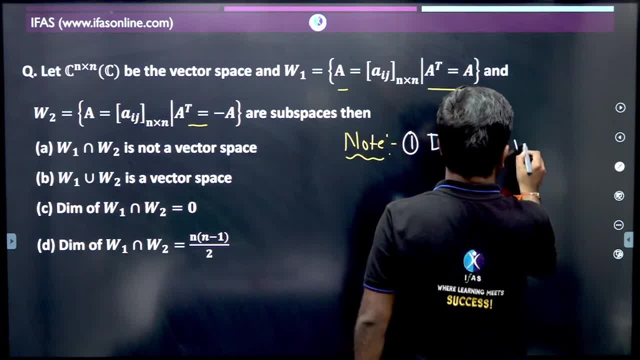 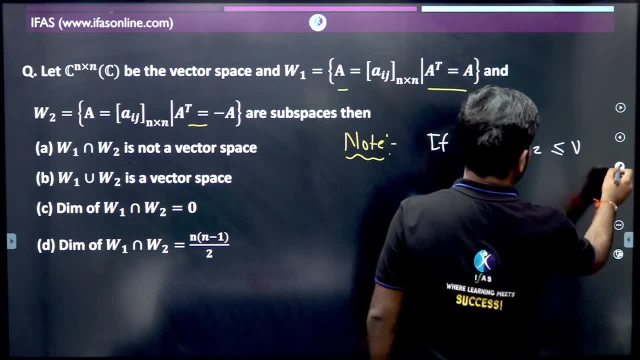 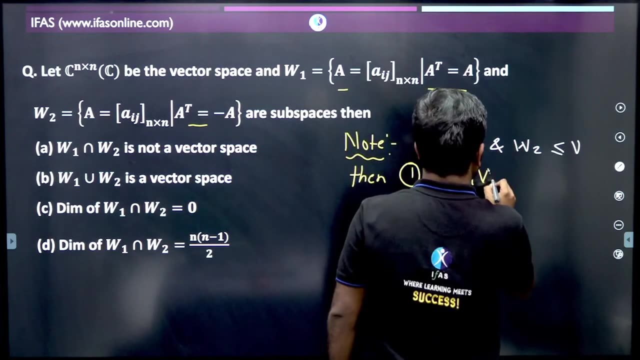 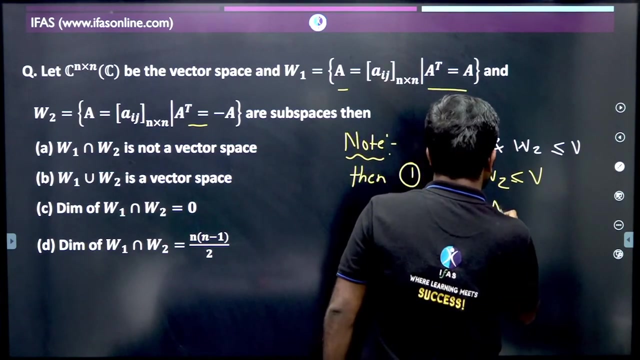 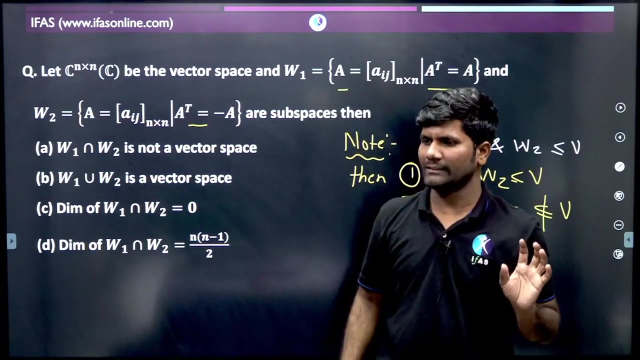 First note: If W1 And W2 Is Subspaces Of V, Then Then First note says W1, Intersection, W2 Is Always Subspace Of V. But Second note says W1, Union, W2 Is Not Necessarily A Subspace Of V. Remember this. This is not necessary. 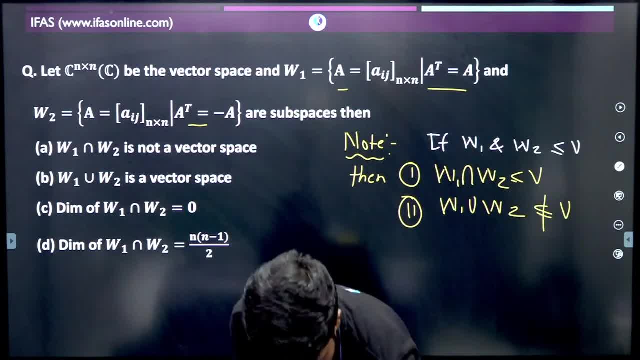 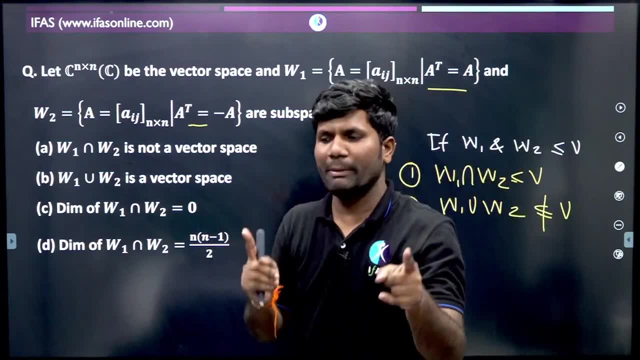 Okay, Now, here you have two results. Now tell me one thing All of you solve and tell me Which matrix belongs to the intersection of W1 and W2. What do you think So quickly solve and tell me? If you have not liked the session yet, Then first of all, 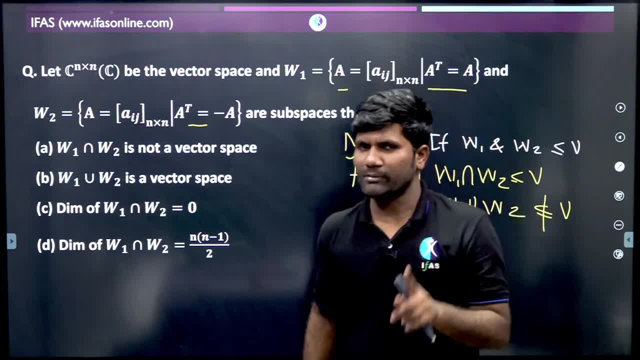 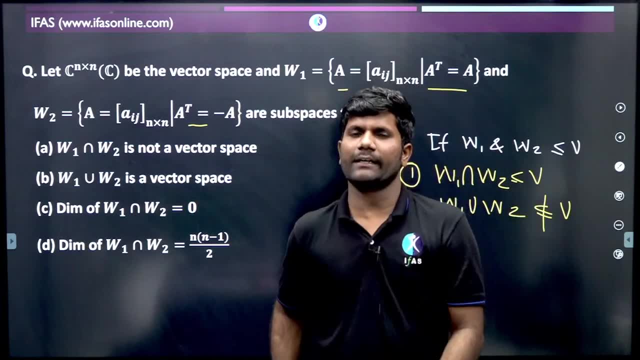 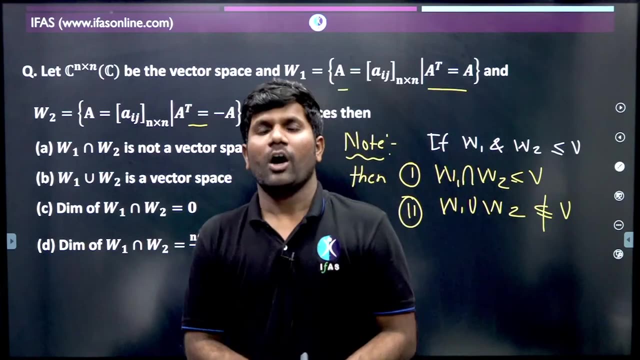 Like: If you are new to our channel, Then subscribe to the channel. Turn on the notification bell. Okay, If you are preparing for PSRNet, Then our offline batches are starting from 1st October And From 23rd, Online batches are starting. Today's batches are starting from today. 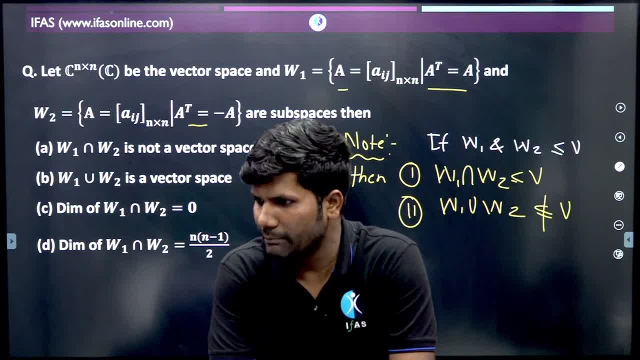 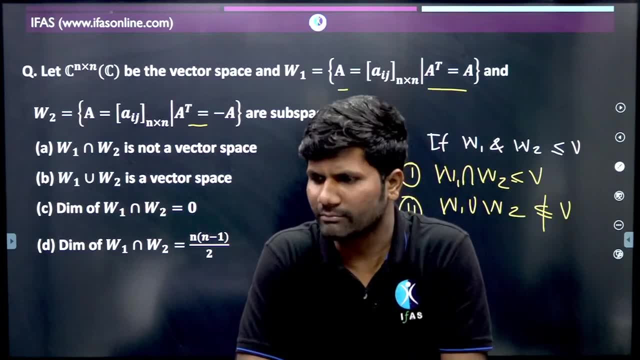 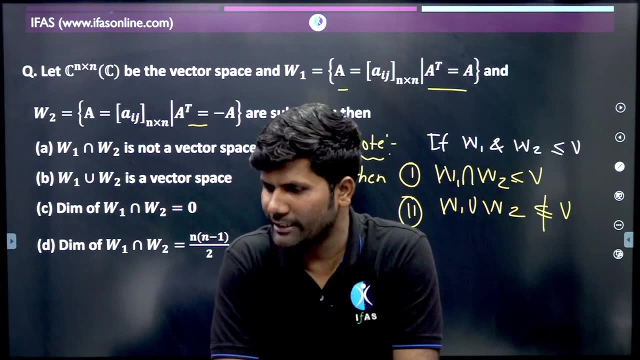 Okay, Where is Arsane B? Priti Nishtaneshi is speaking. What are the other people getting? Tell me one thing: All of you have not liked it, yet I am getting to know. Dilip Vaghmode says Zero matrix. Very good, Dilip. 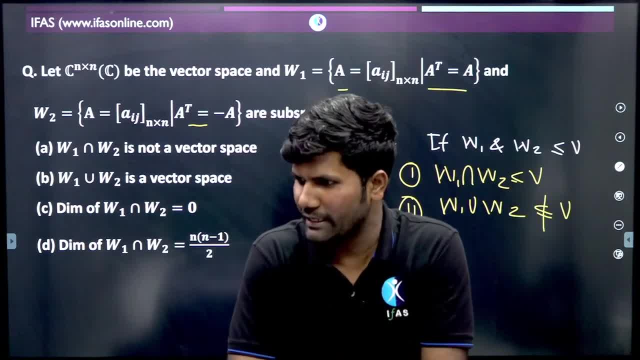 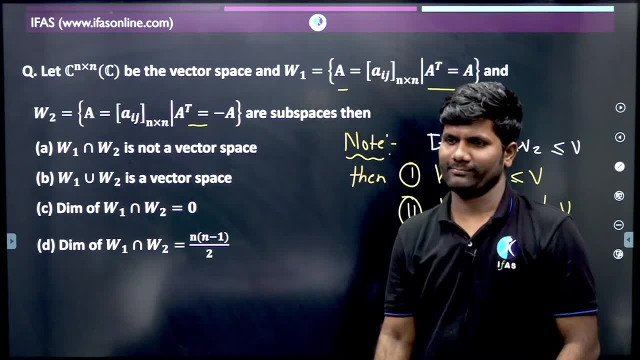 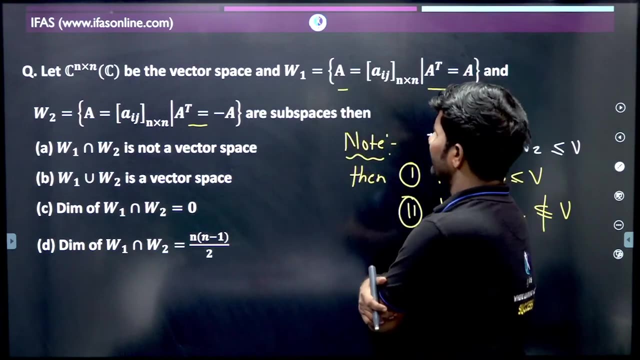 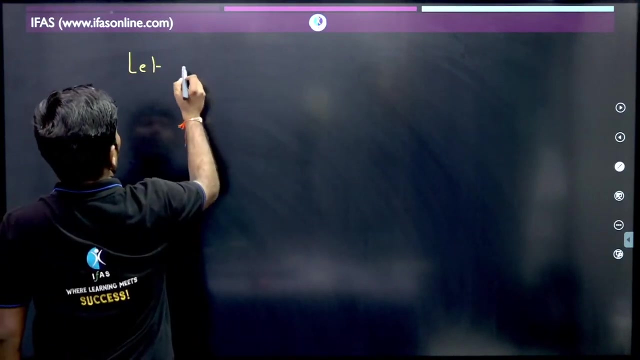 Inspire Maths: Zero. Jatin Jigar Zero. Kia Zero, Ismita Devnath B Zero. Very good everyone. So let's show it once. Suppose you have taken a matrix, For example. I am telling you, I took it in their intersection, So let Let A. Where does it belong? 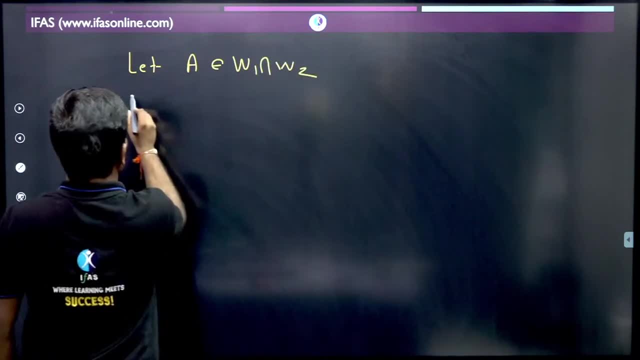 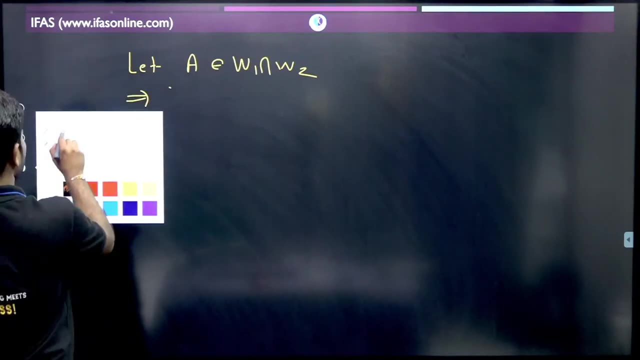 W1 Intersection belongs to W2. If it belongs to W1, It means What can I say here? W1 and W2, Both properties will be satisfied. So here I can say: A belongs to W1 And A belongs to W2 If A belongs to W1. 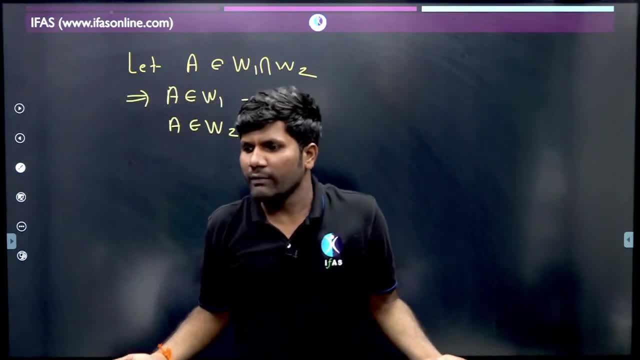 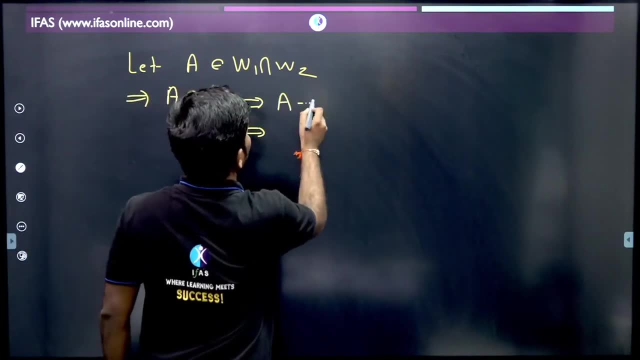 It means W1's property will be satisfied. What is the meaning of satisfying the property of W1? W1's property To satisfy means A is the same as A. transpose Now here. The second thing is: A belongs to W2 If it belongs to W2. 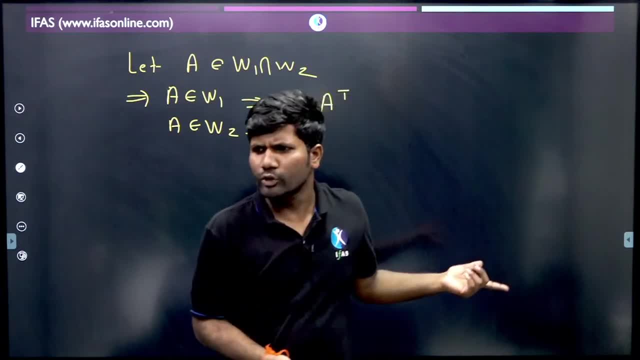 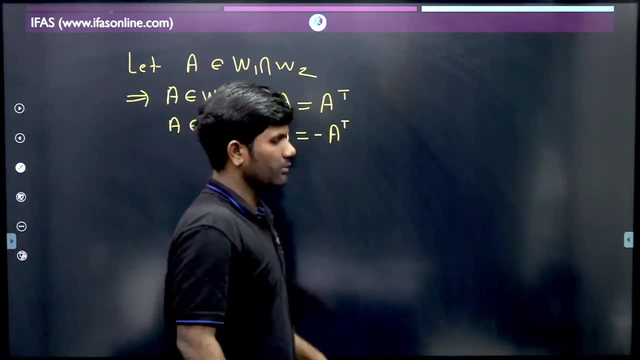 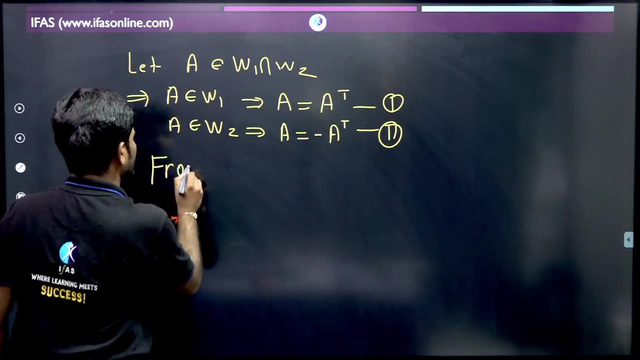 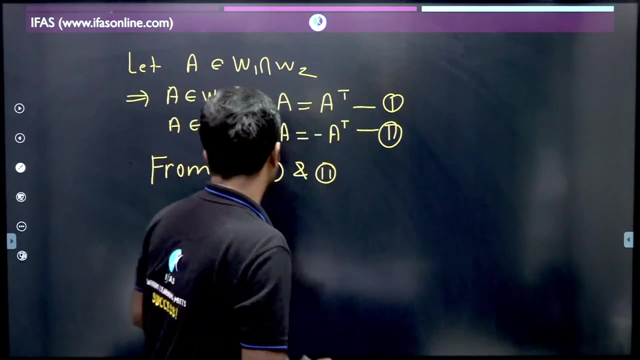 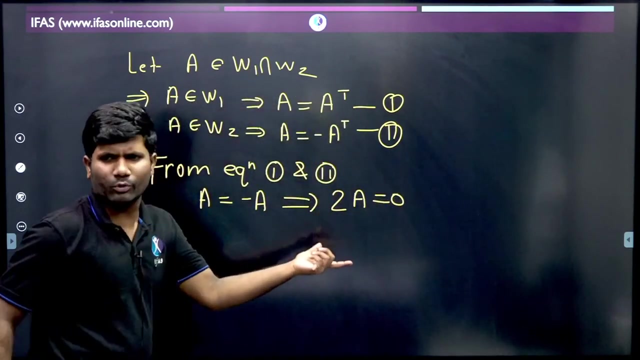 What does this mean? What would it mean? This means W2's property will be satisfied, satisfy. So here we can say: A is same as minus time A transpose. Tell me one thing Now from here. suppose this is equation 1 and equation 2. So from equation 1 and 2 we can say that. So from equation 1 and 2, what can we do? From equation 1 and 2 we can say that A is same as minus A. If A minus A is equal to 2A is equal to 0. But here 2 is not 0. If 2 is not 0, then what does it mean? 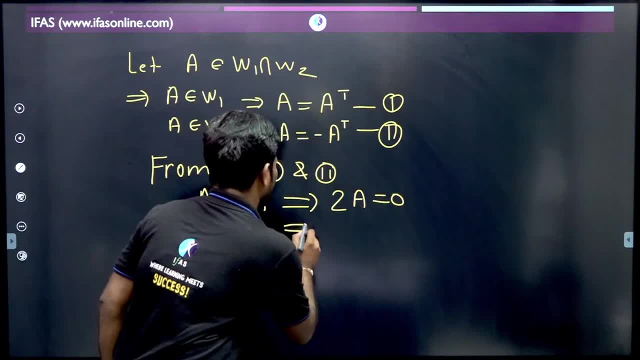 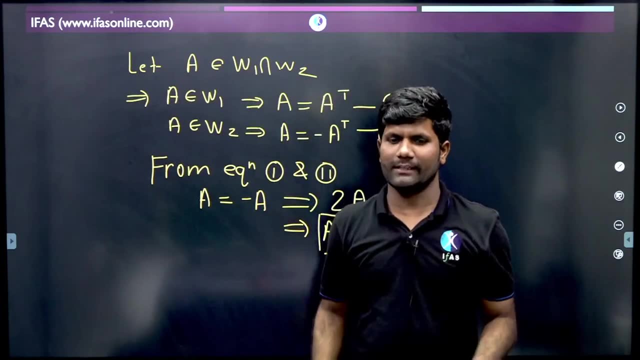 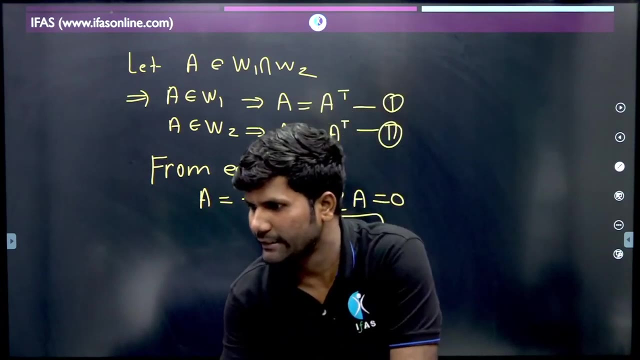 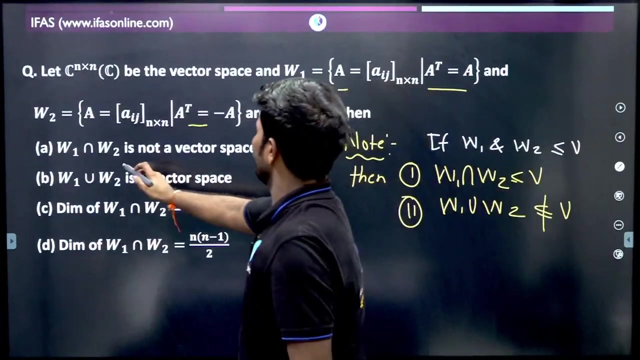 It means that A is 0.. So it means that A is 0.. So here I have taken an arbitrary matrix which belongs to their intersection and finally I have shown that A is 0 matrix. A is such a matrix that it is 0 matrix. Okay, So let's come to the pre-evaluation. See here what is given first. Their intersection vector space will not be there. A is finished. 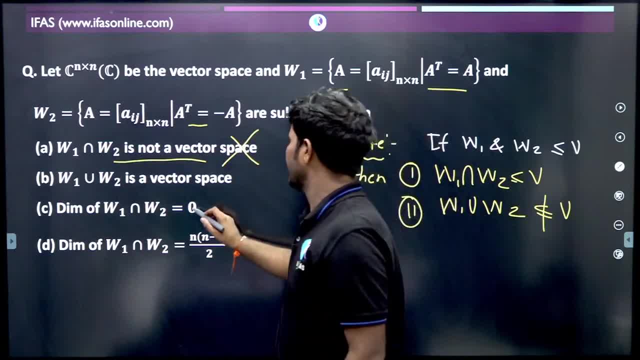 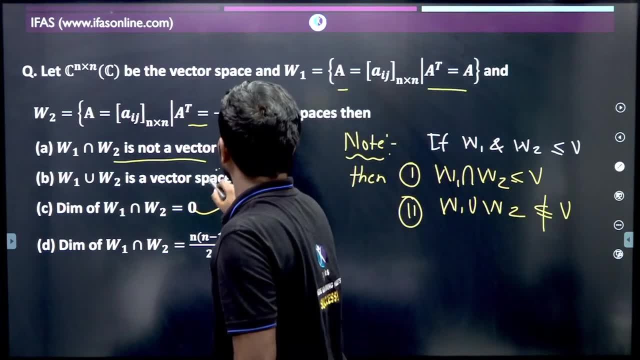 And in the intersection of W1 and W2, 0 matrix comes, It means that dimension A will be there. A is finished Now, union is not necessary that it is subspace. So for this, what you have to do, You have to find counter example. Okay, So clear. 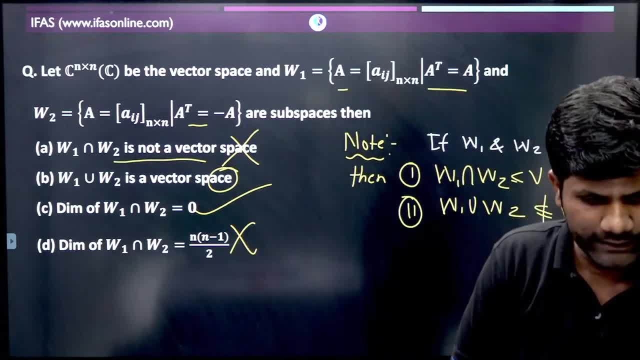 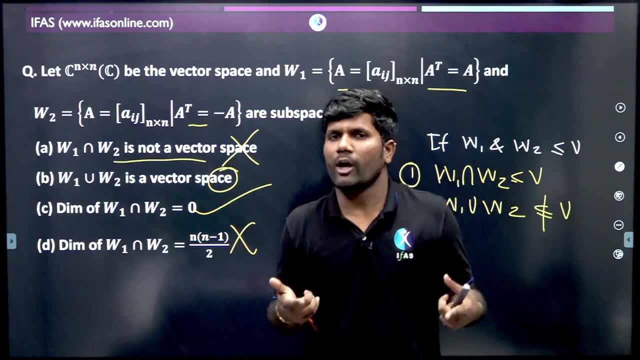 Did everyone understand till here? Once you tell me If it is clear, then I will move forward. Okay, So what to do in this way? You have to think about every option. If any option is correct, then why is it. If not, then why is it not? 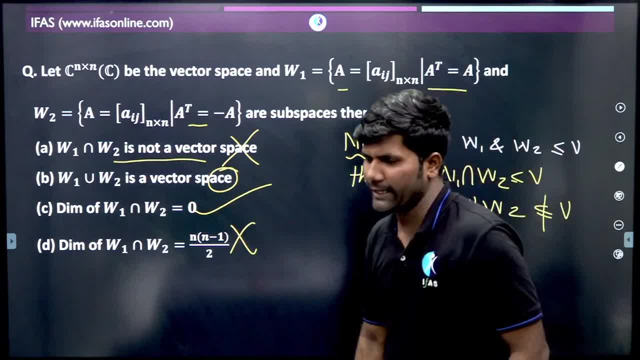 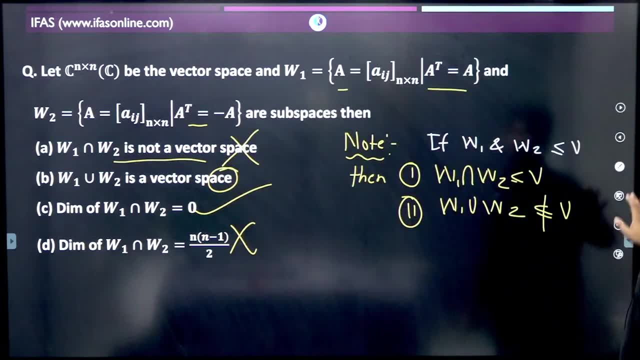 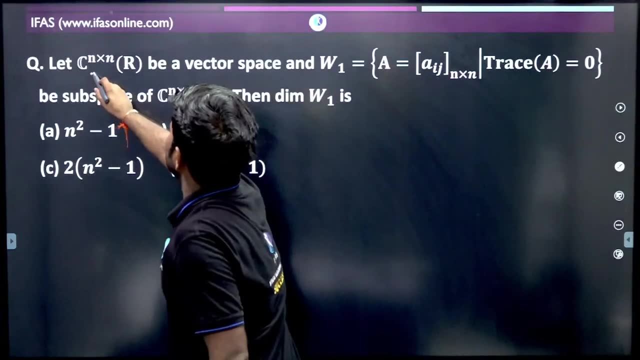 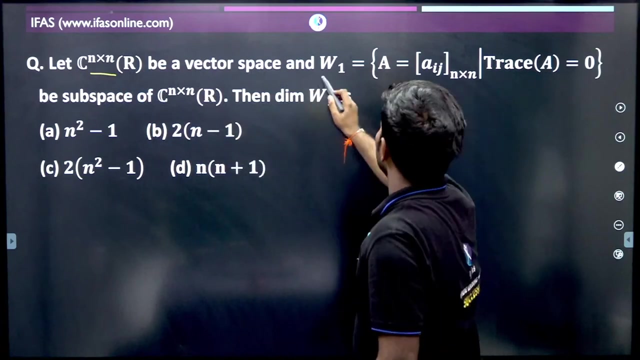 At least think here and go, Okay. So let's come to the next question. Now, here, what is given? It is set of all n cross n matrices and the entrance is the complex number. but field R is given. Okay, And WI? what is given? Set of all n cross n matrices whose trace is 0 and its subspace is 1.. Now tell us the space of W1. 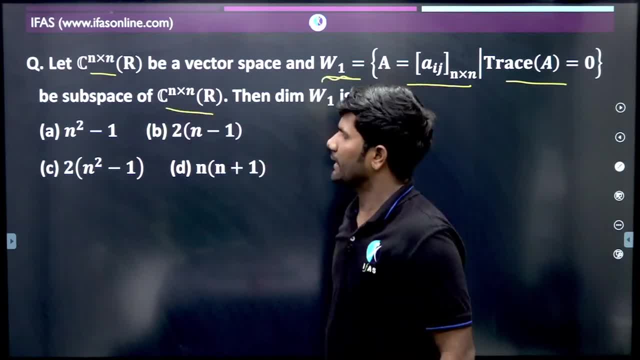 So W3. Let's have a look at that. So this is set of all n cross n matrices. This is set of all n cross n matrices and this is the sub space of W1.. Now tell us the space of W1.. 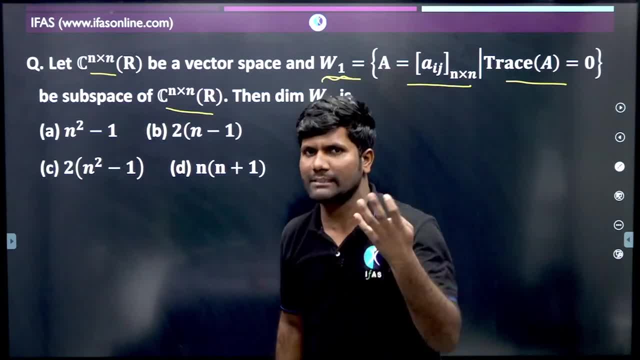 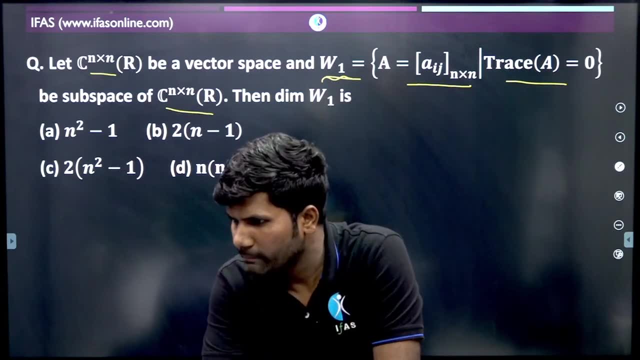 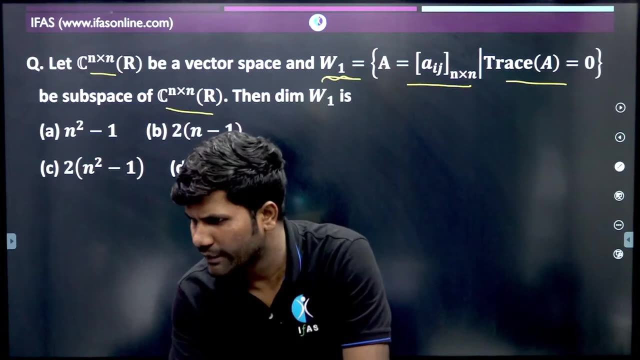 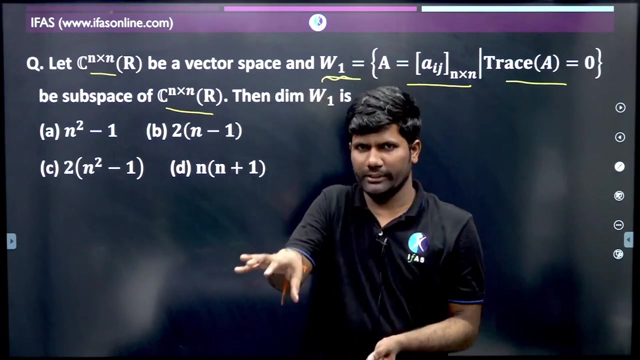 what will be the dimension of vector space? so for dimension of W1 we have four options. now you have to tell me the correct one. ABKarim is asking that, sir, can basis be vector space itself? see, basis is the subset of vector space. when vector space is formed by linear combination of basis elements. 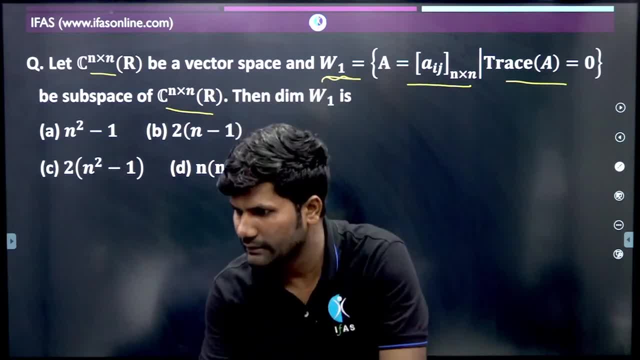 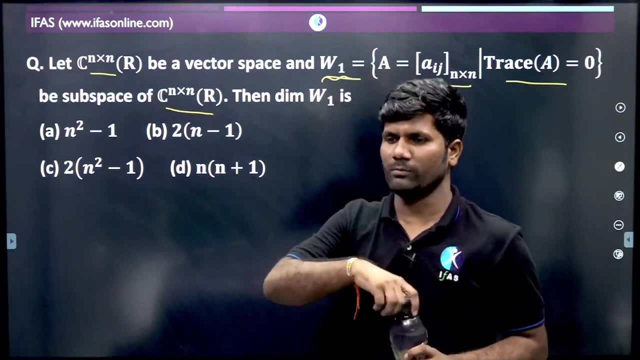 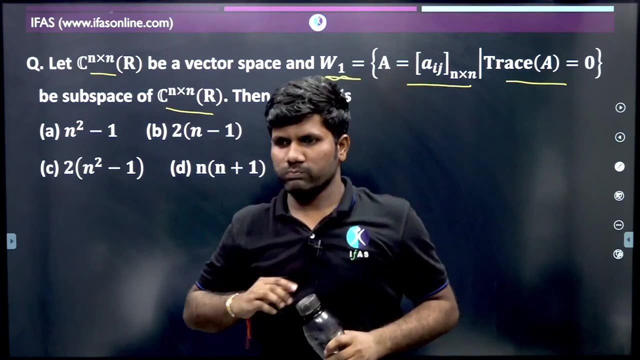 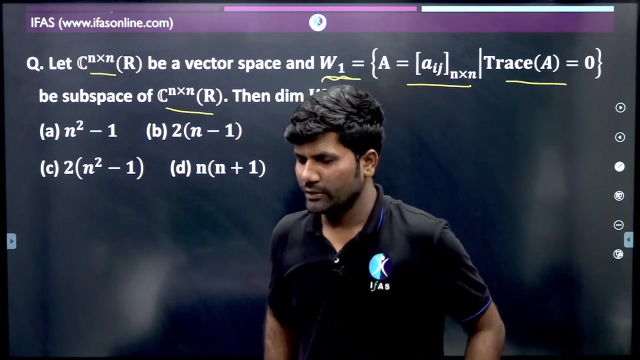 so basis is the subset of vector space. now tell me the correct answer of this. everyone solve it. and tell me what is the correct answer. all students solve it. Pulkit has told what other people are doing. Deva has also told, Smita has told Vivek. Priyadarshi has told. 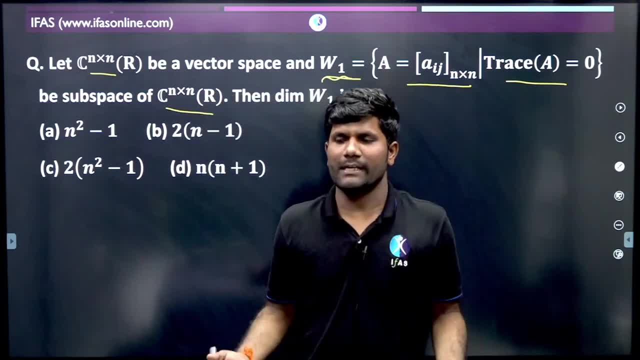 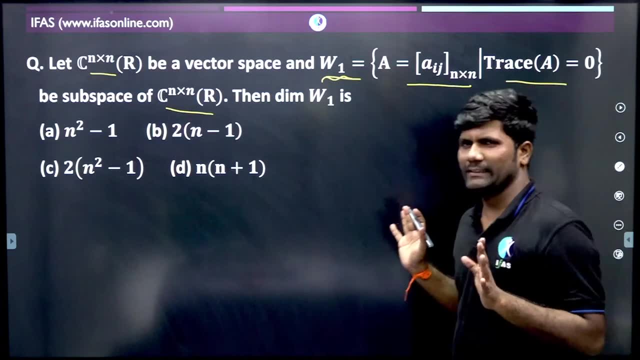 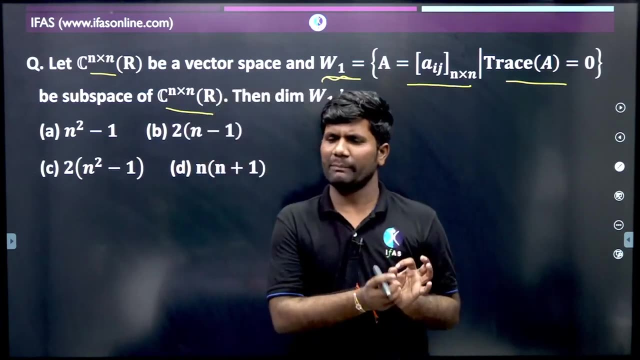 Nikita has told rest of the people. tell me what will be the answer. very good, Sital, Nikita, Vivek. very good. problems will come in the same set exam. they will not be of very high level. you can solve it easily. so, on the basis of dimension, 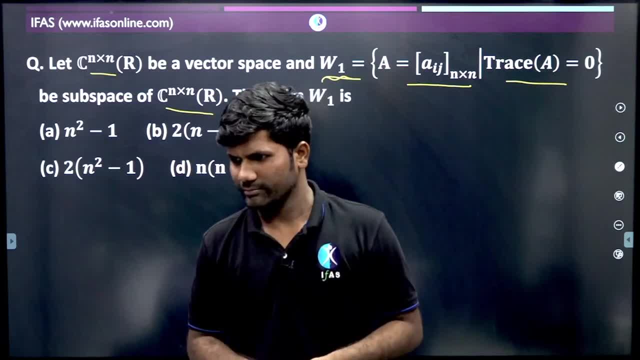 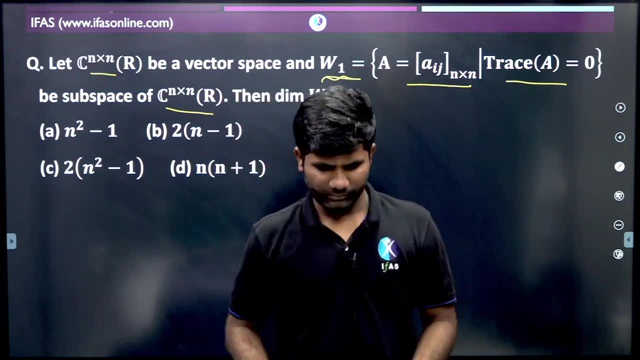 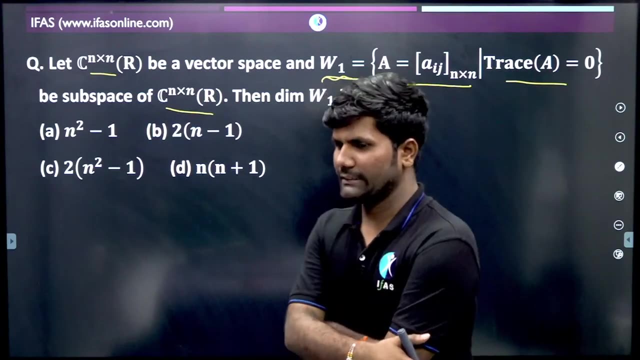 one or two questions will come every time. Ganesh Thackeray is saying that C will be the answer. ok, Ganesh, Ganesh, where are you now? ok, come on now tell me one thing. Amruta is also saying that C will be the answer. very good, Amruta. 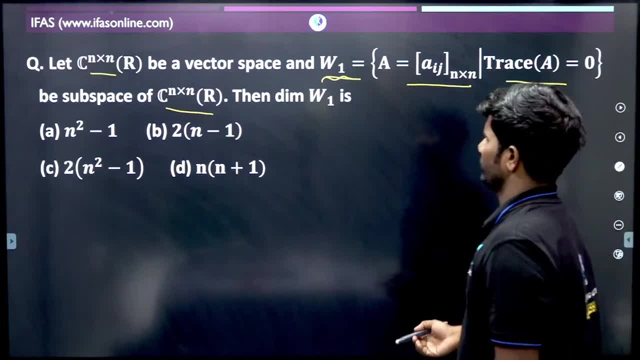 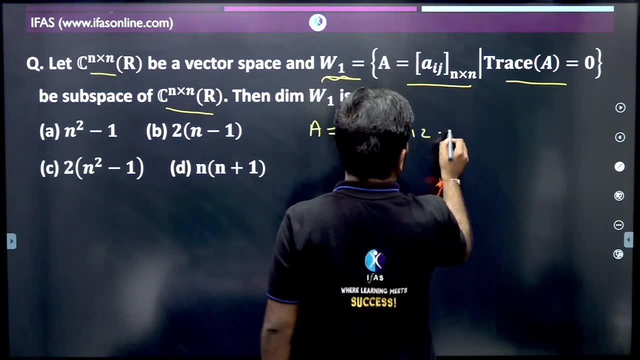 now see here: in W1 there is a matrix whose trace is 0. so in W1, how is the matrix of W1? matrix will be like this: A11, A12 and so on, up to A1N will be there. what will happen here? A21, A22 and so on, up to A2N will be there. 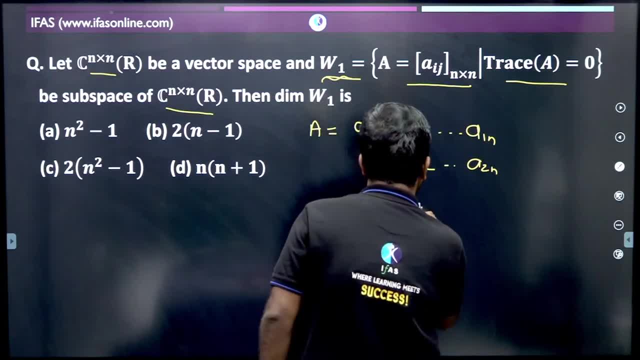 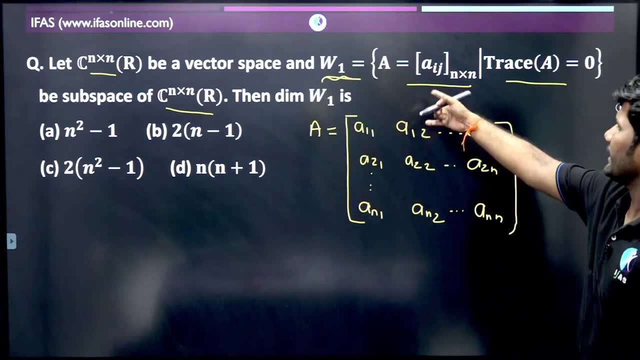 if we continue like this, then what will happen here? AN1, AN2 and so on, up to ANN will be there. ok, we got this matrix. let's assume where it belongs. if it belongs to W1. if it belongs to W1, what will happen if it belongs to W1? 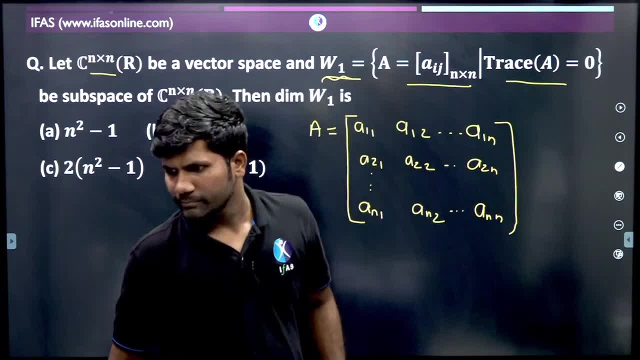 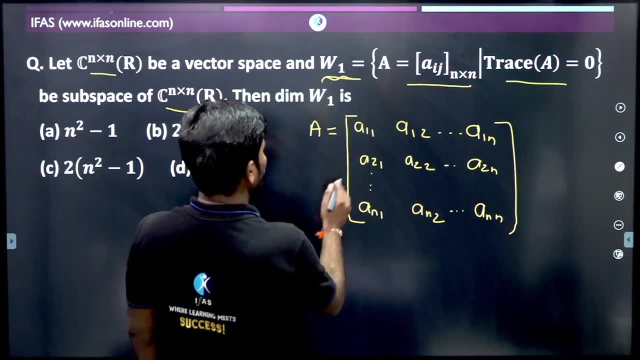 it means I can say here that what will happen? absolutely. this type of question also comes in the java. you will see, you will get it from the previous set. absolutely. so here I can say: what is trace of A is equal to trace of A is equal to 0. 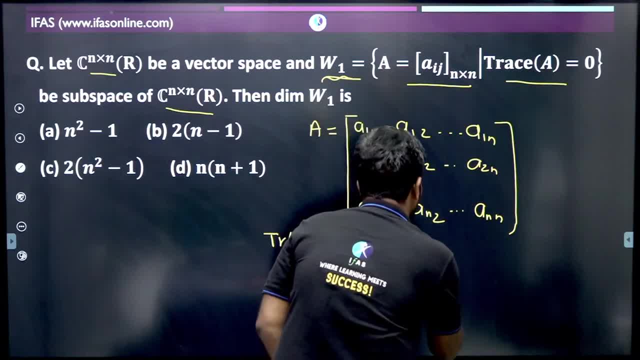 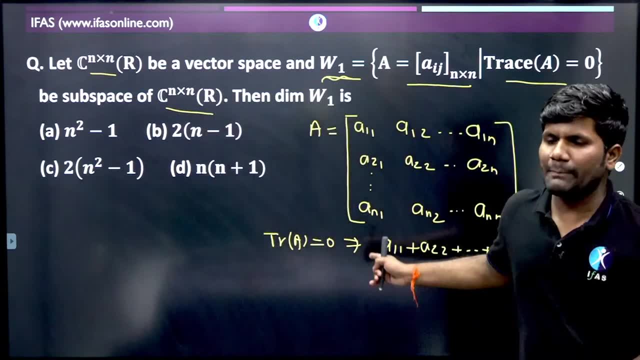 so this means I can say A11 plus A22 and so on, up to plus ANN will be 0. ok, now here, what can I do with any one element? I can write in linear combination of other elements, so let's write. so how will I write here? 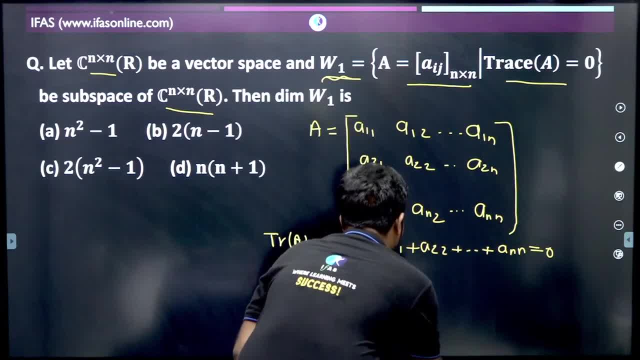 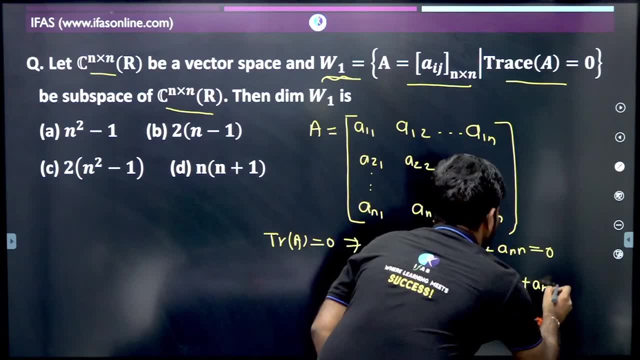 take any one element. suppose I took A11, so A11 can be written as minus times remaining element, that is A22 plus and so on up to ANN. ok, now tell me one thing, now what we have given. we have to generate CN, cross N over R. 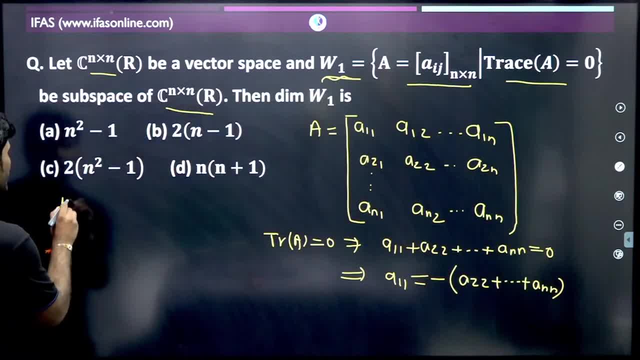 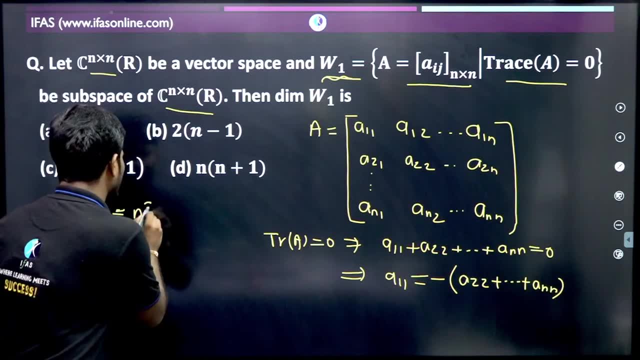 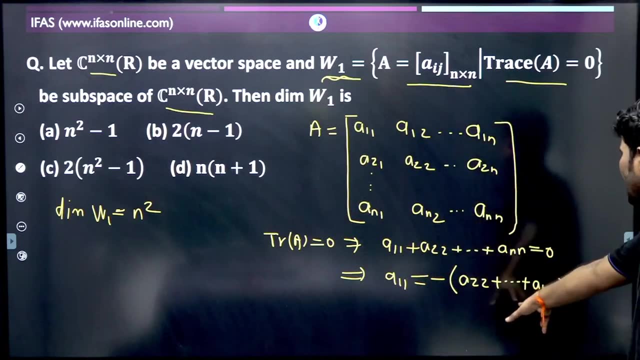 now here in matrix, if I want to find its dimension, so dimension of what will be W1, what is the total element? total element is N square, ok, N square, but in diagonal. in diagonal, to generate diagonal, we need one element less, we need N-1 element. 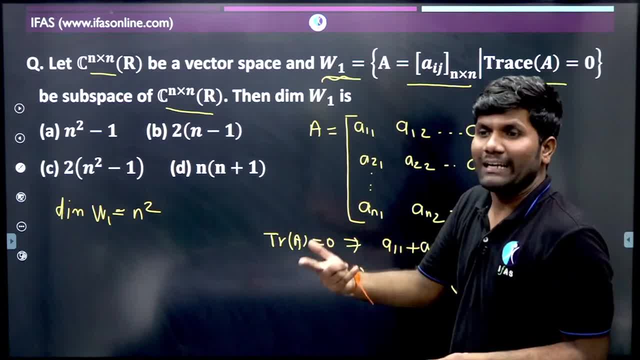 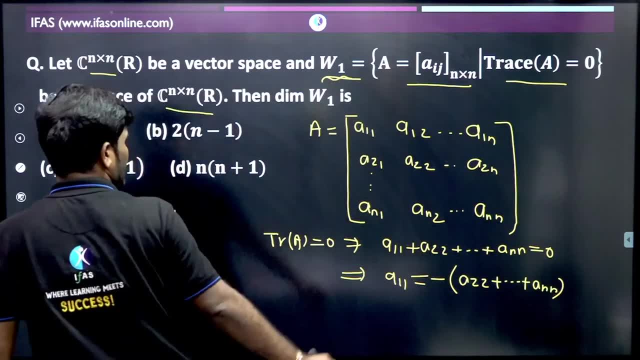 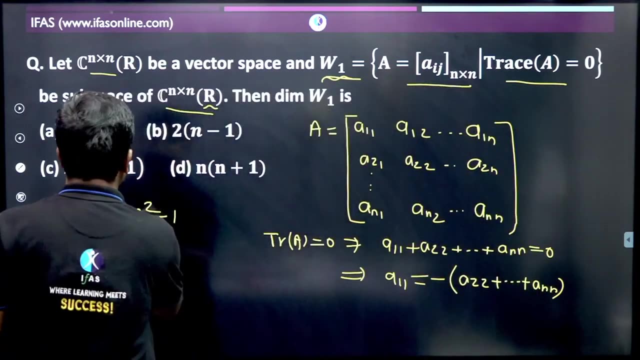 because in other linear combinations we can write ok. so here, what will I do? I will minus one element, one element. what I did, minus its dimension is over C, but what is given here over R is given. over R is given means what you have to do now: you have to multiply it with 2. 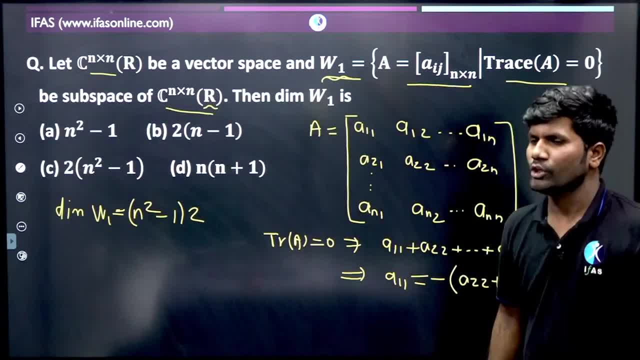 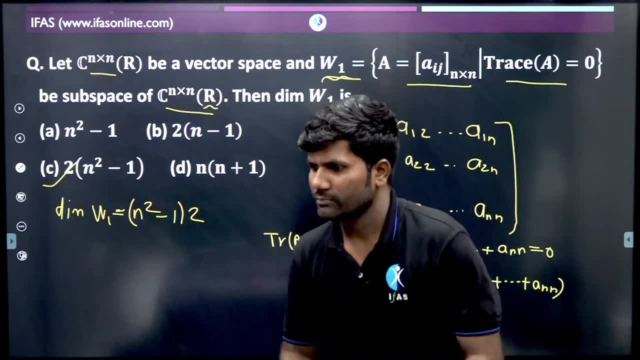 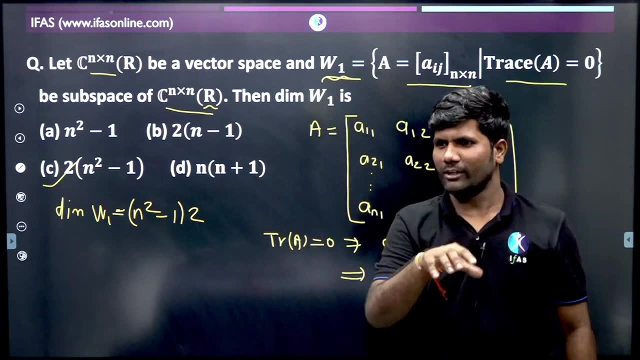 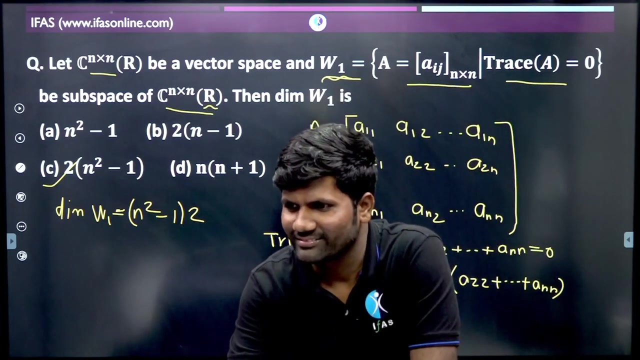 so as soon as you multiply with 2, you will get correct answer. so what will we get? correct answer. so here we will get correct answer. option C: ok, is everyone clear? ok, the question was: ok, perfect, perfect, perfect, perfect, ok, ok, yes, ok, ok, ok, ok, ok. 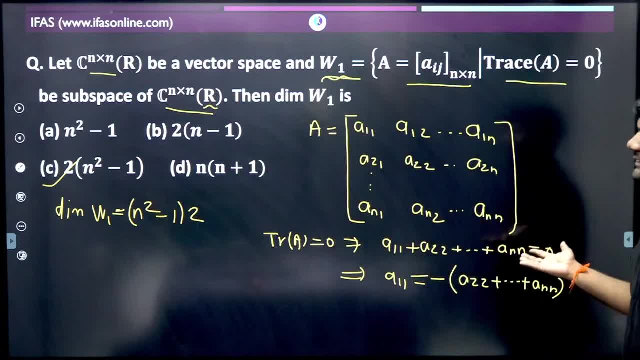 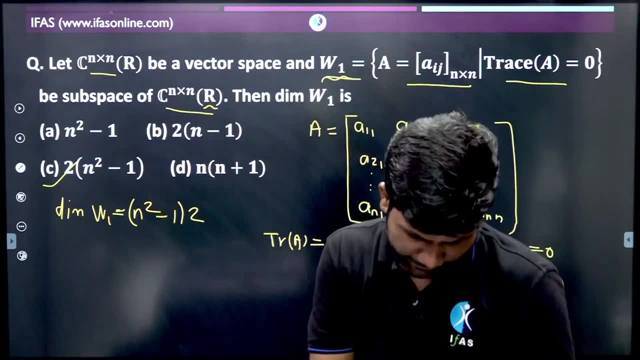 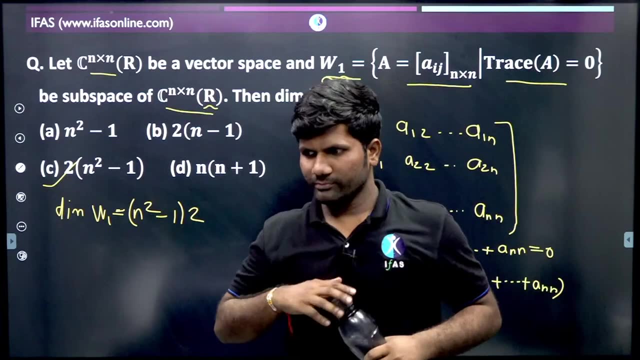 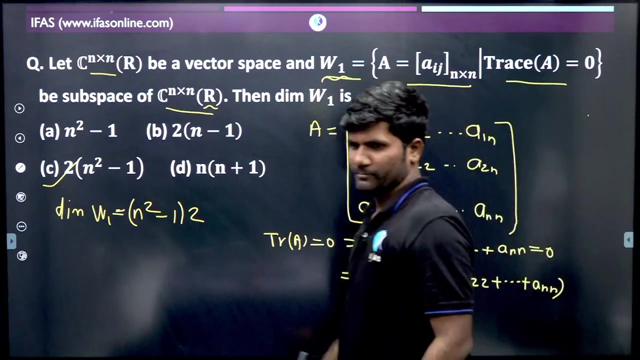 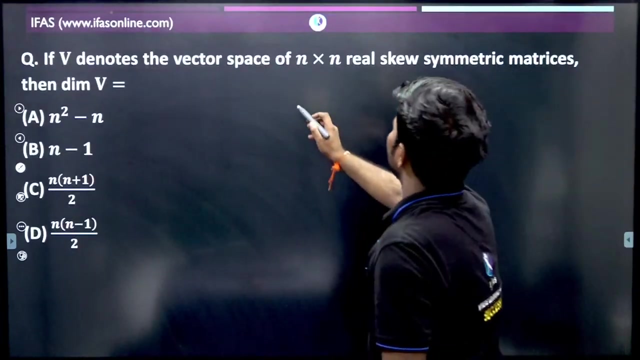 correct. ok, ok, ok, ok, ok, okay, ok, ok, ok, ok, ok, ok, ok, let's assume this is coming to you. let's move ahead now. what we have given here is: let V be a vector space of all n, cross, n, real skew, symmetric matrices. then dimension of V: 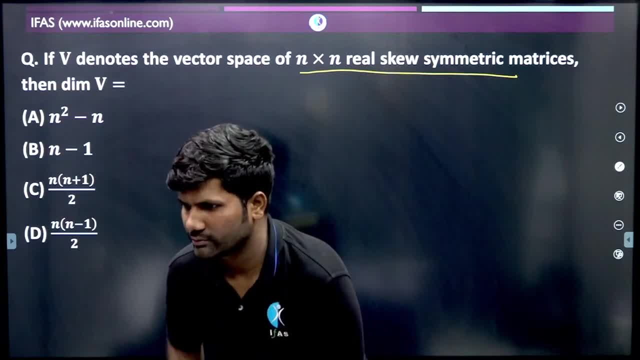 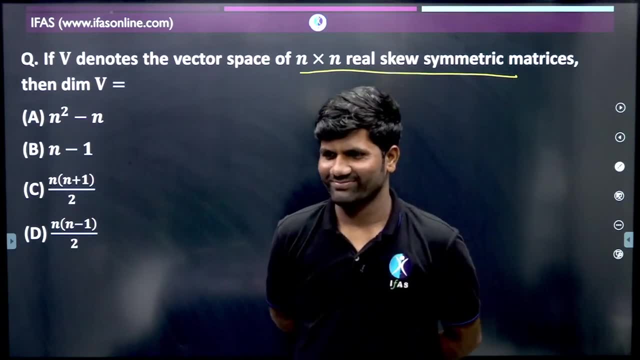 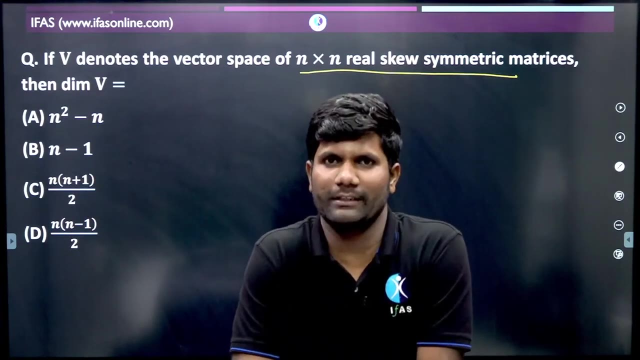 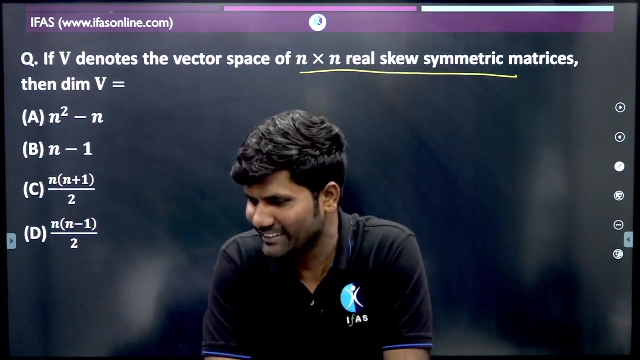 now it is very simple: you have to tell ok. ok, I understood. thank you, Vivek. thank you, ok. actually, what happened is that Vivek's likes were less than what he said. so what I said was: you sit back and come back as soon as you start seeing the proof, nothing else. 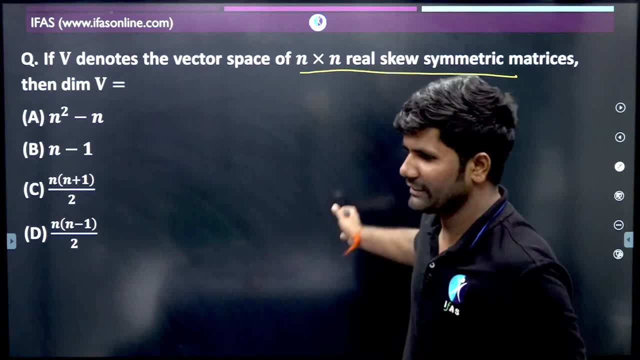 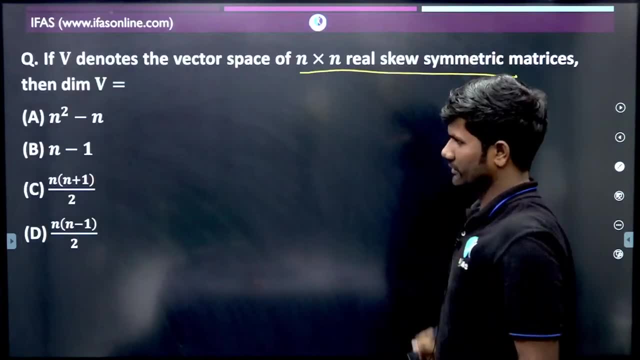 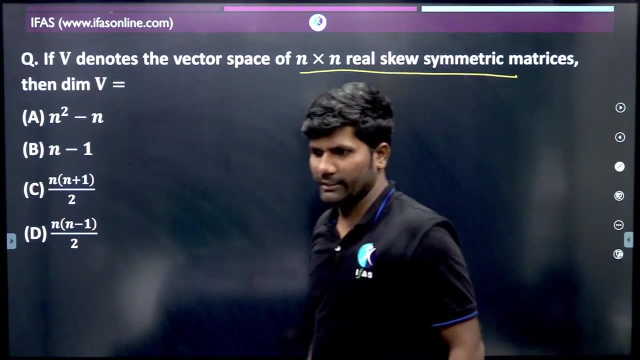 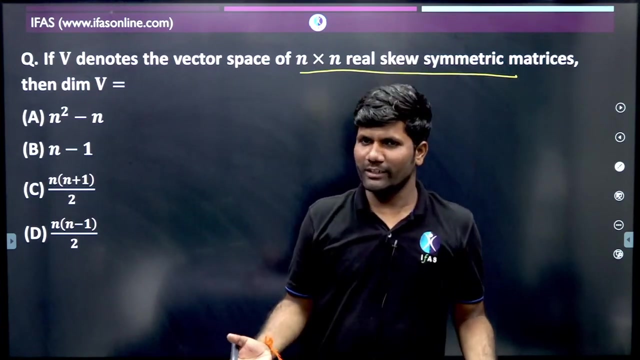 ok, Nandita, what did you get? tell me what you are getting from this. ok, I got it. I thought: what did I do? ok, tell me what is coming. ok, ok, that's the thing. no one is listening to you. he has asked you to like, so do it. 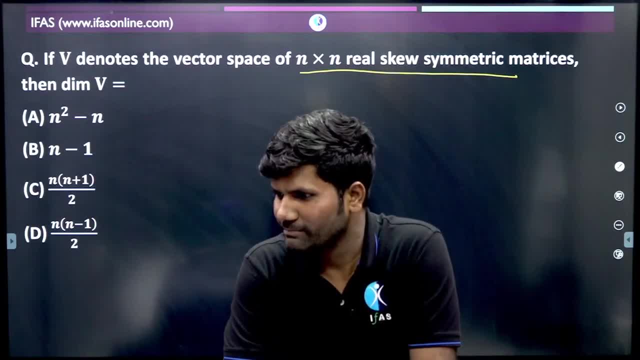 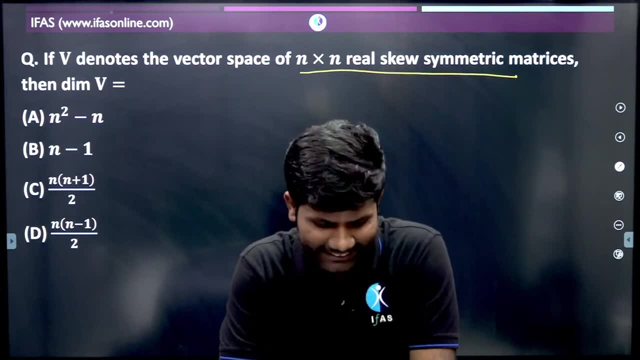 ok, ok. Ismita Amruta Tasleema, Vivek Priyadarshi. yes, that's why I told you, Vivek, once you go out and then come back, see when nothing happens, what is there in the app, what is there everywhere? 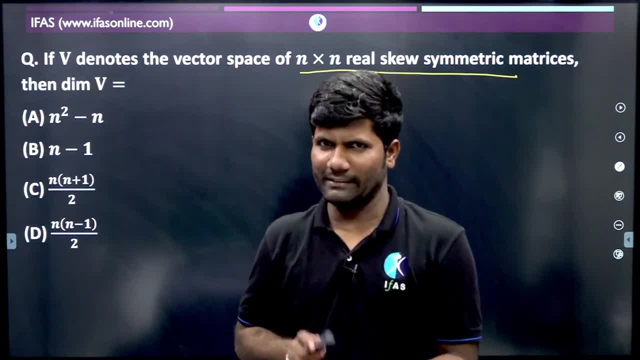 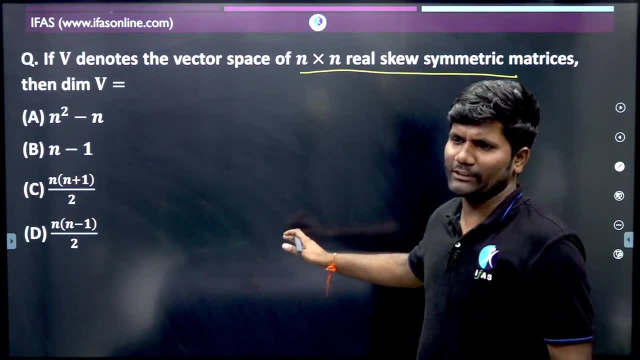 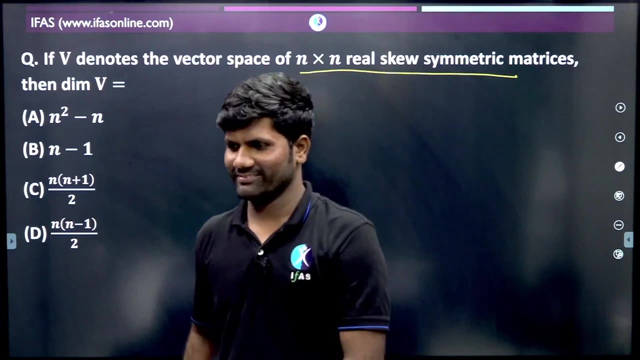 once go out and come back, like our remote gets damaged. then they beat us a little, like that it gets right. ok, come on, now you can solve this easily. no one came tell. tell you guys now what we did. we did this type at the start. 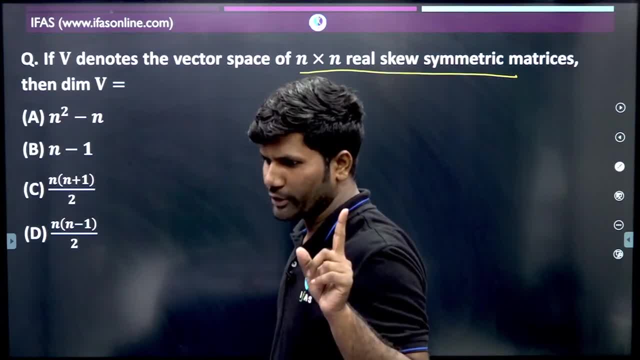 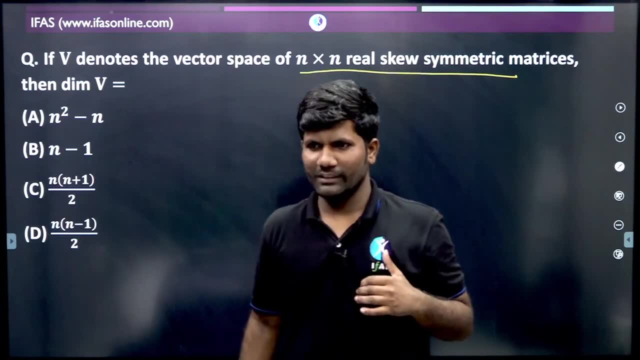 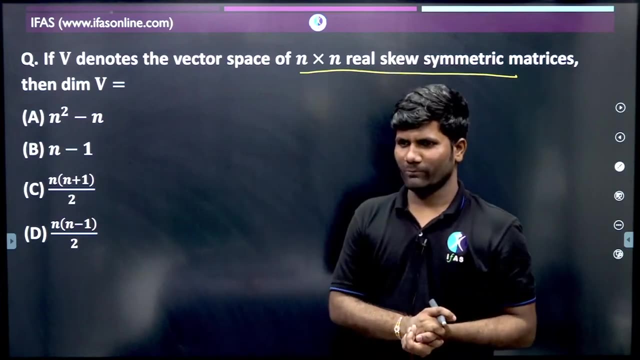 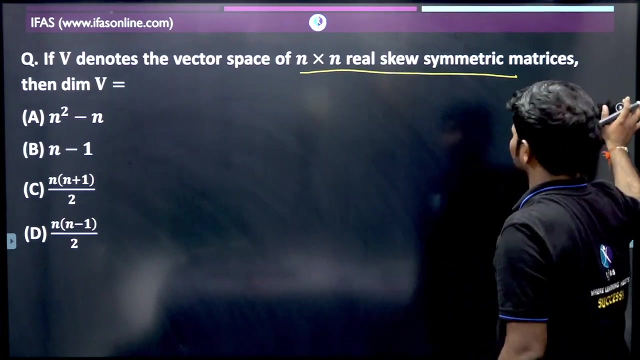 so all of you can do this. Mayuri Shonowne, is it clear? ok, we will meet with Linear in offline. ok, after some time. for whom, Sahil? tell me what exam are you talking about? tell me first now. what did we get here? which of the following? 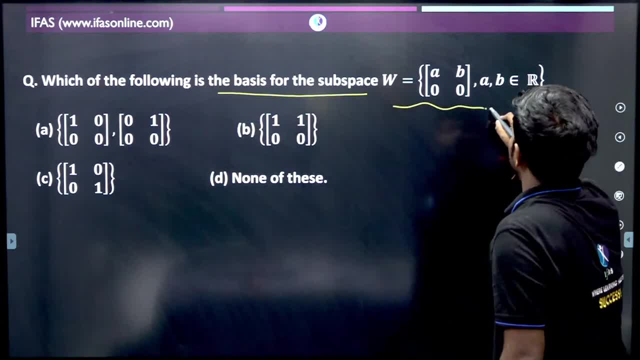 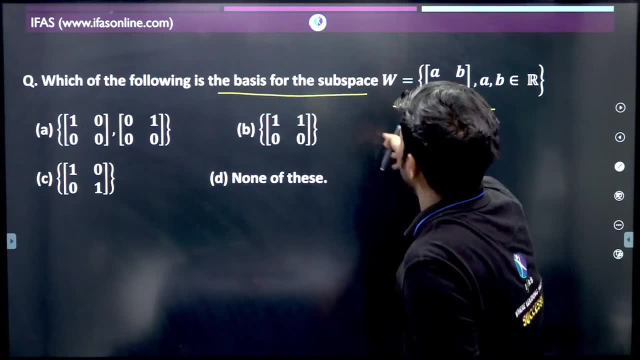 is the basis for the subspace. now we have given a subspace W. this is a vector space. what is a vector space? it is a set of all matrices. now you have to tell what will be its basis. now, there can't be a simple question than this. 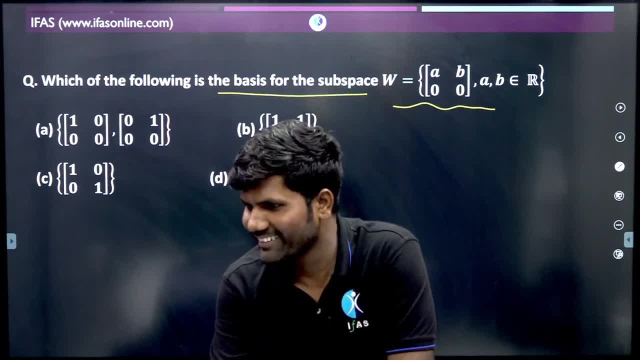 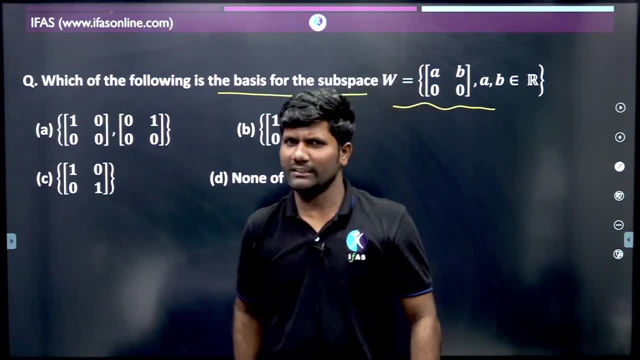 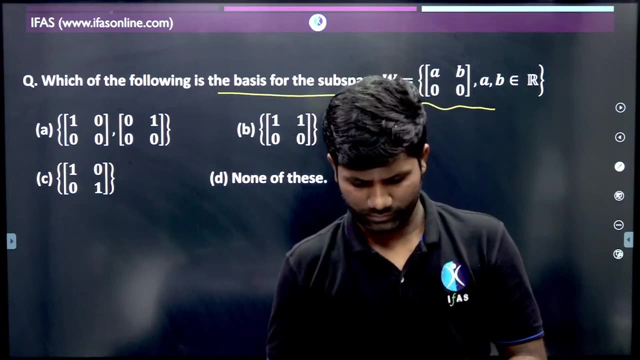 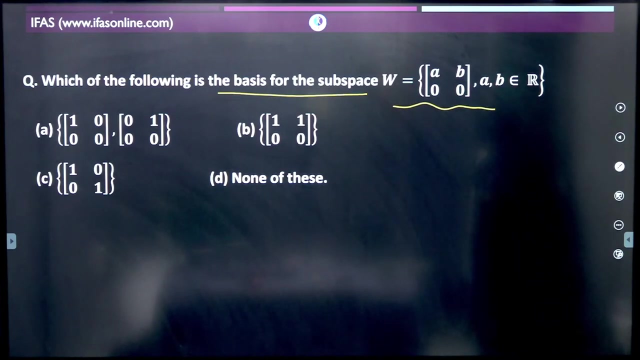 ok, tell Vivek, it's ok. once you read it, all the questions look easy. if you haven't read it, then all of them look like this: yes, I agree, ok, ok, ok, you are so good. ok, ok, ok, ok, ok, ok, ok. 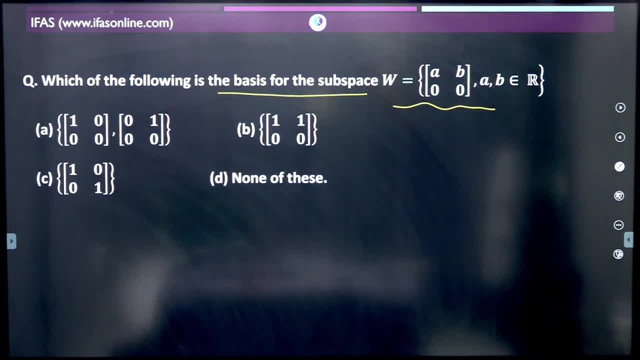 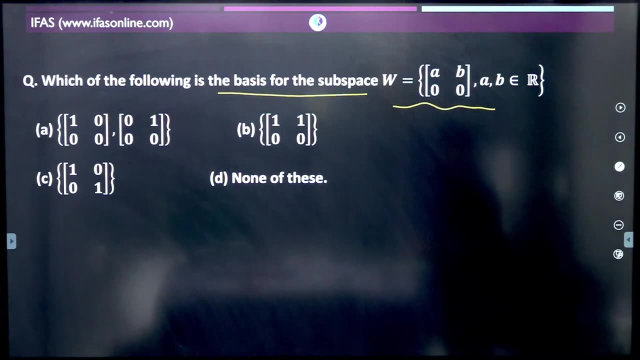 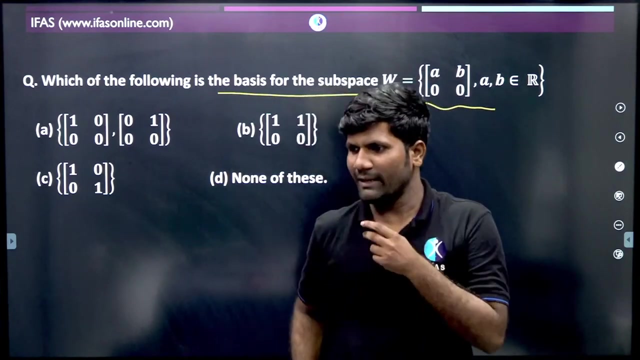 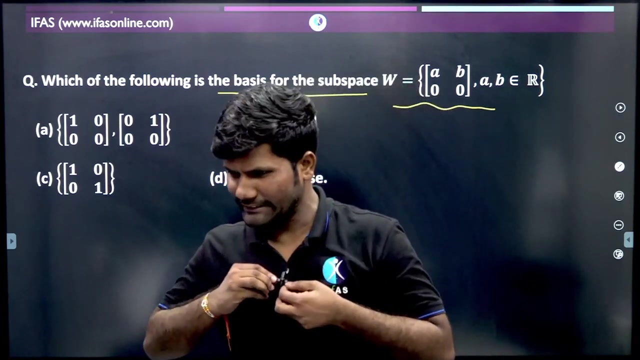 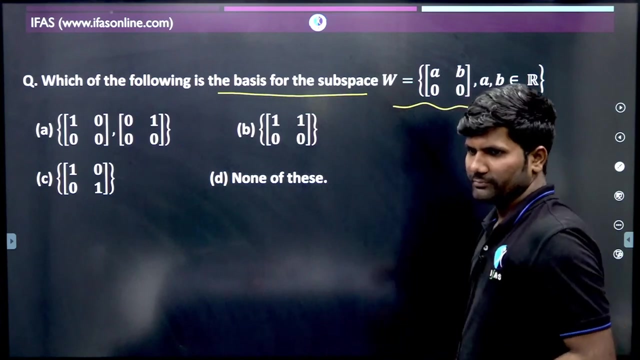 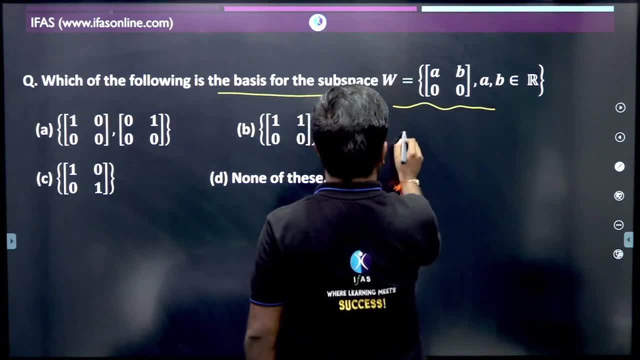 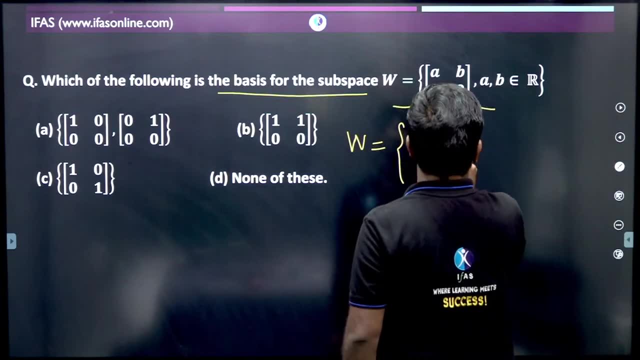 Find the basis of W. then how do I write W? see, what is W. what do I do once I take A as a common and once I take B as a common? now, if I take A as a common, then what did I get? 1, 0, 0, 0,. 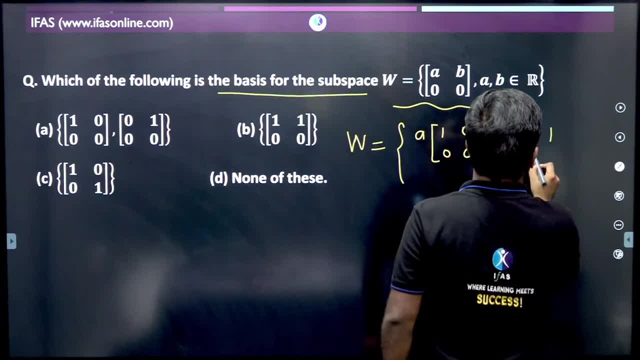 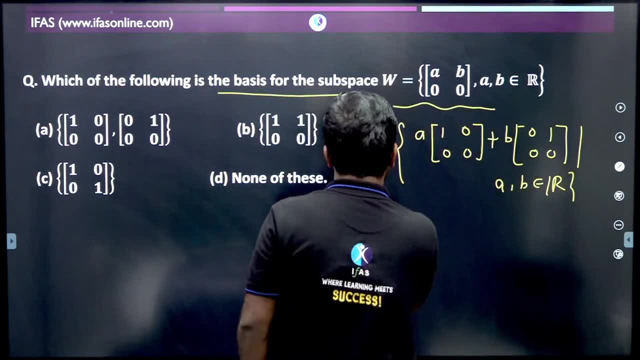 if I take B as a common, then what will I get? I will get 0, 1,, 0, 0, such that where will A, B belong? It will belong to real numbers. so what does this mean? W is written in the linear combination of these two matrices. 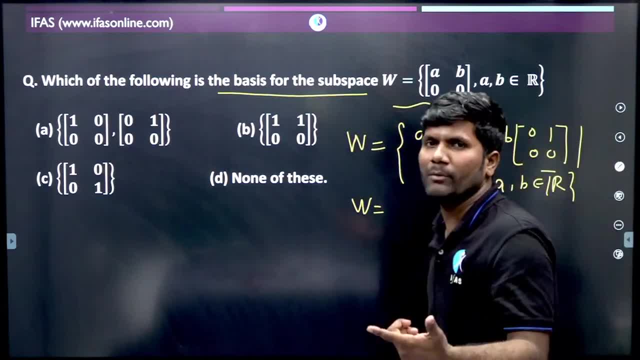 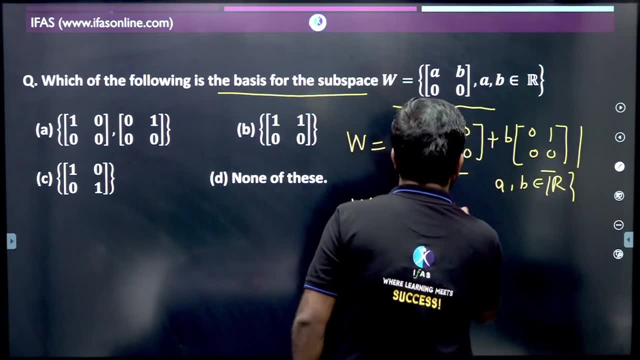 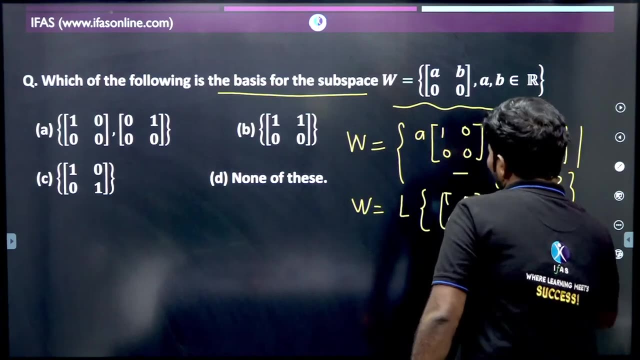 so what does this mean? This means W belongs to their linear span, so we can write W like this: how can we write it Like this? The linear span of this matrix. so we can write W like this: and you will check, you will get linearly independent. 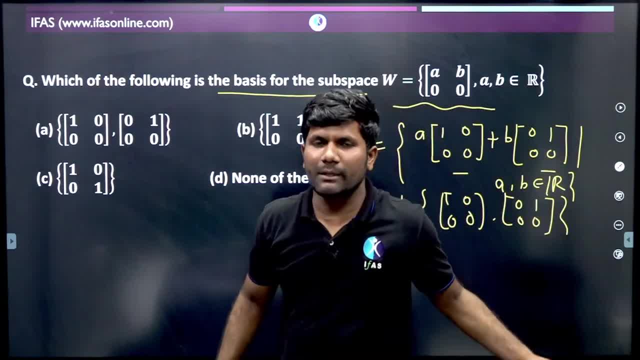 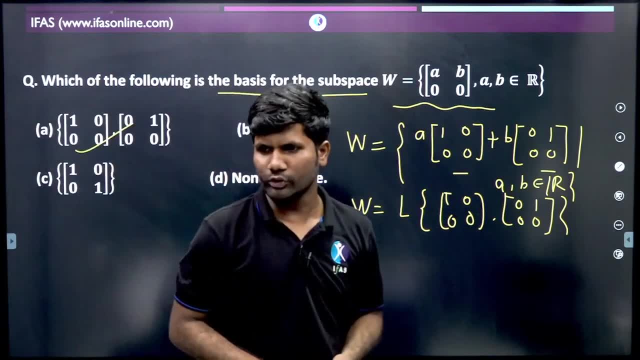 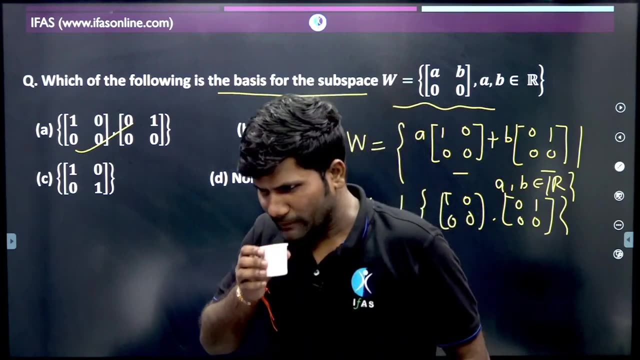 and all the Ws are spanning. what will this mean? This means this basis will be made. see where it is. here it is. did you understand all the students? No one is there. we will give you one day, Ganesh. I will give you one day, Ganesh. I will give you one day, Ganesh. I will give you one day. 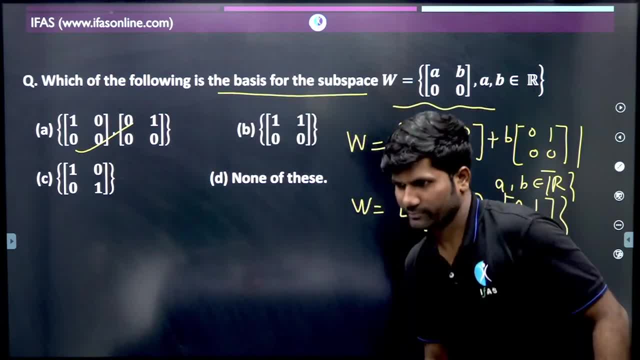 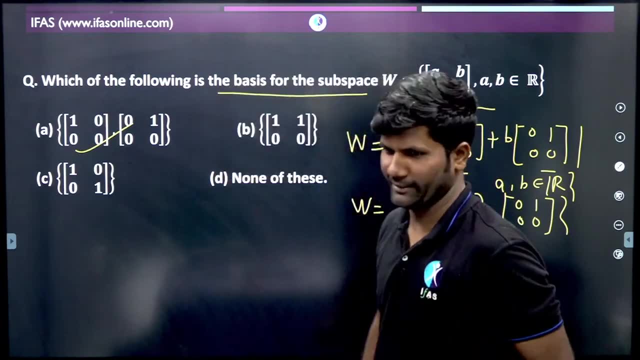 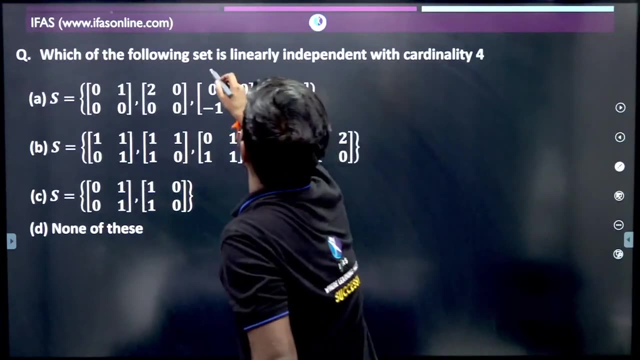 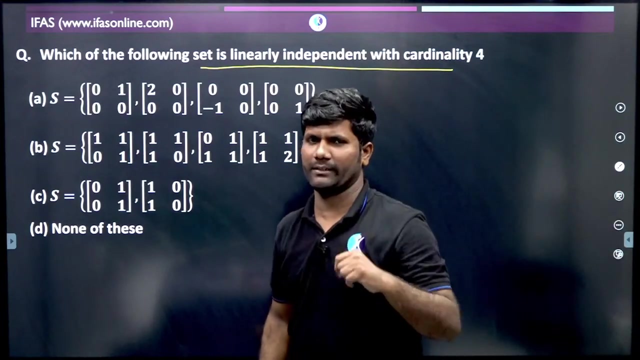 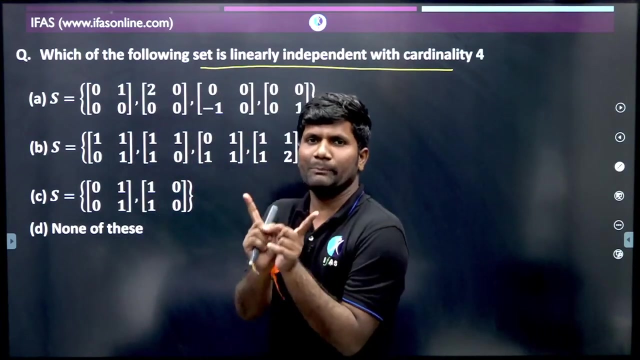 now here, which of the following set is linearly independent with a cardinality of 4? now a state is given to us where there are 4 elements means the dimension of vector space is 4 somewhere. now we are being asked that in a vector space whose dimension is 4, 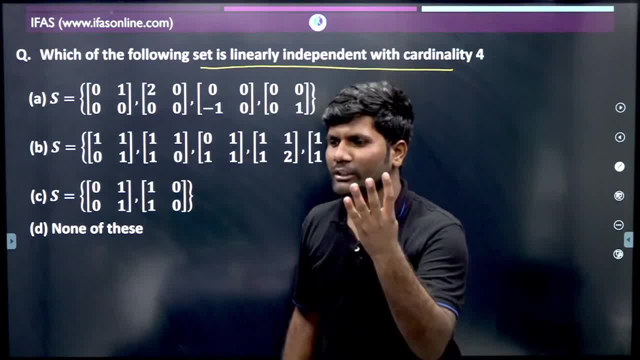 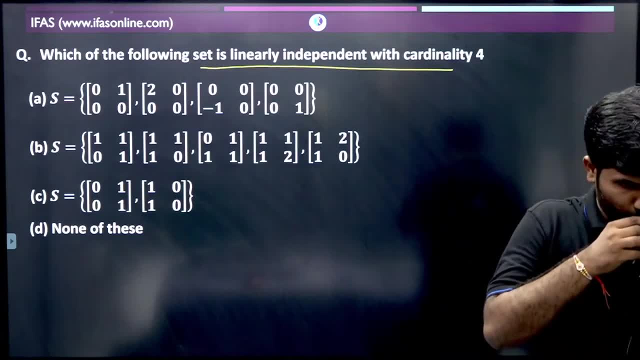 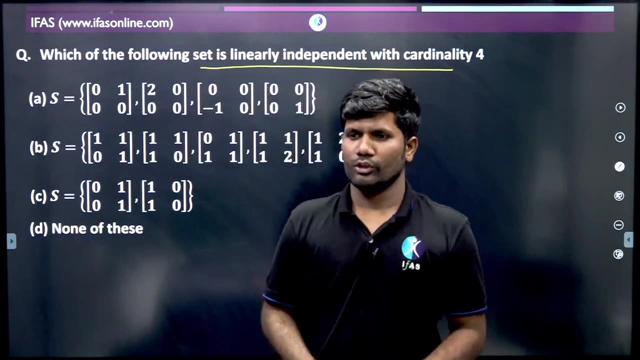 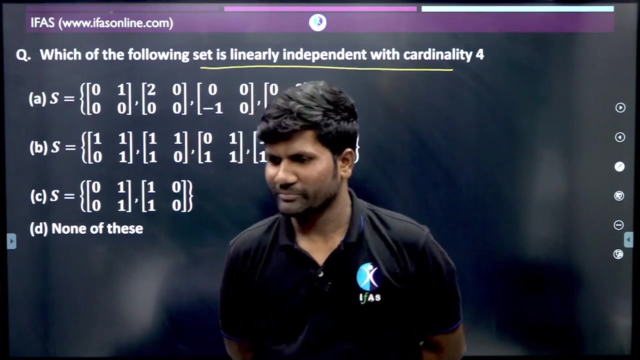 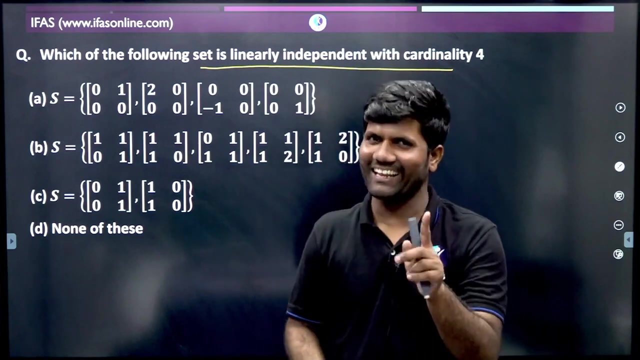 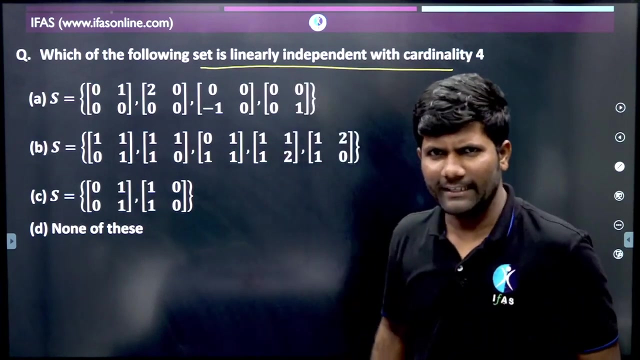 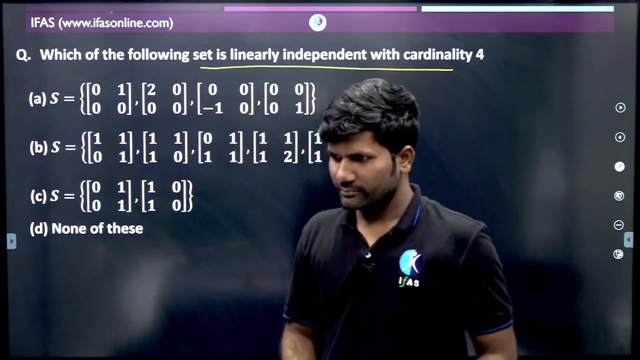 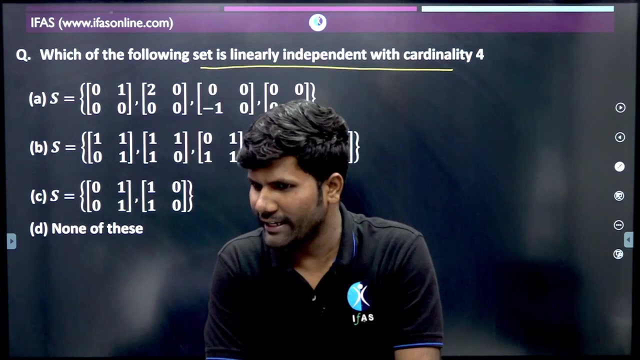 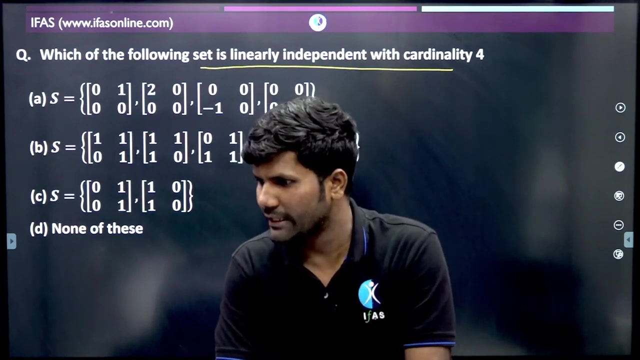 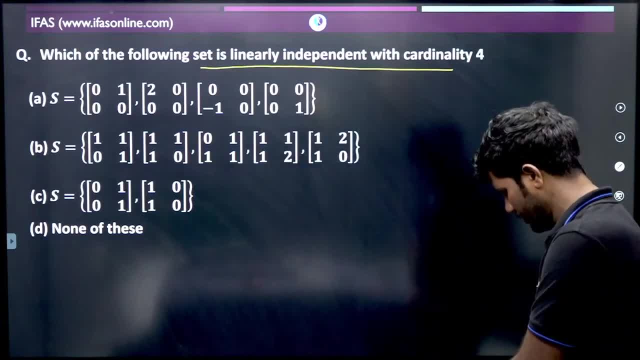 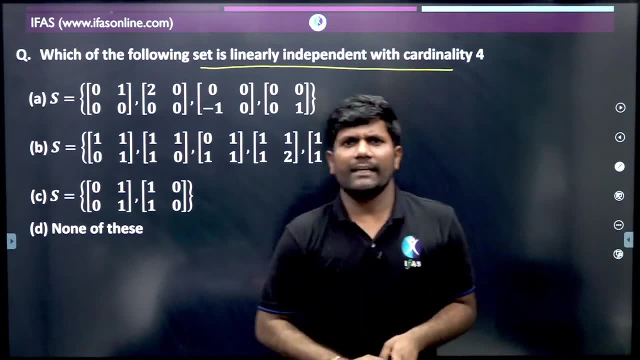 So when you are saying the same thing, we will accept it. Why will it happen? Let's talk about it once. What did we get here? What should be the continuity of the set 4.. Meaning, if there is a space 4, then we need a linearly independent set of 4 elements. 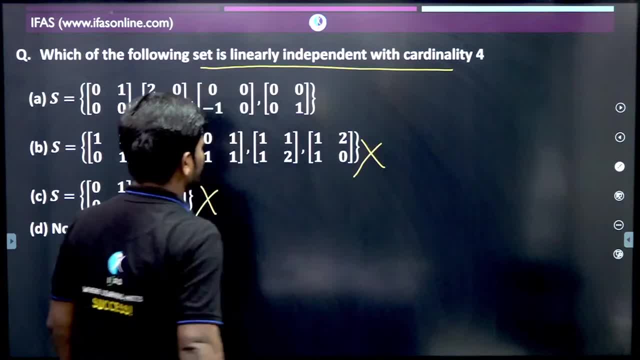 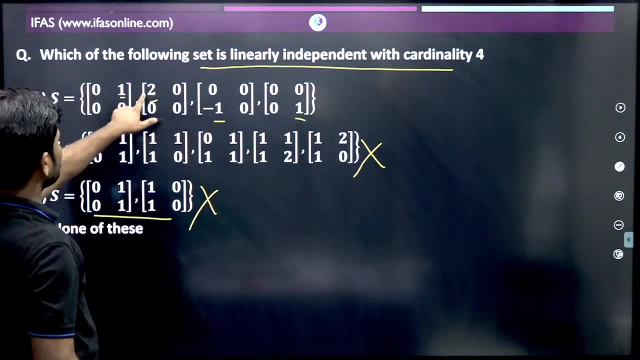 This is seen on 2, we have finished it here. This is seen on 5, we have finished it here. Now, what is left? Just look at it once. All the elements are on different levels: On the first level, on the second, on the third, on the fourth. 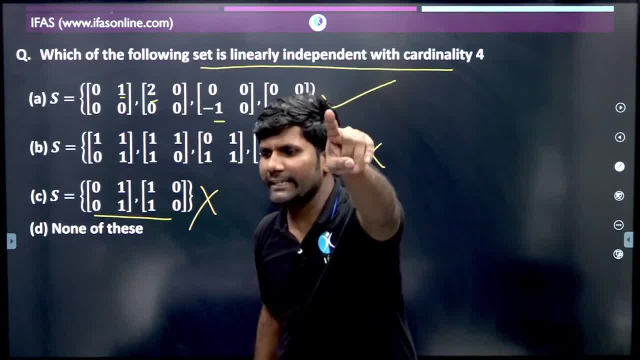 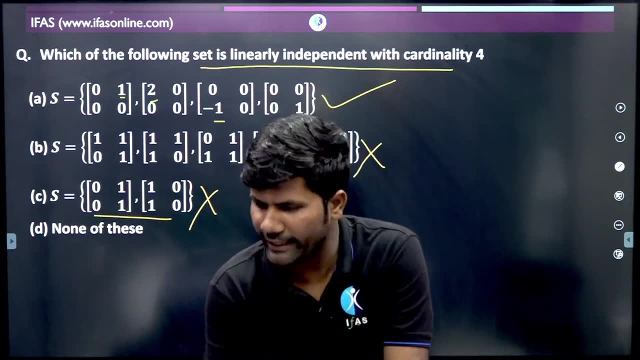 Which will become linearly independent. So who didn't understand? Tell me once: Absolutely A, B, Karim. Very good, You have understood it very well. That's why I said Sital. I will repeat it once. 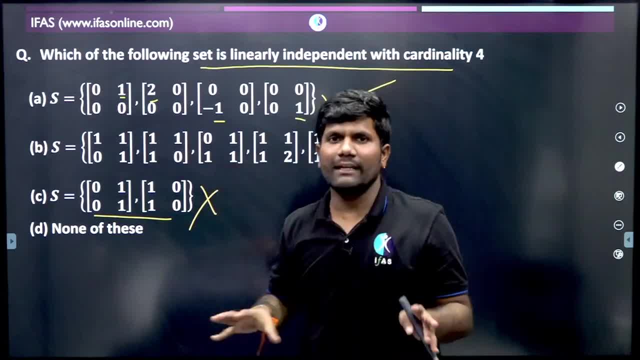 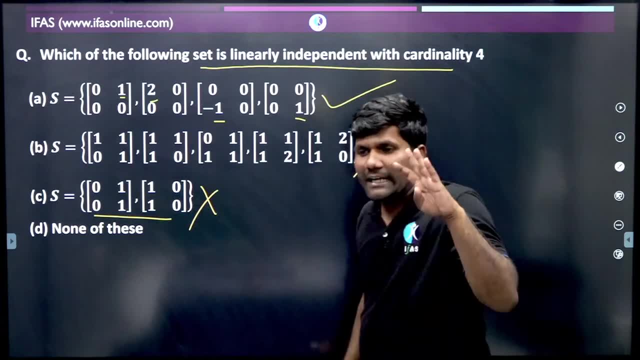 Sital. what we had to tell here is that now the set of 4 elements which is linearly independent, There are 5 in it, there are 2 in it, so they are finished. We had to check the set on 4 elements linearly independent. 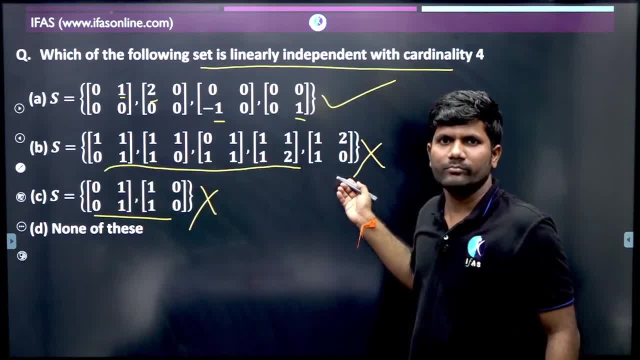 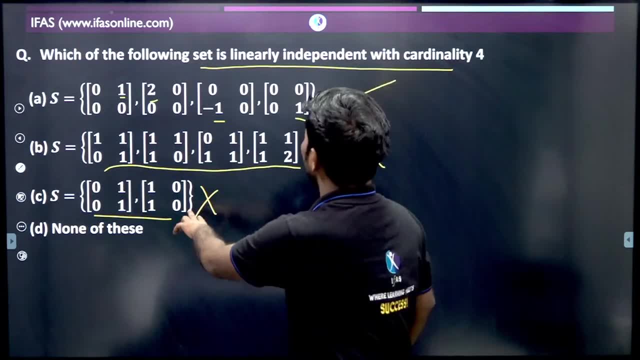 Now on 4 elements linearly independent. here comes the fifth element. What happens when the fifth element comes? It becomes dependent. Dependent means it will not be linearly independent. So we had to check the set on 4 elements. 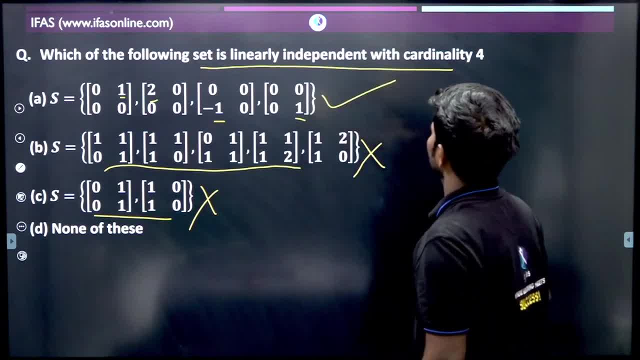 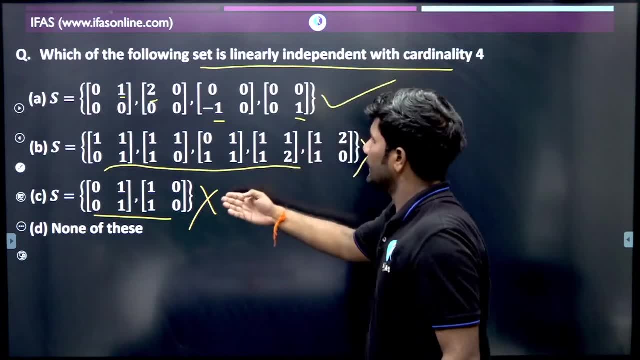 So only this one will be left. We had to find a set whose coordinate is 4 and linearly independent. How much is its coordinate? It is 2.. These two are finished, Only this one is left. And once we had to check here. 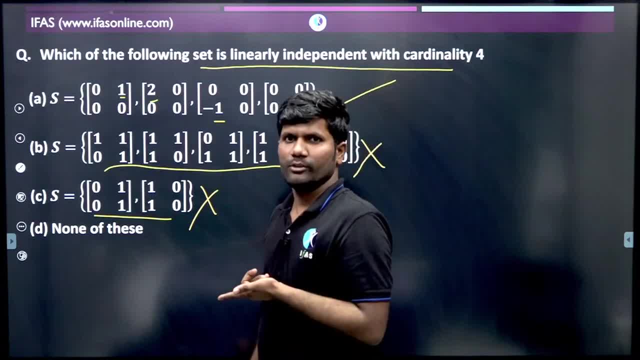 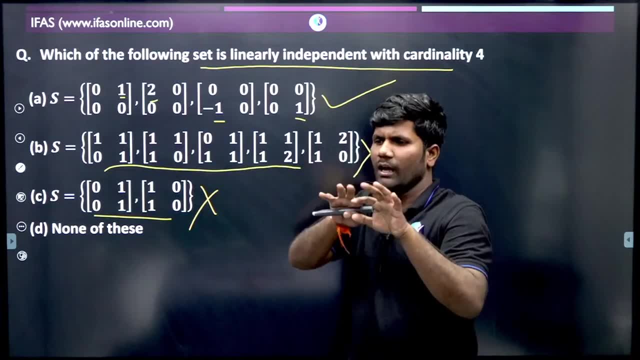 Just don't check like this. We had to check, if it is true. So here, if you see, all the elements are on different levels. There are 4 levels in the matrix: First position, second, third, fourth- All of them are on different positions. 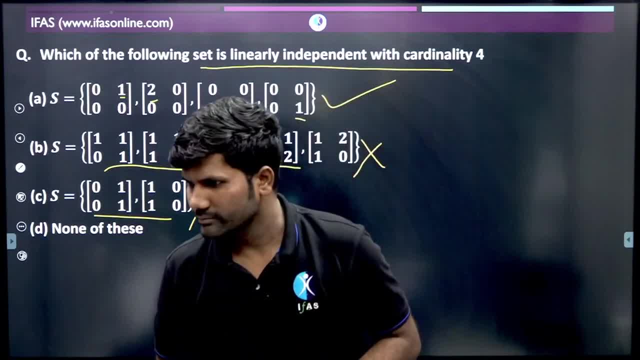 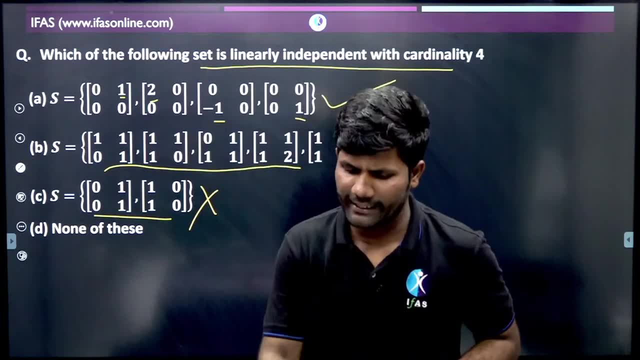 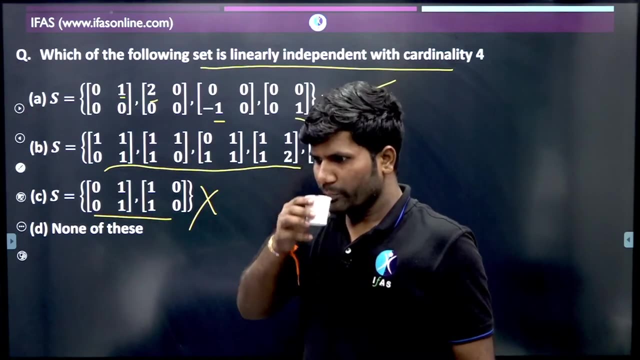 This means that linearly independent will be obtained. Today we had discussed the DPP of group theory for about an hour And after that at 6.30, your integral will continue on it. Till then, study here. So let's check the sky. 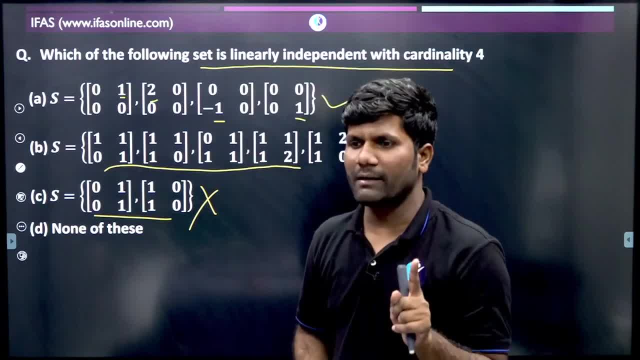 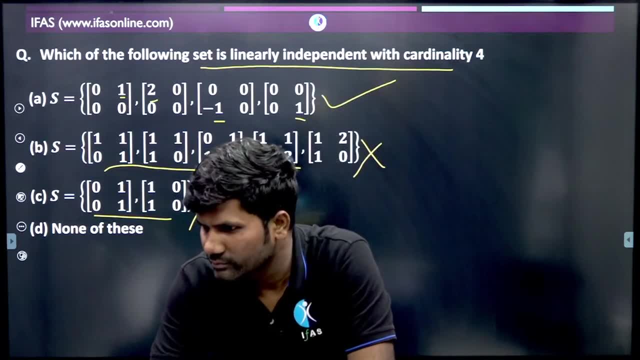 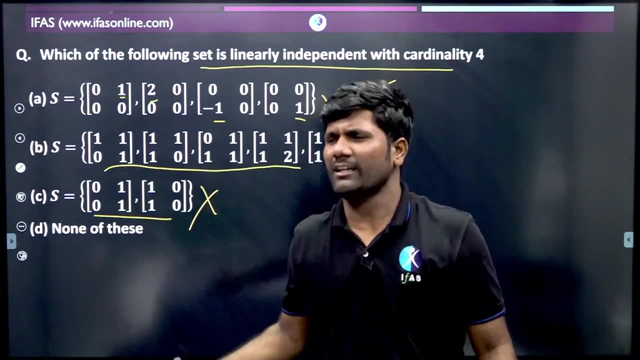 Let's check with linear combinations or matrix, Let's check with whatever you want to do. Okay, Absolutely, Pulkit, Absolutely, You are telling, absolutely right. There are some results of linear algebra. You can do those results very easily. What does one result say? 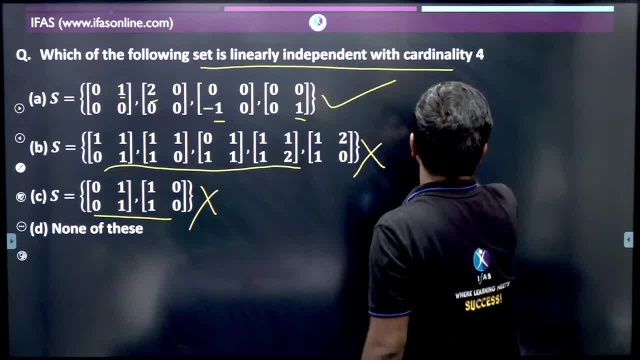 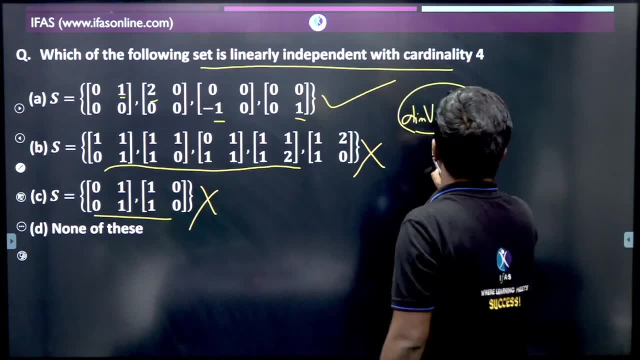 Suppose V is the vector space of dimension n. What is V? V is the vector space. What is the dimension of V? It is given as n. If you want to find its basis, then in the basis how many elements will be there? 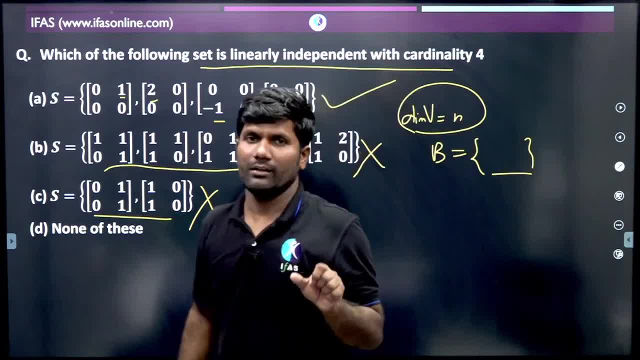 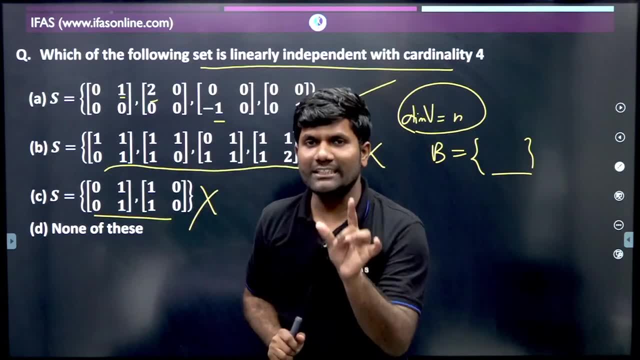 There will be n elements. But if one set is shown to you where there are more than n elements, then it will not be linearly independent. It will be dependent on that. So in any vector space the biggest linearly independent set is the basis. 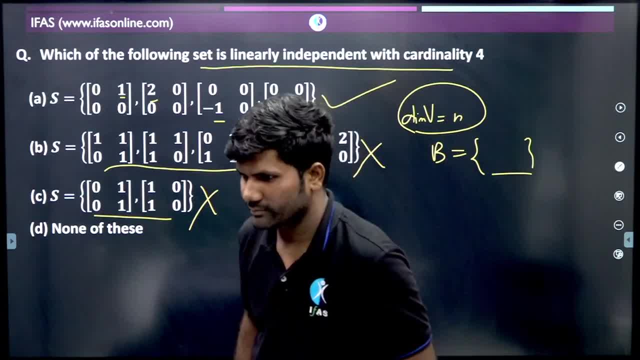 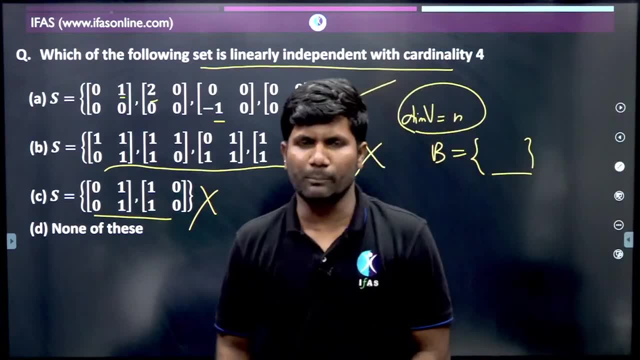 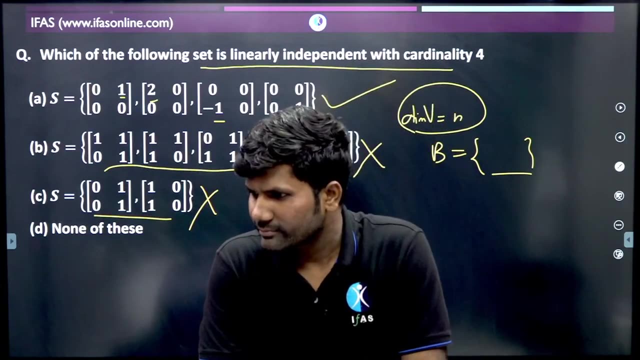 Okay, Okay, let's move ahead. So I hope you all must have understood. If anyone has any doubt, then you can ask, Otherwise we will move to the next slide. The next question is waiting for you. Okay, So what is the definition of linear transformation? 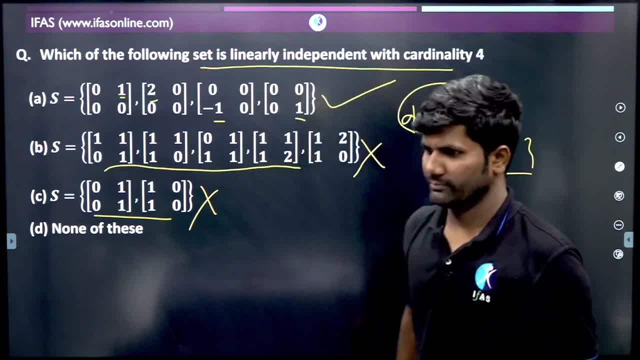 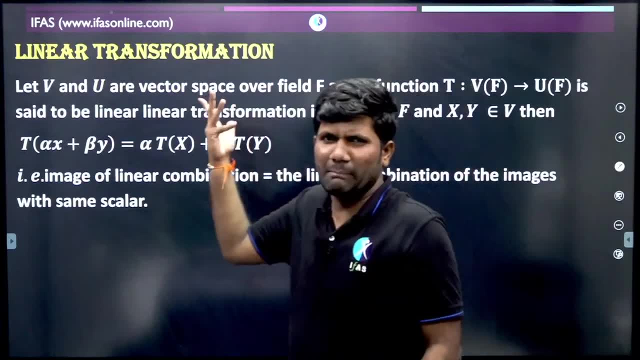 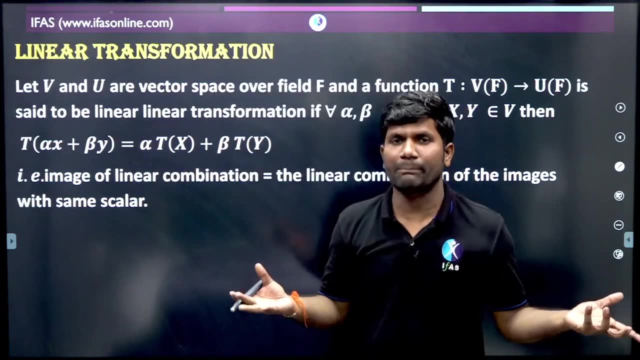 See, I am telling you all this. Okay, let's come to the next slide. You know the definition of linear transformation. What is linear transformation? It is a function, It is a vector space on another vector space which satisfies a special property. 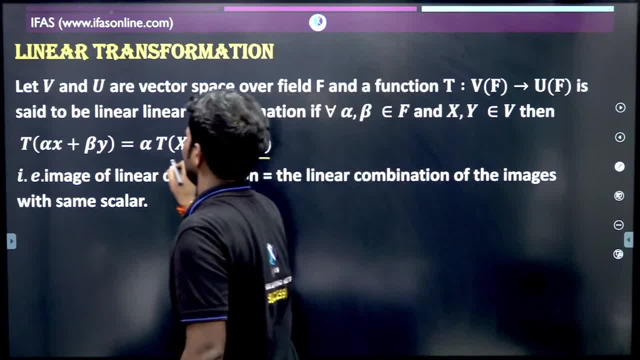 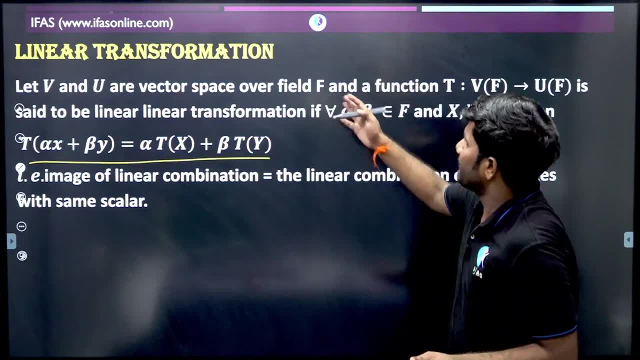 Now let's talk about which special property. This is the special property t of alpha x plus beta y. If alpha times t of x plus beta times t of y is equal, then that type of function or that type of t. 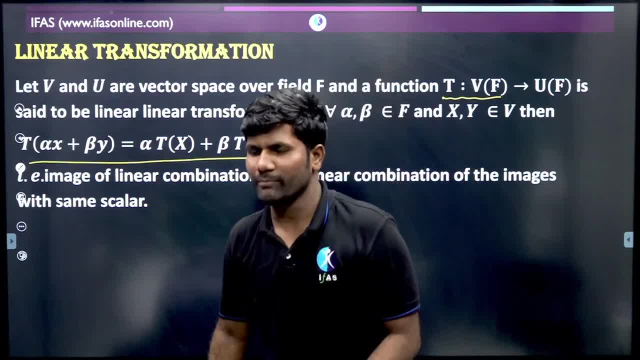 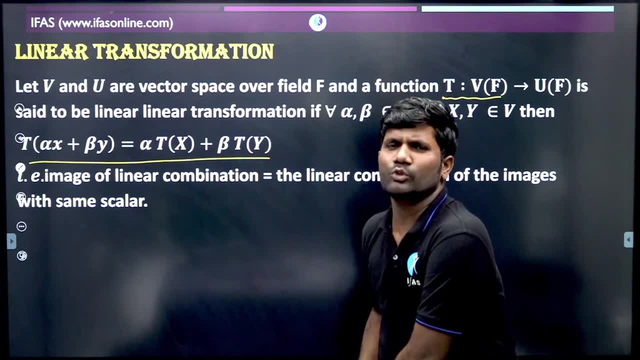 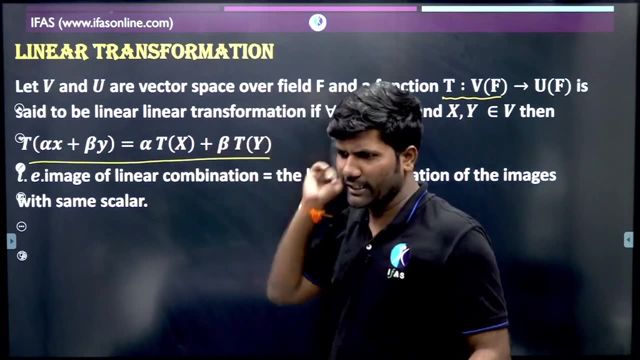 what do we call it? It is called linear transformation. Okay, Now the question arises: Is this the only method to check linear transformation? Basically, this is the only method, But other people can say it in some other way. also, Sahil has not brought the quadratic form today. 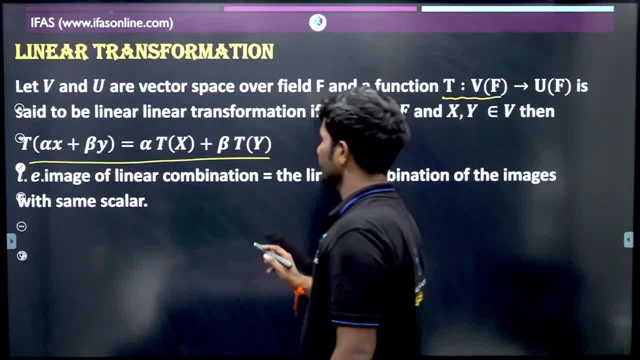 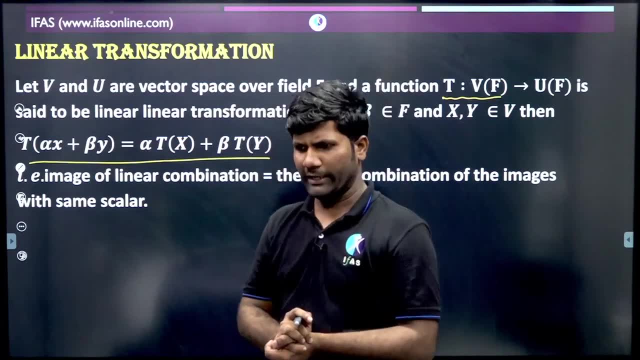 We will do as much as possible. As much as possible. Okay, Now, I think, for a bilinear form and a quadratic form, we will make a separate video for you. Okay, Sahil, We will make it in a few days. 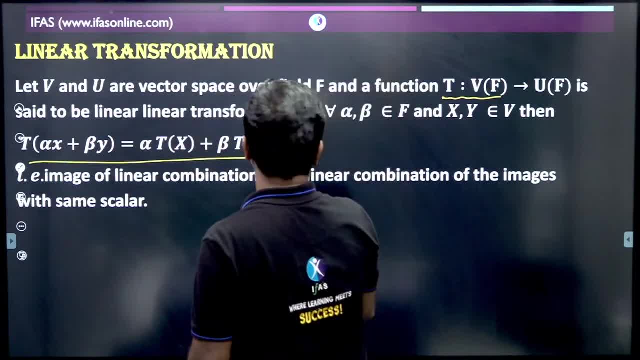 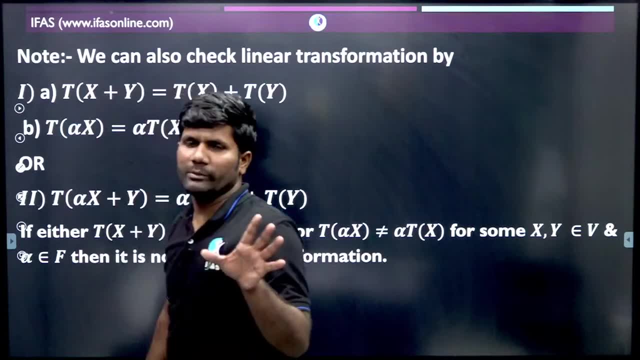 Whenever we get time in 2-4 days, Let's come here That side. Now look here To check linear transformation. you can check it with that Or you can check it like this: t of x plus y is equal to. 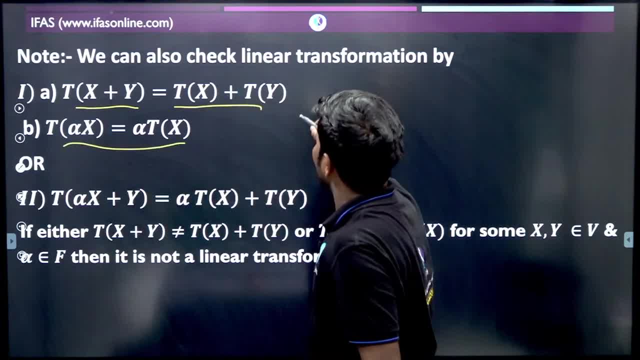 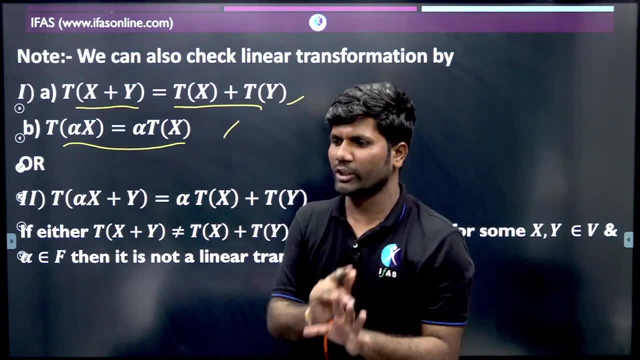 t of x plus t of y, t of alpha x is equal to this. If you get any such element for which any one of these properties fails, then t linear transformation will not happen. Okay, Clear Look here. Either t of x plus y is not equal to. 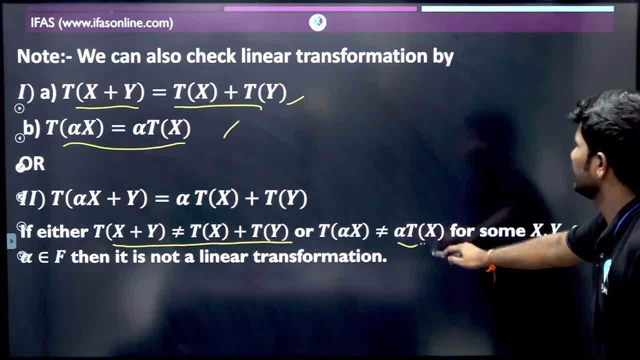 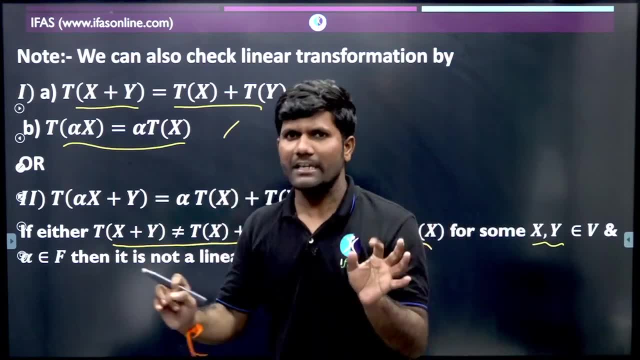 t of x plus y Or t of alpha x is not equal to alpha times t of x. If you get any x and y where a condition does not hold, then that means that linear transformation will not happen. Okay, Now let's come here. 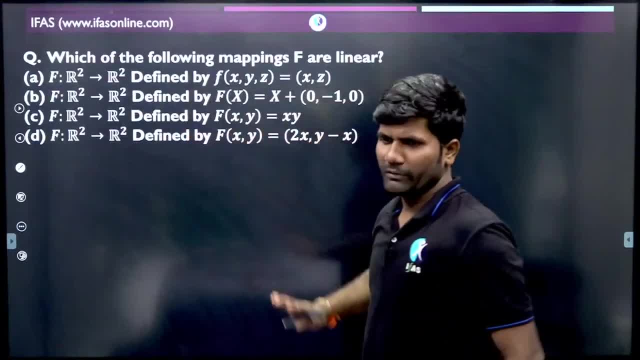 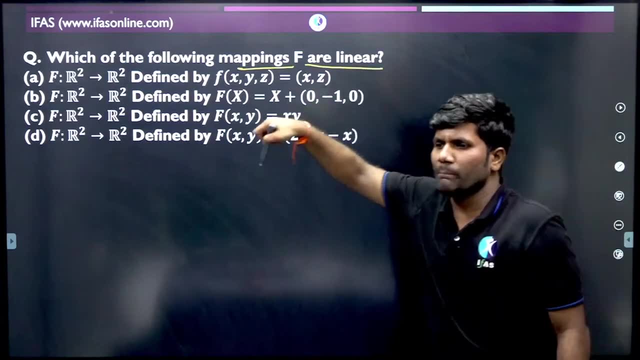 I will show you a small definition and then we will do the question. Okay, Now tell me What is here The following mapping of r: linear. Now I have to tell you Which of these mappings will be linear. Okay, 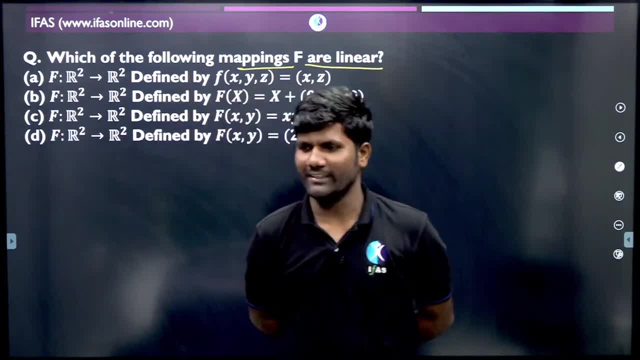 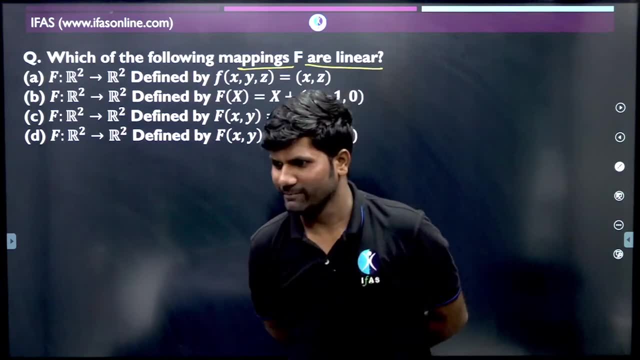 OST method: One step. Okay, yes, Absolutely, Absolutely. If you do it in one method, then do it in OST. If you do it in two, then do it in two-step method. Okay, Good morning, Mukti Ram Shelke. 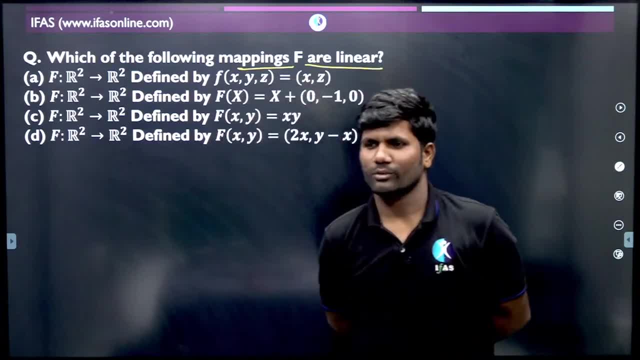 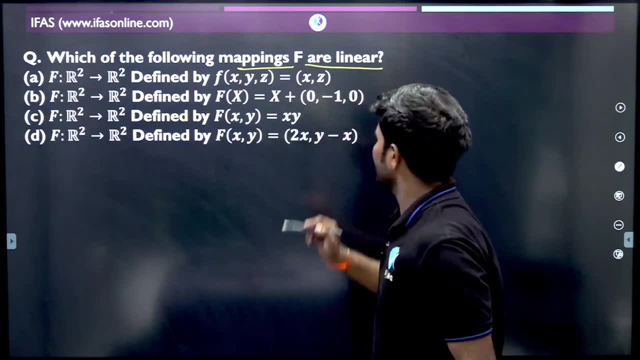 Good morning Saima Sadaf, Good evening everyone. Okay, new people. If you did not like it, if you are joining now, then like it once. Okay, Now tell me Which of these will be linear. 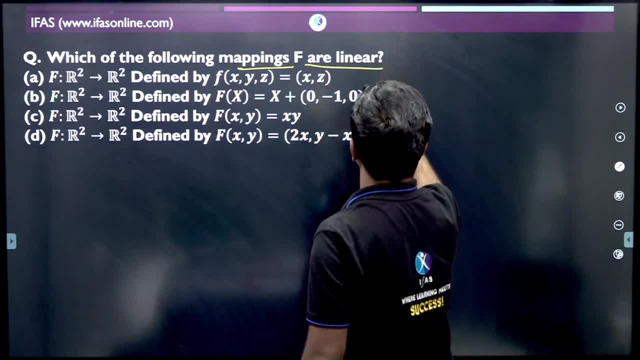 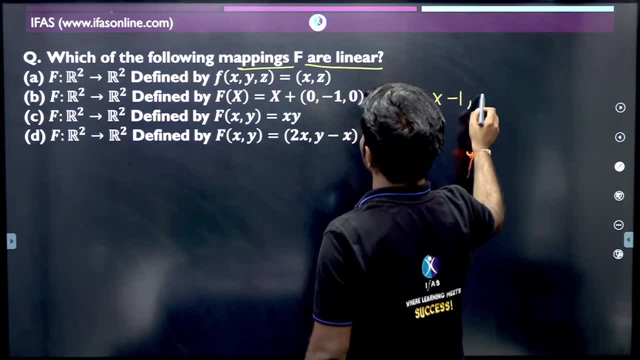 Tell me. See, this is just to confuse. What does this mean? This means: add it. What will happen? x will happen Here. x will be minus 1.. Here, What is x? It is the element of r2.. 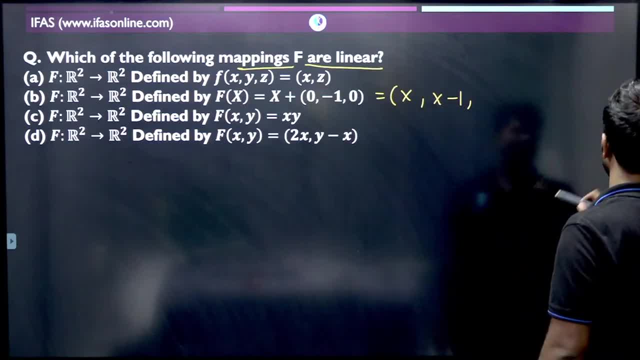 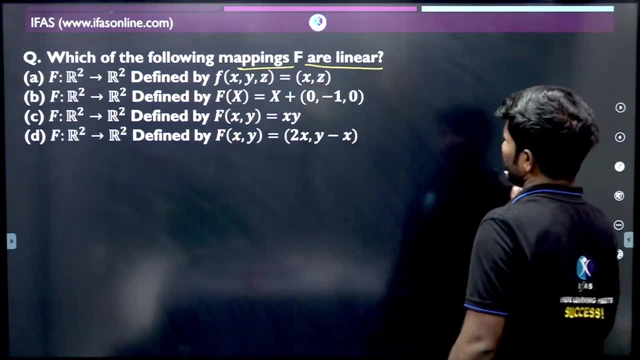 One minute. Something is wrong. We will move this map a little. Okay, This map is not right Here in this map. remove this. This is not a term. Okay, Now, tell me Now what to do here. 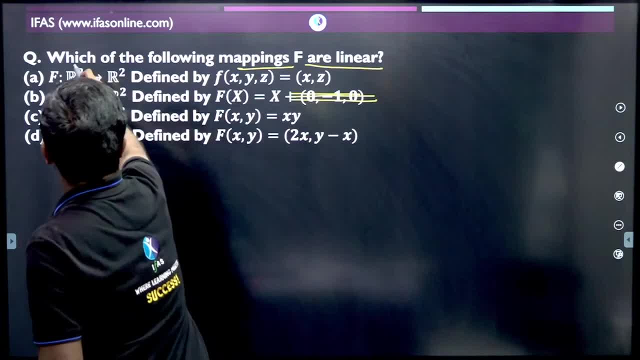 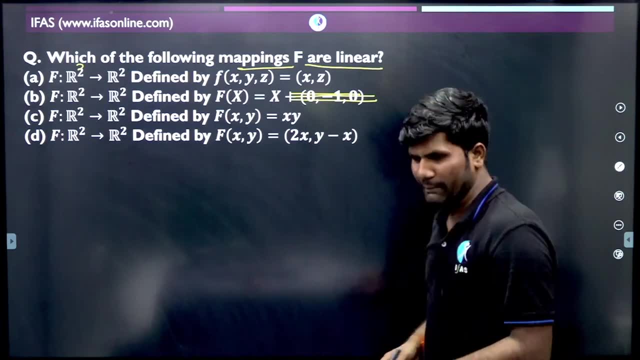 Here do r3. We are mapping from r3 to r2.. Okay, Clear. Now tell me what will be the correct answer for this question. Kalyani Vaidya told me, Sri told me, Bharti told me. 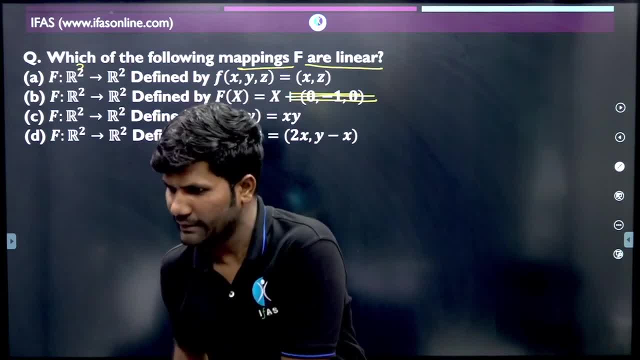 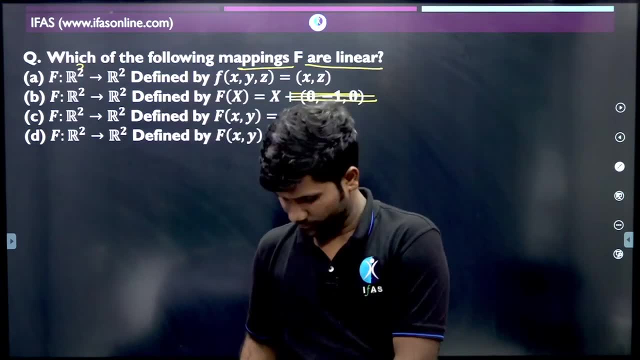 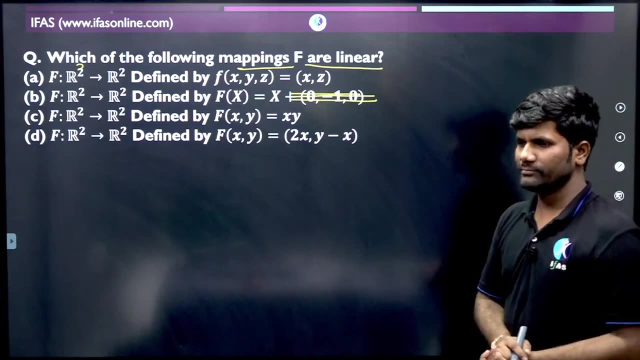 Pankaj told me. Pankaj told me. Pankaj told me: Good morning, you are late today. Okay, So what will other students get? Tell me once after solving Pulkit. told me a and d A. 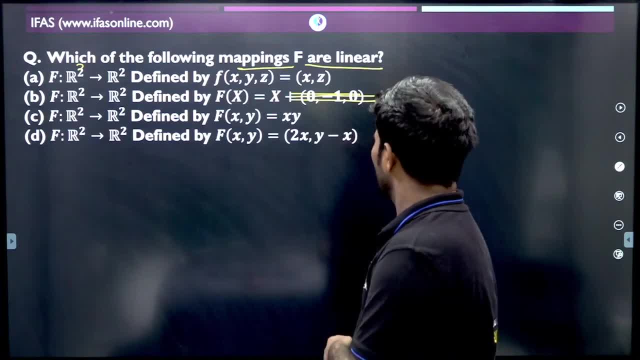 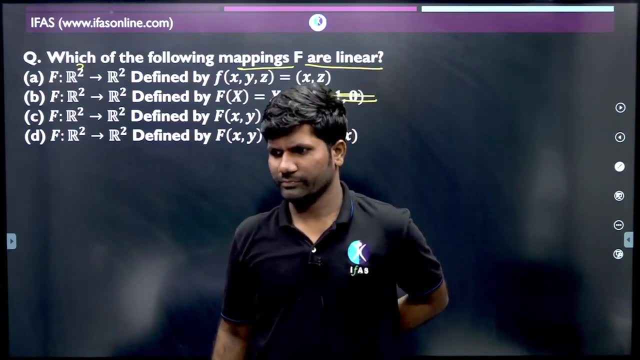 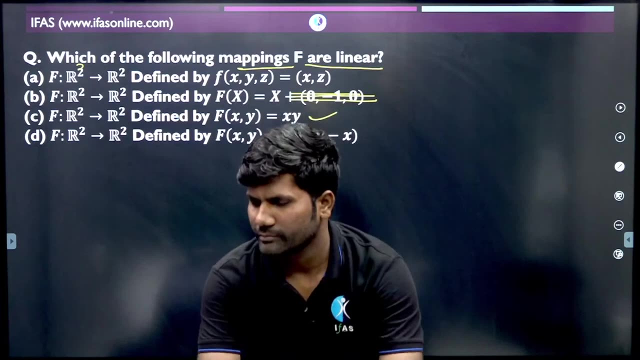 and d will be linear. Why will not b be? pulkit, Tell me, Why will not b be b? Can you give me a counter example where I am not satisfied with a condition? Very good, Bharti. Nagpal Bharti said A, B and D. 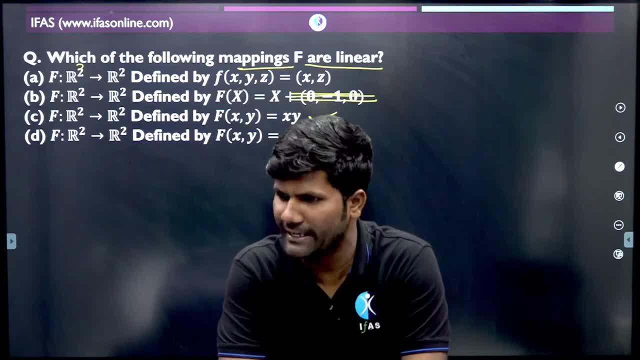 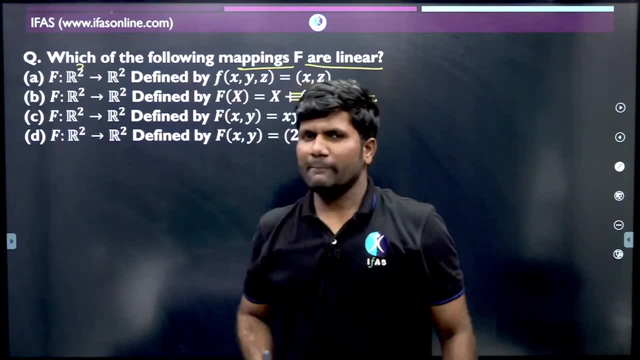 Vivek Priyadarshi is saying D. Amruta is saying A, B, D. What do the rest of you think? What can be the correct answer? Tell me one thing. I know that you can prove it to be linear. 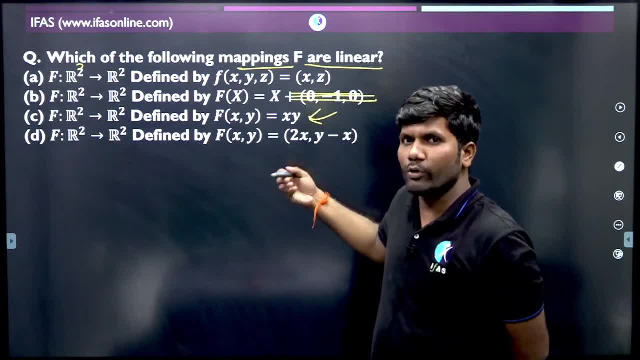 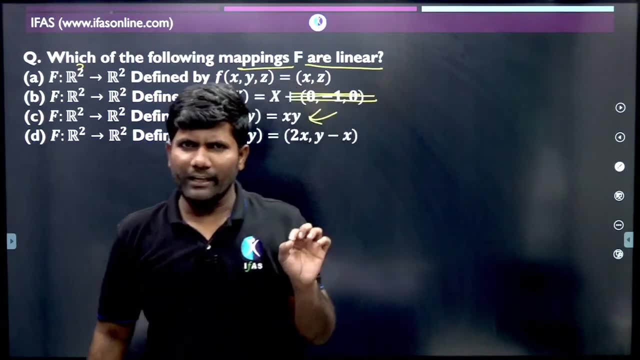 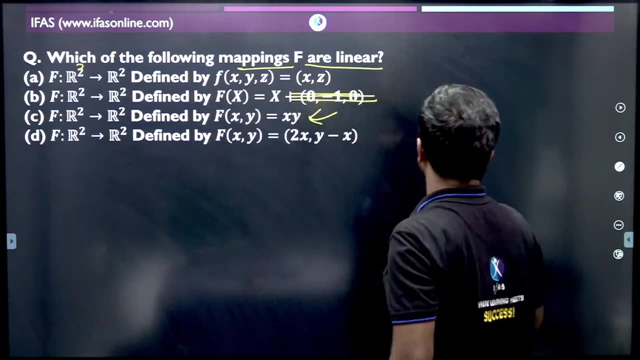 For this? tell me a counter example. If it is not linear, then give me two examples Which I will tell you that the condition is not satisfying. Tell me, Look. let me tell you one thing for all the students: To check linear transformation. you know that if T linear is a property, 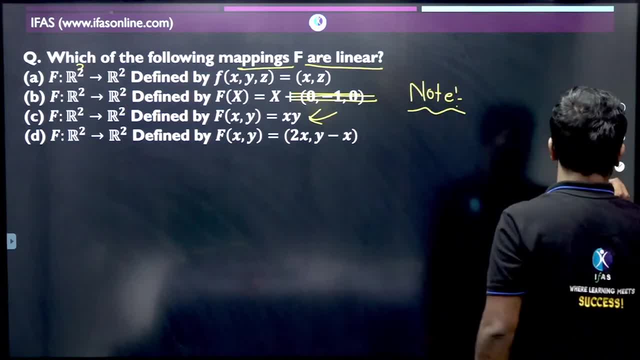 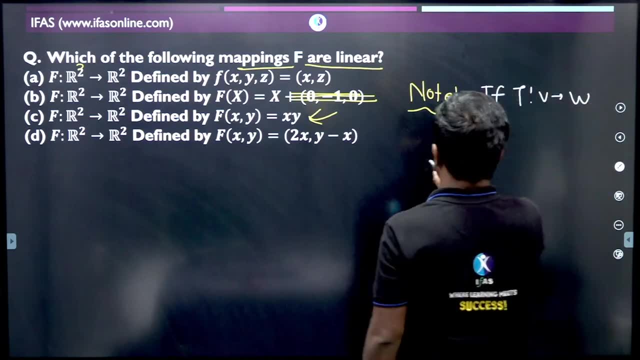 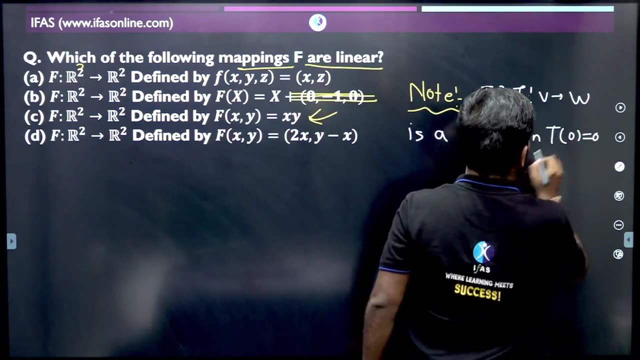 which is for you. keep in mind. it is useful. Sometimes linear transformation comes To discard another option: T from V to W. If T is a linear transformation, then T of 0 will always map to 0. This is the condition If I call it note number 1.. 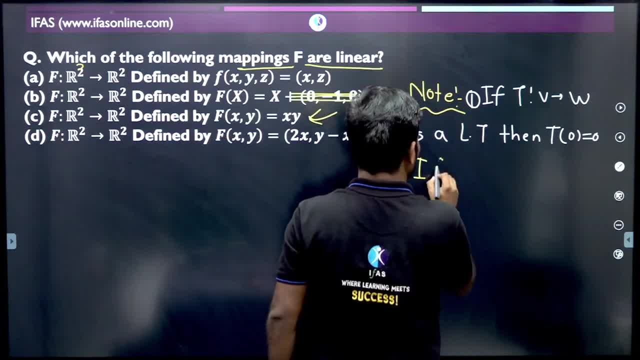 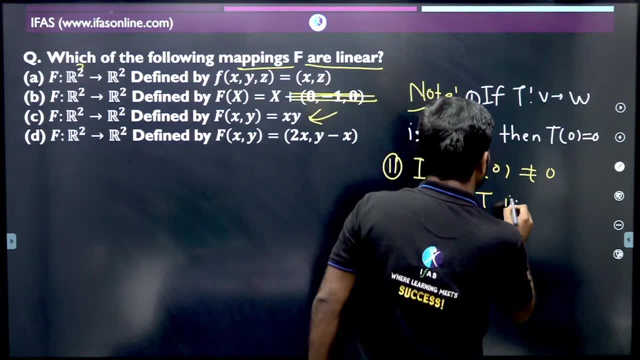 If I take the negation of this, then what will I make? note number 2? If T of 0 is not equal to 0, it means that then I can say that T is not a linear transformation, T is not a linear transformation. So here T is not a linear transformation. 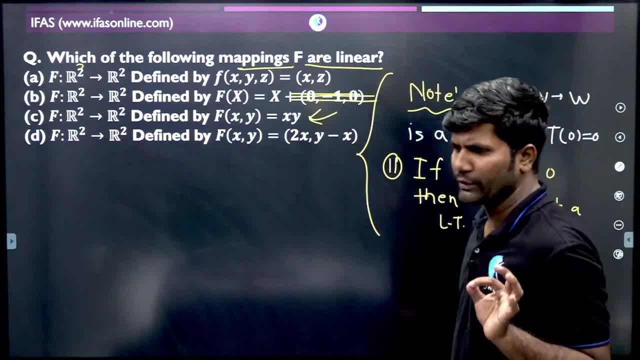 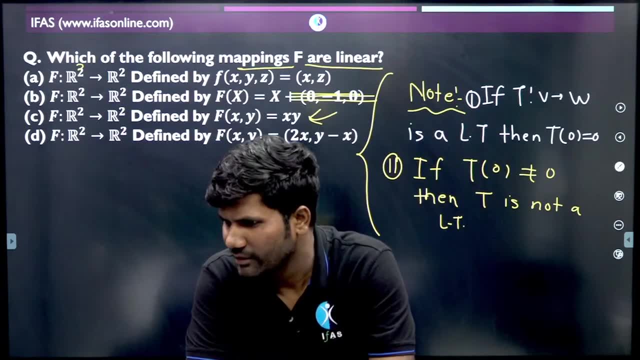 This is a very useful property. If there is a question of linear transformation, one or two questions are solved from here. Aditya, it is okay, I am telling you in Hindi. Just tell the name of it in English. The rest of the things I am telling you in Hindi. 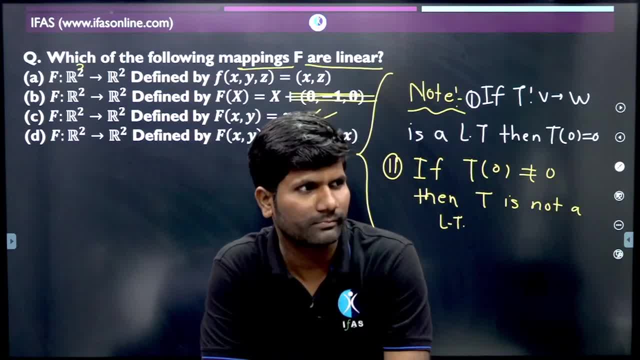 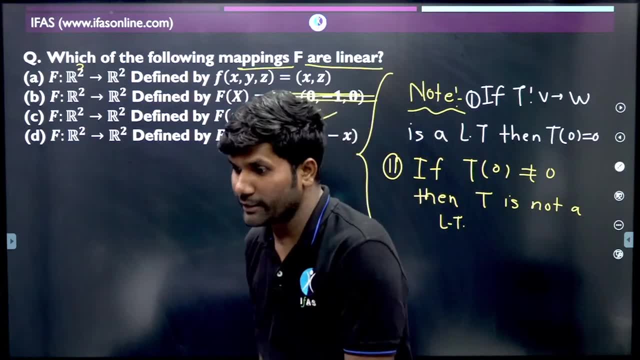 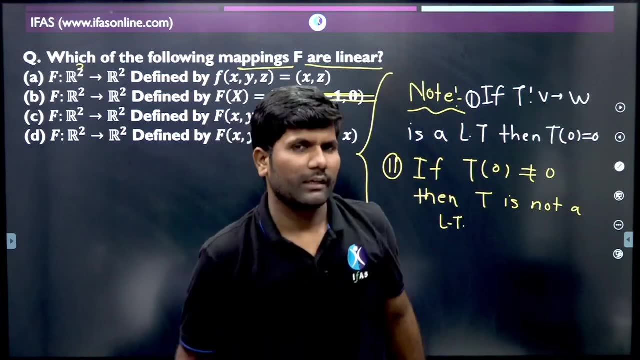 Okay, Come on, we will do as much as we can. Okay, By the way, I am not Aditya, I am Ajit. Okay, I understood Ajit. Good morning, HMI Academy. Good morning, Okay. And yes, keep one thing in mind: 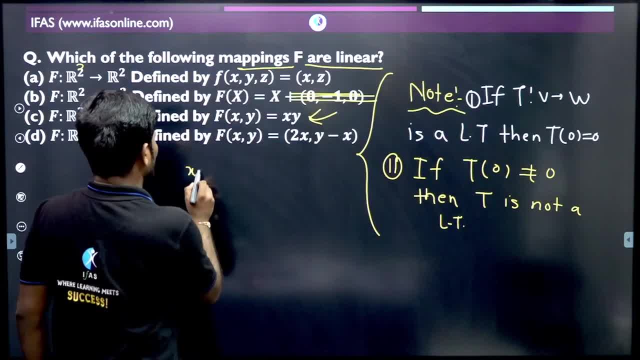 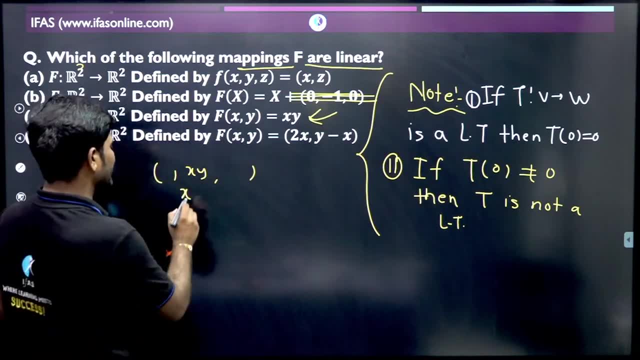 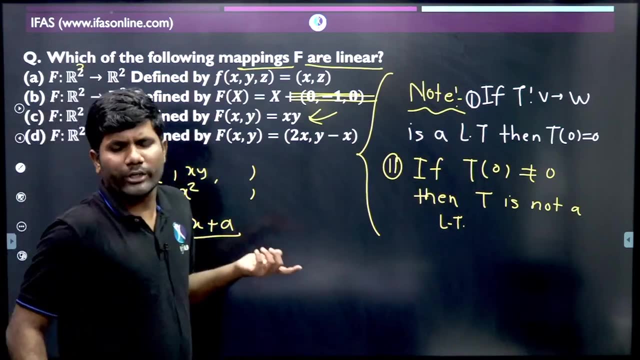 Whenever, like, you get the term of xy or if there is a double somewhere, like if you get the power of xy somewhere, or if you get the power of y somewhere, or if you get x plus 1 or some constant, y plus some constant. 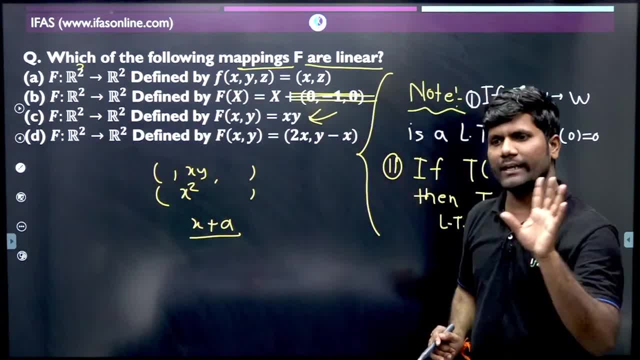 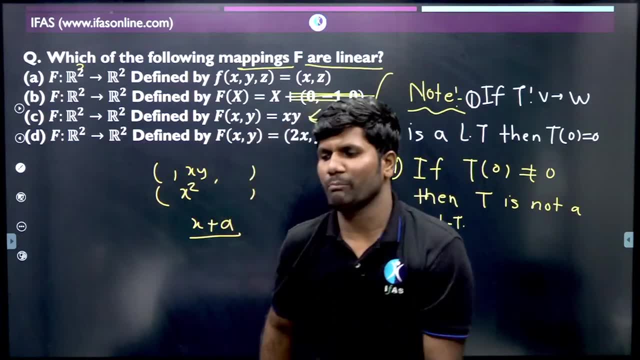 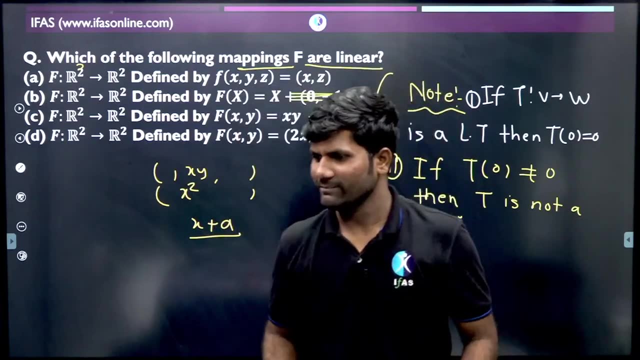 then always keep in mind. in that case, there is never a linear transformation In 99%. Yes, yes, Pulkit, I thought, but I said it. I thought that you did not remove it at that time, No problem, Okay. 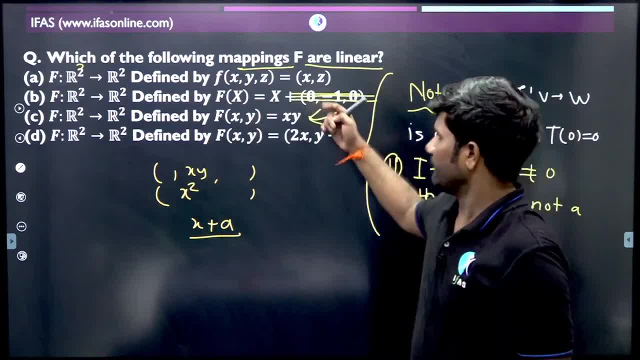 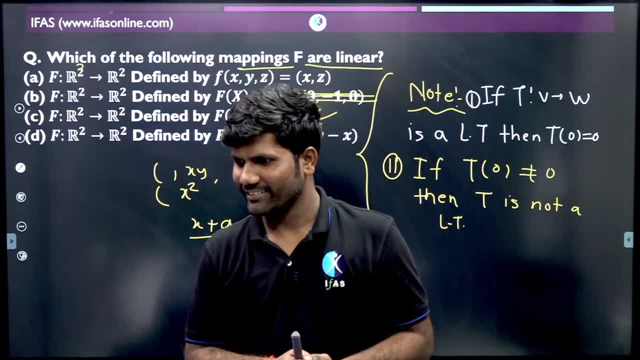 Okay, Pulkit, Come on. Pulkit, tell counter example for this For option C. For option C: no one told counter example among these. We know that Vivek will not be option C, So you tell counter example. 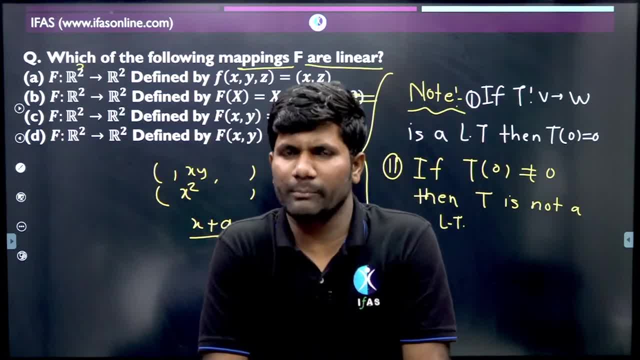 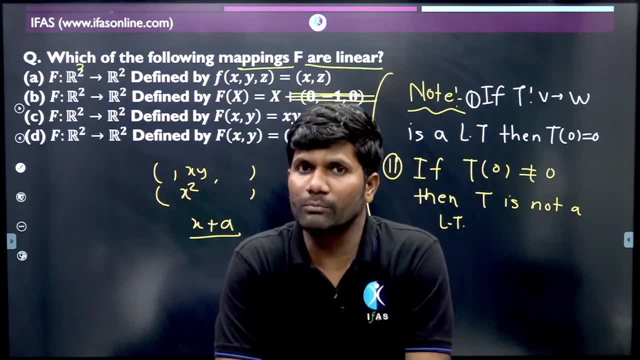 See, if any result is proved, then we have to prove it. If it is not, then I have to give an example that it does not satisfy. If I do, then my work ends there. So I hope you tell counter example. 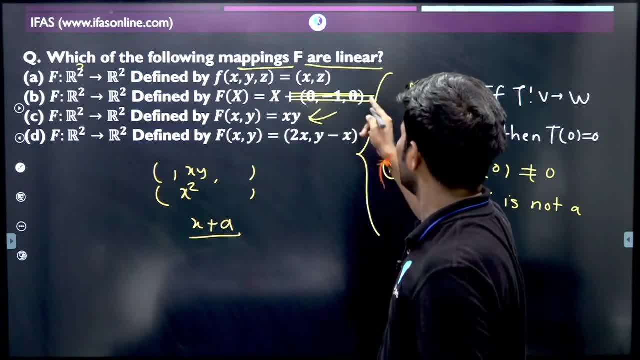 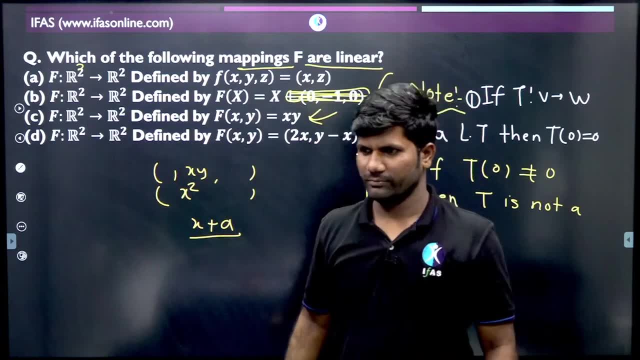 Dilip, see. Dilip said with confidence only one. He said: Dilip, see, here we have removed this. Okay, See, confidence is like Dilip, There is nothing wrong with it. You will learn Dilip. 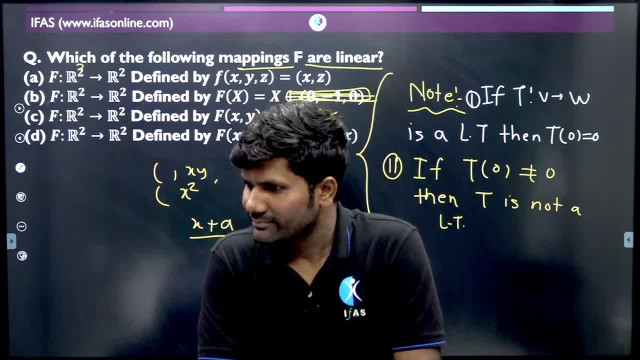 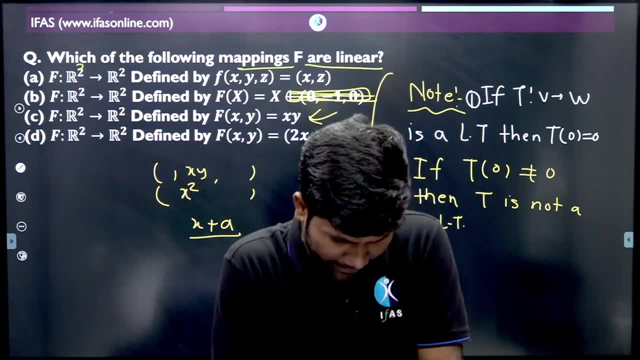 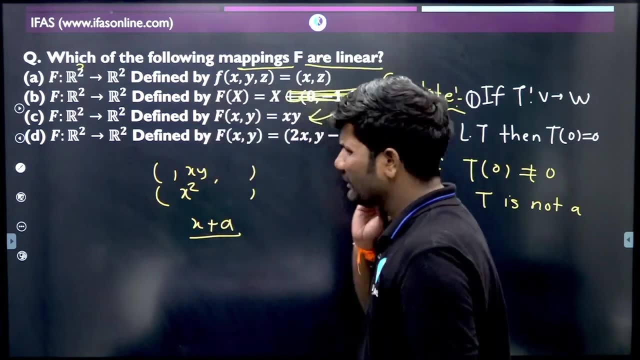 Okay, What is the answer you are getting? Pallavi said 1, 2.. Pallavi is saying 1, 2.. 1, 2.. Okay, Let's take 1, 2.. Come on, Let's see for Pallavi. 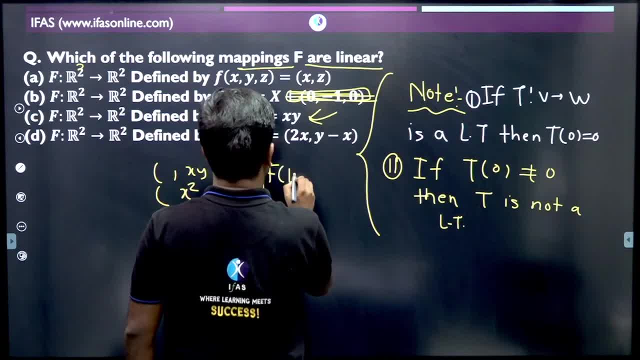 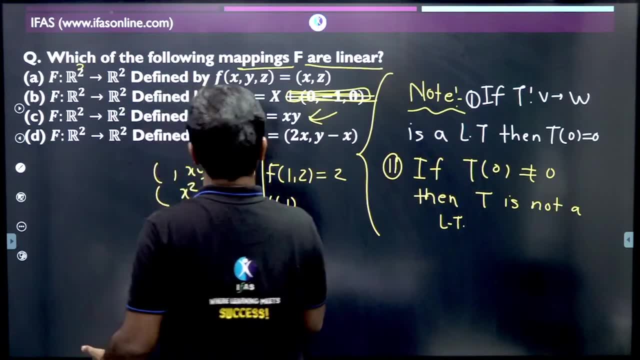 Does 1, 2 work as counter example for Pallavi? Let's see what happens. What will happen for f of 1, 2?? It will be 2, but f of 1.. Yes, We want 2, right. 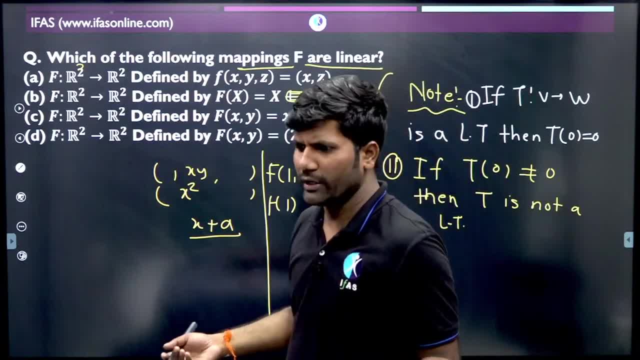 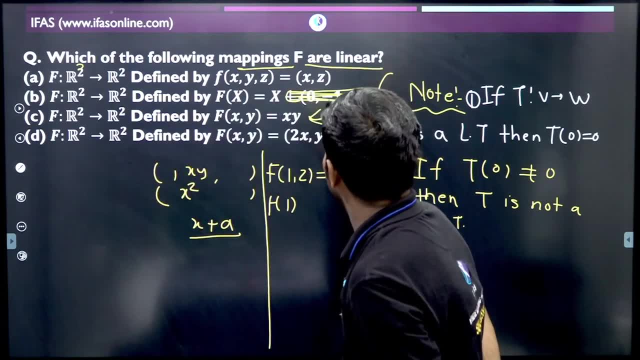 Pallavi, Pallavi, give 2.. How can you give only 1?? What shall I call 1, 2?? Give something else right. A, B curry mask, Very good. If you put 0,, then no option is being discarded. 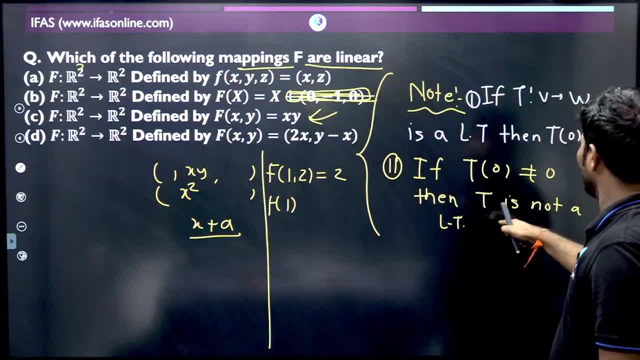 See: if t of 0 is not equal to 0, then matrix: linear transformation is not. no matrix, no map: linear transformation will not happen. If t of 0 is not equal to 0, then matrix: linear transformation. 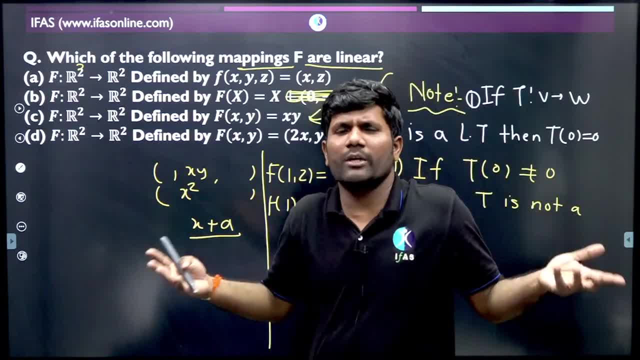 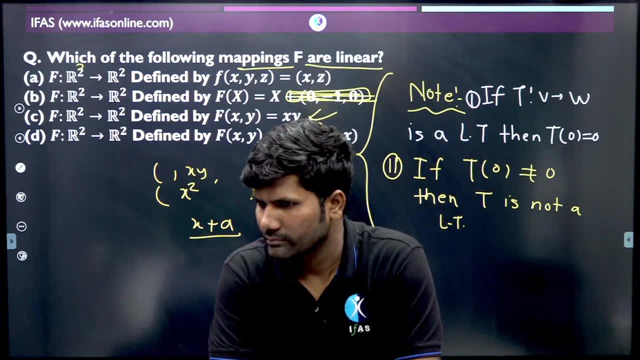 no matrix. no, If T of 0 is equal to 0, then it doesn't matter, It can happen or it can't happen. Yes, yes, Pallavi is saying for learning. Okay, Give me some counter example. 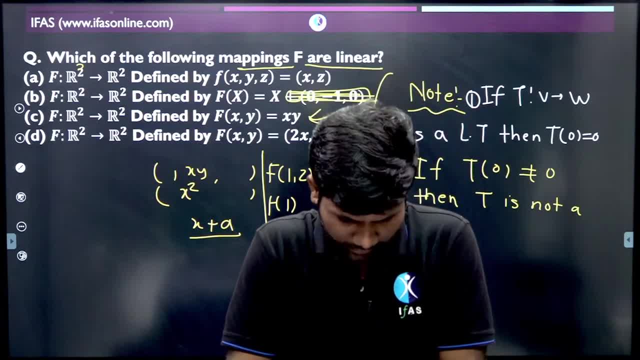 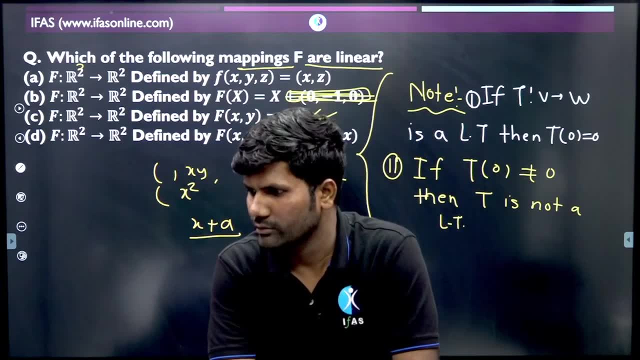 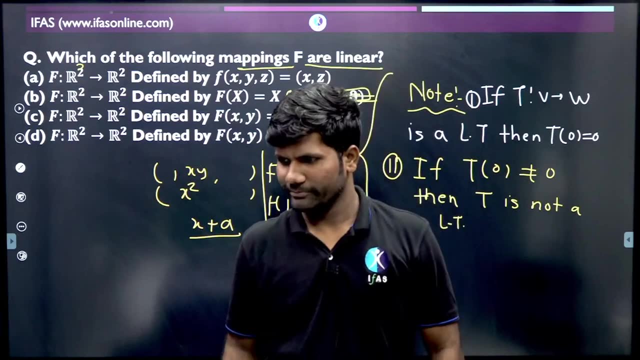 I will have to make this too. What should we do offline Sayyam. What should we do available? Do offline, Yes, tell me. Our offline classes are starting from 1st October. Come to Pune now. Okay, Tell me counter example for this. 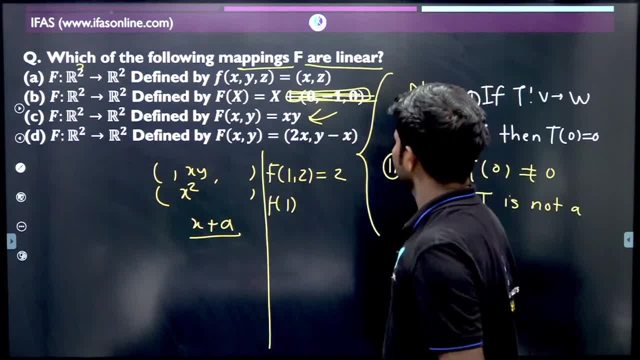 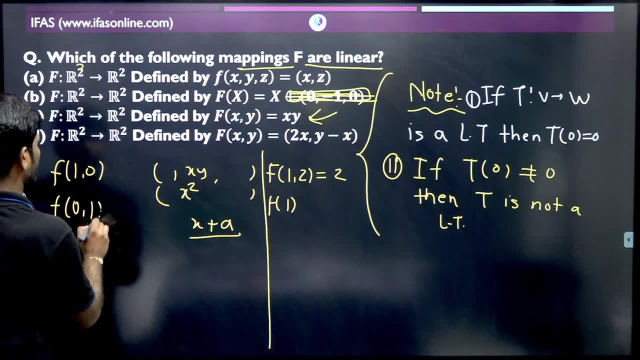 What will happen? There is no answer. Take F of 1, 0 and F of 0, 1.. So what will you get? You will get 0 and he will get 0.. When you add both, that is, when you add and find. 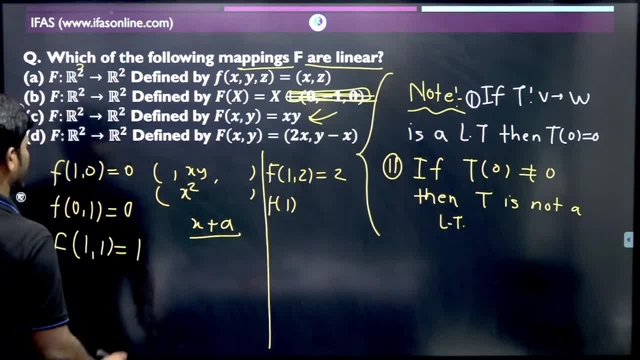 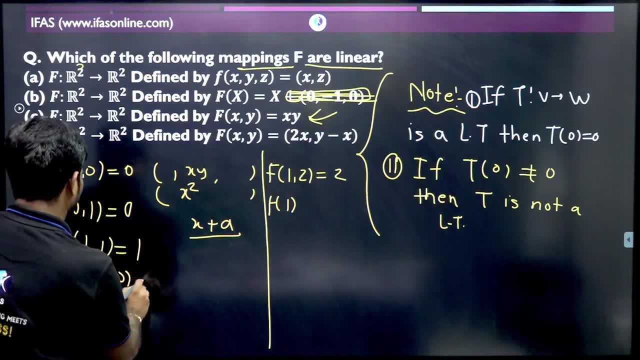 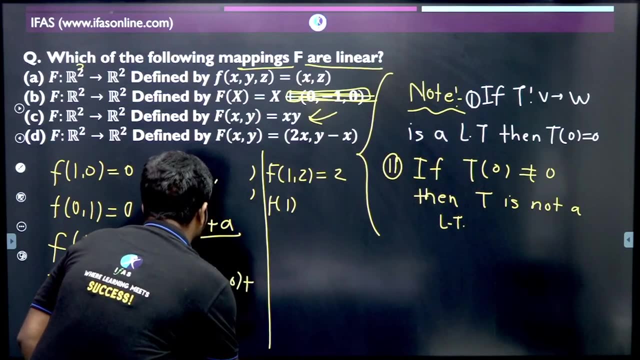 then if you add this, it will become 1, 1.. Which will be what You will get: 1.. So here you will clearly see that F of 1, 0 plus 0, 1 is not equal to F of 1, 0 plus F of 0, 1.. 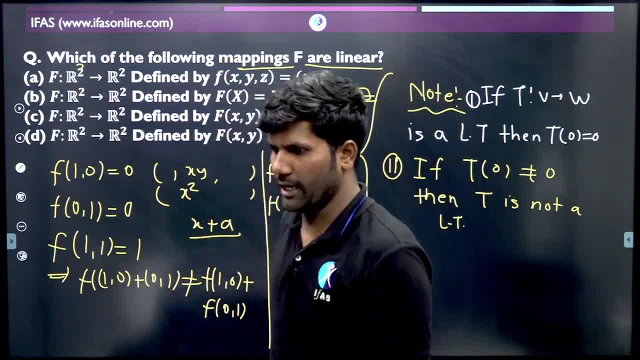 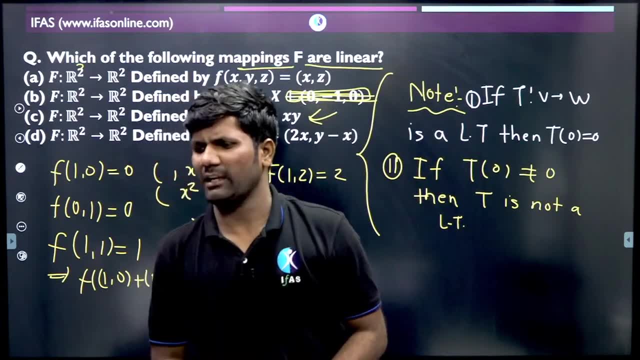 Okay. So here is the counter example. Is it clear to everyone? Yes, very good. Kalyani gave it. Okay, Aakansha also gave it. No, no, Pallavi is not in Nagpur. You will have to come to Pune. 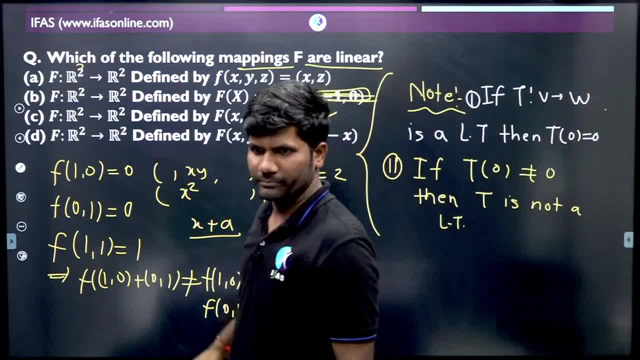 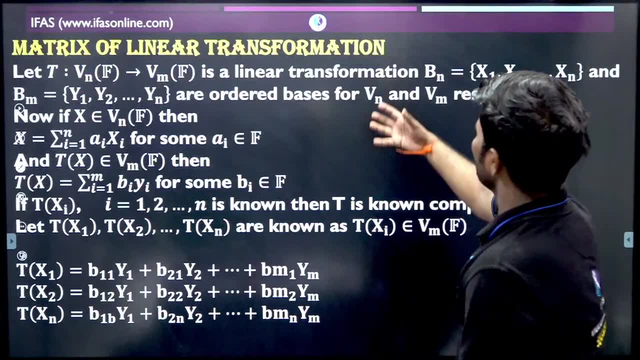 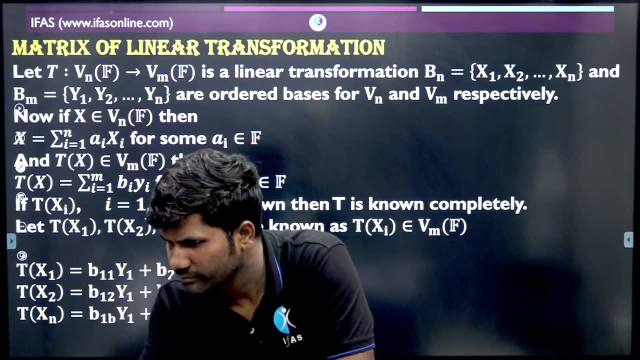 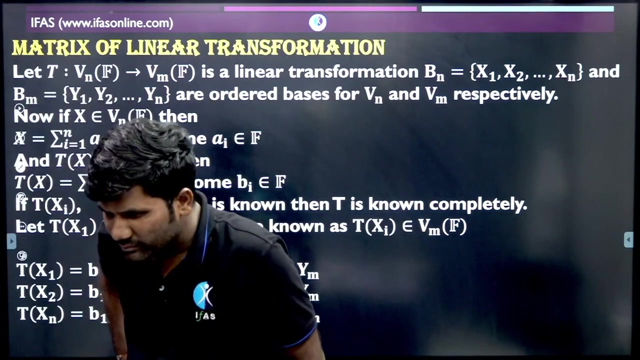 Okay, Let's come to the next question. Now, here is a matrix representation of linear transformation. How do we convert linear transformation into a matrix? That is what has been given. Okay, okay, okay, Pulkit, Okay, Pulkit. 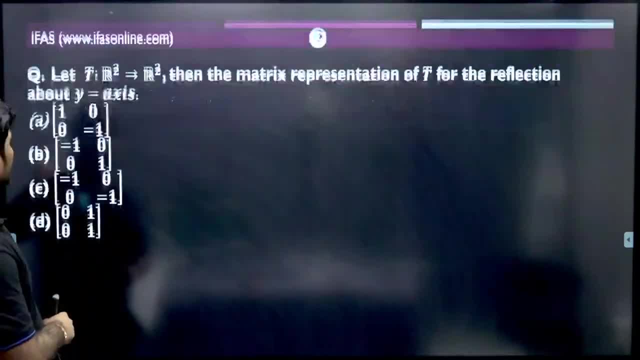 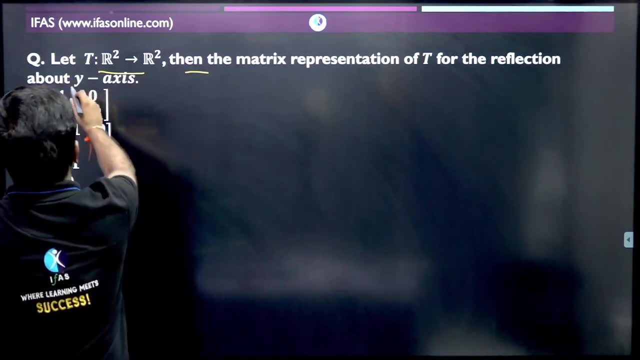 Pulkit, without counter example, No problem. Now what has been given here: Play T from R2 to R2.. Then the matrix representation for the reflection about Y axis. Now what has been given here? Matrix representation for the reflection about Y axis. 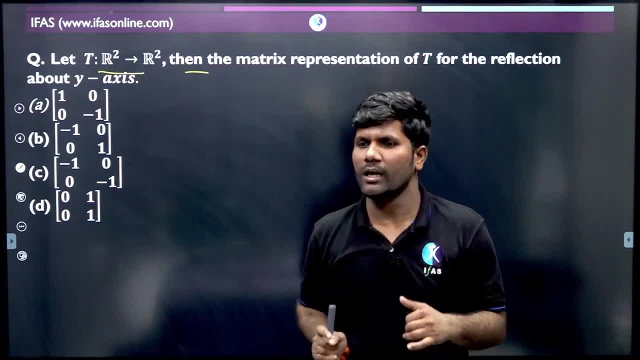 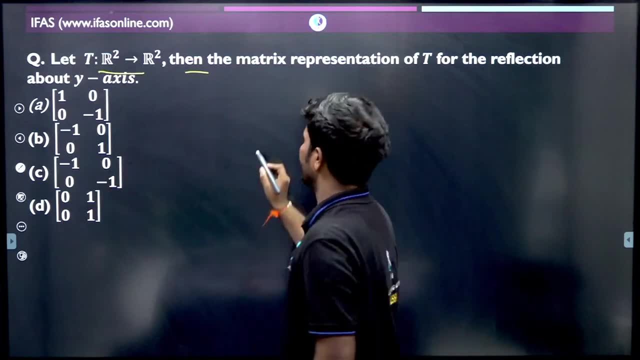 Now what do you have to do? Tell me T First of all. this will be our biggest work. We have to find T. How does T look? Now tell me who can tell how the map is defined here? What will we get T of A comma B. 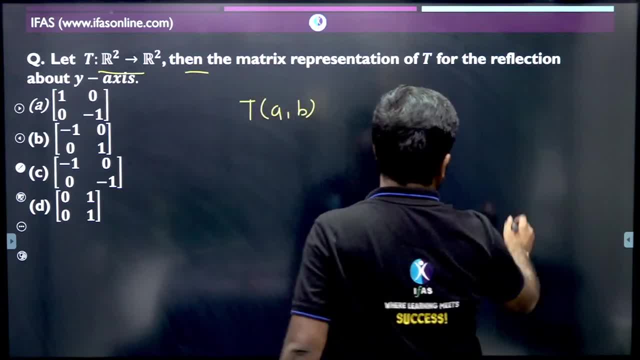 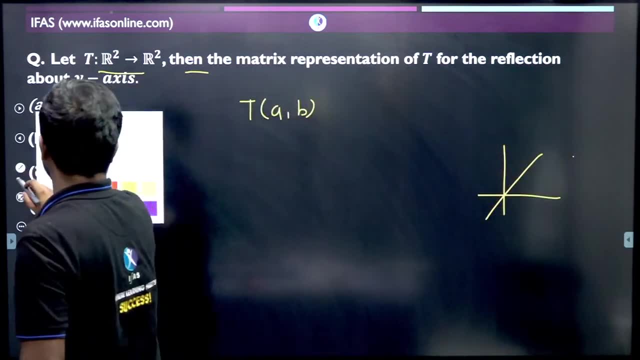 What has been given to us? Reflection about Y axis. About Y axis, You are taking any element, Whatever element it is. What will you do? You will reflect about Y axis. Okay, This kind of map has been given. So what kind of questions are there about linear transformation? 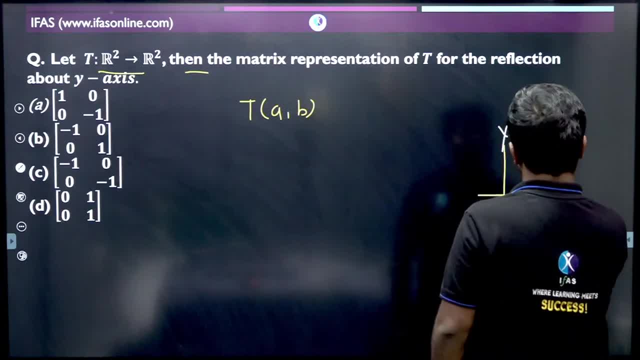 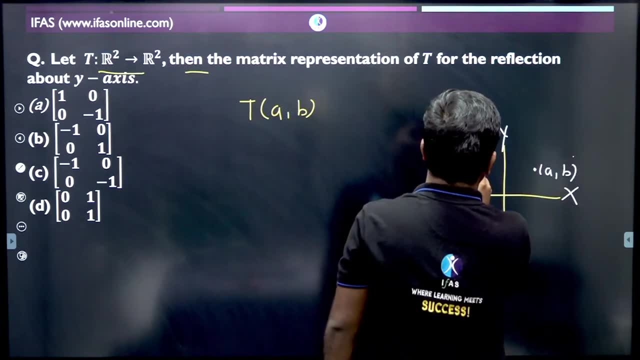 Okay, Here is the X axis. Here is the Y axis. What do you do Reflect with this? If any element is here- A, comma, B- When you apply T, it will reflect and come here. What will happen when it comes here? 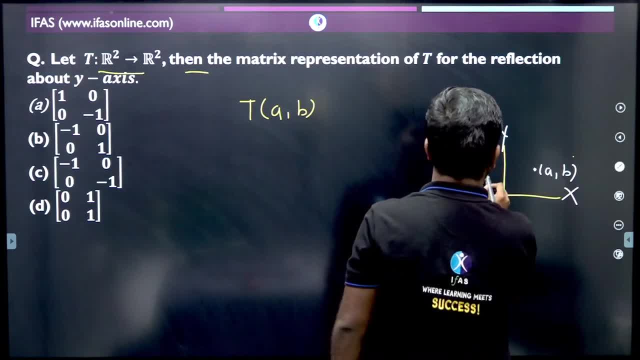 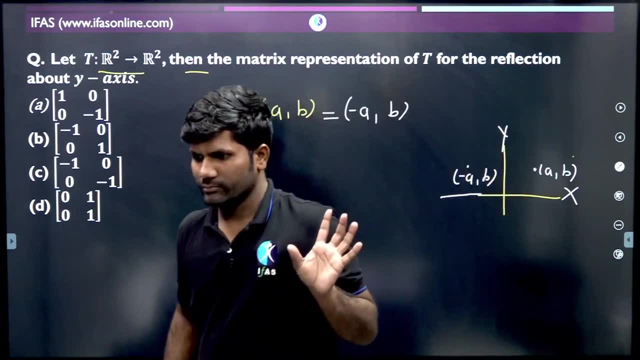 A will be B as it is Here, it will be minus A comma B. So where will T of A comma B be mapped? It will be mapped at A comma minus B. Now you can find it easily. Tell me. Kalyani says Sir. previous 5 years paper. 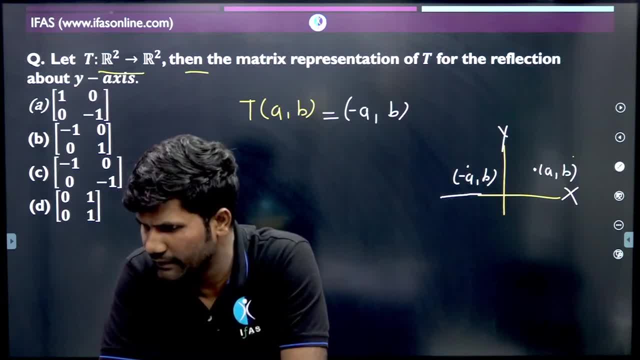 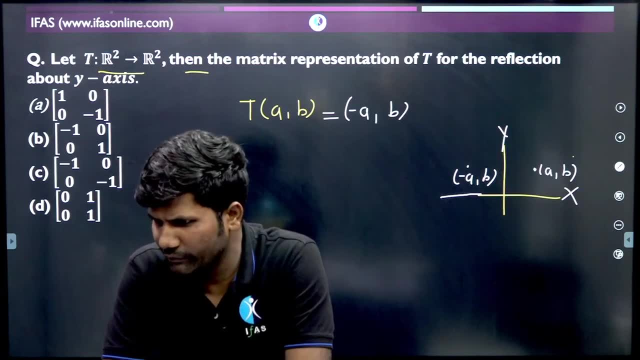 Are these studied videos of linear Vivek Priyadarshi? what happened? Where did you put your message? It has been put for review. Okay, Don't do anything. Okay, Bharti has also been put. Why are you putting? 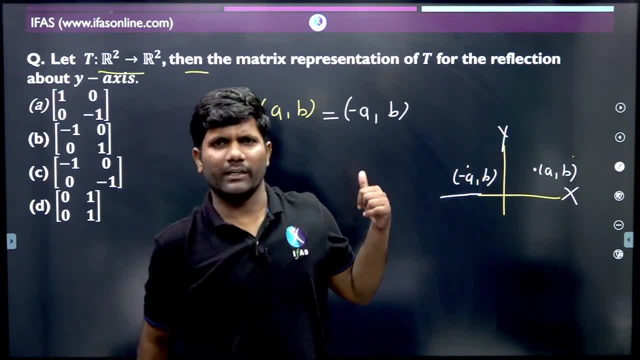 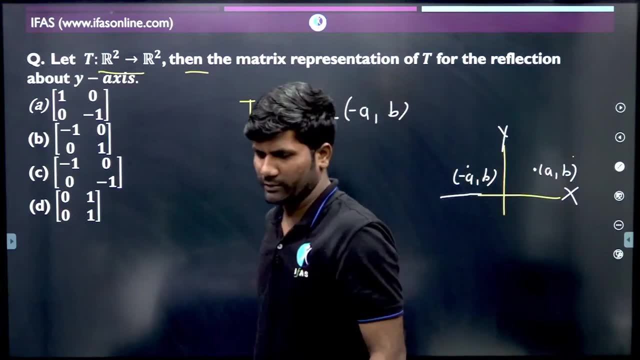 You are writing Yesterday. you should see the website once on YouTube. There will be some 3-4 years available. You are talking about. discussion is not available on YouTube. Okay, what are the rest of the people getting the answer to this? 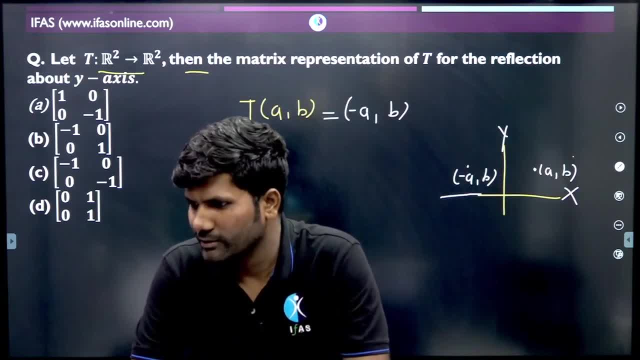 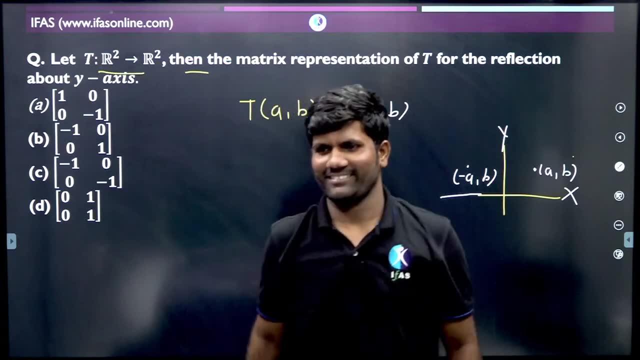 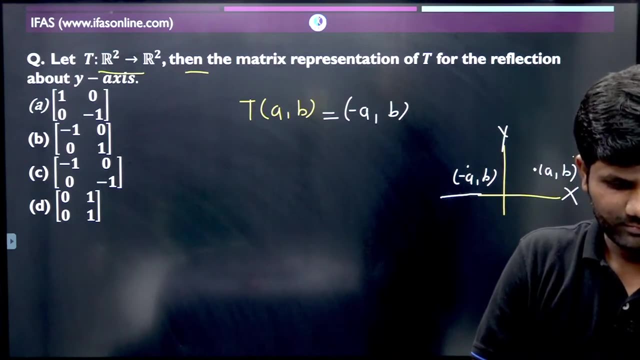 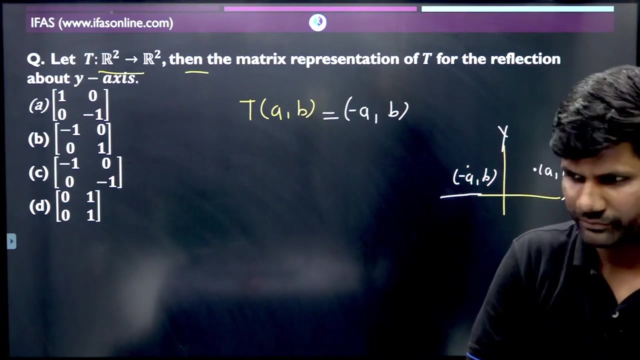 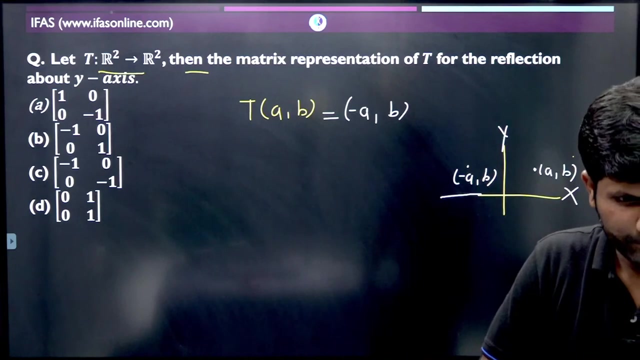 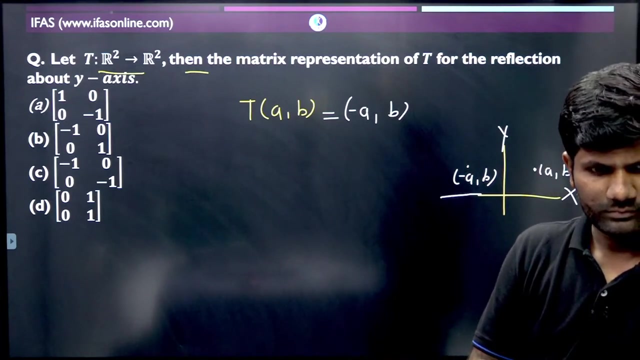 Very good, Bharati. Look, Bharati. now your review is over. okay, Tell me what will get the answer. Pooja Mohre B. Bharti Nagpal B. What are the other people saying? Say something. Neha Kumari B. 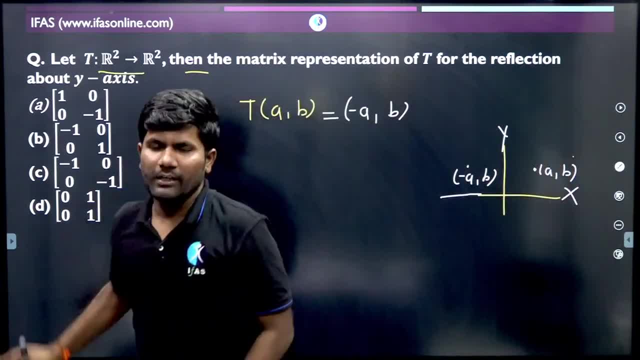 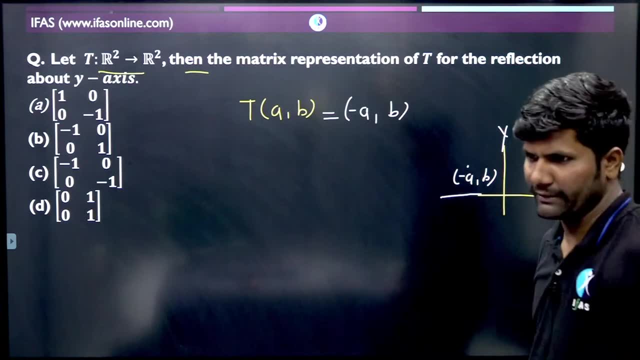 See, this is very simple, What we have to do here. If we are not given the basis, then what we have to take for the basis? We can take the standard basis. If the basis is not given, then you have to take it as a standard basis. 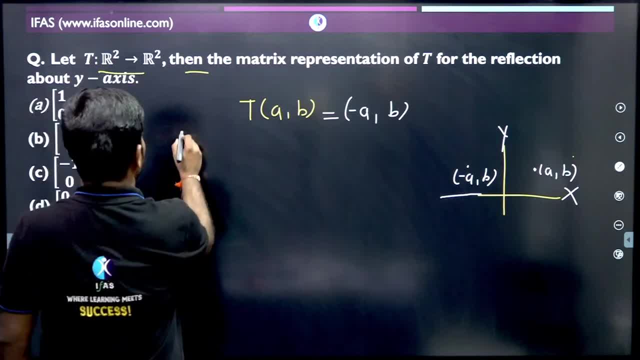 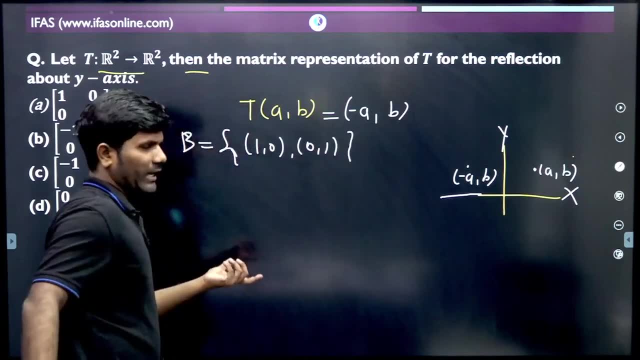 If you take the standard basis, then what is the standard basis of R2? This is 1, 1,0 And 0,1 is the standard basis of R2. If this R2 Is the standard basis, then with respect to the standard basis, 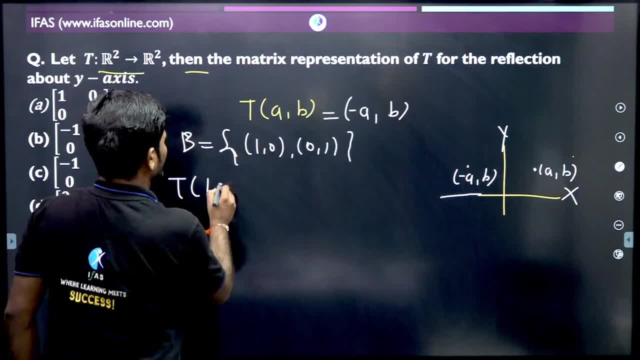 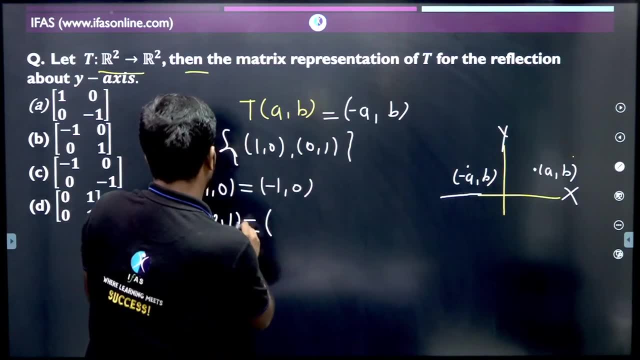 We have given you a map to convert. So where will the t of 1,0 go? It will go to minus 1,0. And where will the t of 0,1 go? Minus first couple, minus second, as it is, So it will go to 1,0,1. 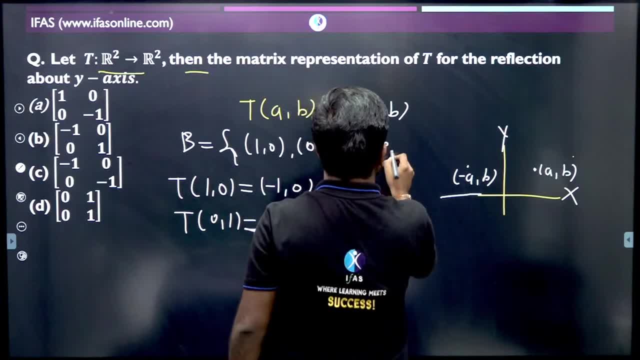 Now what you have to do is write in their linear combination. so let's assume this is E1, E2. What you have to do is write in the linear combination of E1 and E2. Now, in the linear combination of E1 and E2. 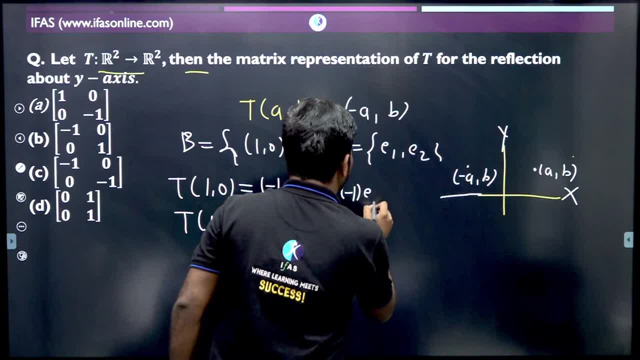 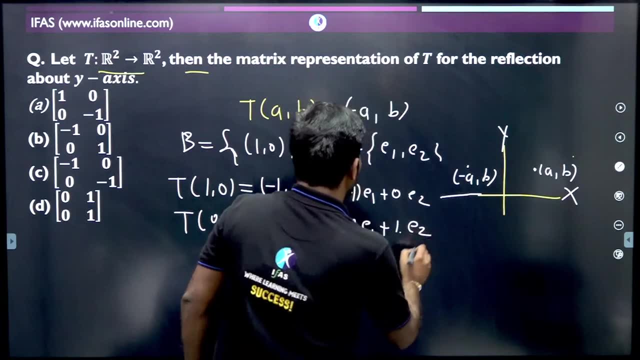 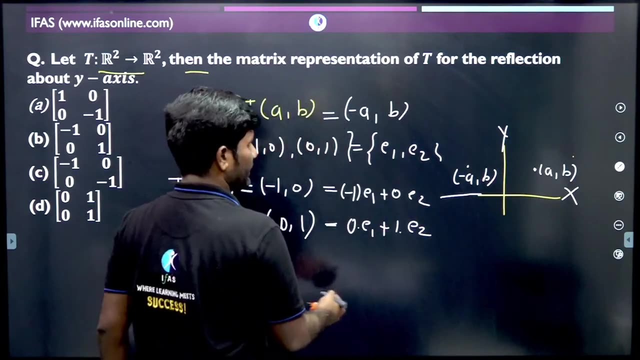 It is very easy to write How: Minus 1 times E1 Plus 0 times E2. And you can write this: 0 times E1 Plus 1 times E2. Now the coefficients here. Write them in the column. Got the matrix representation, So let's write: 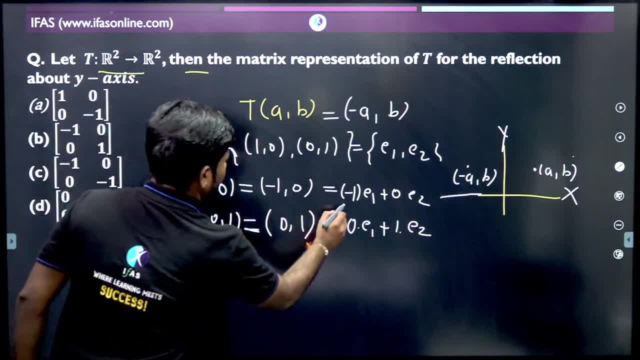 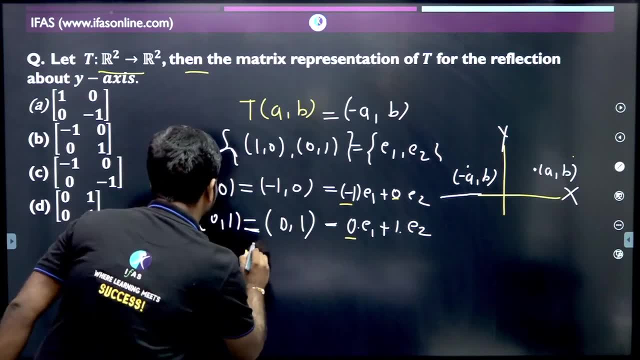 If you write in the column, then suppose the matrix you will get in the column. This is the first second element: Minus 1 is 0 And here 0 is 1 And 1. Now see which matrix is like this, See which one is. 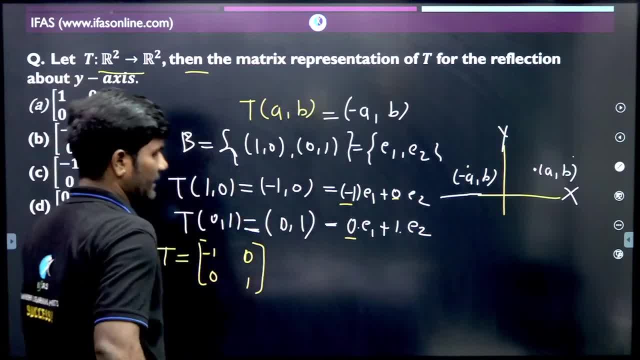 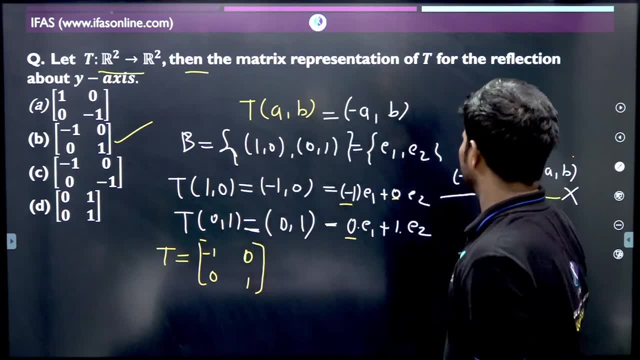 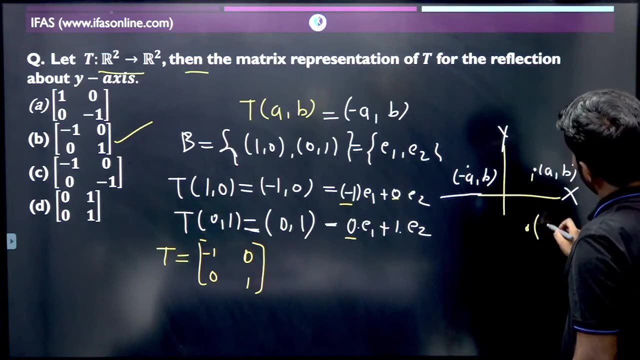 I think this is the B one. So this means what will be the option B Will be correct. Is it clear, Mayuri? when there will be a reflection on the x-axis, Then this point will rise from here and come here. If it comes here, So now it will be as it is. on A, what will be B? it will be minus B. 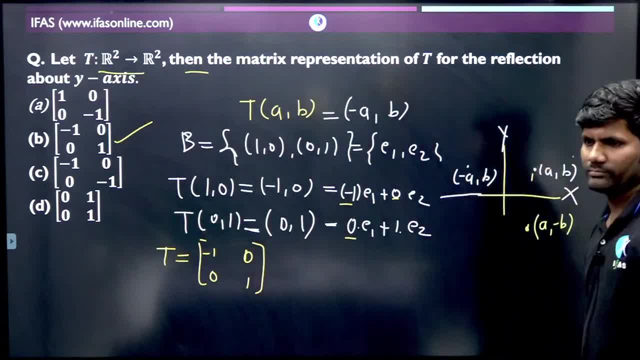 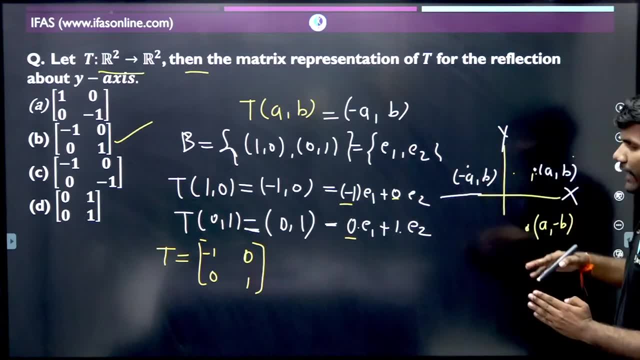 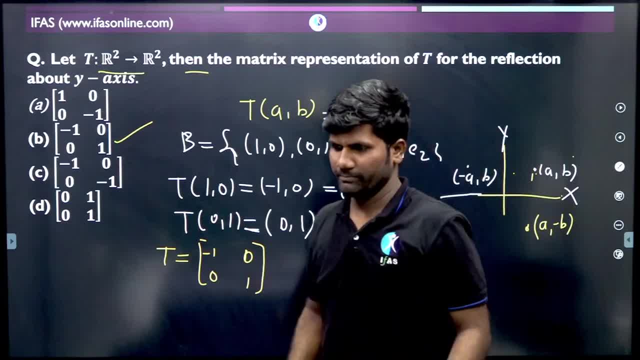 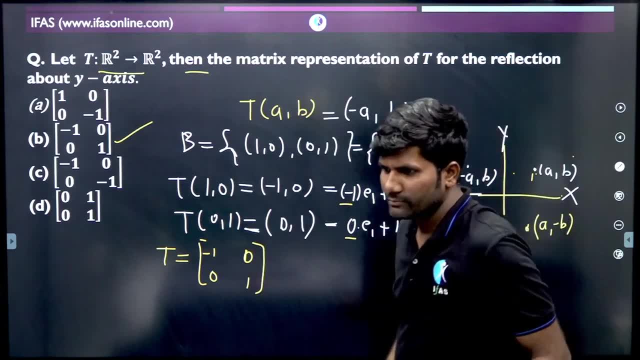 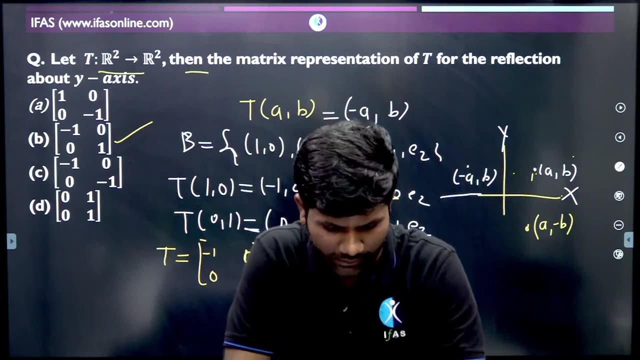 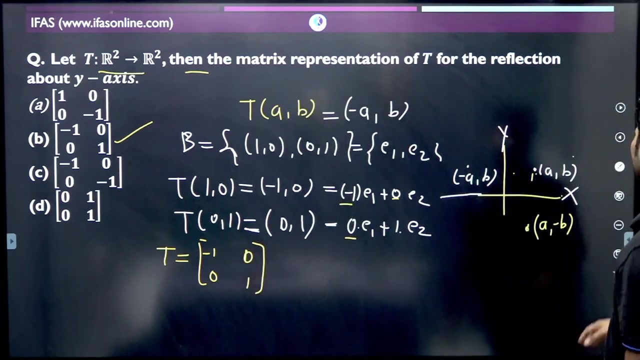 Lower point will go up Reflecting: Ok, Clearing up to this point. Fulkit will work now, Don't worry. Ok, Be prepared, It will work till 7 PM, no problem, Lets go Next, Fulkit. There are a lot of questions to be done. Let's come to the next slide. 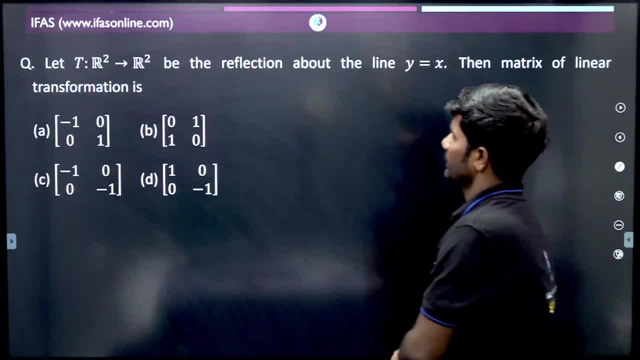 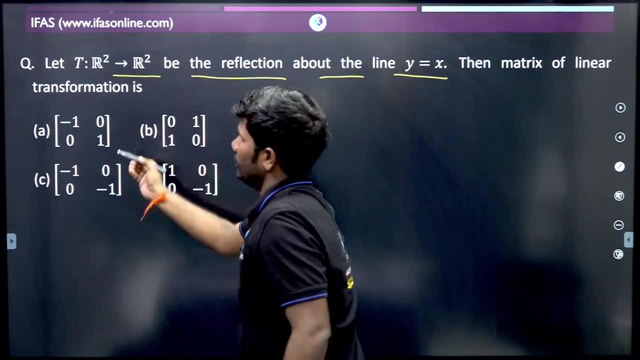 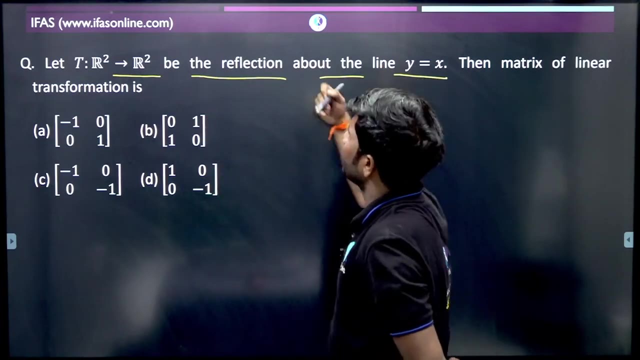 You will definitely like something in today's session. Here we are given T from R2 to R2 is a reflection about the line Y is equal to X, Then we have to tell the matrix of its transformation. Bharti, tell me one thing Now: how will you define the map of its reflection? 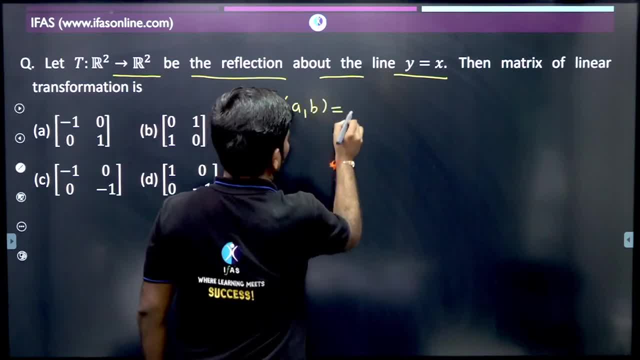 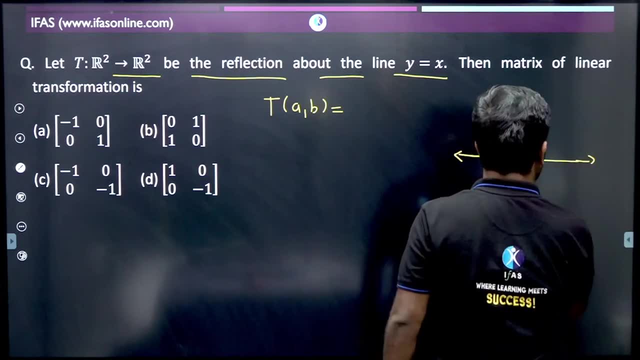 So what will be T of A, B here? Now tell me one thing: Now we have to take the reflection here, But now we don't have to take it on X axis and Y axis. Now where do we have to take it? It went that side. I don't know where it goes. 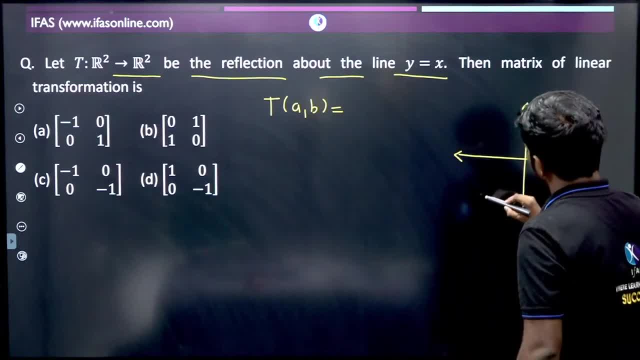 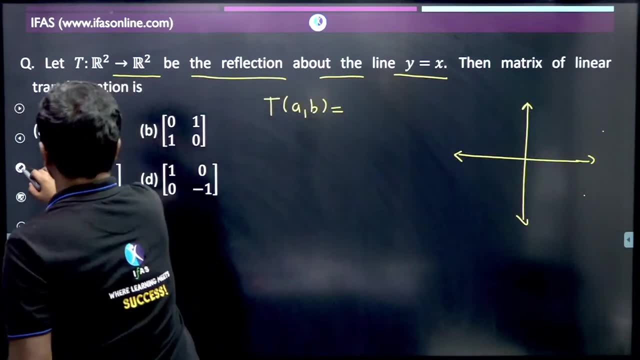 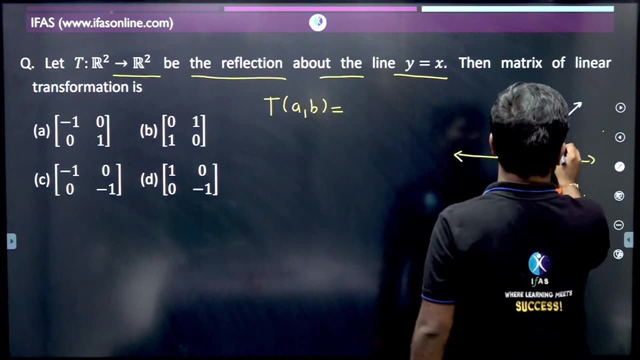 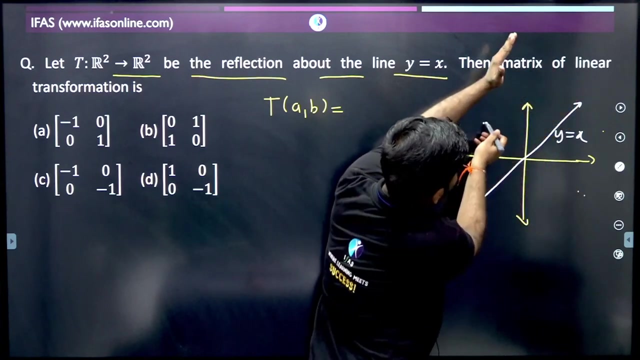 Now, where do we have to take it? Y is equal to X. So this is Y is equal to X. This should come in the middle. This is Y is equal to X. Now. Now I have to take it as the main axis and reflect it here. The elements here should reflect like this: 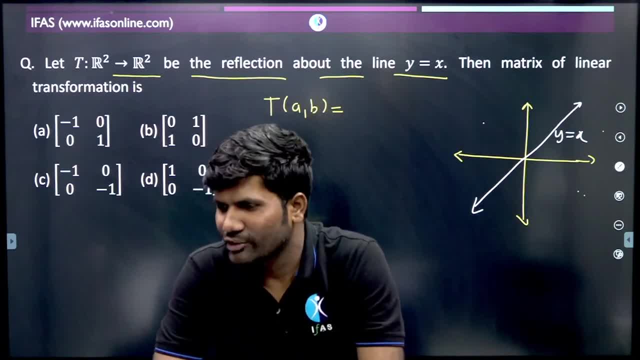 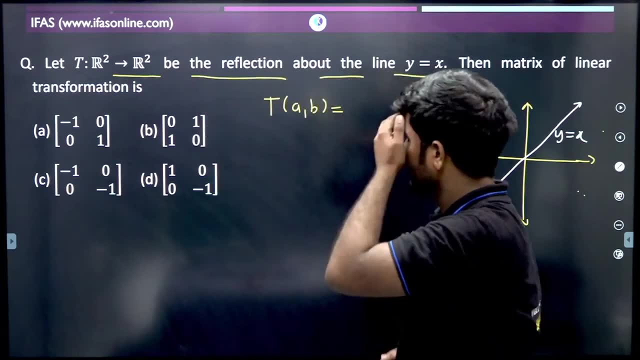 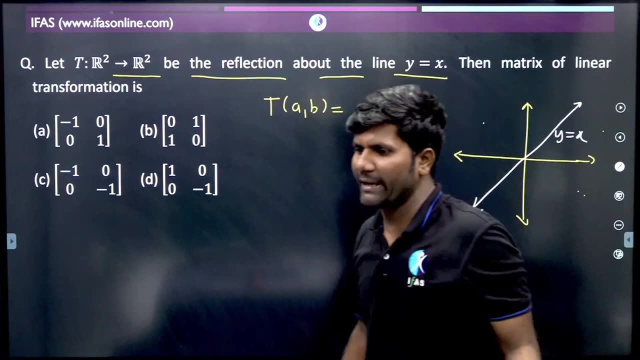 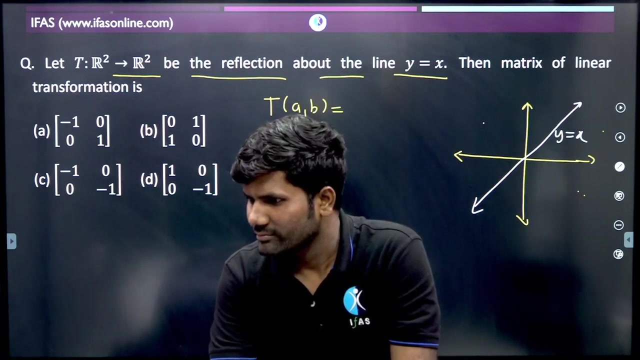 Now tell me what will you get. So go to 6.30 Pulkit, No problem. Till then, read: Akansha has given the answer. Akansha first, tell me the map. How will the map be? Tell me how will the map be? Bharti, Bharti. 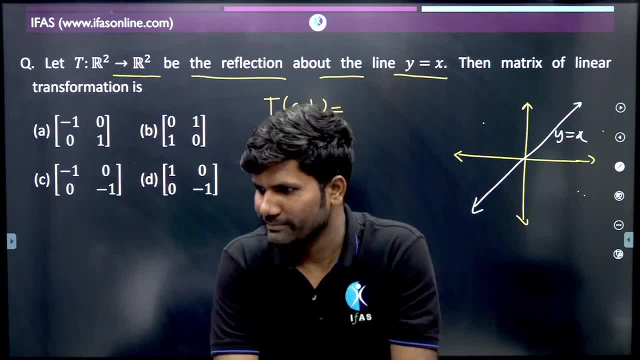 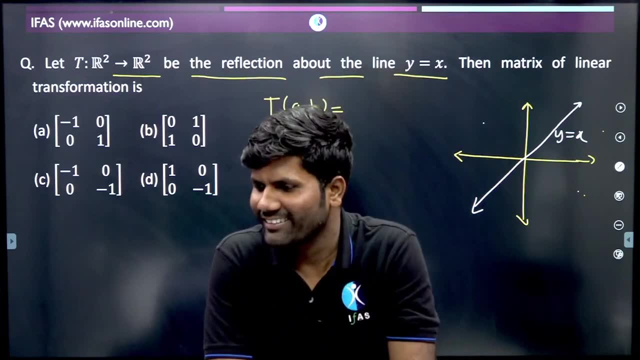 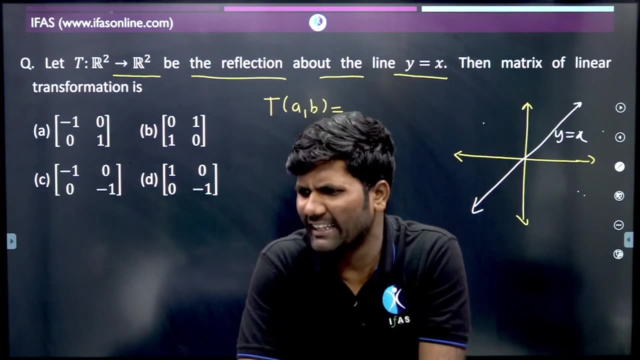 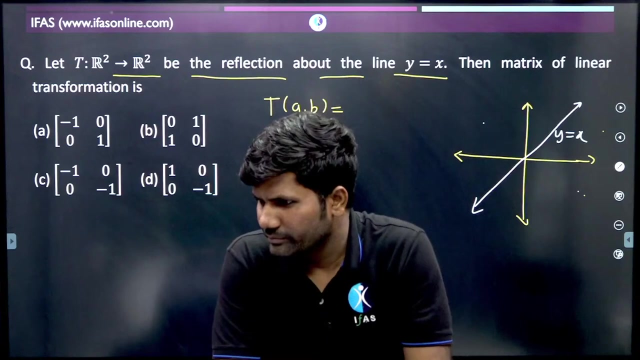 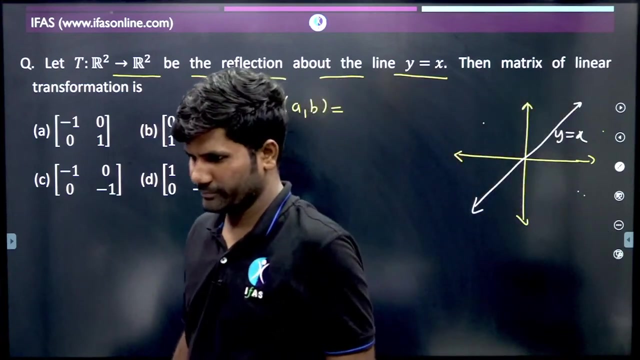 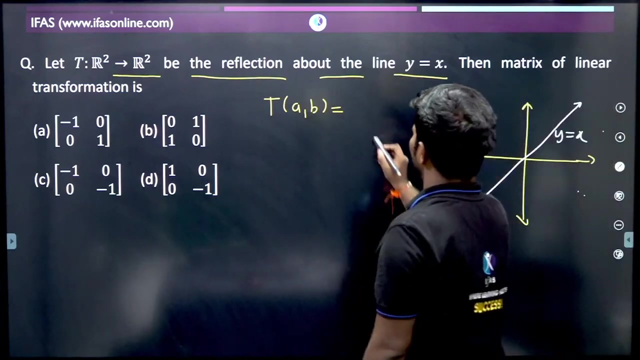 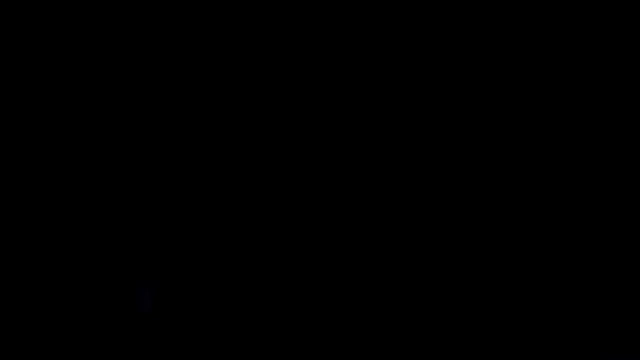 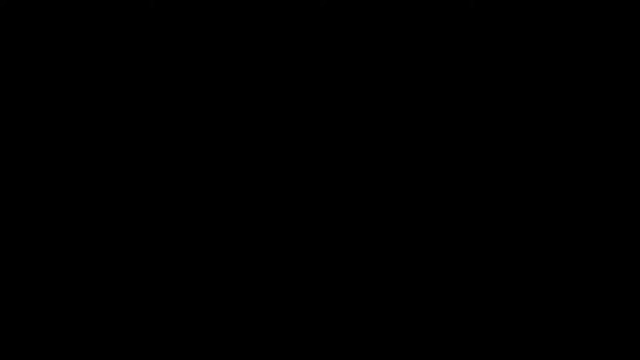 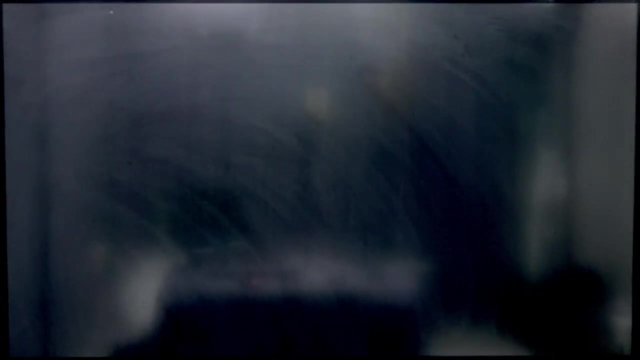 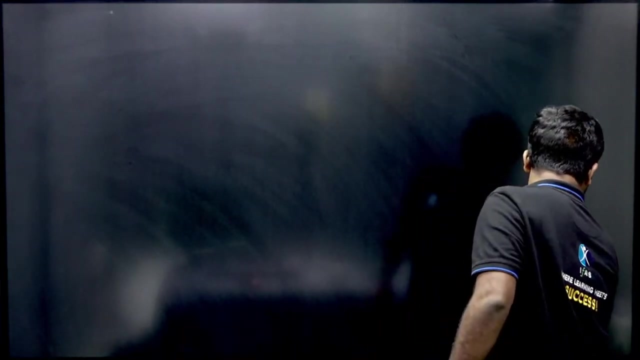 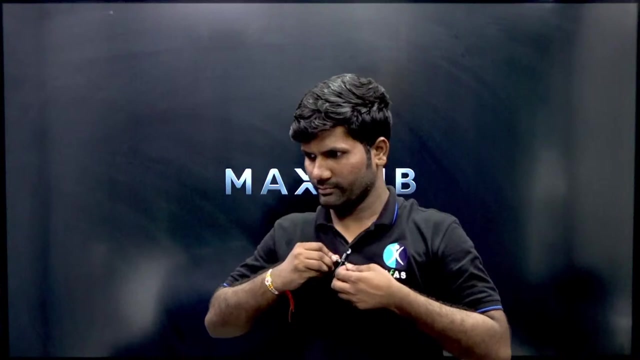 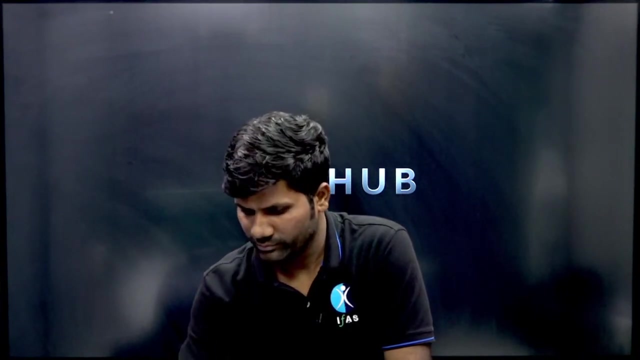 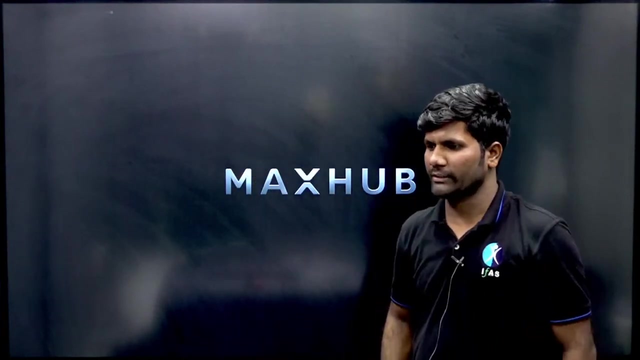 Subtitles by the Amaraorg community. Subtitles by the Amaraorg community. Hello, hello, Are you getting the audio and video? Just wait, we will continue. Okay, Let's just turn on the smart board once We will have to do everything again. stop. 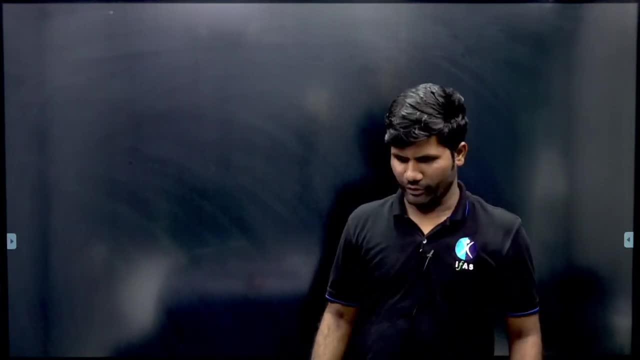 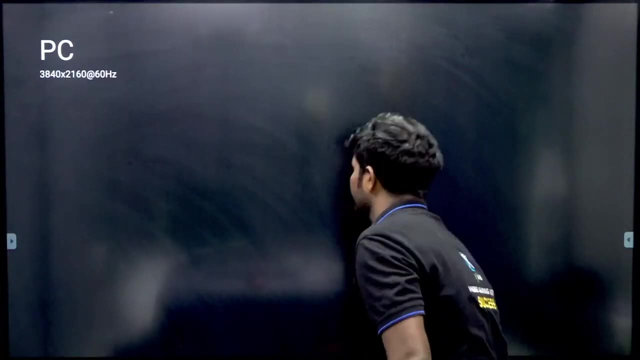 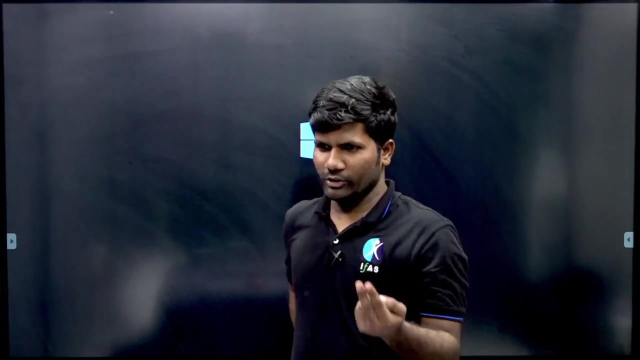 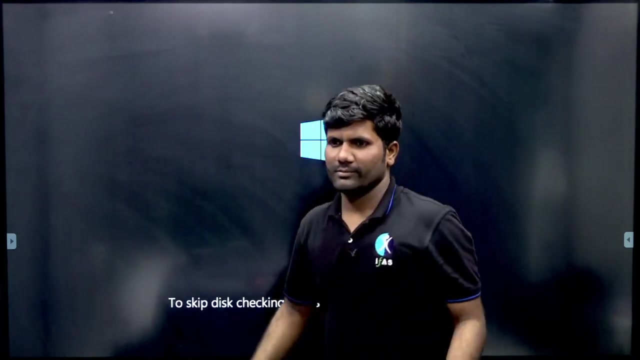 Yes, yes, the light went off. that's why it will work. Wait, now it will come. it will come. Stop, It is turning on. Yes, you will get the title in just two minutes. Okay, Now I can see it right. You guys at least do it live once. 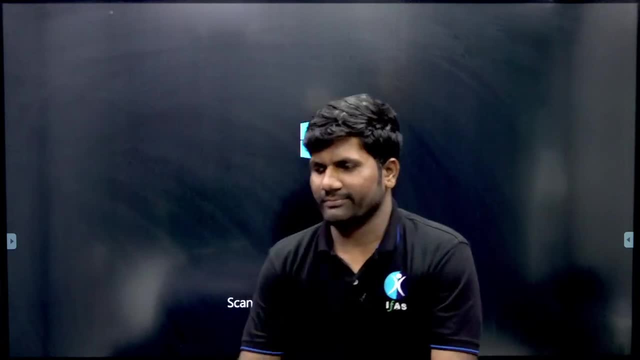 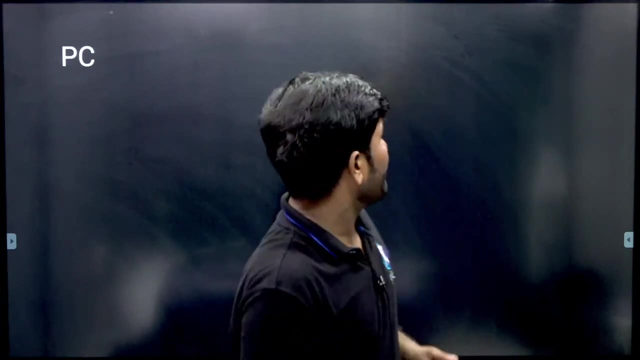 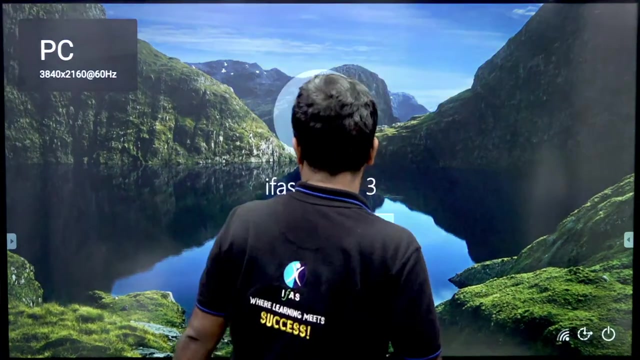 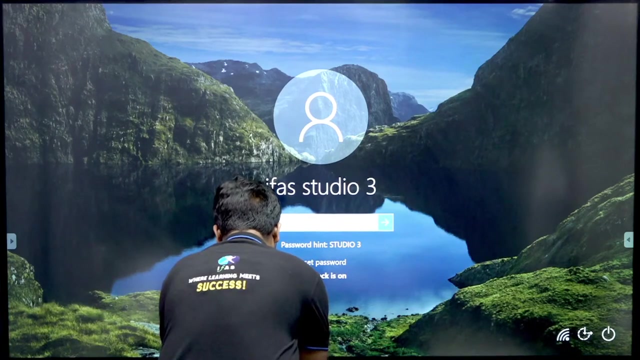 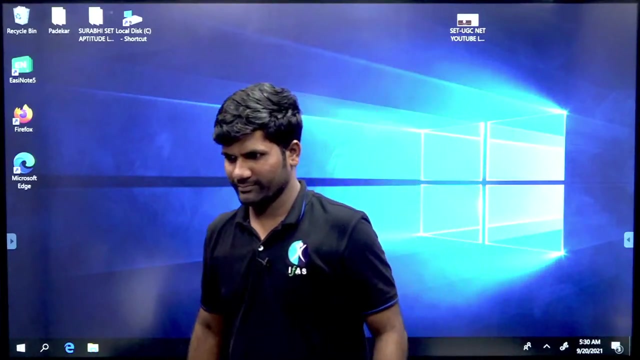 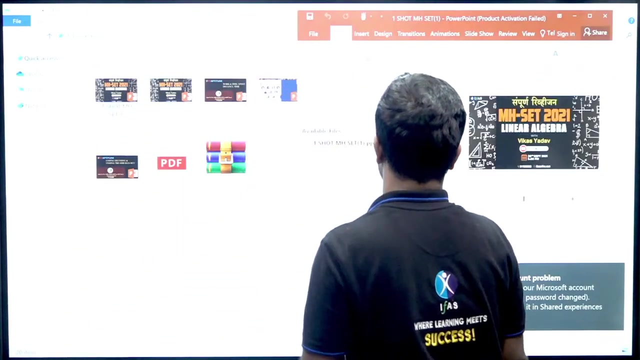 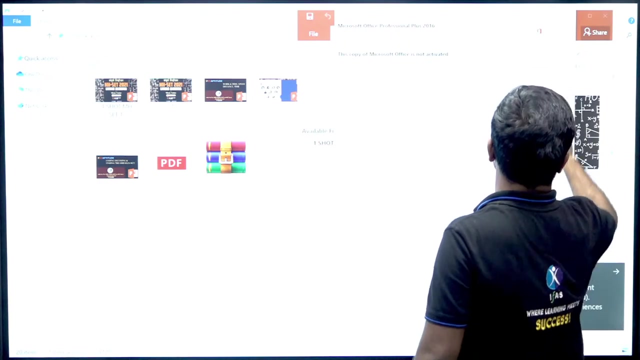 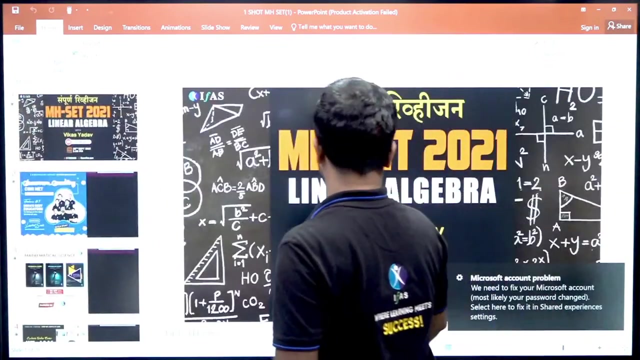 You are going back a little, So Is everything clear for you guys so far? Yes, Let's get back. if you want to Wait, we are going continuing. okay, Press switch, Click. Okay, Done. We were on the same slide. Now we are finished. 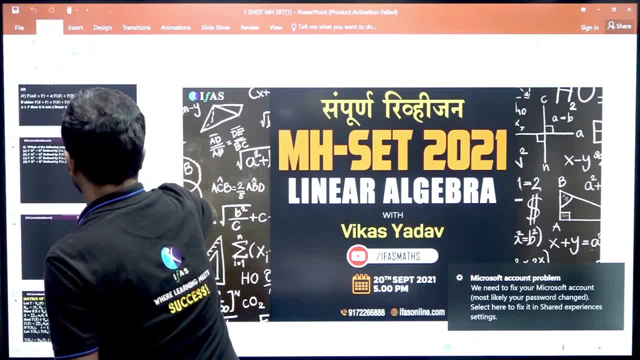 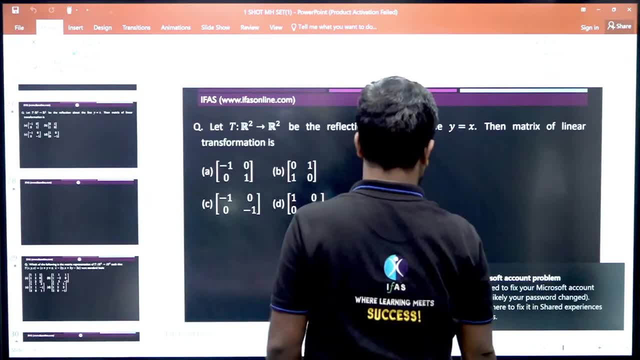 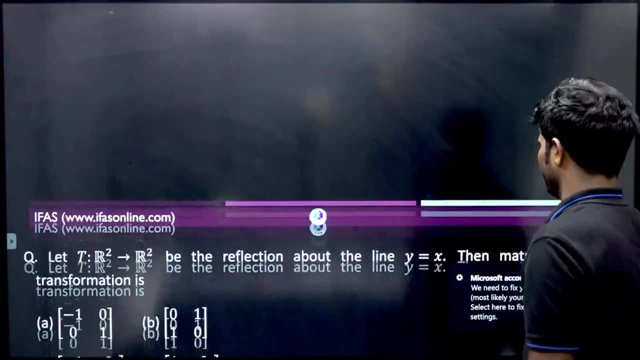 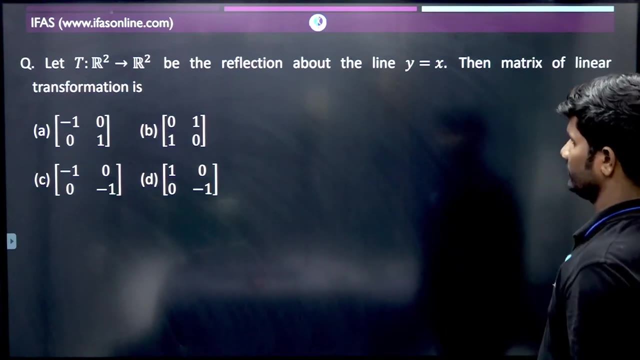 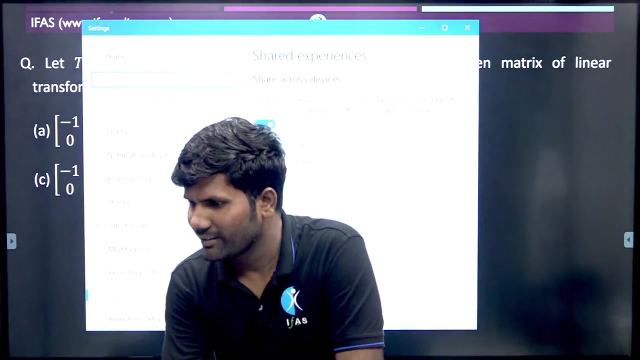 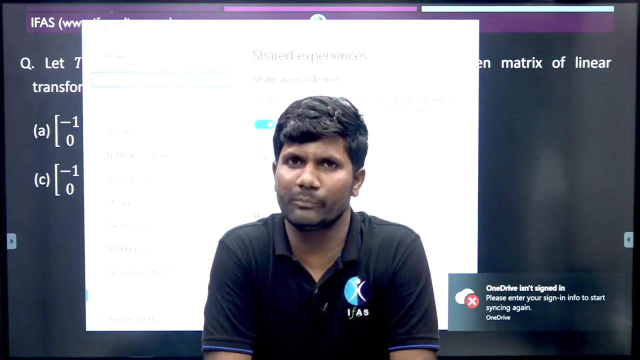 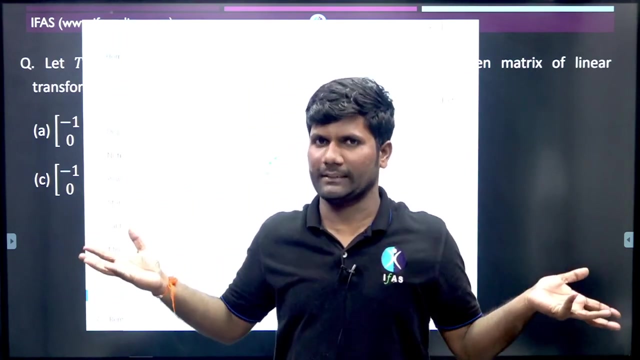 Okay, Can you see it? now? This too, Karim. I am telling you if we are talking about the basis. what is the basis? It is the subset of vector space. Okay, We make vector space with the linear combination of the elements of the basis. 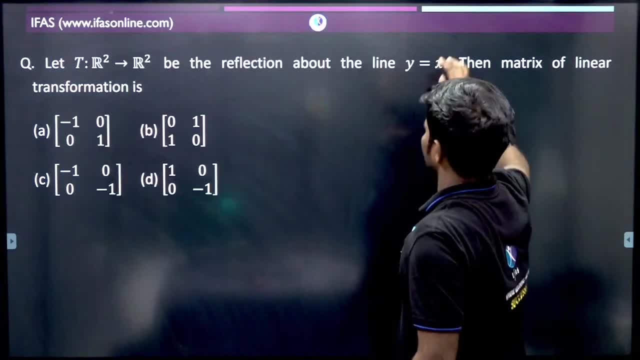 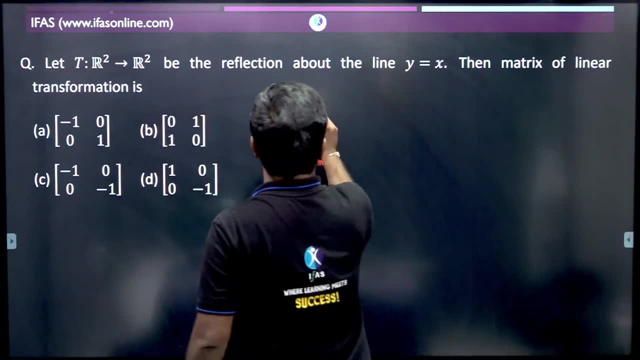 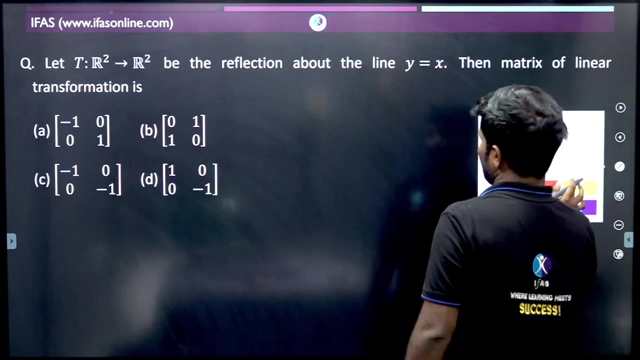 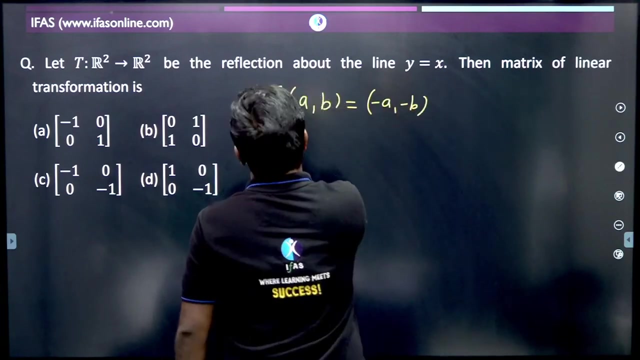 Okay, Okay, Come here. Now, come here. Let's continue here. How was the map here, The map given here? how was f It was? Now tell me the map here, the linear transformation. how will the matrix be? 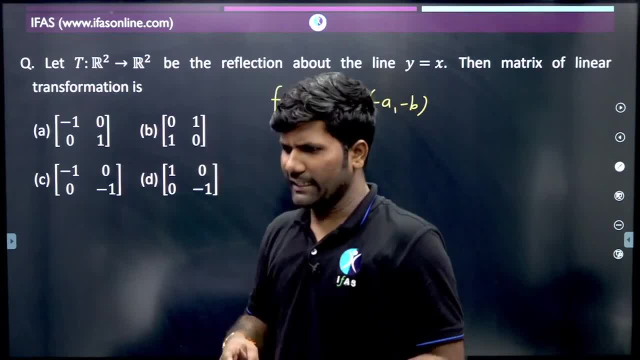 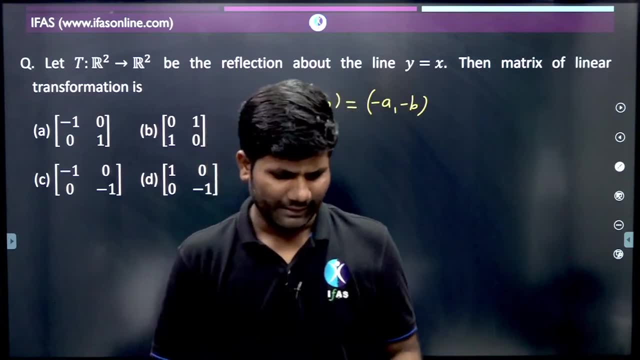 Okay, let's do as much as we have. Let's see what will happen on this. There is a formula for rotation. If you keep that formula in mind, then you can do the whole rotation, Okay. Okay, now let's do a lot of things. 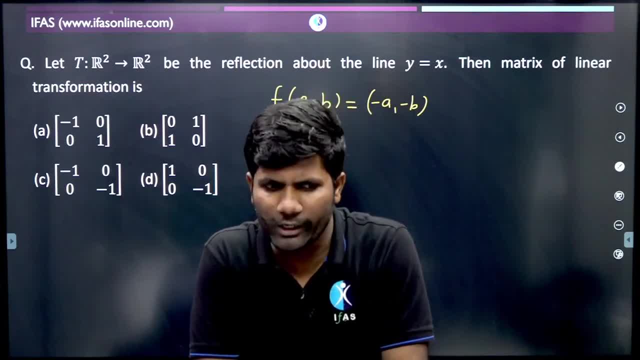 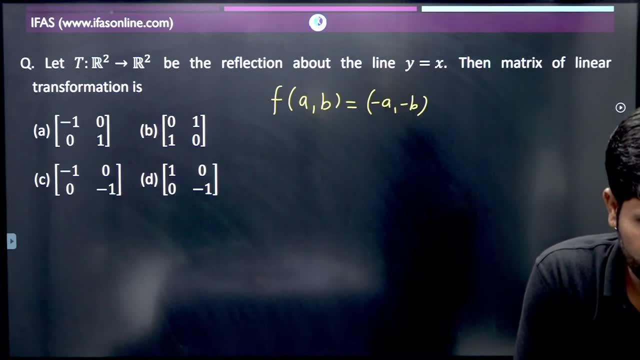 In today's lecture. Now tell me, is everything clear? Is there any problem with the audio and video? Tell me once. I feel like you are looking back a little bit. Do it live? Okay, Now go and say: 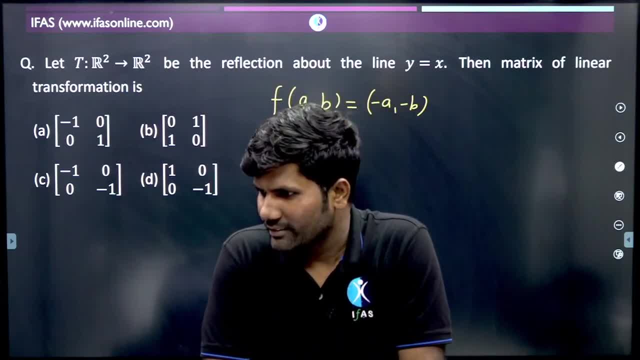 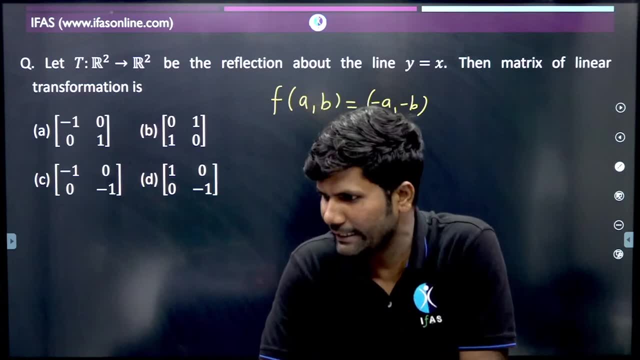 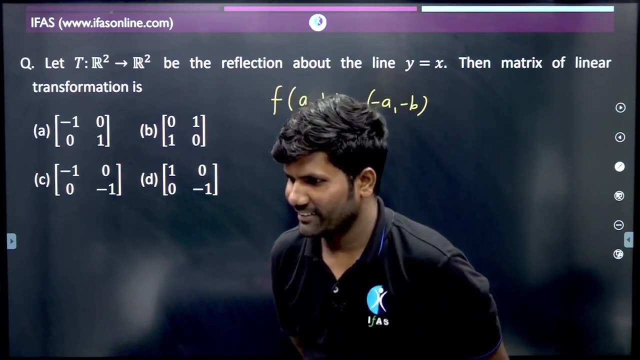 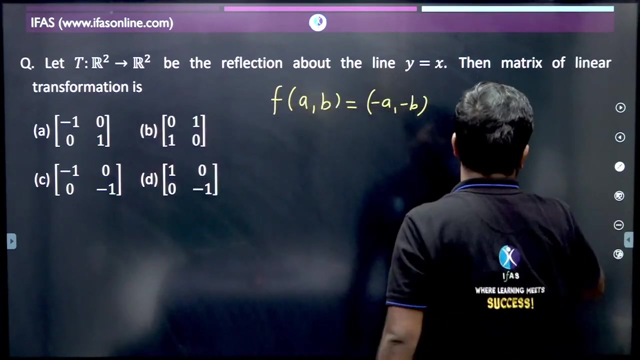 everyone has liked it. Mayuri Sonao has said it four times. That means so much confidence. Okay, Very good, Mayuri. Now let's go and see. 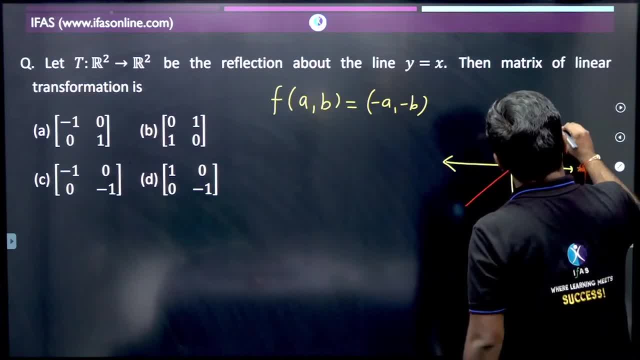 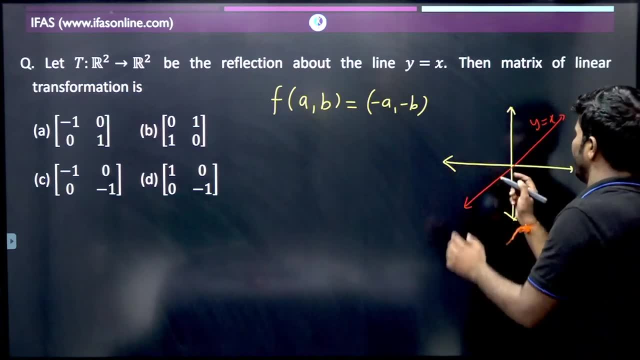 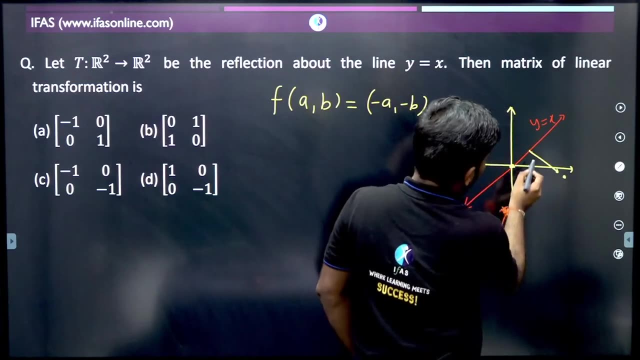 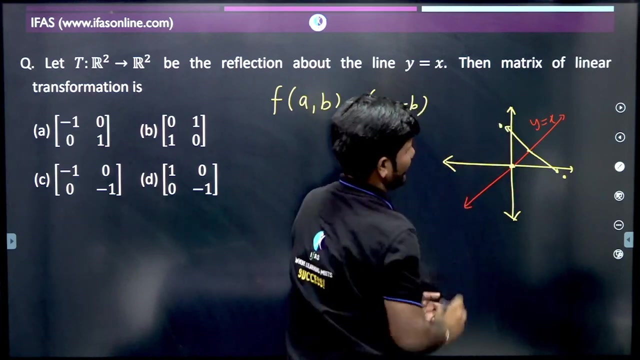 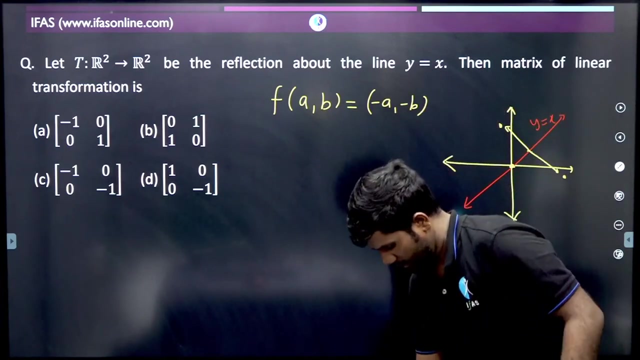 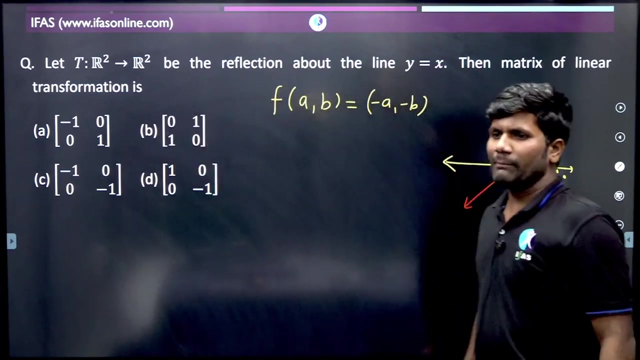 we have given basis, we have not given 1,0. 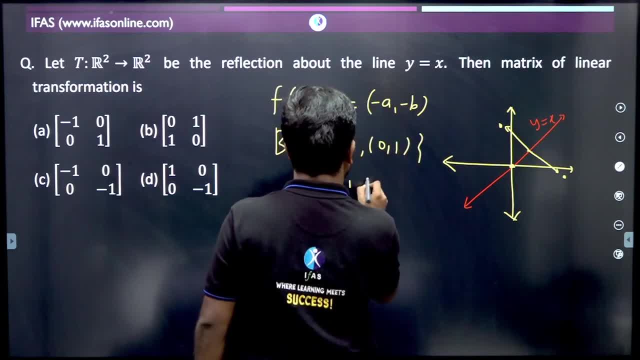 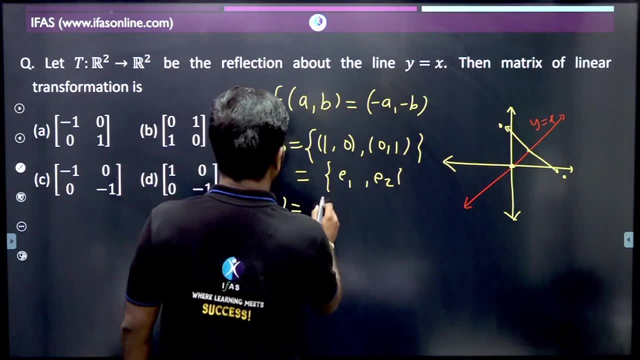 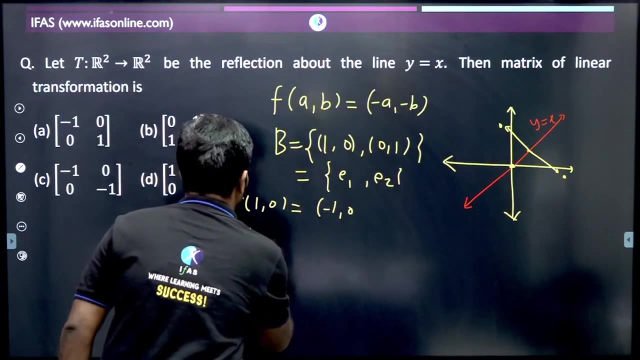 so we will take standard basis, which you call E1, E2, with love. if you convert in matrix, then t of 1,0 we will get minus 1,0, and and t of 0, minus 1, 0, minus 1. 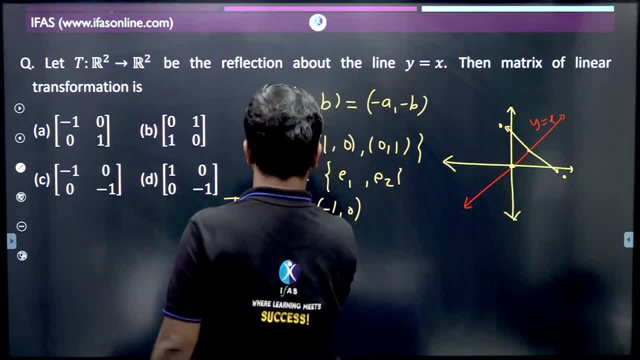 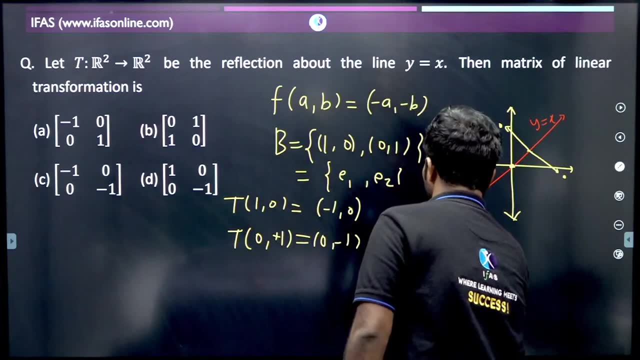 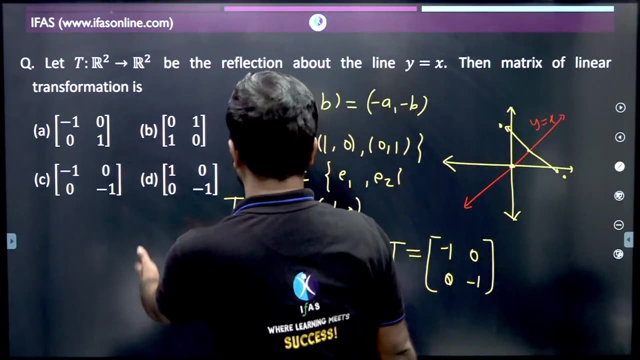 what will we get? we will get 0, plus 1, not minus 1. we will get 0, minus 1. if you convert in matrix, we will get minus 1,0,0 minus 1, so we will get A. so what will be the correct answer? 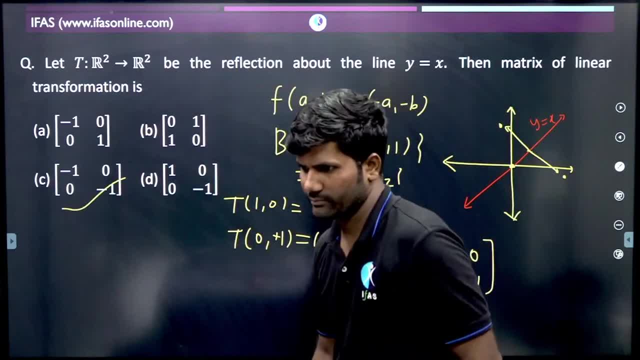 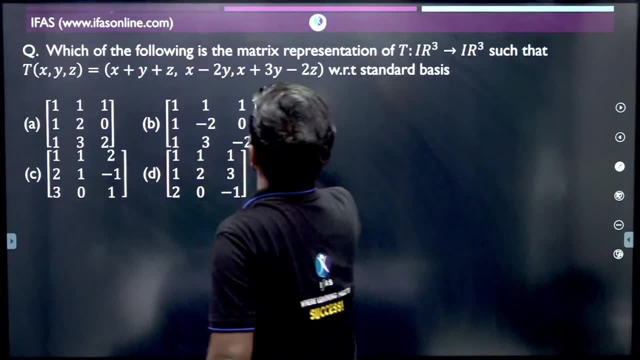 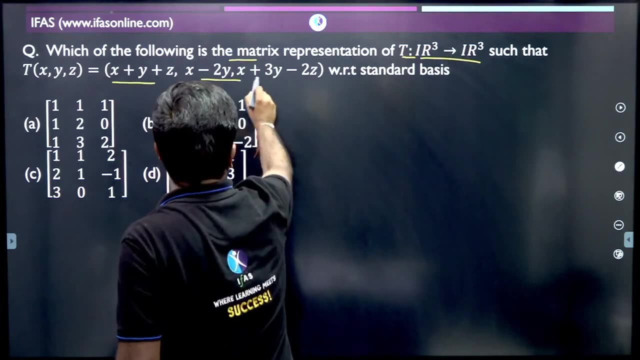 we will get C, so option C will be correct. ok, let's go now. here we have one more question. which of the following is the matrix representation of R3 to R3, such that we have given this? ok, now tell us if you convert in matrix with respect to standard basis. 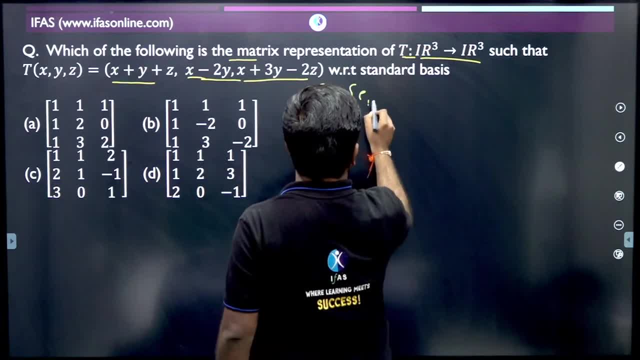 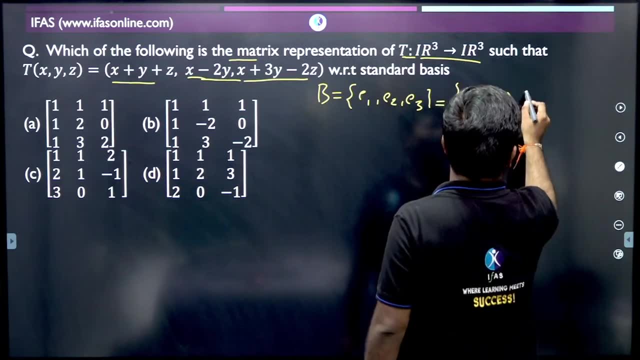 so what is the basis of R3? basis of R3 is E1,E2,E3. so here, what is E1? we have given E1 is 1,0,0, E2 is 0,1,0 and E3 is 1,0,0,1. 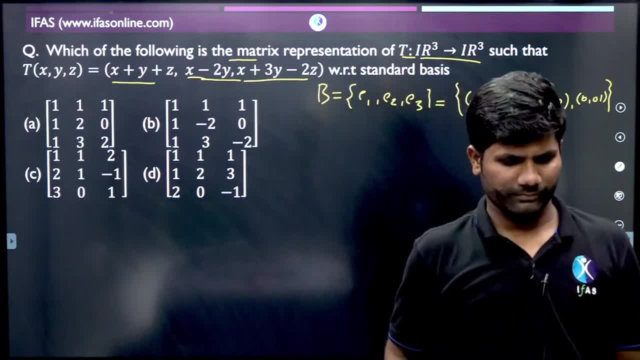 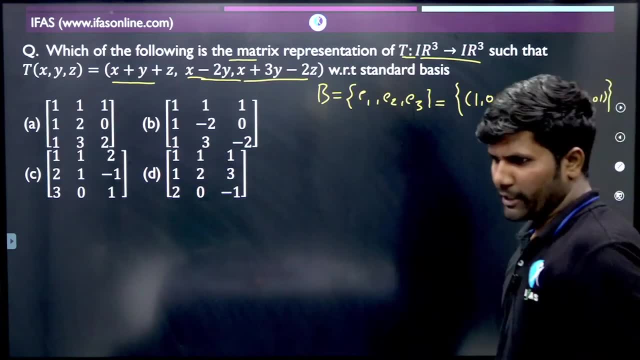 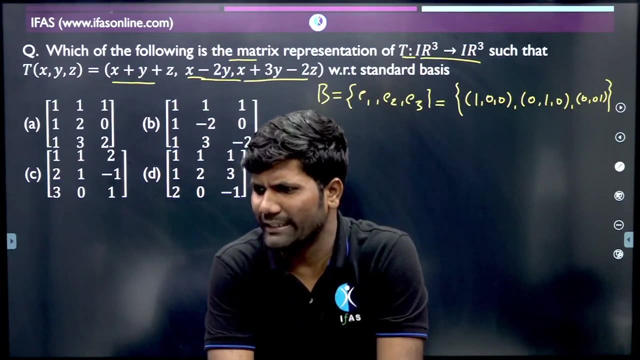 now tell us, if you convert in matrix, what will you get? tell us, we will do first, we will do this much in today's slide and you will get one or two lectures where rotation will also be there in linear transformation. I have taken one lecture series. 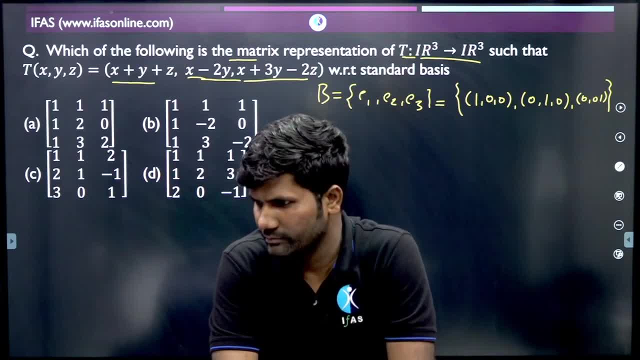 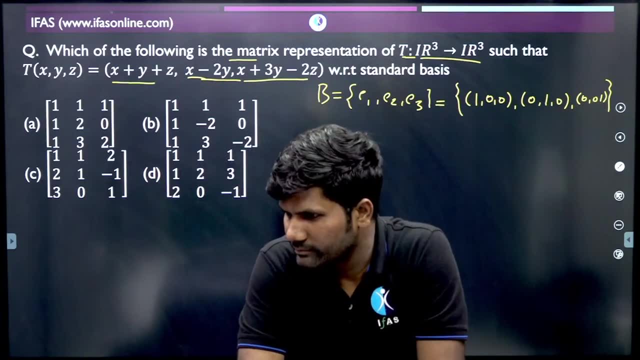 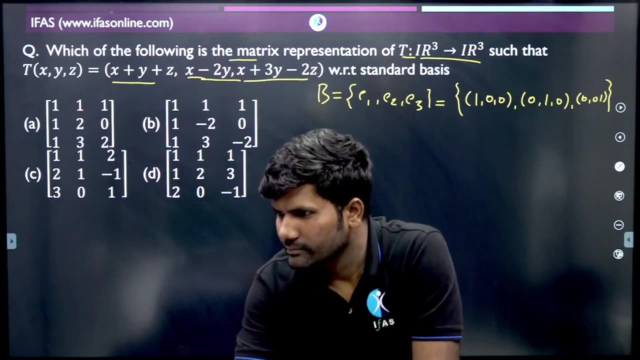 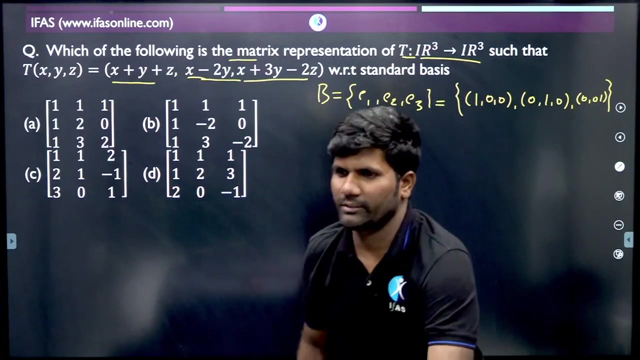 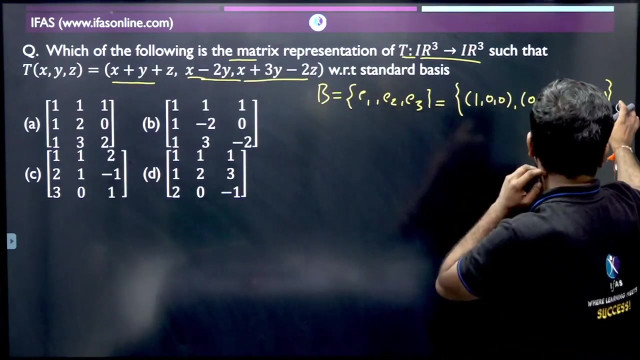 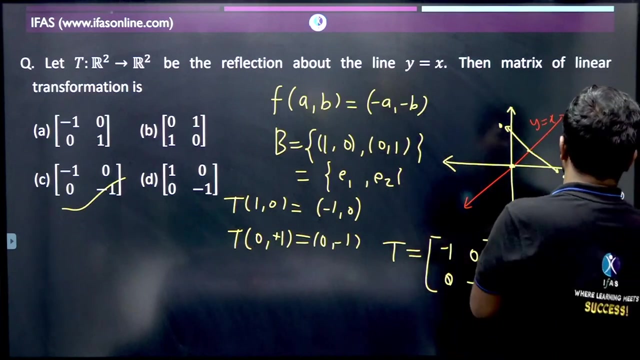 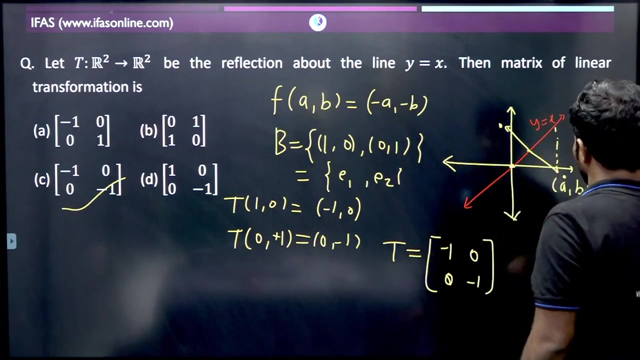 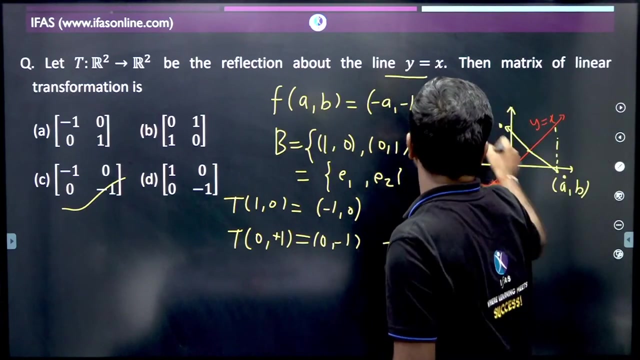 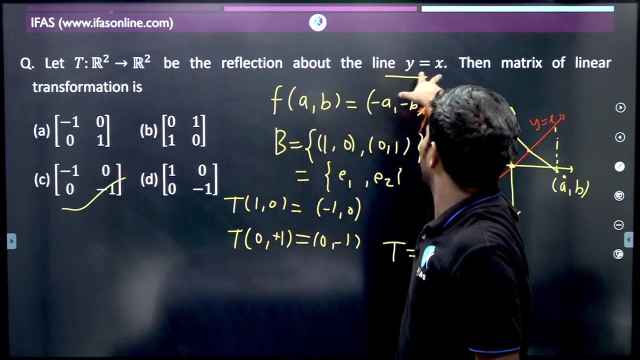 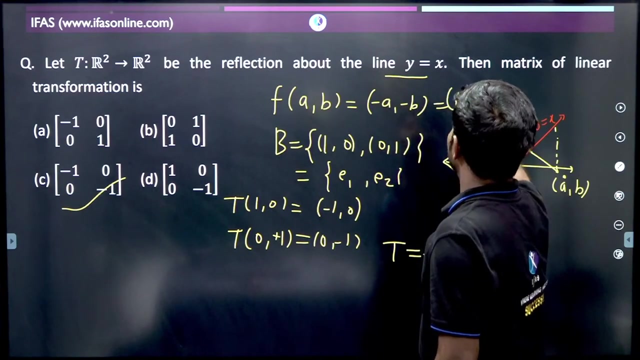 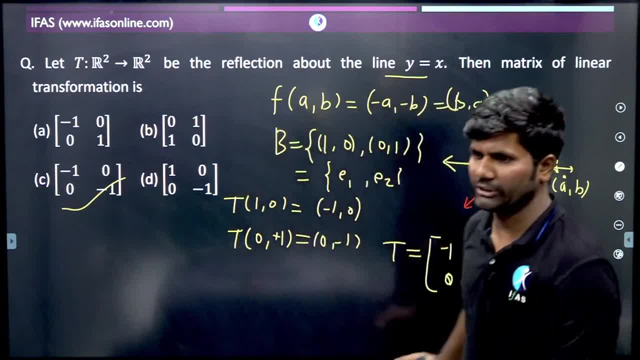 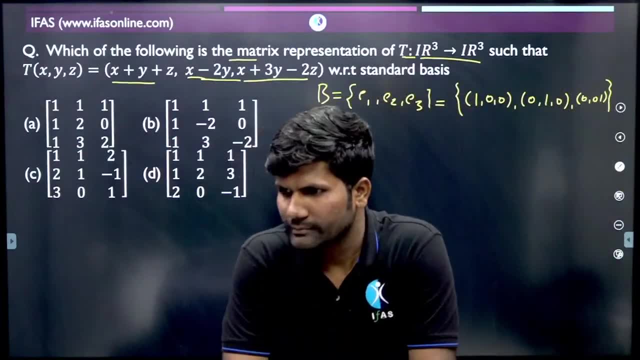 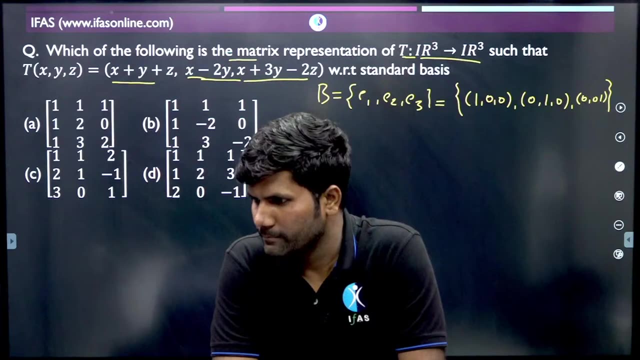 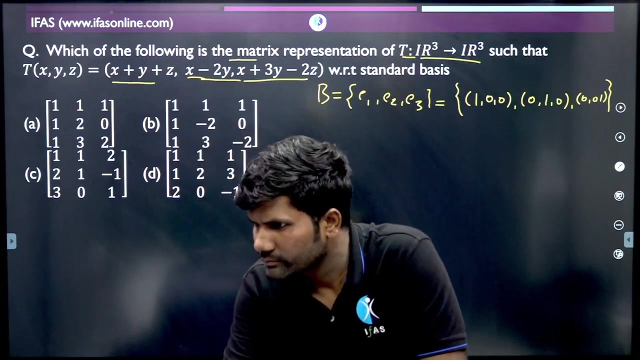 Okay, Come on. Okay, Let's come to the next question. Now convert here and tell me: Okay, Deba, Okay, Yes, Bharti, Bharti. And who told you: Very good, Bharti, Okay. 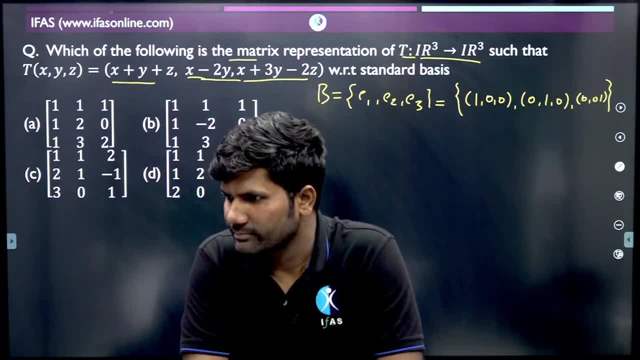 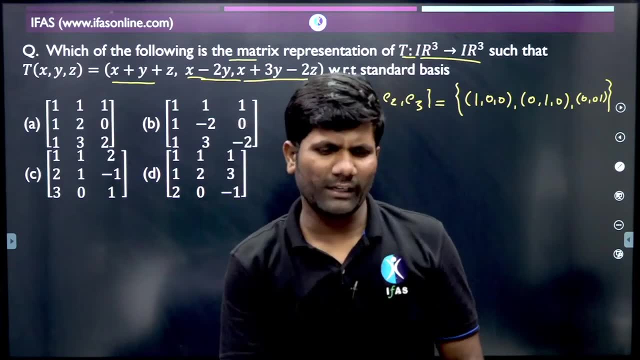 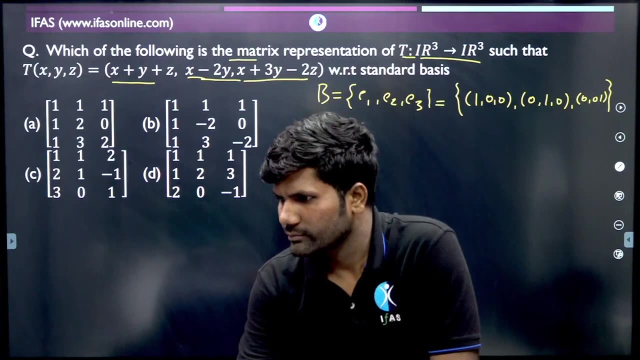 We have seen till the end. Okay, Okay. What is the answer to what the rest of the people are getting? You guys solve it. It is a simple question. You can solve it easily. Okay, Sital B: almost everyone is telling B. 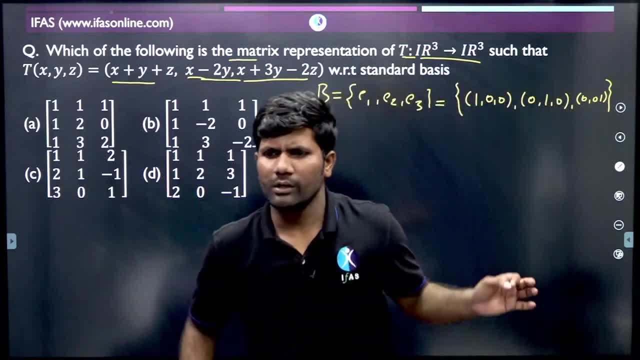 So it means that it will be B only. Okay, So you can do this. So this is a homework for you. I will tell you: Convert in the matrix. If you have given the map here, then you can do it easily. 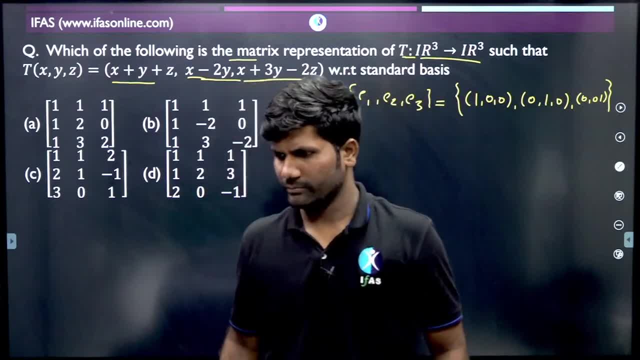 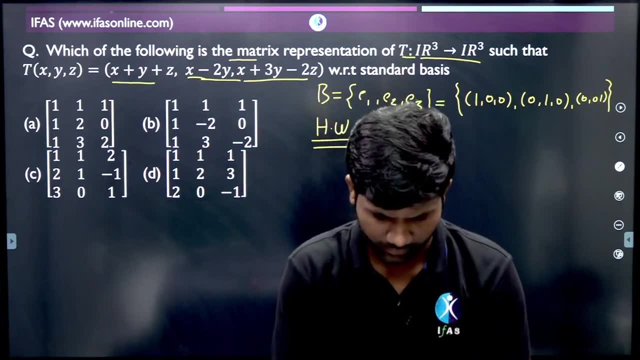 We will go ahead. There are some more questions. Let's do that. Okay, All students are clear. Come on, come on. So come on. This is homework for you. Let's come to the next slide. Okay, Okay. 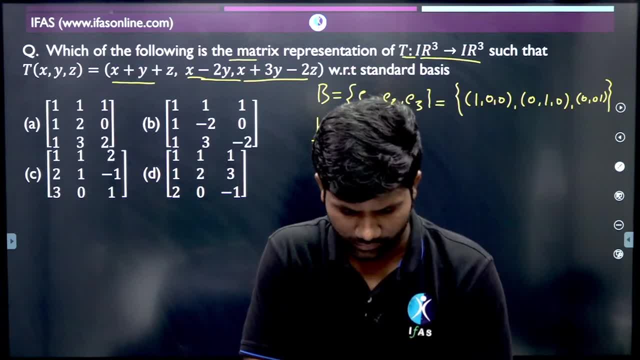 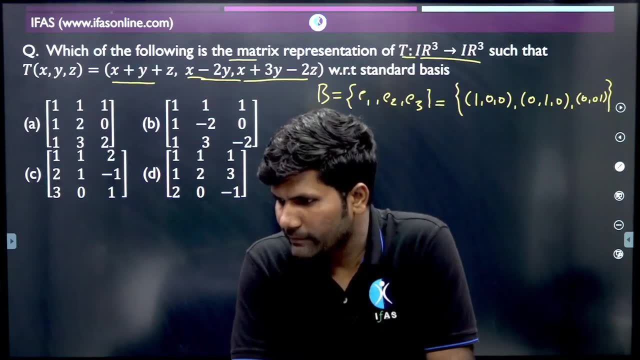 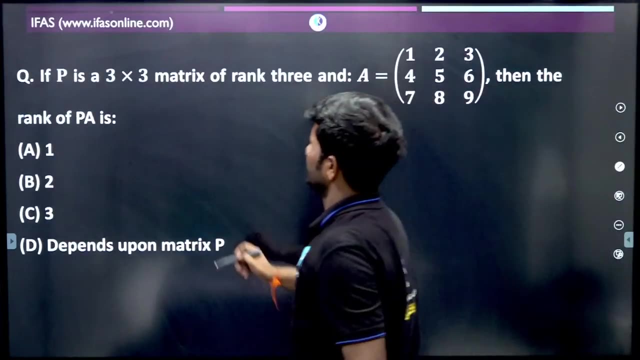 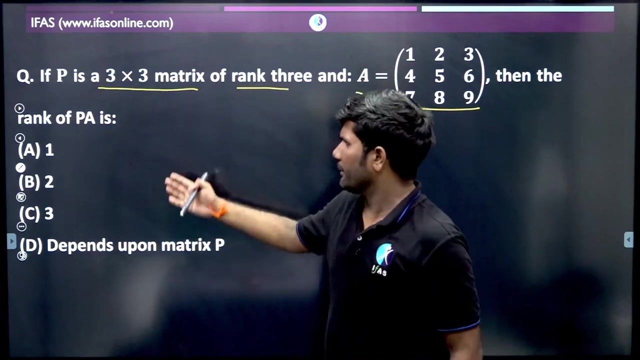 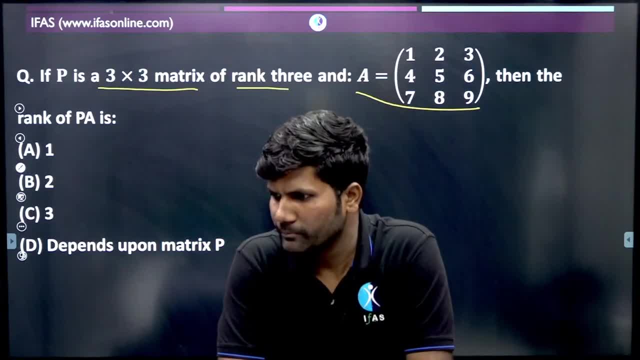 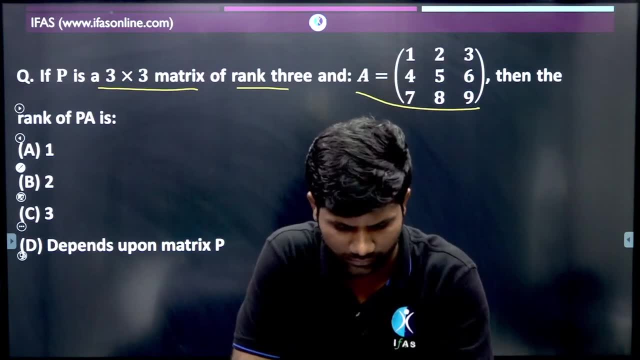 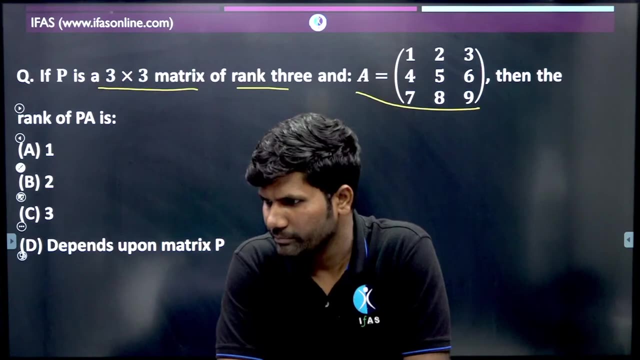 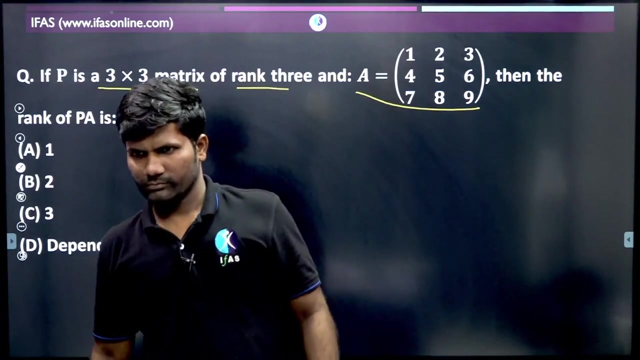 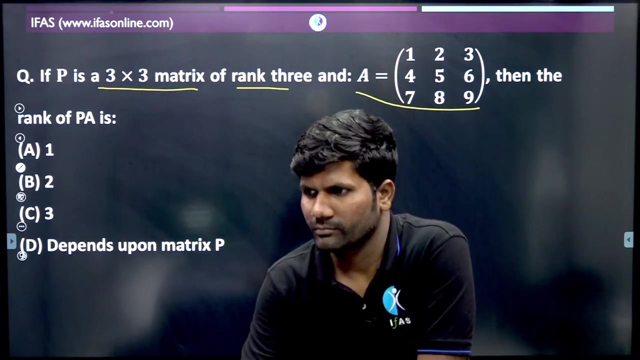 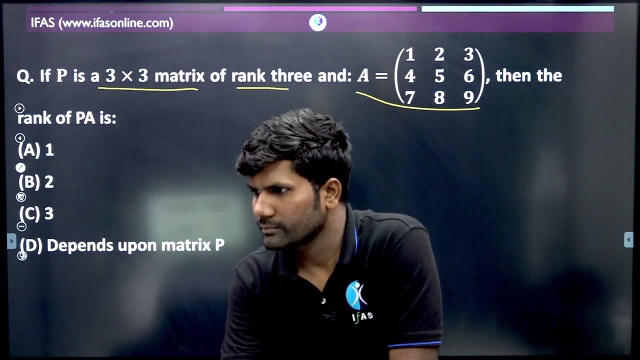 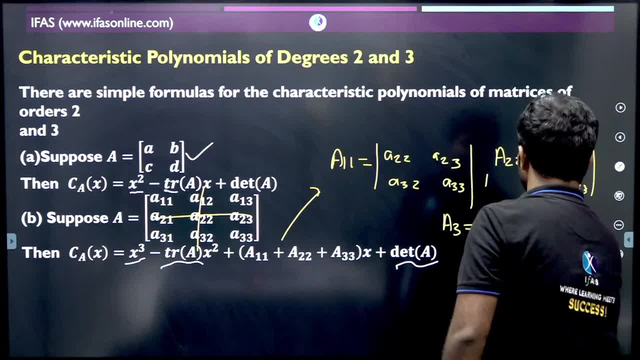 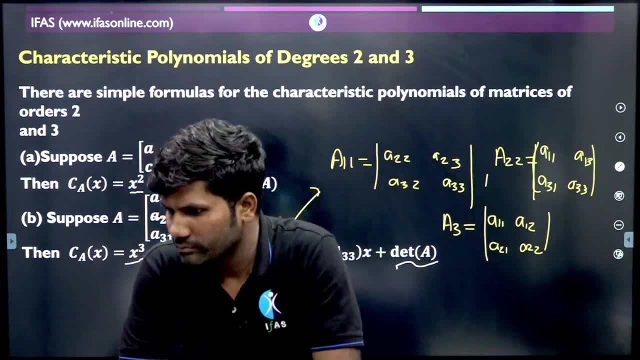 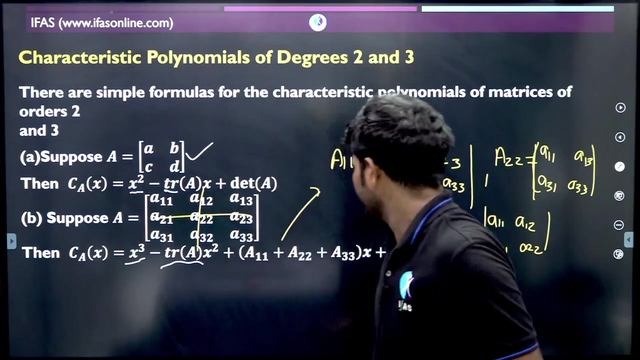 so what will happen here? A11,, A12,, A21, A22? so find the determinant of this, just substitute here you will get the answer. ok, is AB Karim buffering? is he buffering? what are you making of buffer? yes, here minus, plus here minus will come. 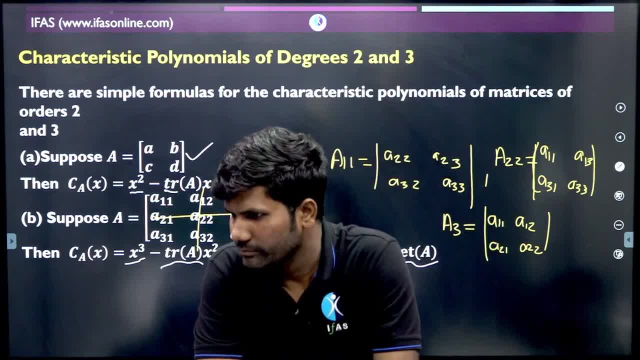 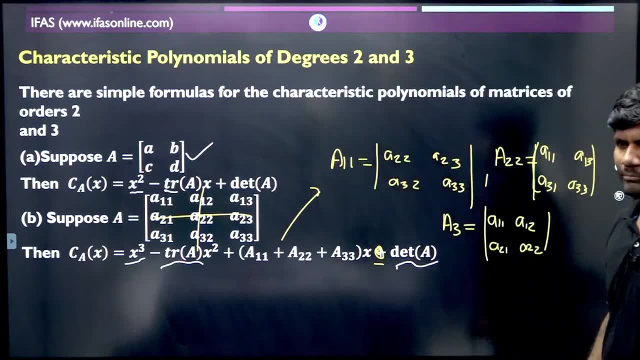 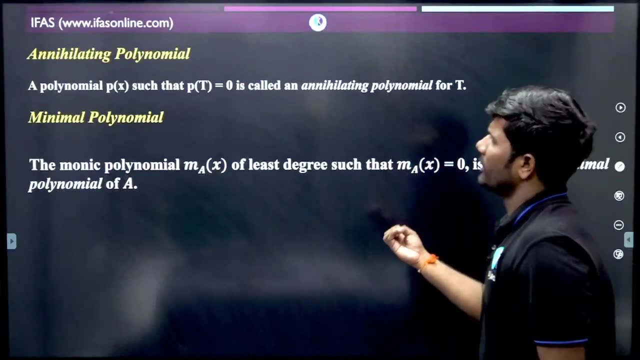 ok, it works with alternate sign. coefficient: ok, here minus will come. see here plus minus: plus minus will come. ok, it works with alternate sign. ok. what is annihilating polynomial? annihilating polynomial is any polynomial which is satisfied by matrix. it is called as annihilating. 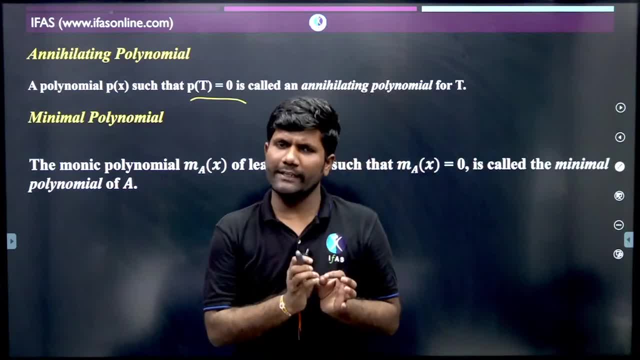 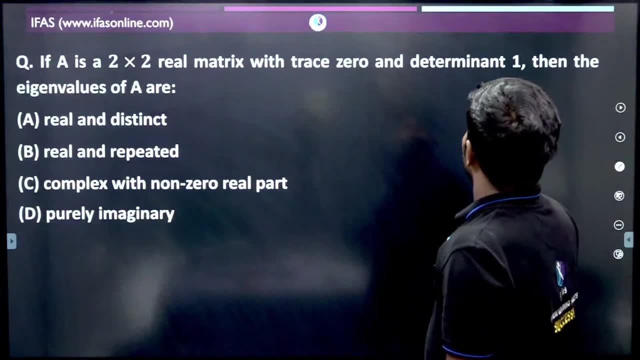 and what is minimal polynomial? the smallest degree of monic polynomial which is satisfied by matrix. it is called as minimal polynomial. ok, now let's come to the question here. what did we get late? AB is 2 cross 2 real matrix with trust 0 and determinant is 1. 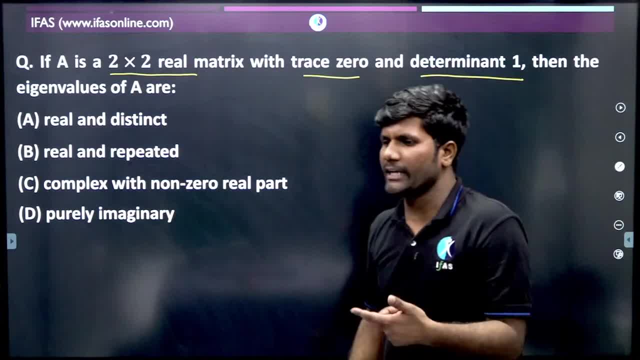 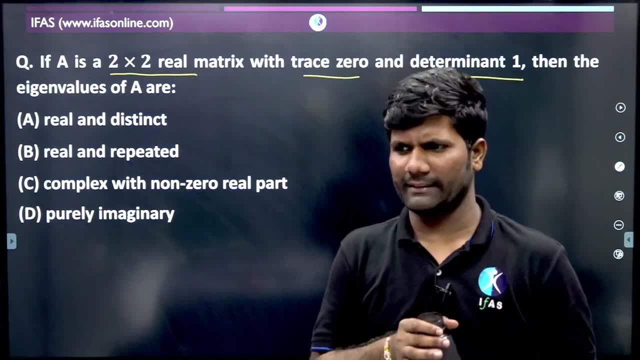 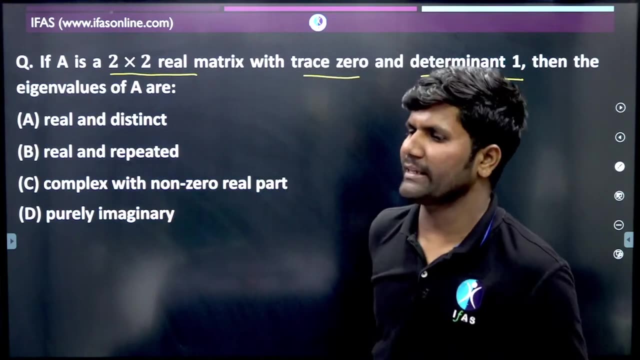 10 eigen values of A. now you have to tell what will be the eigen values of A. so quickly, solve it and tell. so this type of question comes in exam in state. so all students solve it and tell: what are you getting? Subadip, what happened? 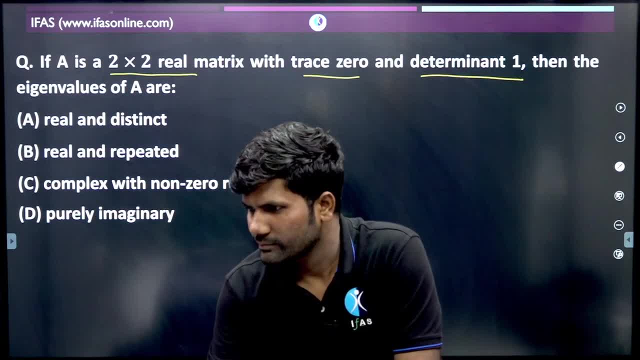 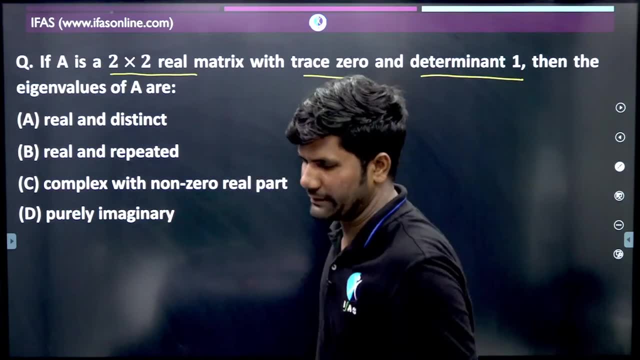 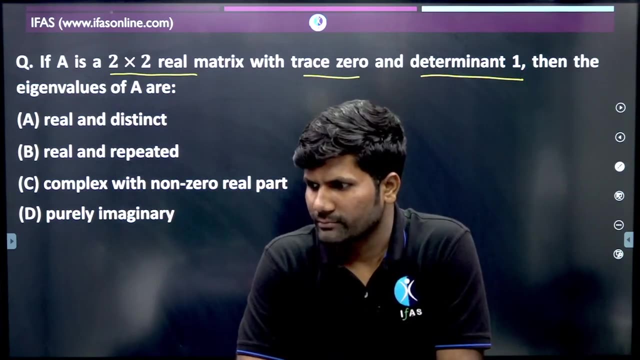 why did you delete it? ok, yes, yes, you have done a majoring. that was a typing mistake. ok, rest of the students. what are you getting? quickly solve it and tell. Nikita told it, Sultana told it, Tasneema told it, Arvind told it. 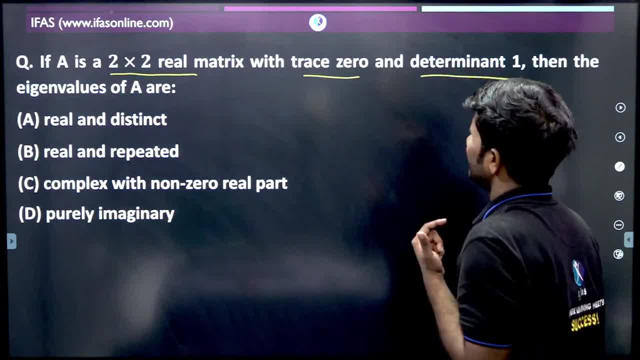 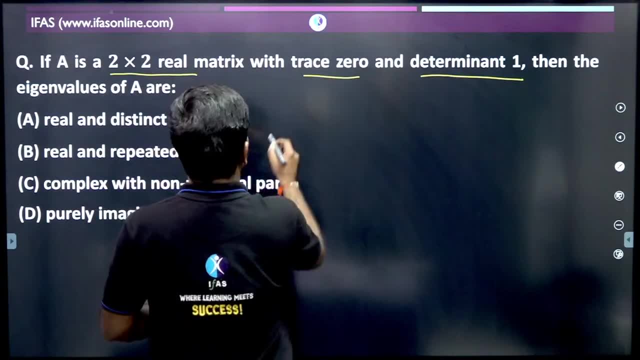 D is purely imaginary number. ok, let's see what is this? 2 cross 2 matrix with trust. now see, I had told you about 2 cross 2 matrix, shortcut what we used to do, what will be the characteristic polynomial CAX is equal to. 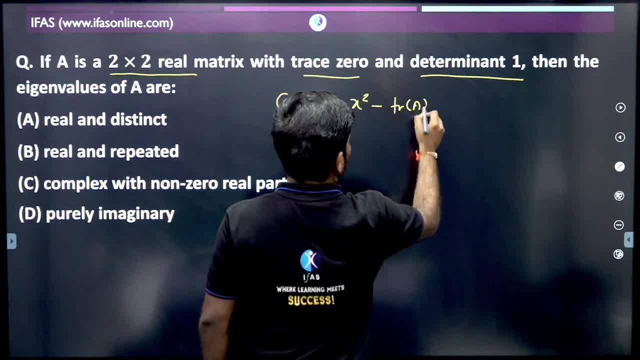 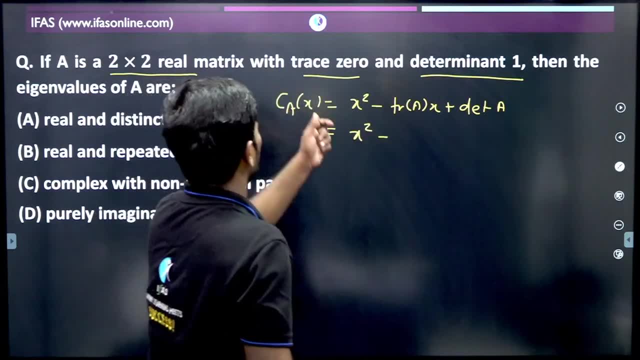 X square minus trust of A into X plus determinant of A. ok, this happens. now what will happen here? X square minus trust. how much trust did you give 0? so do 0 into X plus determinant of 1 will happen. so what will you get? 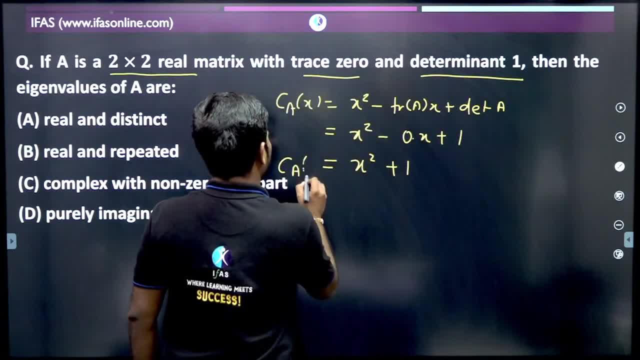 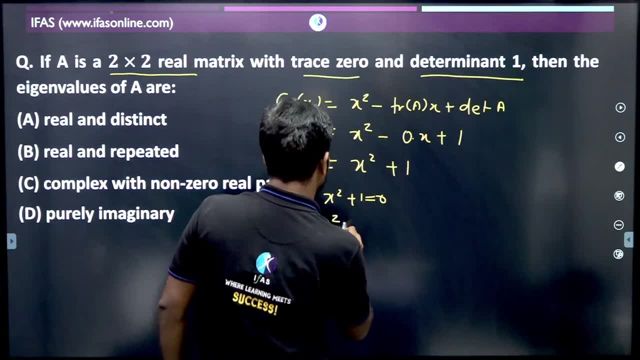 X square plus 1. now tell me once. characteristic roots are called eigenvalues. so if you find its roots, X square plus 1 is equal to 0. so what will you get? X square is equal to minus 1, so X is equal to square root of minus 1 plus minus. 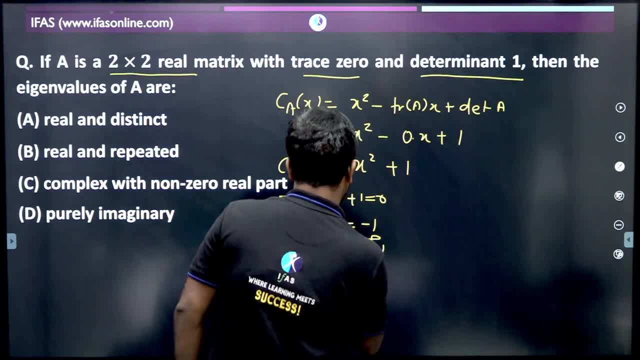 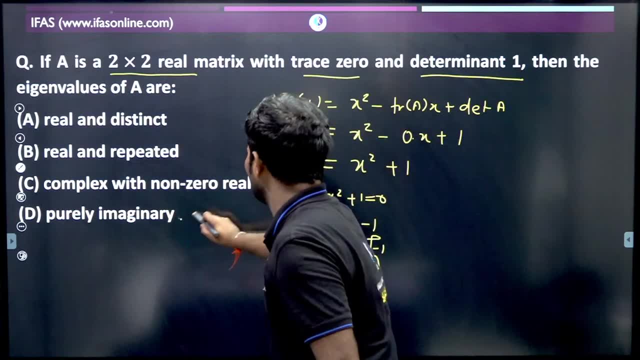 so what will be the value of X plus minus? I will be. it means its eigenvalues will be purely imaginary numbers. ok, so it means what will be option D? here it will be correct. so till here are you clear. all students are clear. 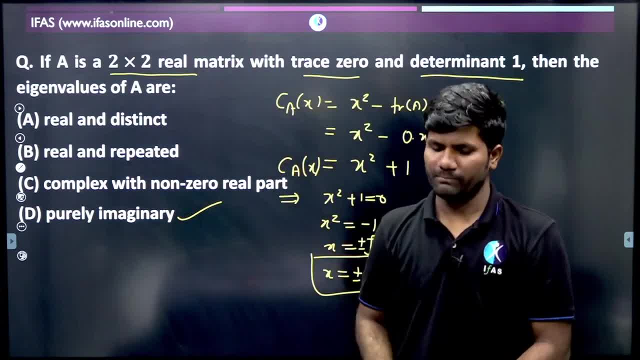 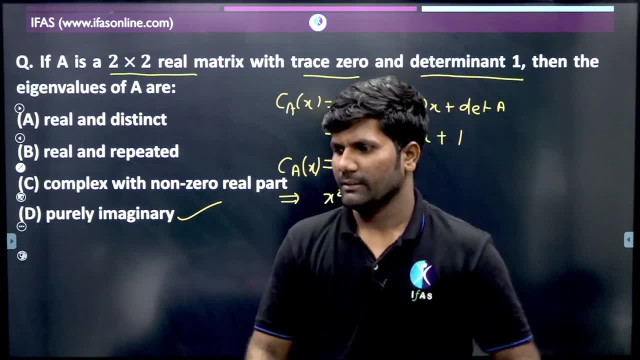 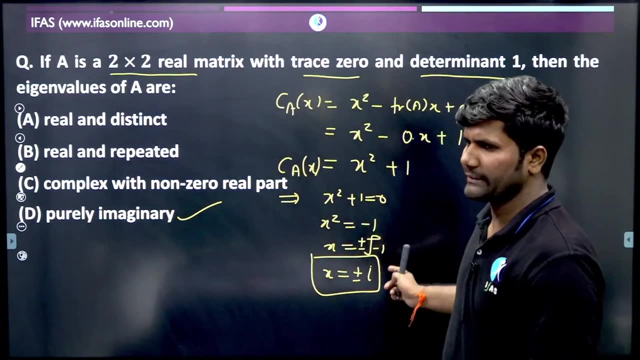 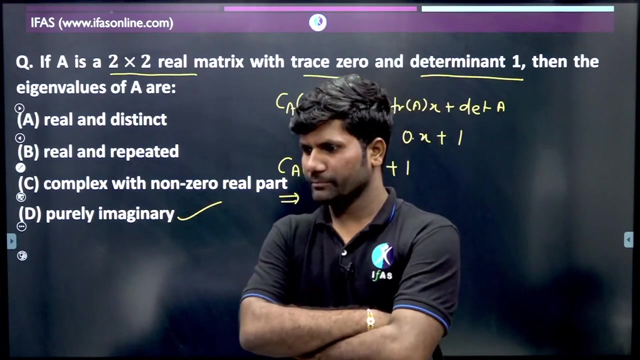 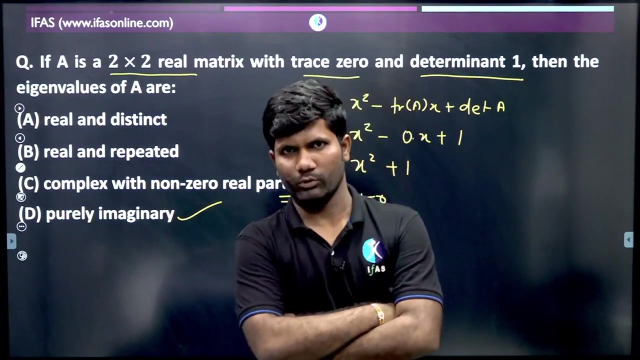 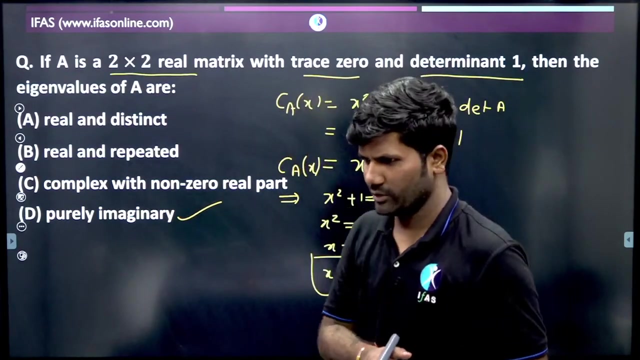 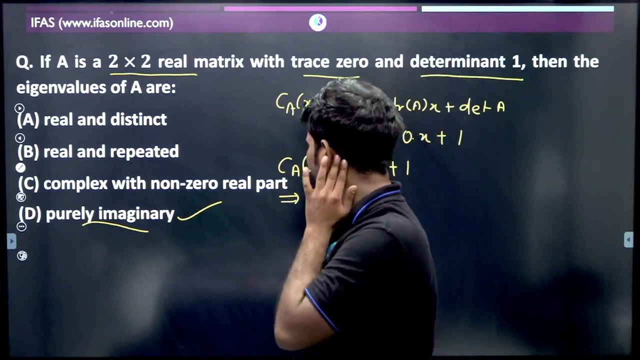 any doubts, otherwise we will move to next slide. tell me once: ok, are you clear? you can move to second question or we can move to next slide. answer: purely imaginary and imaginary is basically same. purely imaginary means that there aren't the real parts. complex with non-zero real parts. 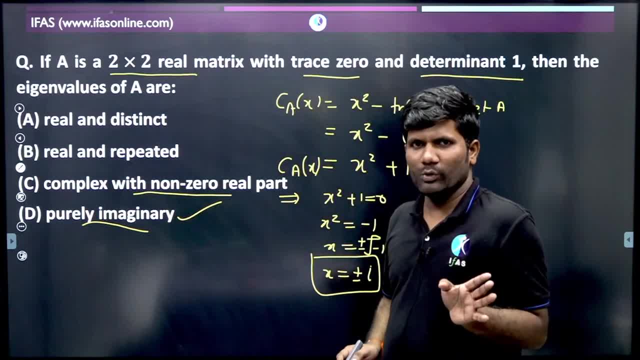 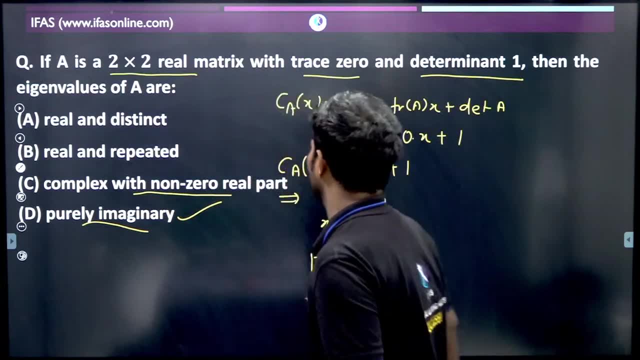 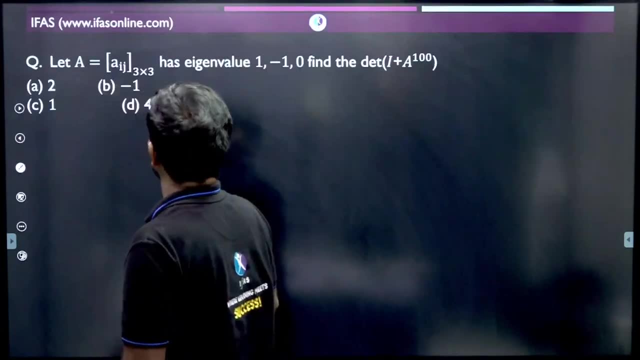 so Chicapuri budget is coming and real parts are also coming, not visible, only imaginary part is there here. the correct answer will be d. now let's come to the next slide. now here we have given: a is 3 cross 3 matrix whose eigenvalues are given. 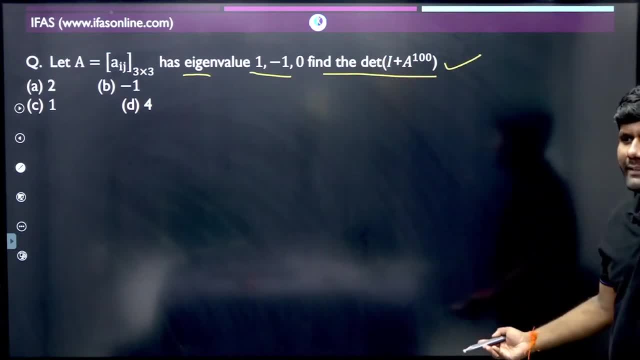 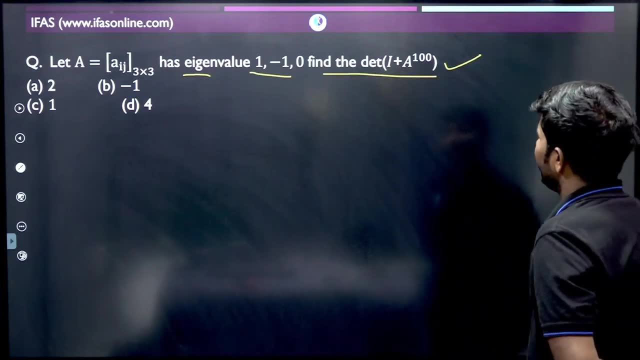 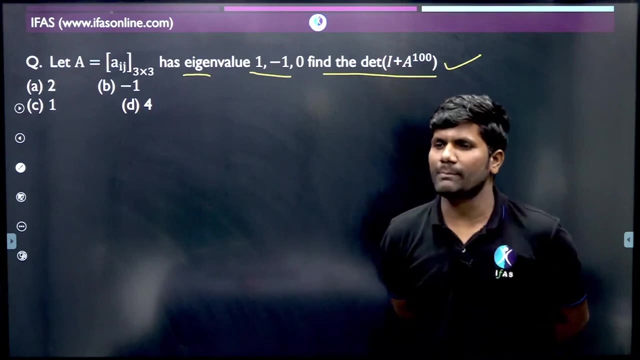 we have to find its determinant. now tell me what will be its determinant. what will be its determinant? what is the hint for you? sum of eigenvalue is same as the determinant. no product of eigenvalue. sum of eigenvalue is same as the trust. okay, now you guys solve and tell me what answer you are getting. 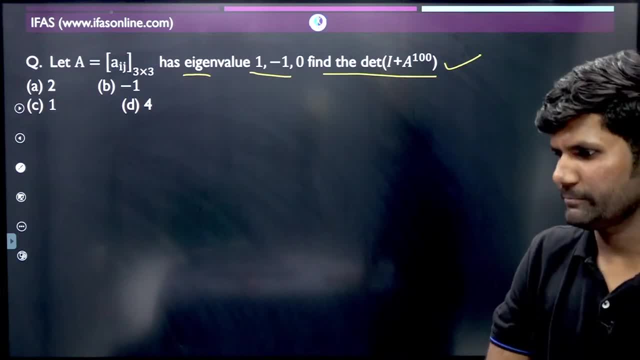 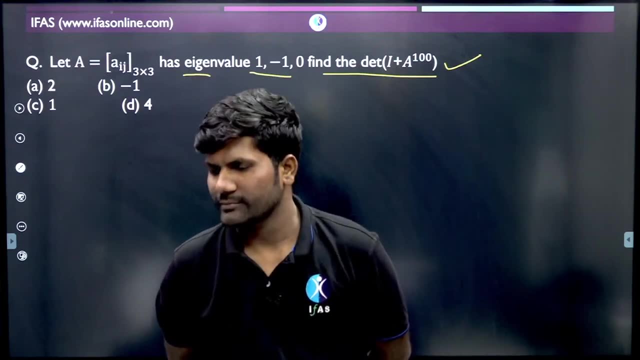 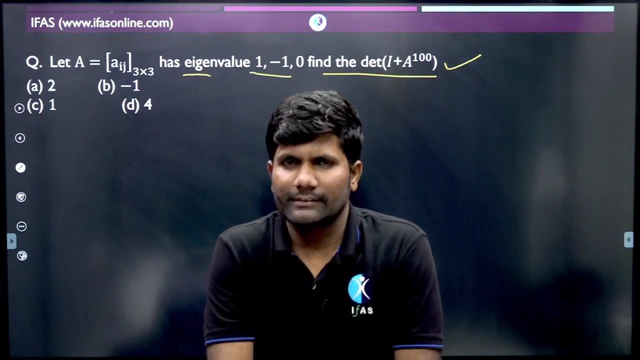 all students solve and tell me what you have got. so if you have not liked it yet, then first of all like it. subscribe to our channel and keep the notification bell on so that you can get notification of new videos of the state and hall ticket. hall ticket is here. 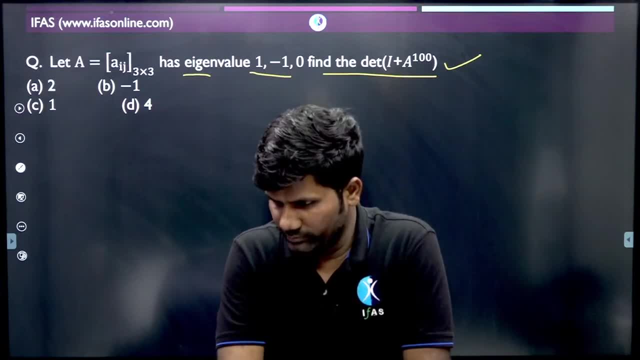 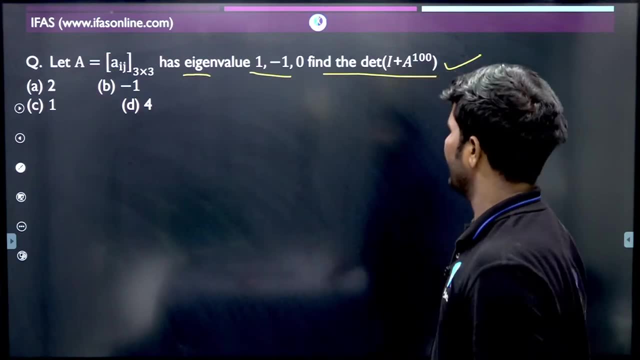 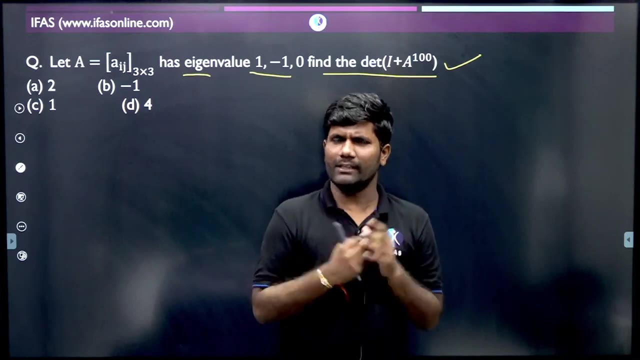 okay, let's go. Dilip Waghmode, Nikita has given the answer. where is bb? tell me one thing: we have done a result. what does a result say? suppose lambda is an eigenvalue for some matrix a, then p of lambda is the eigenvalue of the matrix p of a. 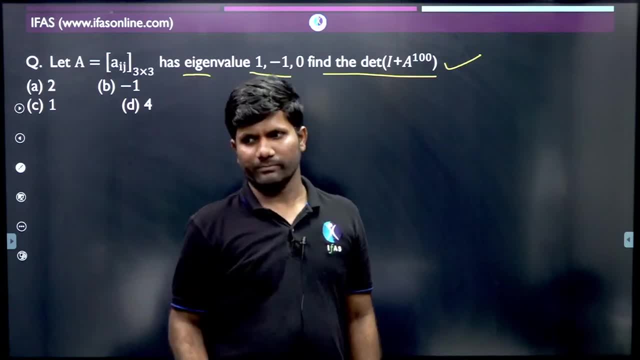 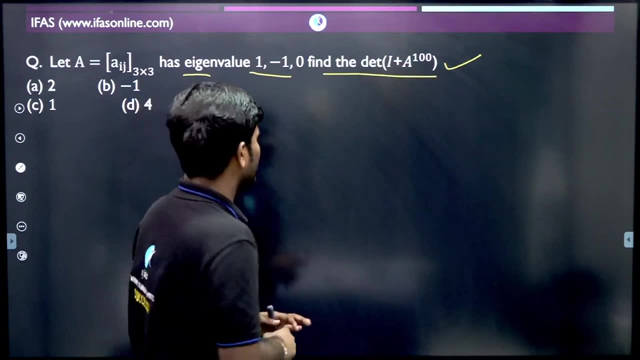 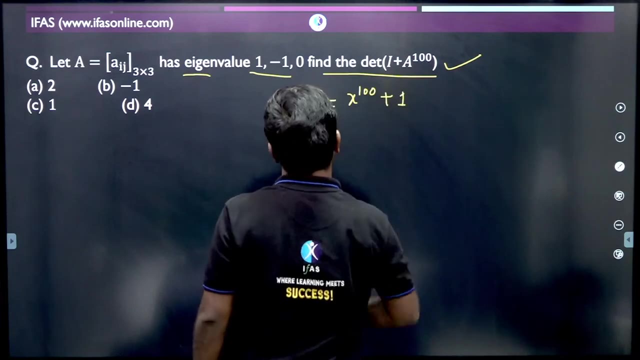 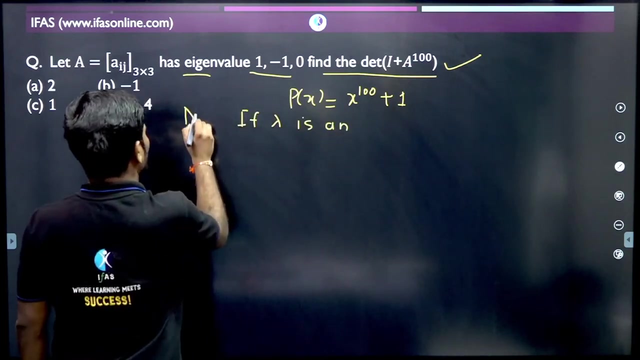 okay, so we have to use it here. see, everyone is giving d answer maximum. okay, so what i do here? i make p of x polynomial. what will be x? raise to 100 plus 1. now, if lambda? if lambda is an eigenvalue, write a note here. 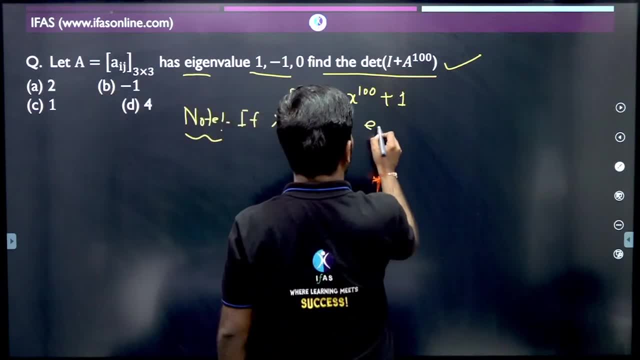 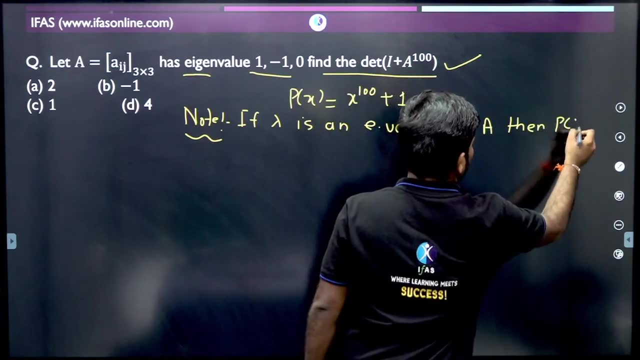 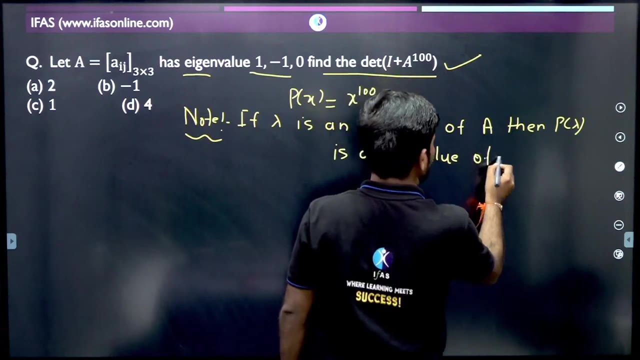 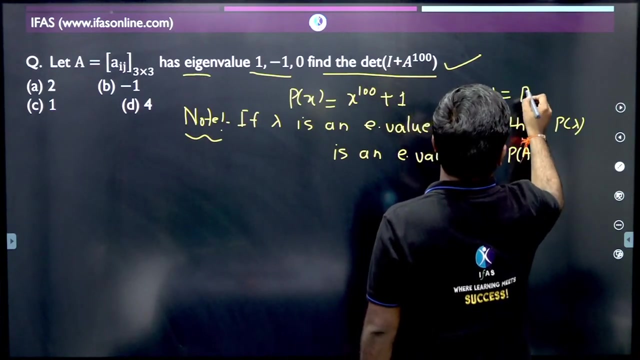 which result i am using. you should also know that if lambda is an eigenvalue of the matrix a, then p of lambda is an eigenvalue of p of a. so here you can write: p of a will be x raise to 100 plus identity, which means: 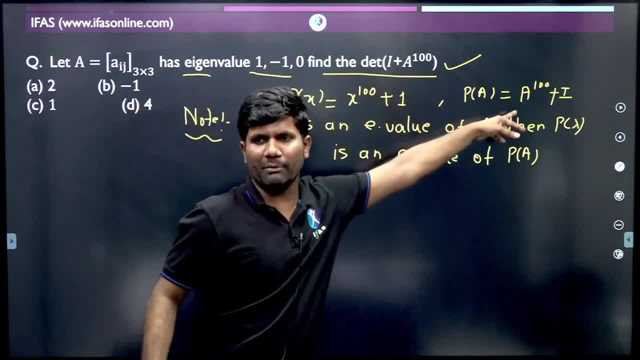 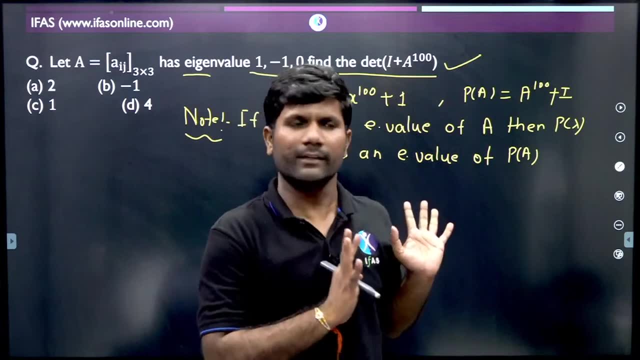 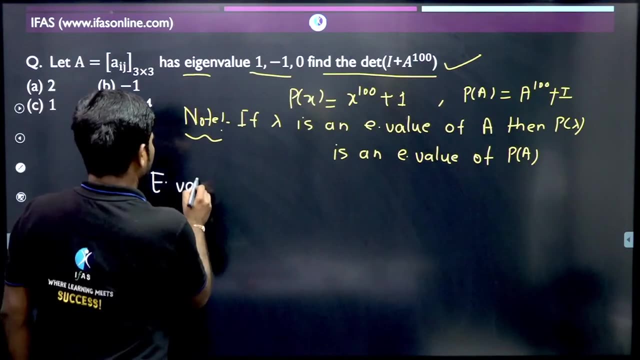 if you find its determinant, then you will get a. you have to find this p of a. if i know eigenvalues of p of a, then my work will be done, because product of eigenvalues is same as determinant. okay, now let's come here. tell me one thing. 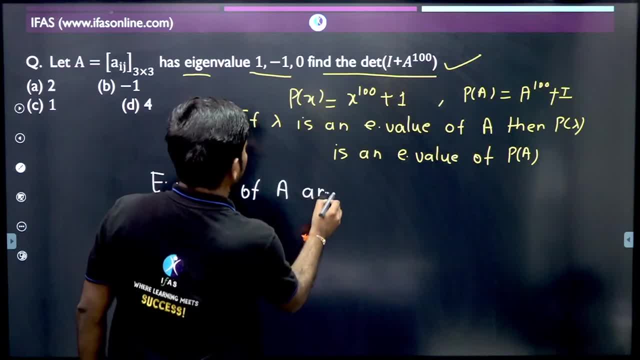 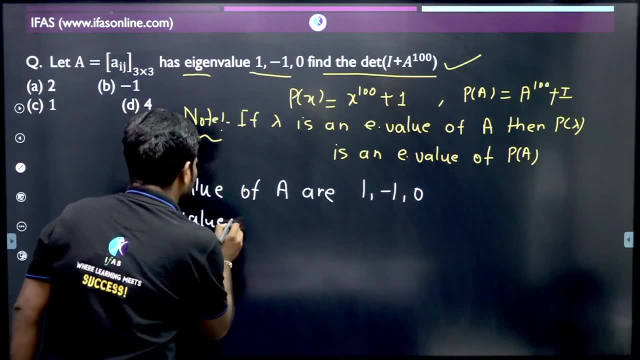 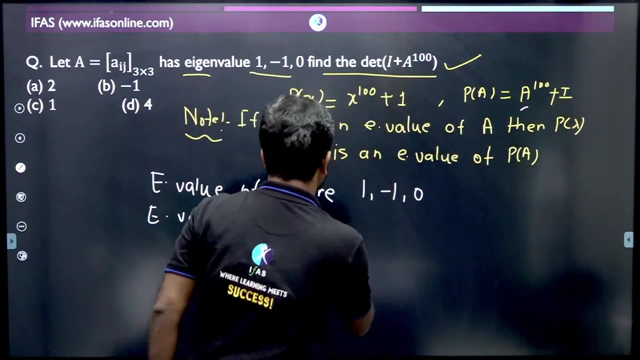 eigenvalues, eigenvalues of a. where are the eigenvalues of a? one minus one and zero? what are the eigenvalues of p of a? p of a eigenvalue means for this matrix eigenvalue. what will we get here? it will be 1 raise to 100. 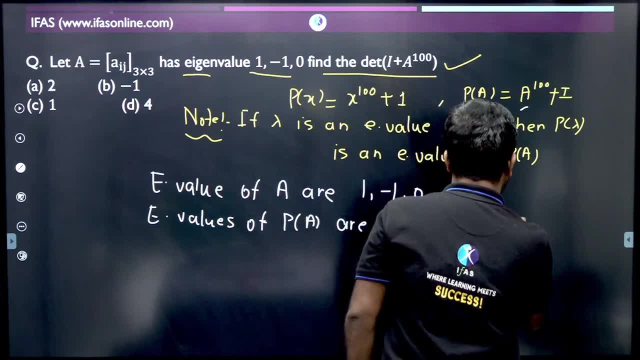 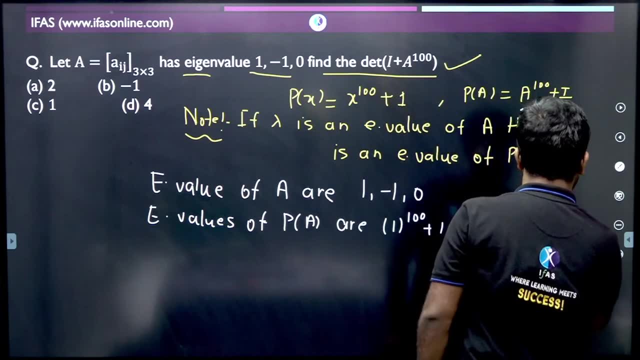 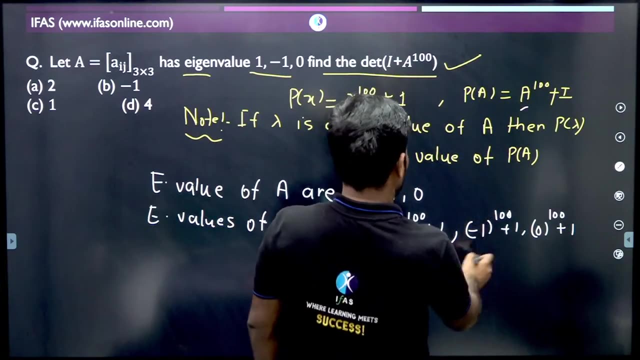 plus 1 minus 1 raise to 100 plus 1 and 0 raise to 100 plus 1. so if you do, what will you get? 1, 1, 2, and here 1 1, 2 and a will be 1. 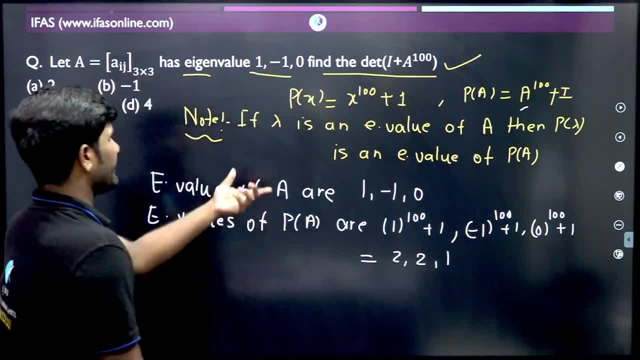 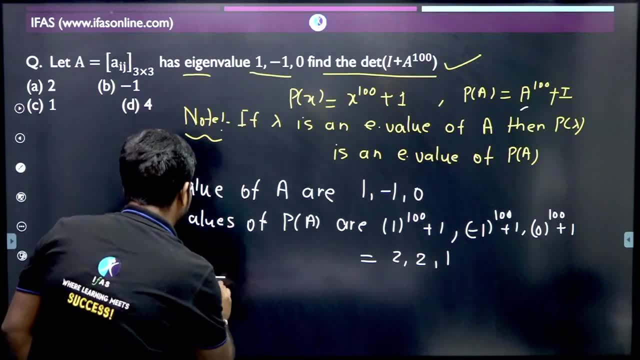 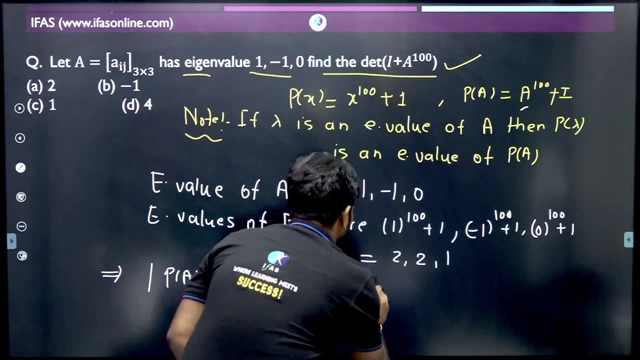 this will be okay. now what we had to find, its determinant. so what is determinant? so determinant of p of a determinant is same as determinant of i plus a raise to 100. the determinant will be product of eigenvalues, that is, 2 into 2 into. 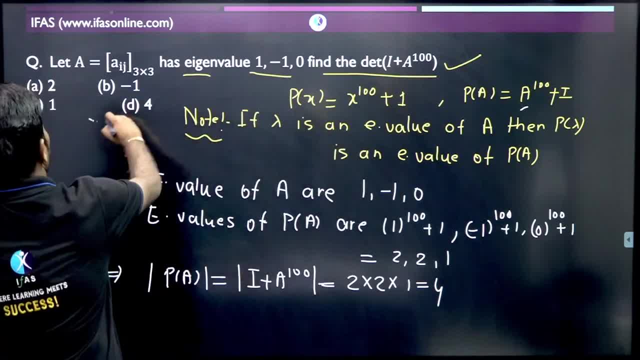 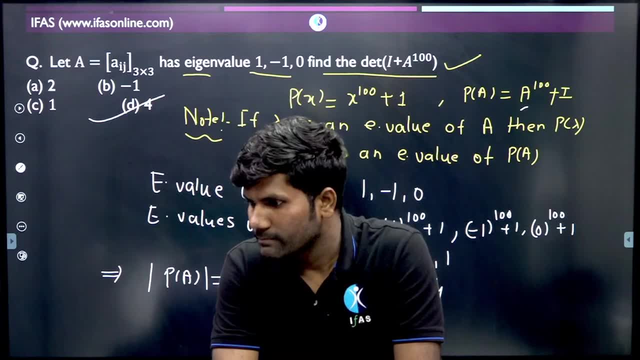 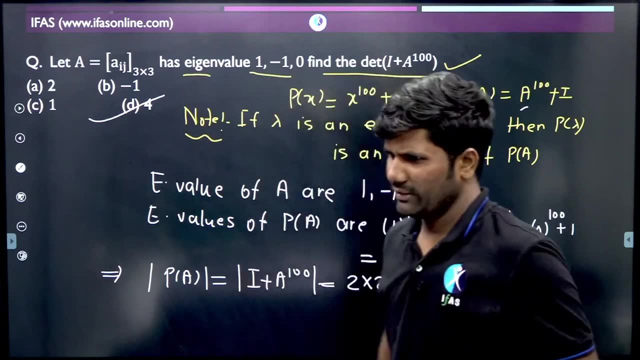 1, which is equal to 4. it means that correct answer for this question is option b. is it clear to all? delhi says: product of eigenvalues, 0 will come and 0 plus 1 is one determinant. from where are you doing this? see here you will get. 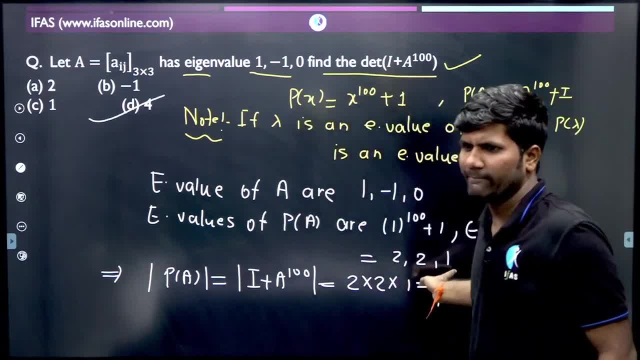 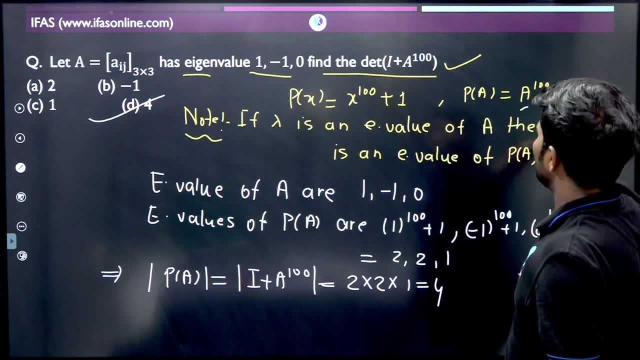 delhi. see, did you understand where you made a mistake? see here: whose eigenvalues will you get? what you have to do: if lambda eigenvalue is of a, then p of lambda, whose eigenvalue is p of a. so what you have to do is find p of 1 here. 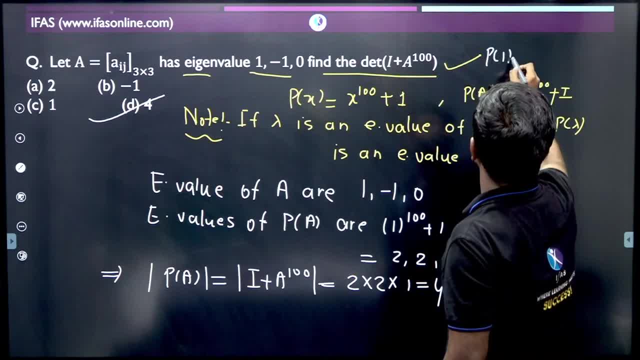 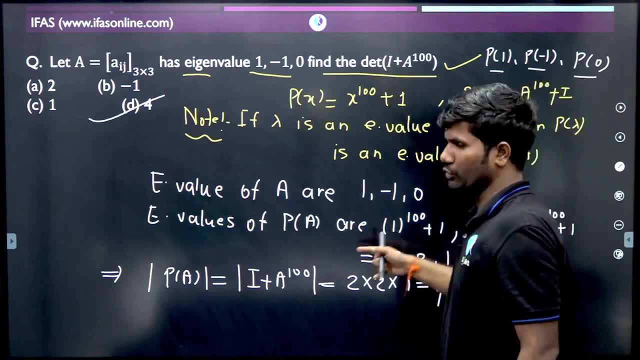 what will be its eigenvalues? what is its eigenvalue? 1? so what will be its eigenvalues? p of 1, p of minus 1 and p of 0. so find all of these: p of 1, p of minus 1, p of 0. 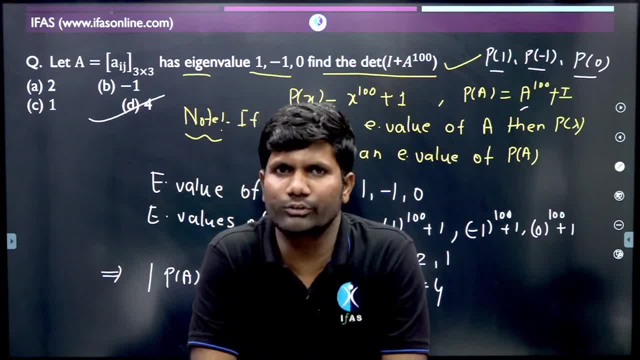 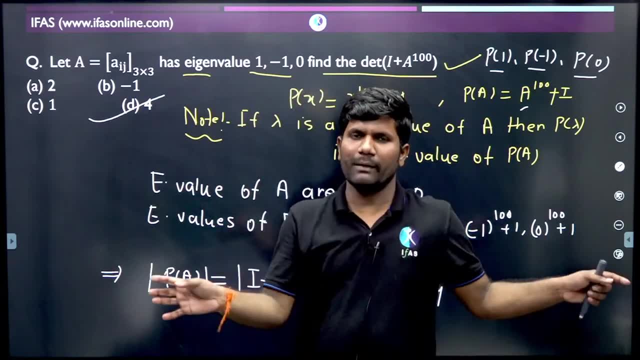 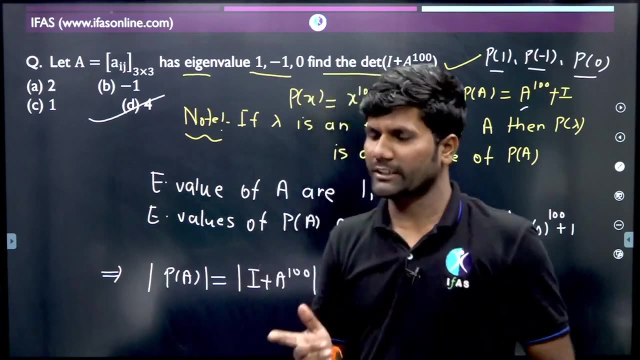 its eigenvalues will be. okay, delhi, did you understand all students clear? you see, determinant of a- b: when multiplication is there, then you can do. if multiplication is not there, then it is not equal to determinant of a plus determinant of b. okay, you can do in product. 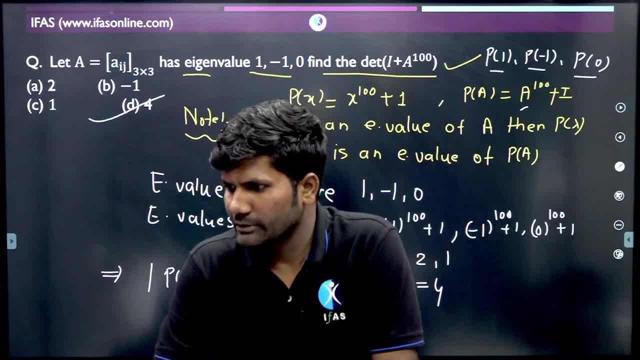 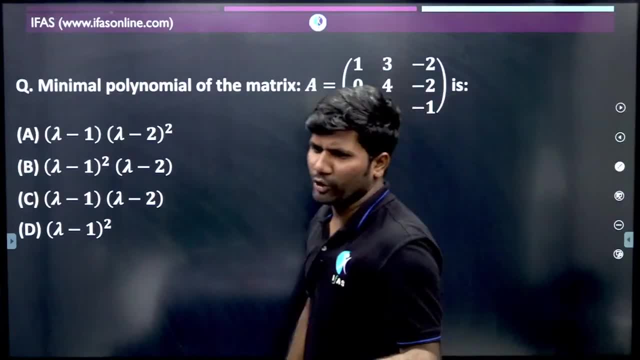 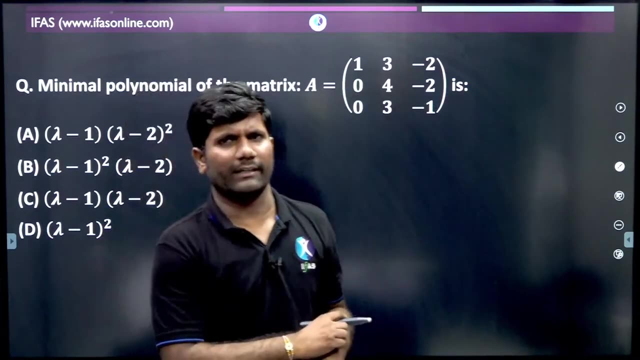 is it clear? let's go to next slide now. tell me its minimal polynomial simple question. i think it is asked in some exam. you tell me what will be minimal polynomial. you have to do this first of all: find out its characteristic polynomial. tell me what will be its characteristic polynomial. 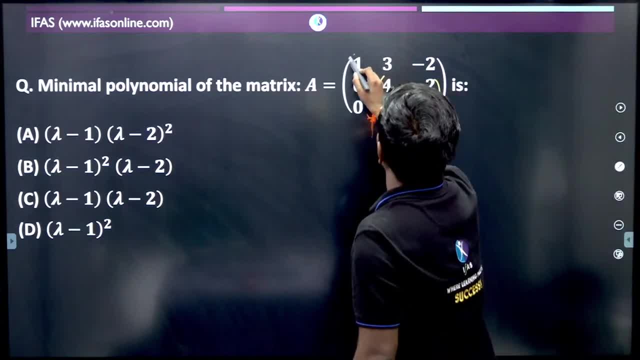 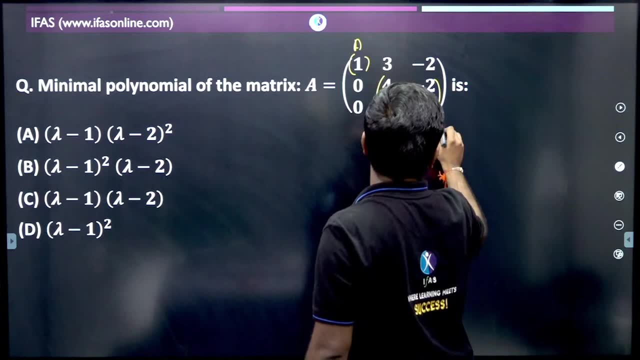 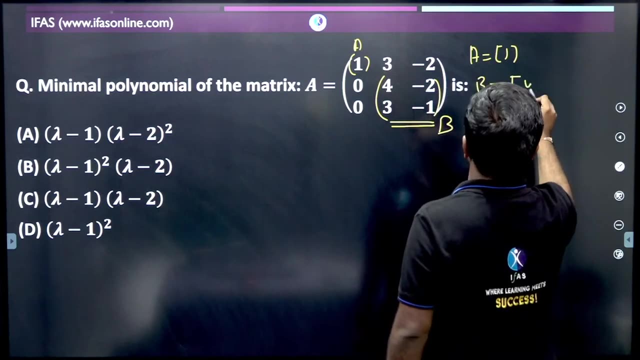 you can divide it like this: find it and find its characteristic polynomial. what will be its characteristic polynomial? suppose this is matrix a and this is matrix b: a is 1 cross 1 matrix and b is 2 cross 2 matrix. now find its characteristic polynomial separately. 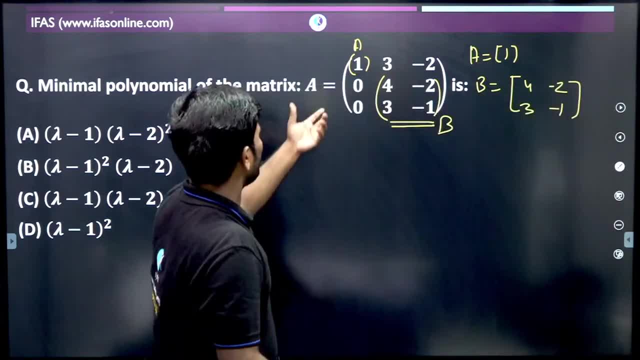 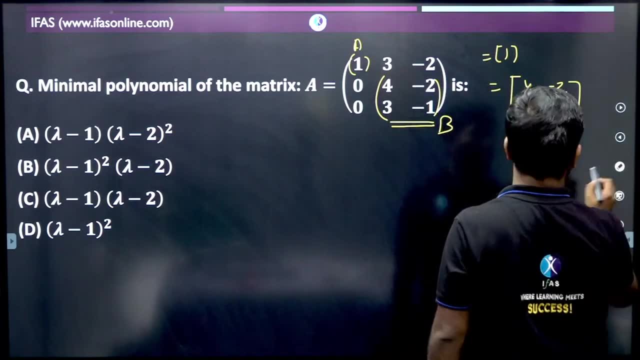 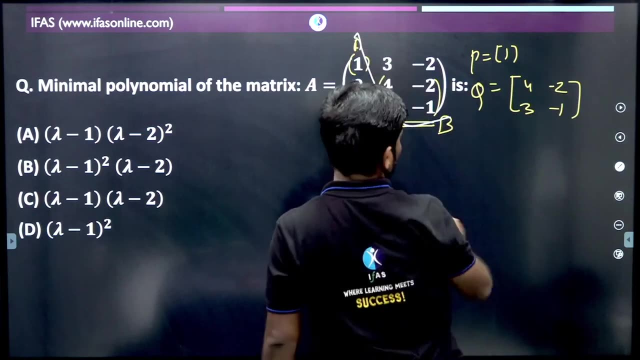 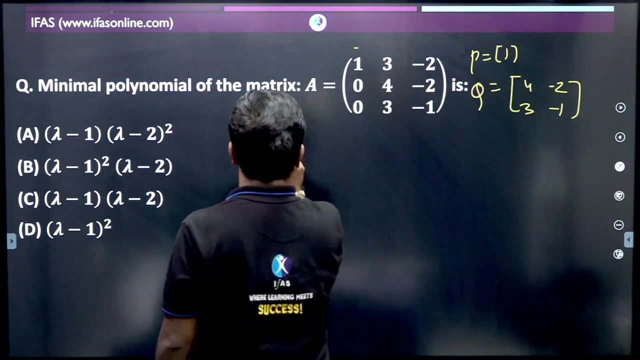 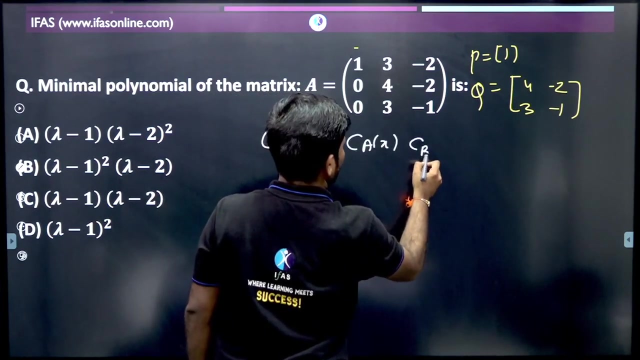 what will be characteristic polynomial of a? here, a is already. let's take p and q, because a is already there, p is already there and this is q, so so. so. so now let's see characteristic polynomial of a. what will be characteristic polynomial of a into characteristic polynomial of? 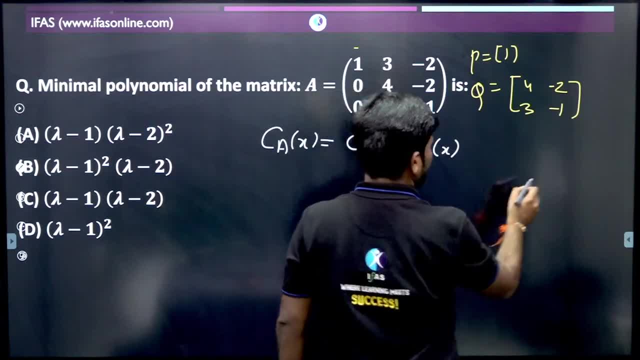 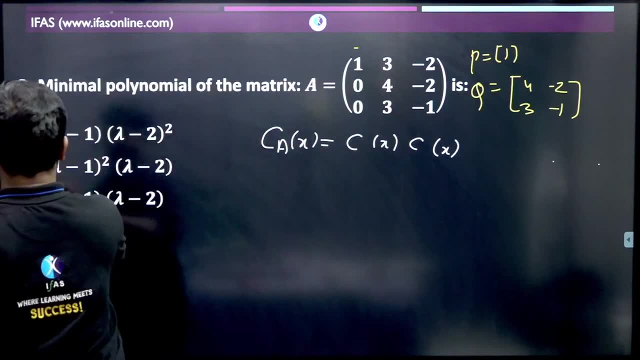 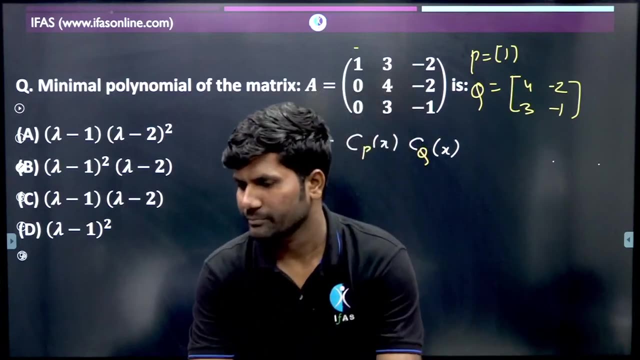 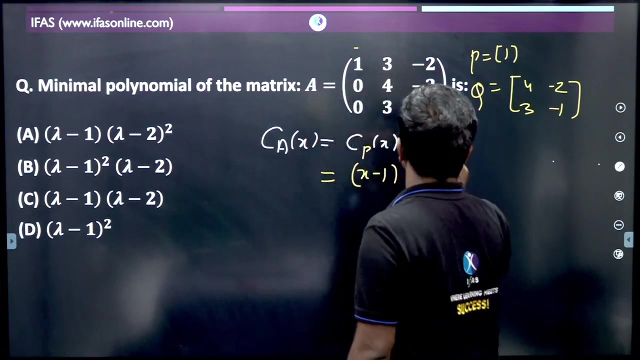 p into characteristic polynomial of q, so you tell me what will be its characteristic polynomial. it is here. Now tell me what will be the characteristic polynomial. If you find the characteristic polynomial, then you will get x minus 1, and if you find it here, then what will you get? 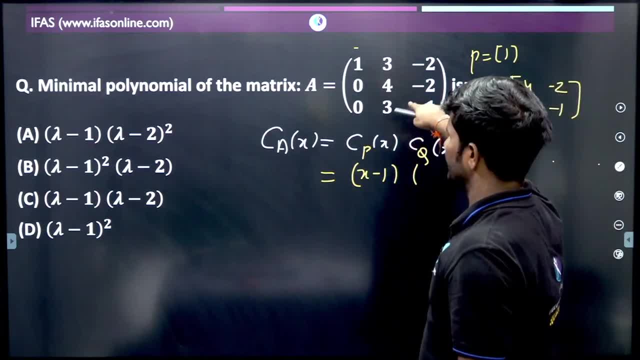 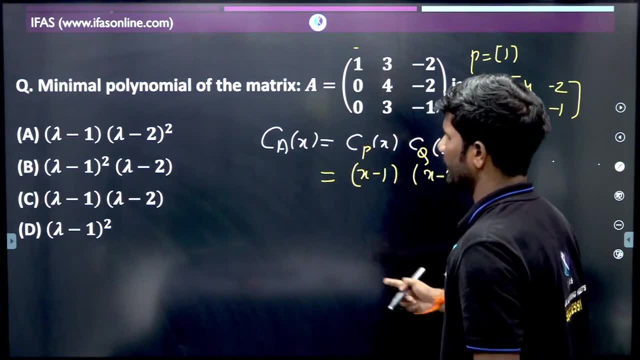 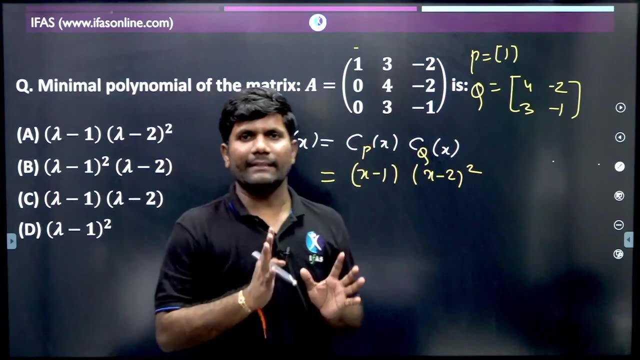 How much is the sum of each row? It is 2.. So somewhere here you will get x minus 2 square. This will be the characteristic polynomial. Now tell me one thing. One result says that the irreducible factor in the minimal polynomial and the characteristic polynomial is the same. 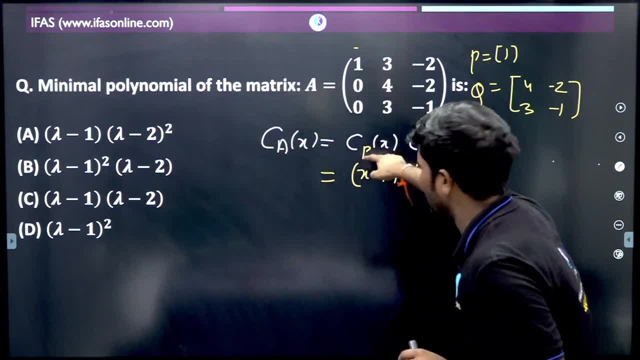 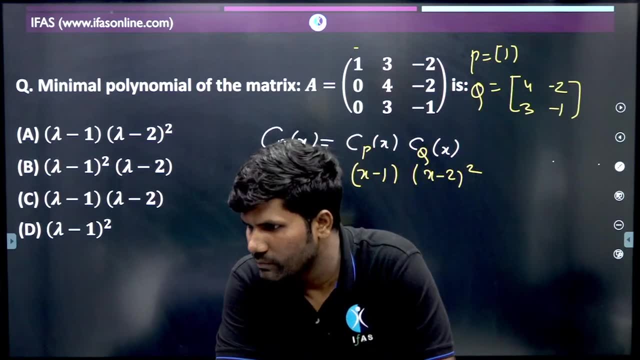 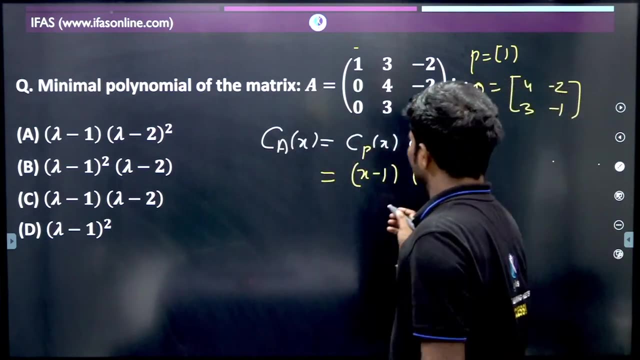 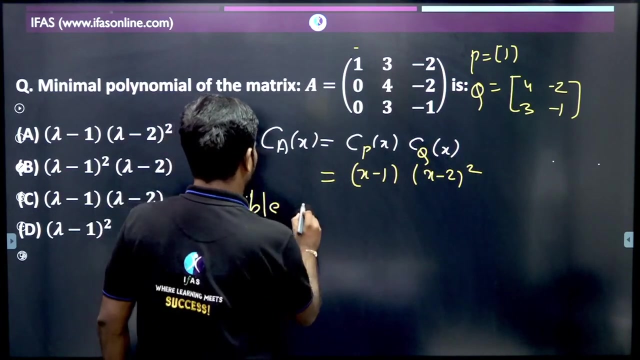 Irreducible factor means that the roots in the characteristic polynomial are the same roots in the minimal polynomial. Now let's move ahead. If I talk about the possible minimal polynomial here, then I am talking about possible. Now we have to select possible. So what will be the possible minimal polynomial? 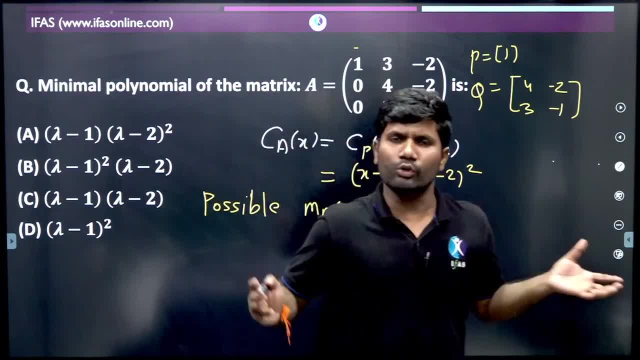 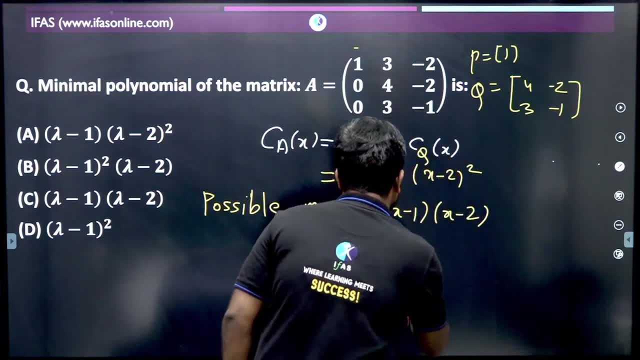 Look, there should be 1, 2 and root. It is fixed. So the possible minimal polynomial is x minus 1 and x minus 2 square. Either it can be a or it can be x minus 1 and x minus 2 square. 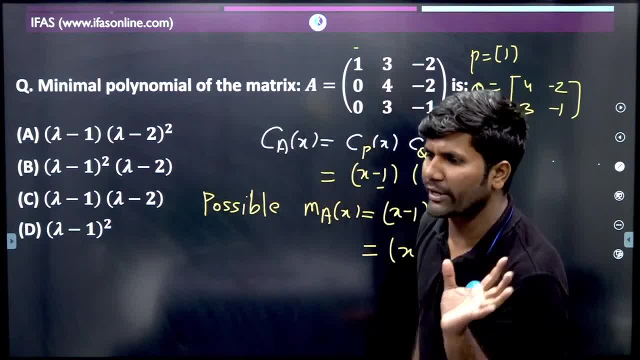 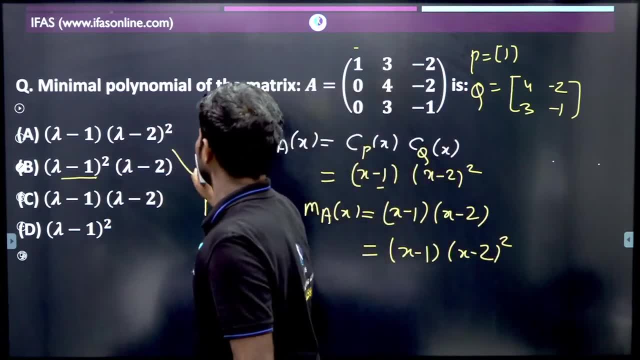 There will be a minimal polynomial between these two. Apart from this, no one can be So. look here: its degree is more than this. A is over here. A is over here. There is no root of 2 here. This means that there will be one of this and one of this. 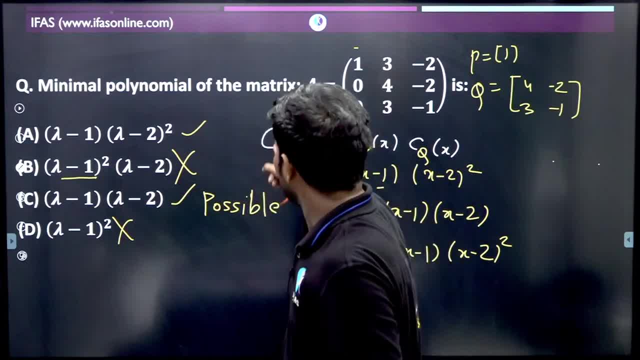 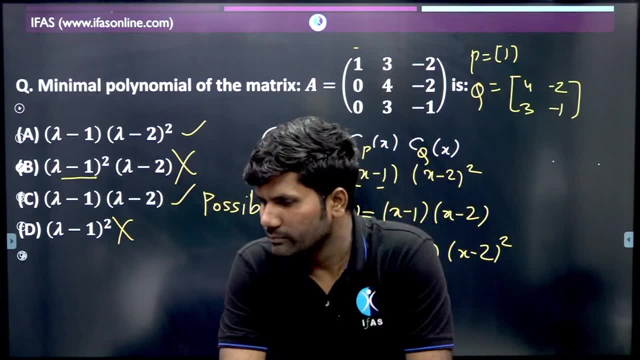 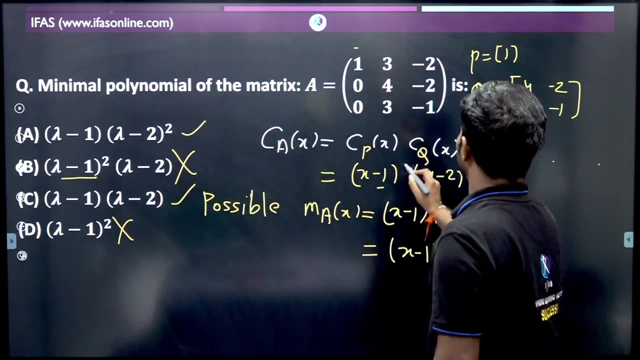 Now, Taslima, you also said so many times that there is a minimal polynomial here. B cannot be. Look Now you tell me, Is the characteristic polynomial upside down? Have you got the characteristic polynomial A? Fine, So find the characteristic polynomial once. 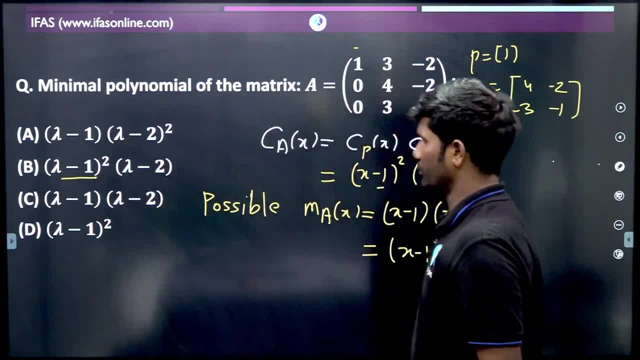 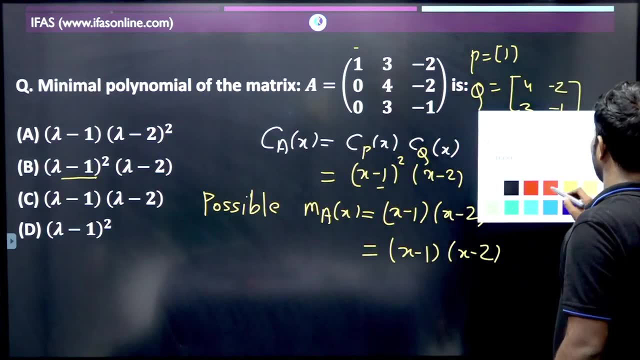 If you get the characteristic polynomial A, stop, Taslima, stop, stop, stop. If you get the characteristic polynomial A, then what will be the possible minimal polynomial here? The minimal polynomial can be like this: Here power 2 will be. 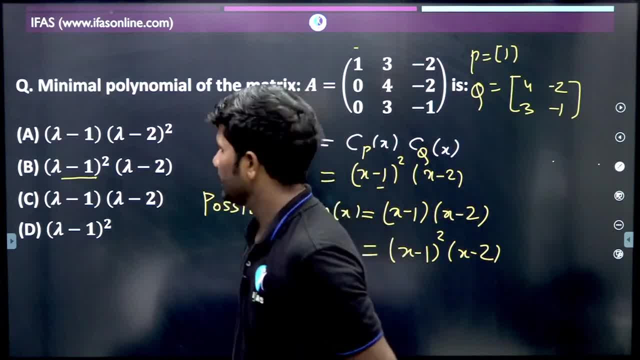 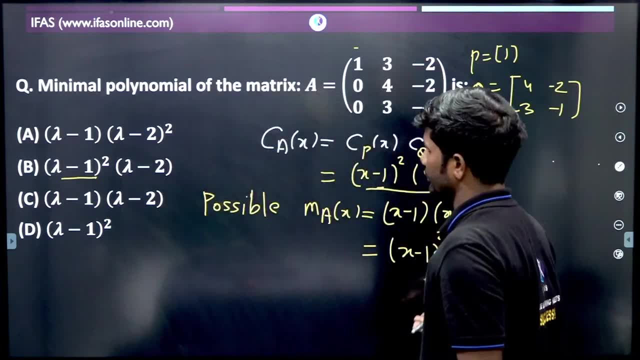 Fine, Yes, yes, absolutely, Vaishnavi, Got it. got it. Characteristic polynomial A will be found. Fine, Now look here. So it has a minimal polynomial. It can be either one of these two, So the first one is over. 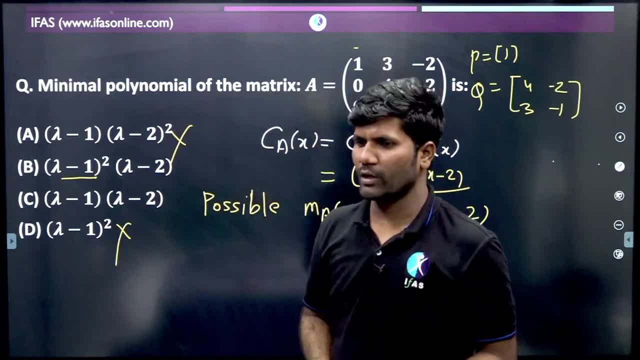 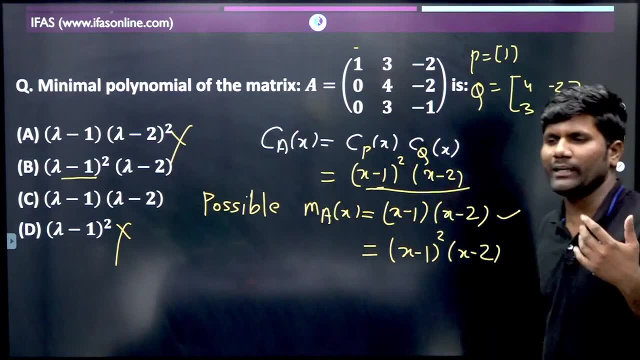 And the last one is over. There will be one of B and C Now in B and C first you check it. If A is zero, that means A minus identity into A minus two times identity. If A is zero, then this will happen. 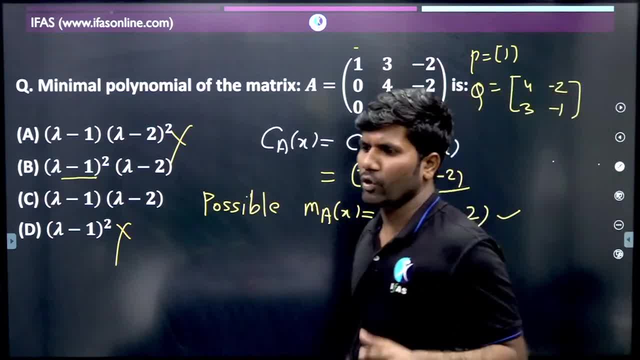 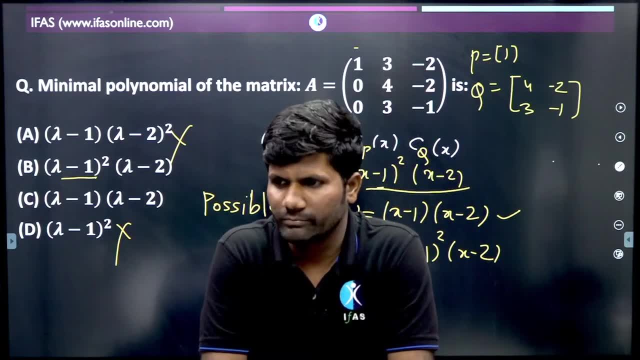 If A is not, then this will happen. One of the two will be one: Check it, you will get it. So now you have to check here. Check it and tell me what will happen. Fine, So check it quickly and tell me what you will get. 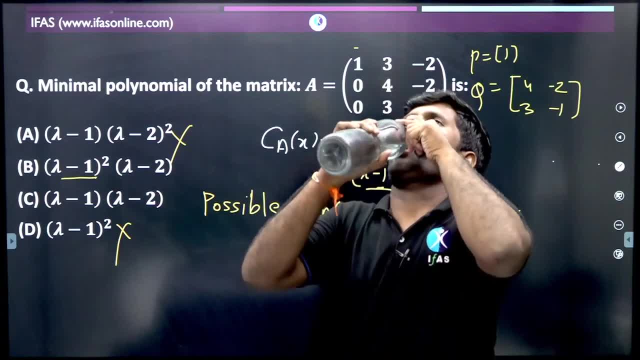 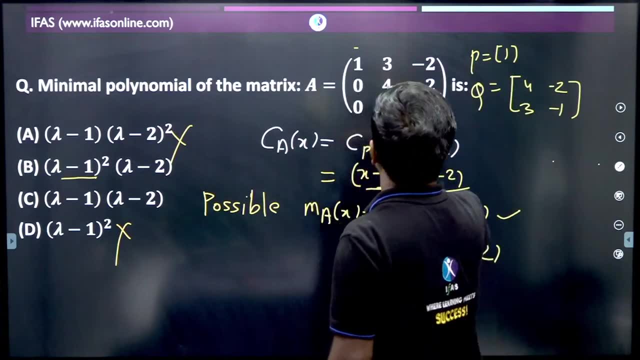 Yes, Arvind, let's tell the characteristic again. Come on, Arvind, let's tell the characteristic polynomial. Arvind, look to find the characteristic polynomial. if you see that I have made two blocks square, then it is zero. 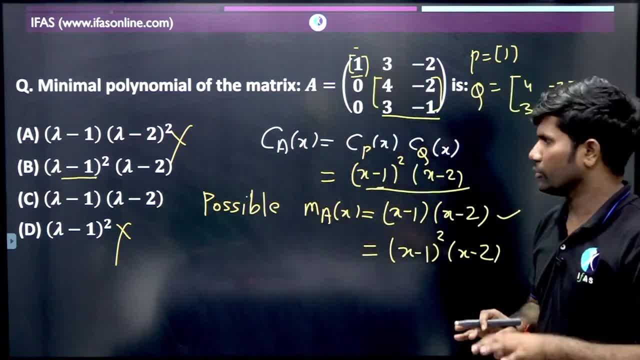 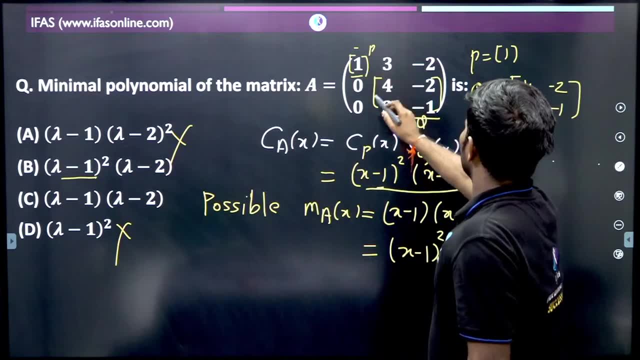 So I will find its characteristic and multiply it. So I did the same: I called it P and called it Q, The characteristic of P and Q. You will get P's x minus one. If you find Q, you will find its characteristic polynomial. 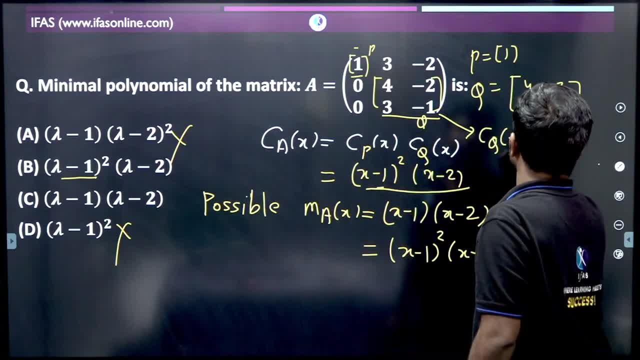 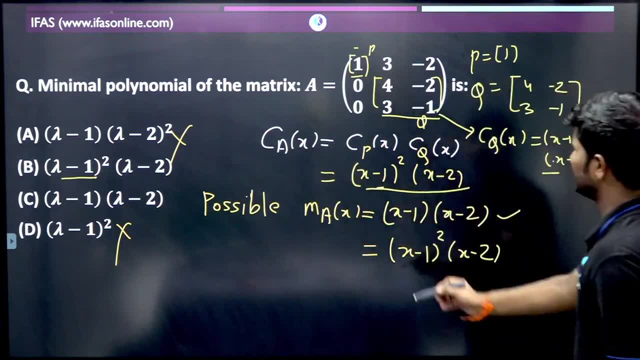 which you have just told me, And I believe what I got. I think I got x minus one and x minus two. So now, if you multiply all these people, you will get their characteristic polynomial like this: Fine, Who asked? Who asked? 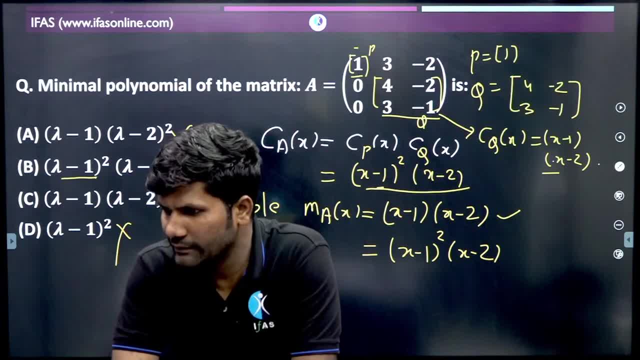 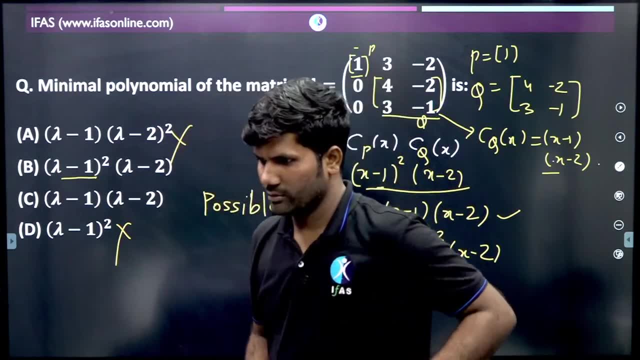 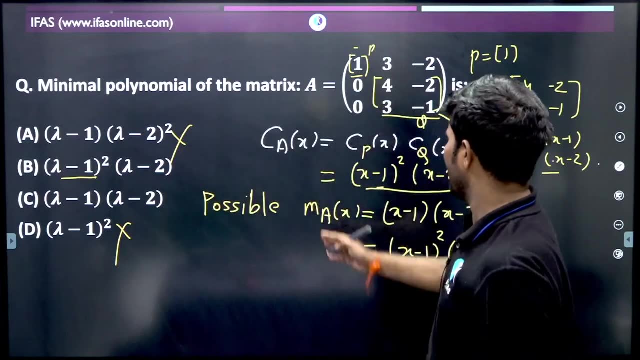 Yes, Pooja Pooja, I did it. Fine, Arvind Arvind Bhaare, Fine, Yes, absolutely, absolutely, absolutely. Yes, Bharti, you can do it in that too. Now, here you have to decide what will happen. 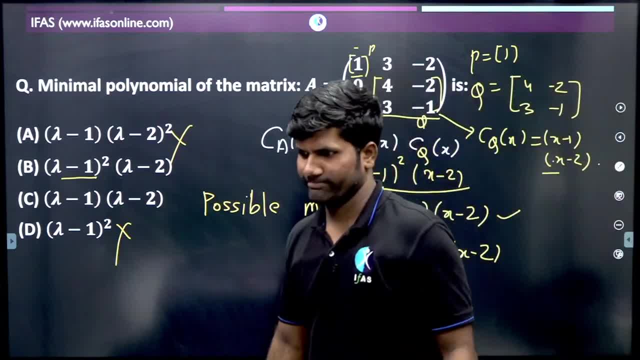 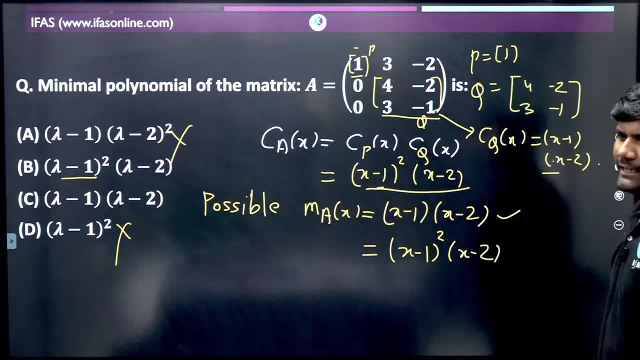 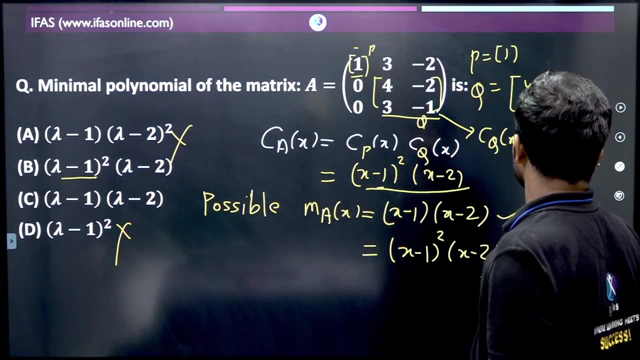 LCM. Absolutely, absolutely Fine, Bharti, you can also use LCM result. So now, here you have to decide its characteristic. Now you have to decide what will be its correct answer. Fine, Now, if you know its minimal polynomial. 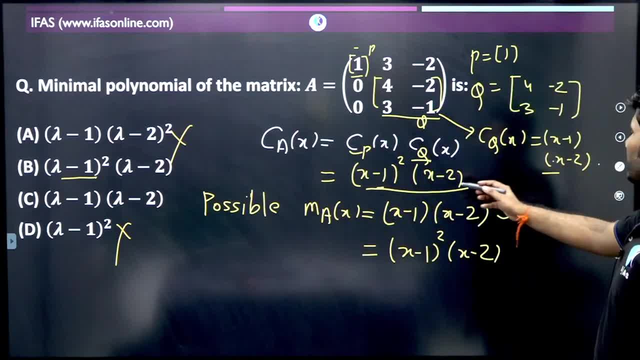 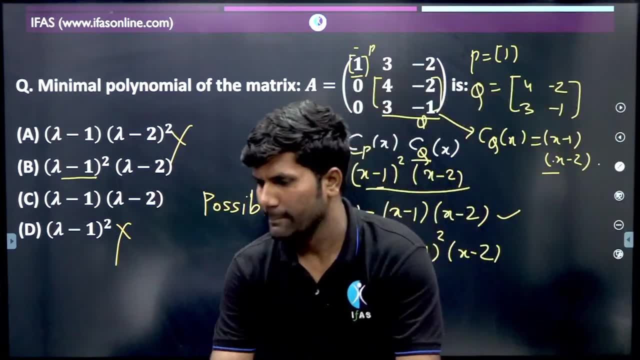 take LCM of both its minimal polynomial. If its minimal polynomial will be the same, because it is the same Now, if you take LCM of its minimal polynomial, then what will you get, Tell me? So I think this will go to option C. 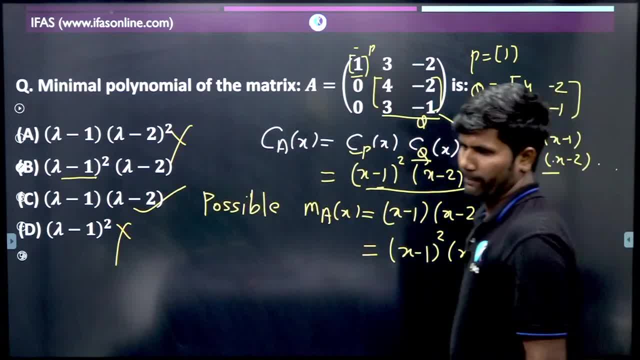 Fine, So here option C will be correct. You can also do it with LCM. Fine, Now here we have. let's take T from art. I have defined a map. T of q is mapped here. Now we are being asked: 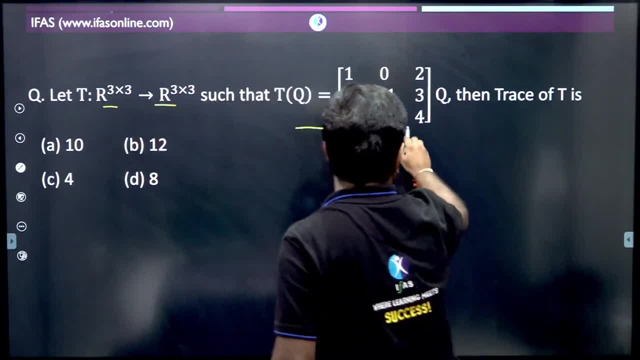 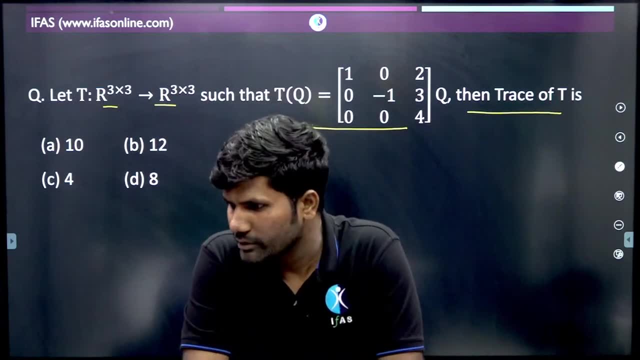 what will be the trace of T? Now tell me what will happen. Fine, Bharshali, Bharshali, double one, double one. I told you T, Fine, What is the answer of the rest of you? So there is a result for this. 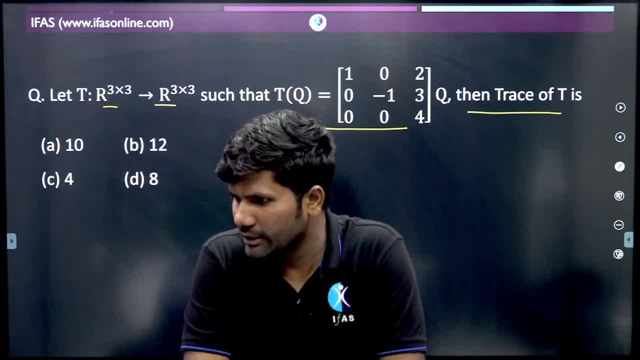 If you know the result, you can easily do it. What is the result? The result is: if you know it, you can easily do it. If you know it, you can easily do it. So what is the result? If you know the result? 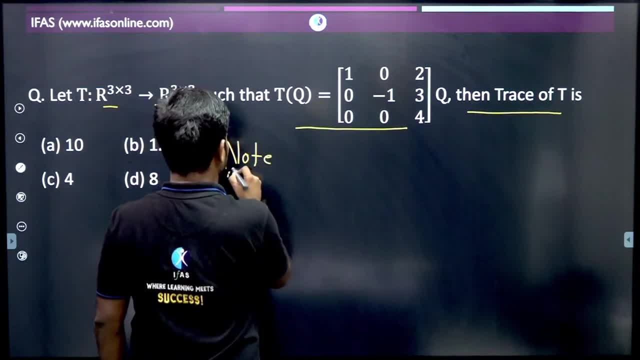 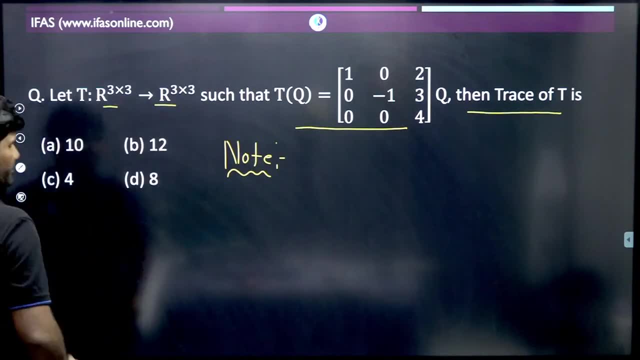 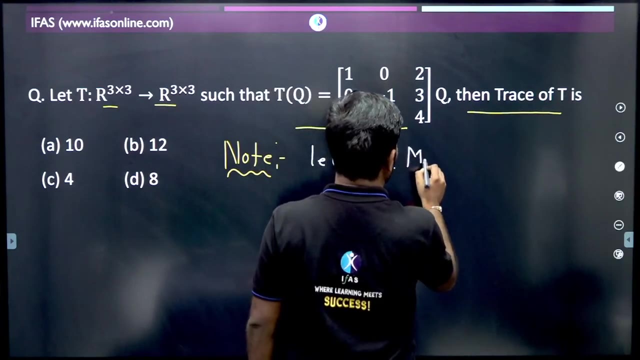 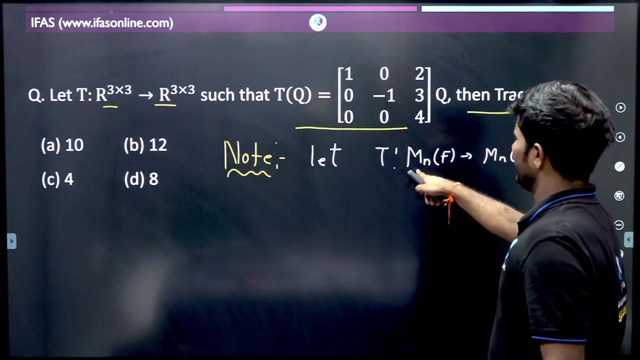 you can easily do it. What is the result? Let's see what was the result. It was a result that Let T give a map from MNF to MNF. MNF means You can write like this: N cross, N. Write like this: No problem. Defined by. 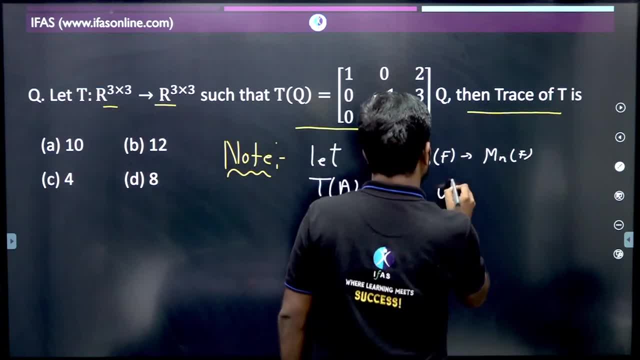 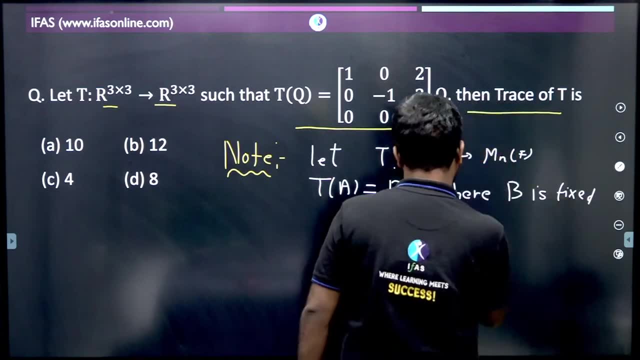 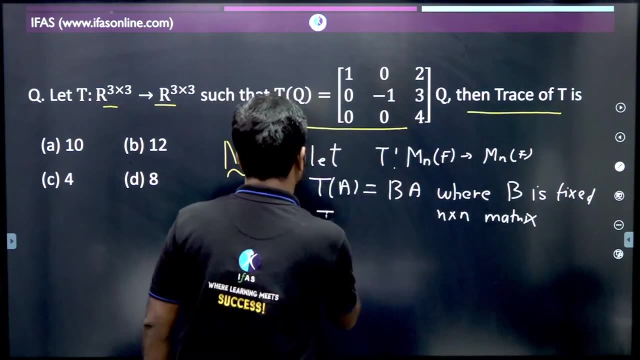 What was defined. T of A was mapped on B, A, Where It was said that Where B is a fixed matrix, B is a fixed N cross N matrix. Ok, In that case, What used to happen in that case Then? So here were some results. Let's see one by one. 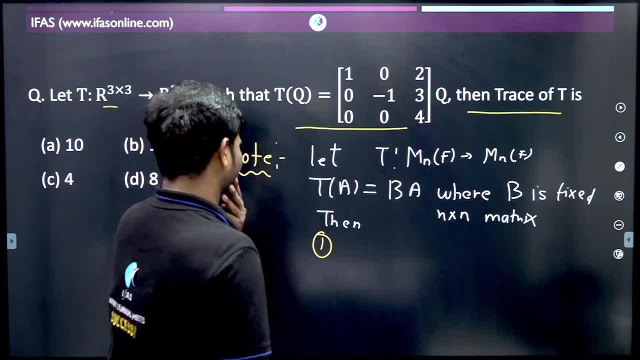 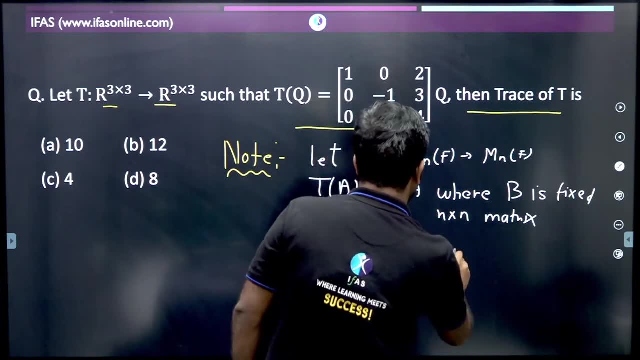 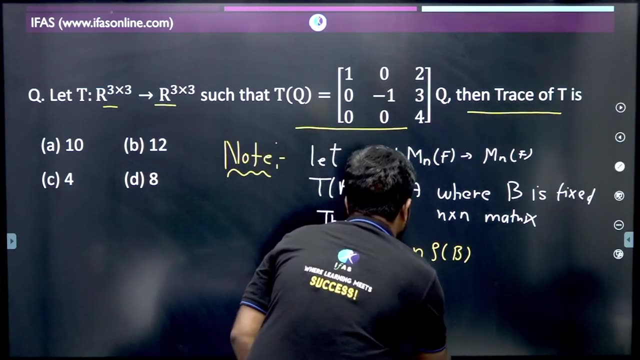 So what was said before? Now, here it is asked: Rank of Rank of A is equal to N times Rank of B. Ok, Second result: What was said: Rank of A is equal to N times Rank of B. And Third result: What was said? Third result: A was said. 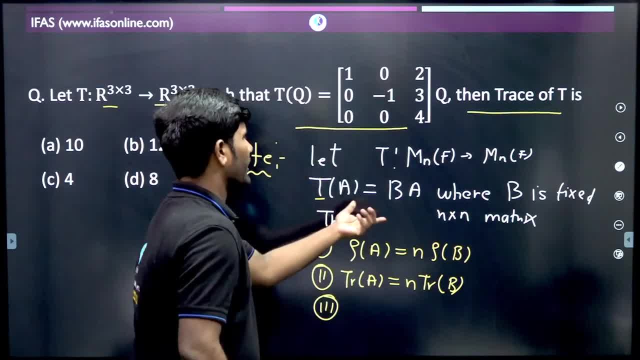 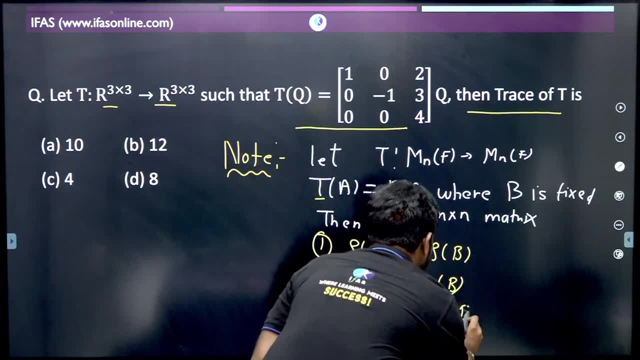 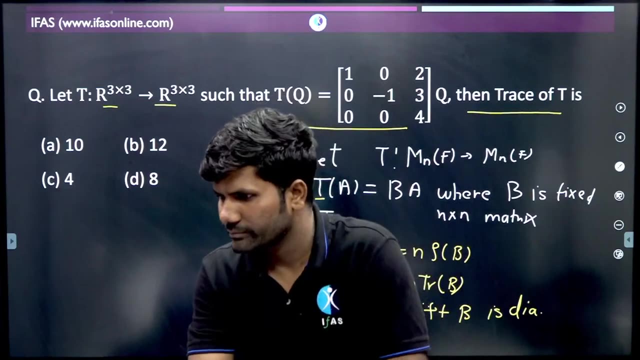 That This T. T is diagonalizable If and only B is diagonalizable. T is diagonalizable If and only B is diagonalizable. Ok, So What you have to do? Use this result Now Use it. You tell me What you get For Sum of A, For sum of. 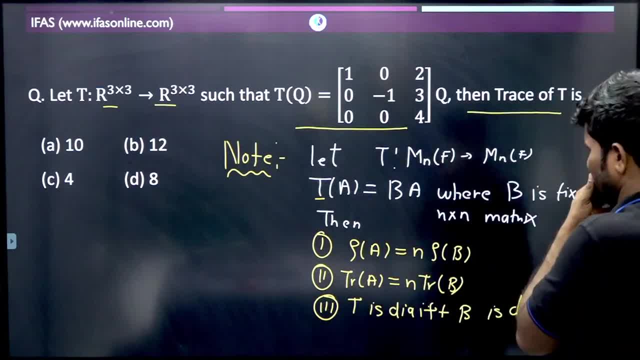 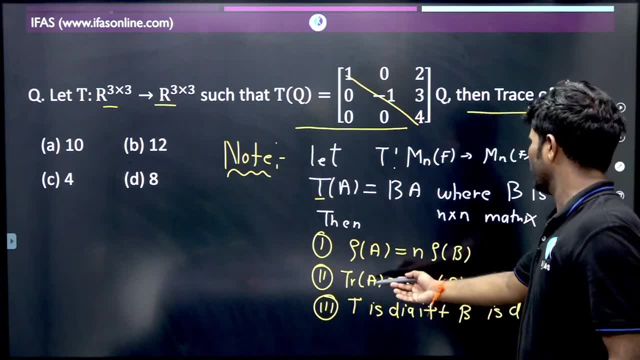 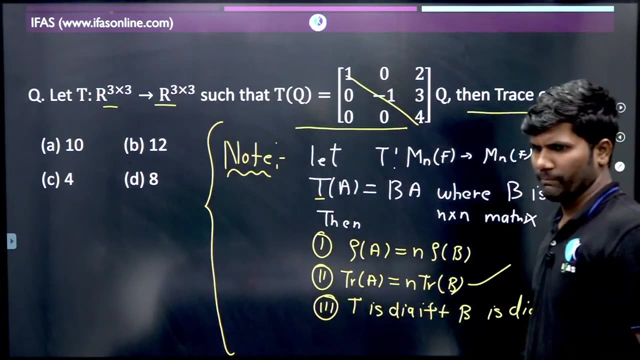 Eigen values- Triangular matrix. Ok, Sum of Eigen values. If you find, How much will you get Eigen value of this Sum of Eigen value? Or Find trash, Use this result. You can tell easily. If this result is known, You can easily Solve this question. Ok, So all students. 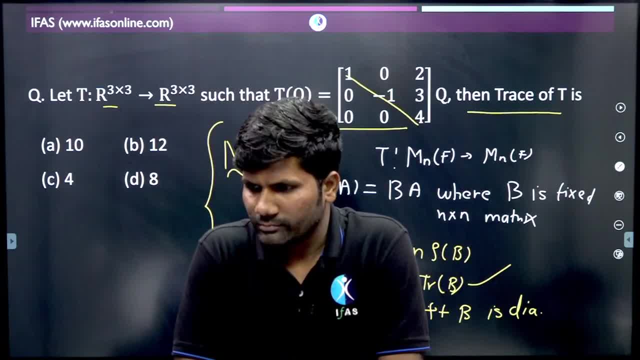 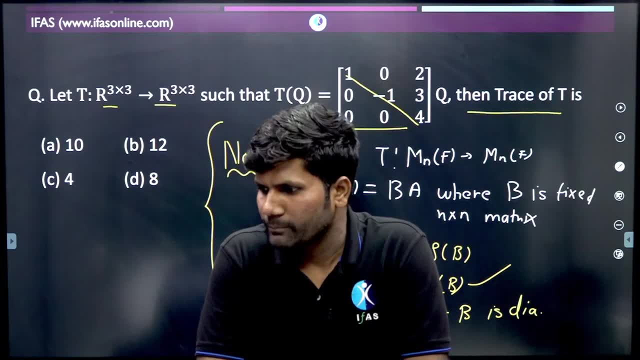 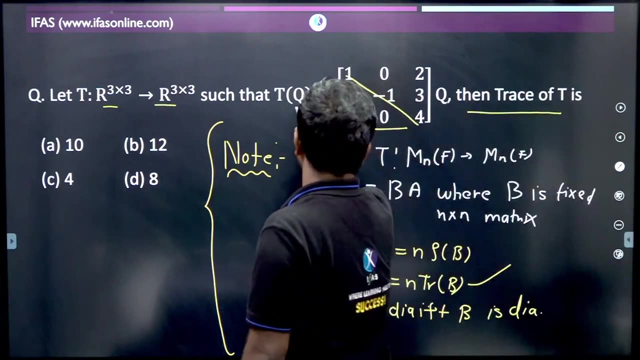 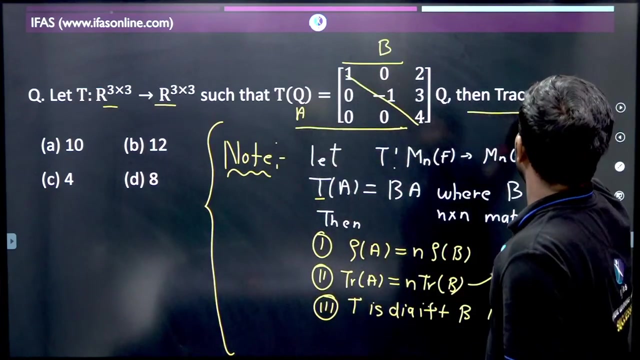 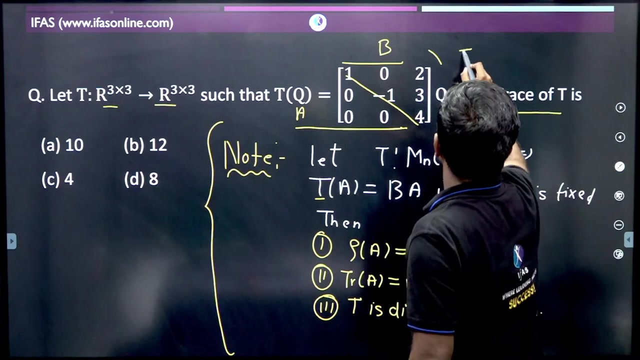 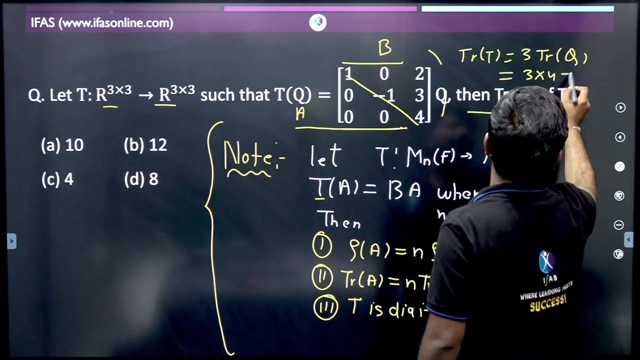 Solve. Tell me What will happen. Yes, All People. Tell me What will you get? Answer: See, See, This is All Very Wonderful. The Here Pay Pay. You Have Your Pass cortex Comp identification is: I Have Bottom tiene A Too. I Am So Want. Does So I? Next, and the correct answer will be given here. 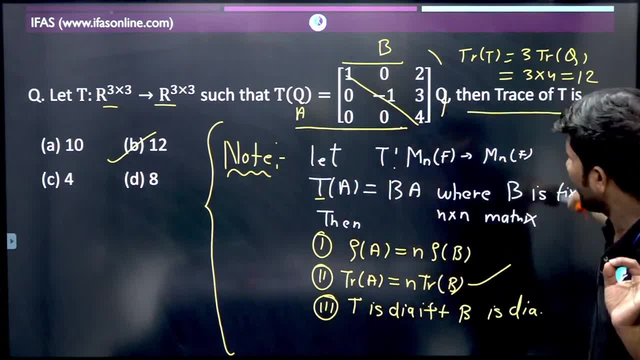 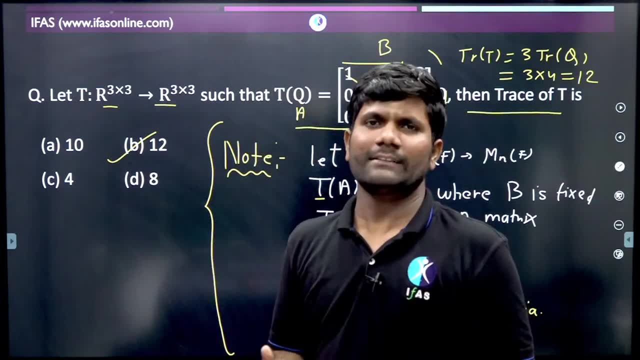 did you understand. so just keep this result in mind. if you know the result, then you can solve it easily. this type of question is asked in JAMA and NET, so there is a chance that Maharashtra will also come in the state. ok, just keep this result in mind. 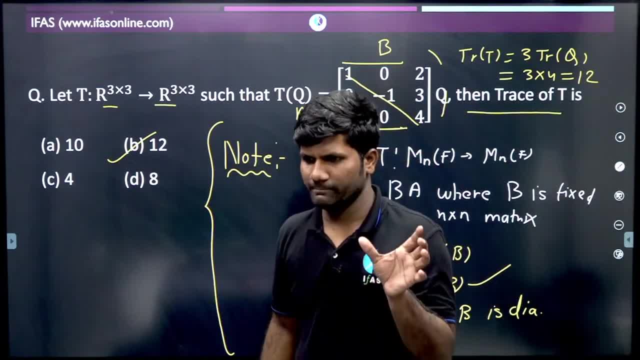 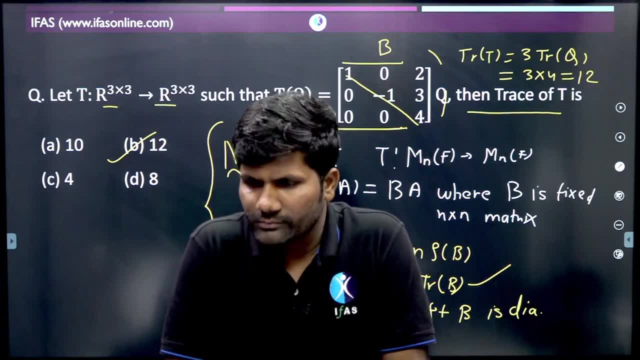 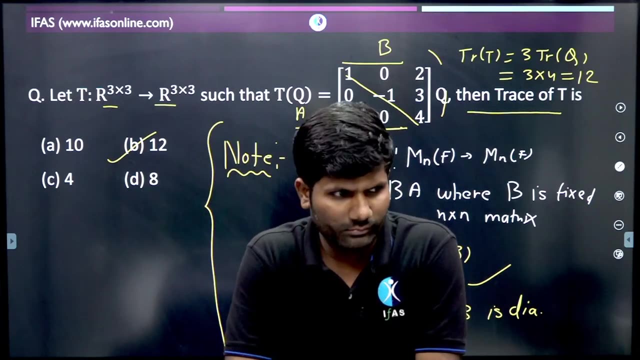 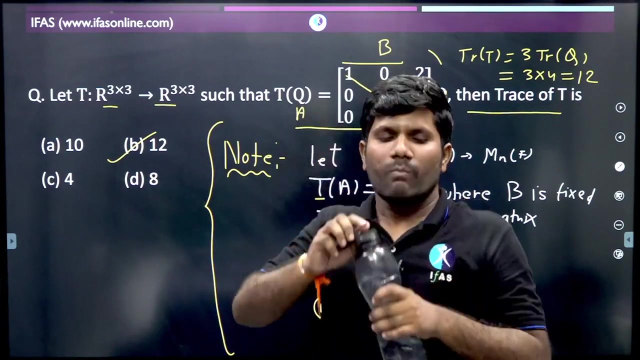 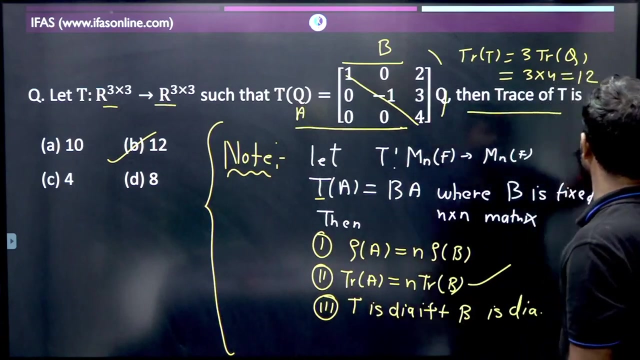 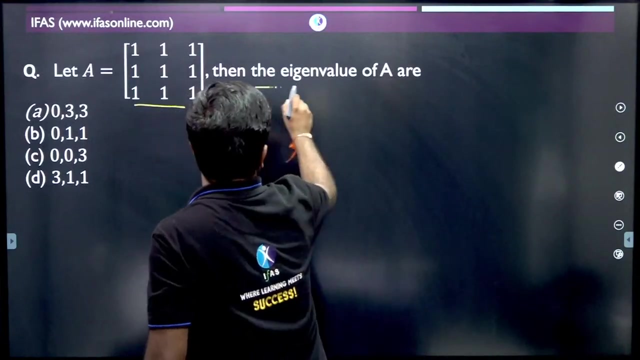 so you can solve it easily. is it clear, all students, let's go ahead. tell me once. is it clear, all students, let's drink some water, let's go ahead. so here we are, given a matrix, then the eigenvalues of A. so here we have three options. 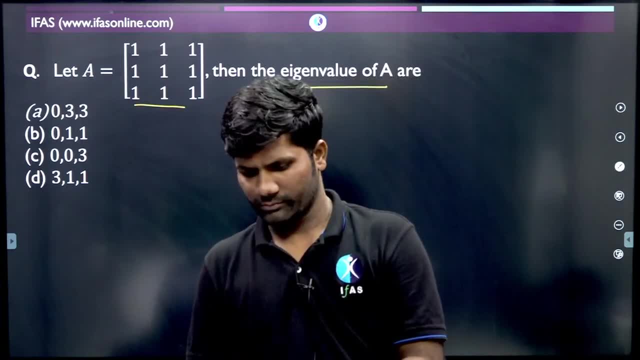 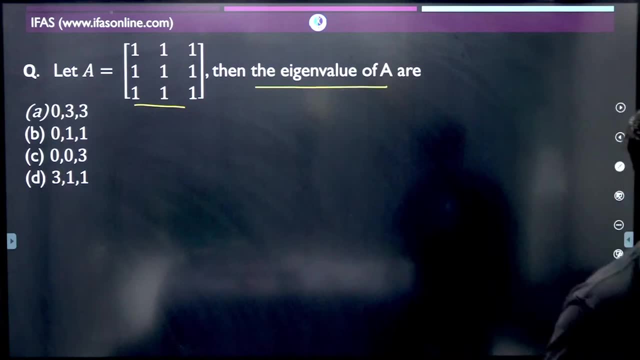 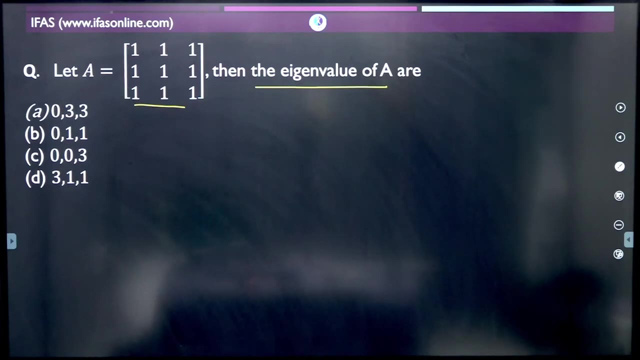 solve it and tell me, will we get the correct answer quickly? ok, it's very simple. what's the question, what's the answer? OK, but I don't know. we'll see what's the answer. ok, as you can see, there is a very long. 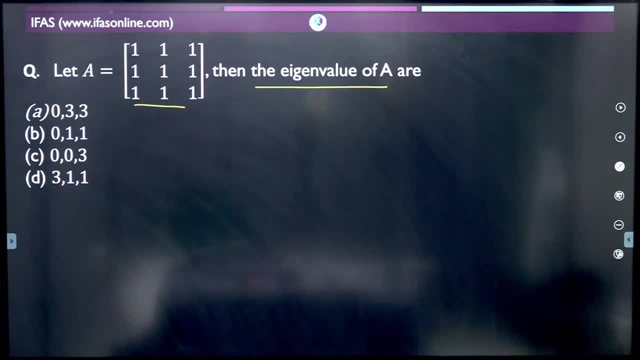 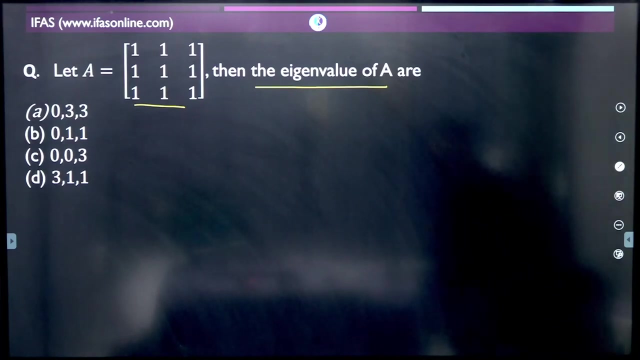 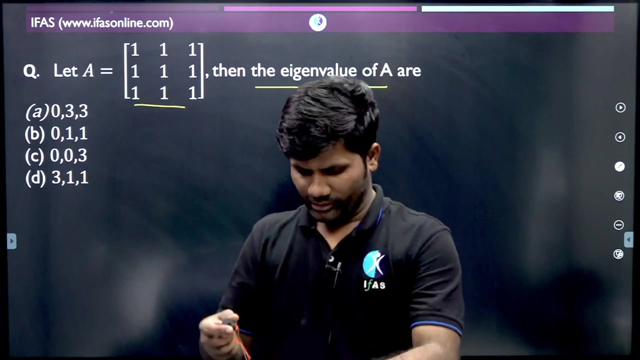 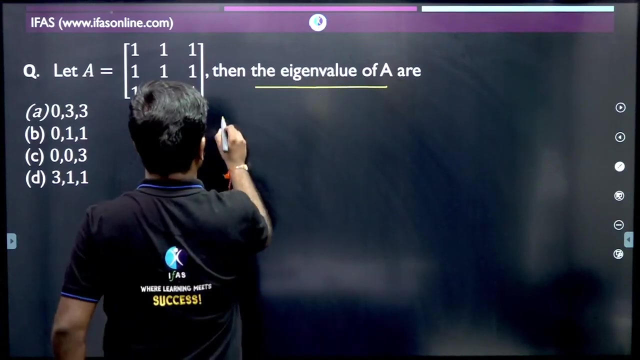 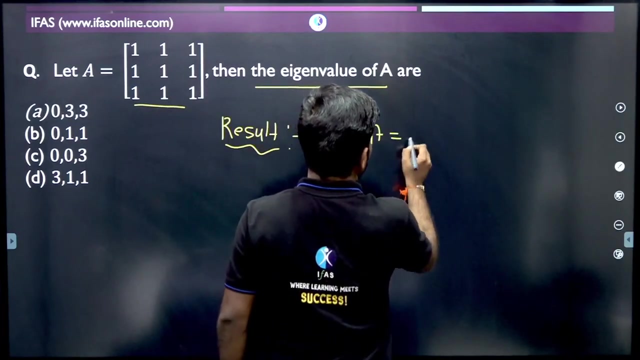 sequence of answers. you let's go tell what you got answer. so almost everyone is saying cc, let's go for. this is a result. what does the result say? if you know the result, then you can solve it easily. let's give this matrix: what are all the entries of? c, c, c, c, c. 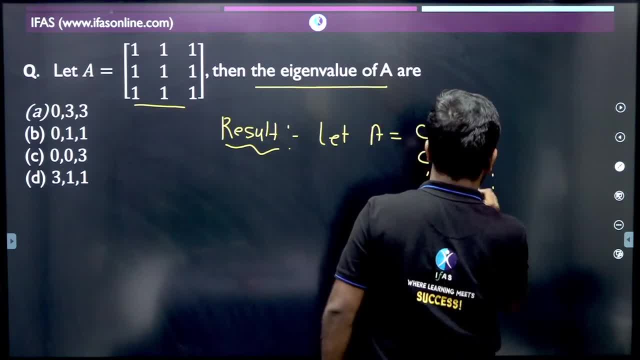 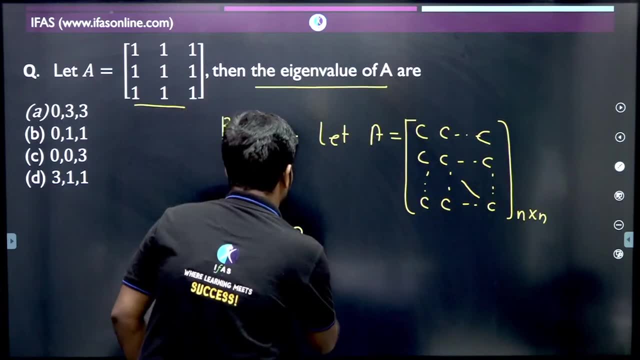 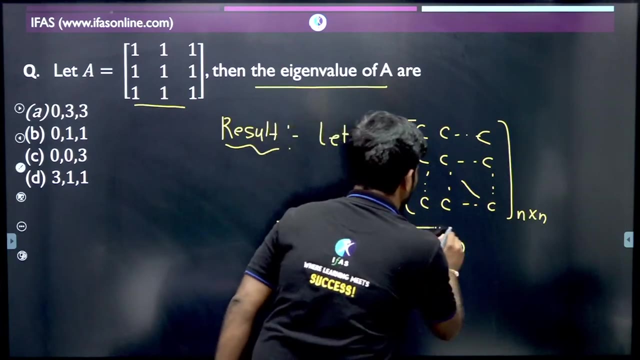 give some constant. all the entries are c, c, c. here is some constant. in that case, characteristic polynomial is c, x, x raise to n minus 1 and here will be x minus n, c. so what you have to do is use this formula. you can solve it easily. 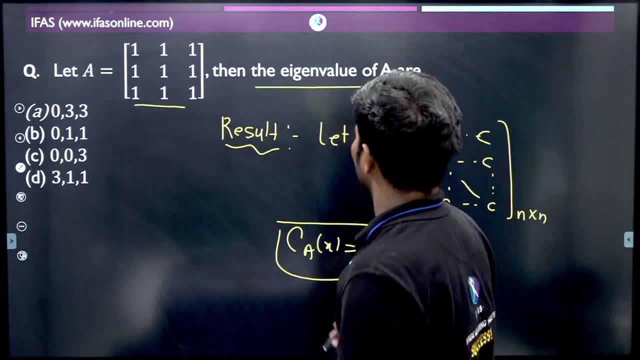 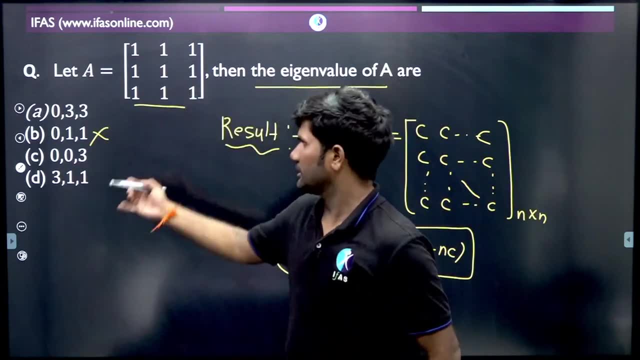 if you see here, there is one result and sum of each row is 3, which means 3x will be its eigen value. so it will be finished from here. 3 is not in this. if you see here: if you substitute the value for 1, then what will you get? c, ax. 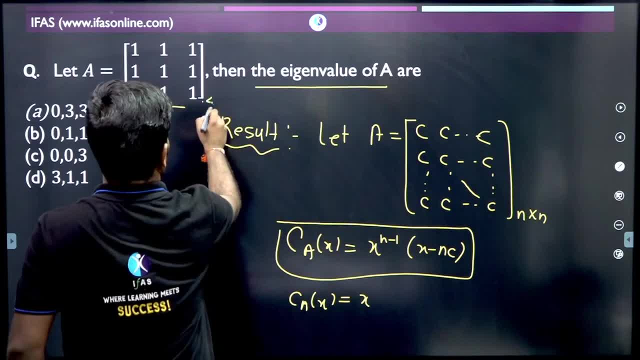 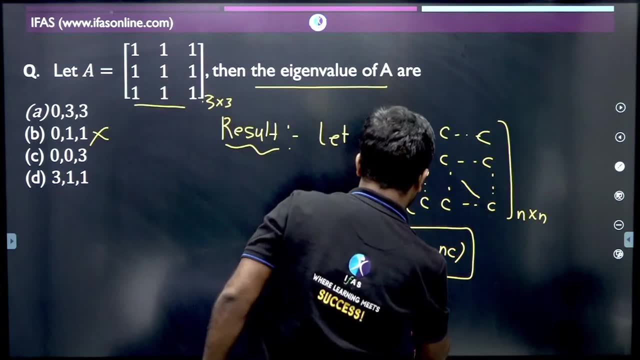 x raise to n minus n has value 3, cross 3, so here n has value 3, so x square. and here x minus 3 into 6th element is 1, so it will be 3, so here eigen value will be 0, 0. 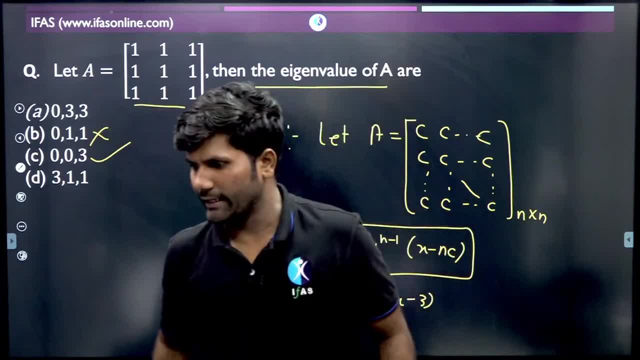 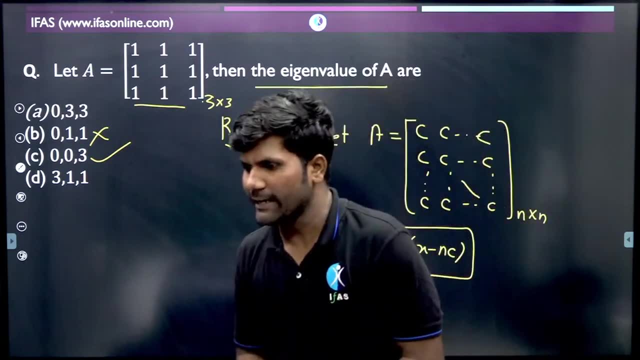 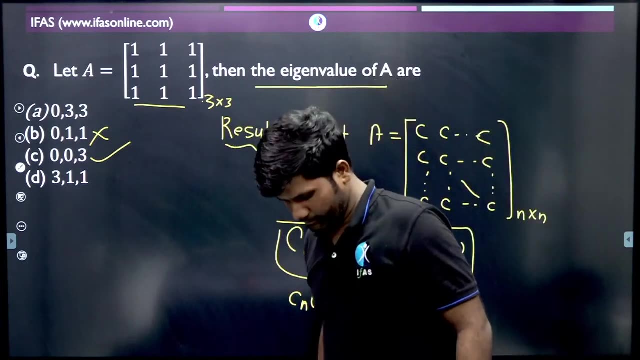 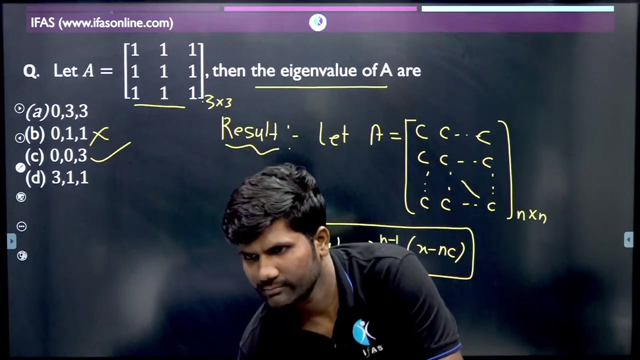 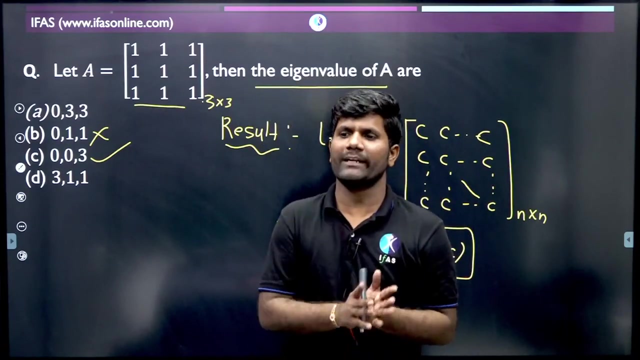 so this name means the option is correct. perchali, do like this, this go faster. ap kareem, do like this, you will get faster. ok, for constant. there is collect result. ok, everyone keep moving forward. you are getting cheese, ok. ok, If it is clear, then you guys comment once, let's go ahead. 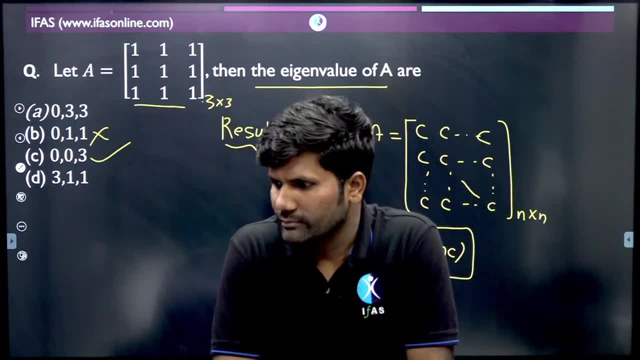 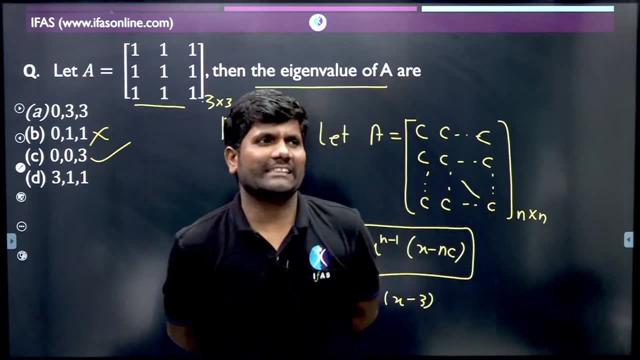 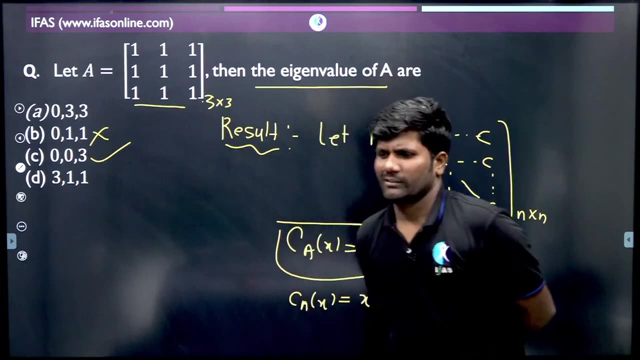 All students quickly comment. Is it clear to all of you? So such questions can be asked in Maharashtra set. So what you have to do is linear. questions are simple. You don't have to take it lightly thinking. it is simple. 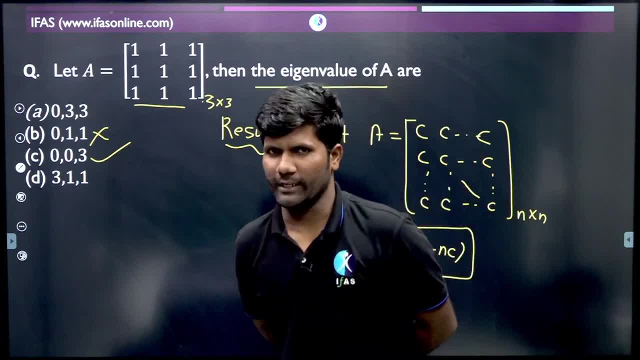 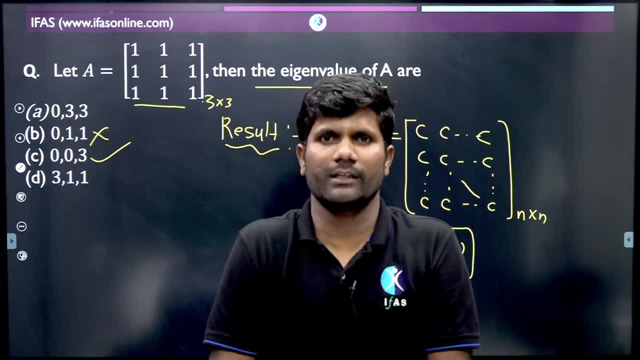 You don't have to do that. if I know it suddenly, then it goes wrong there. Okay Means you don't have to do difficult questions to pass the exam, You have to do simple questions. If you have done simple questions wrong, then you can't pass. 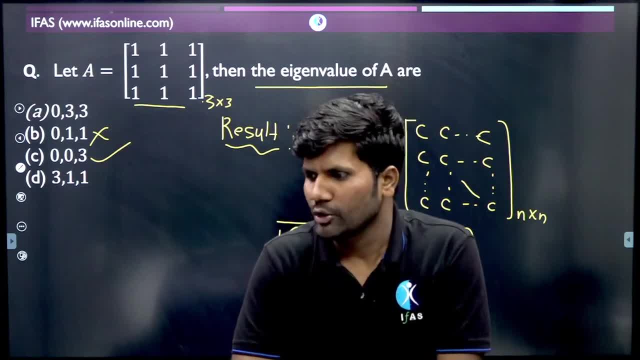 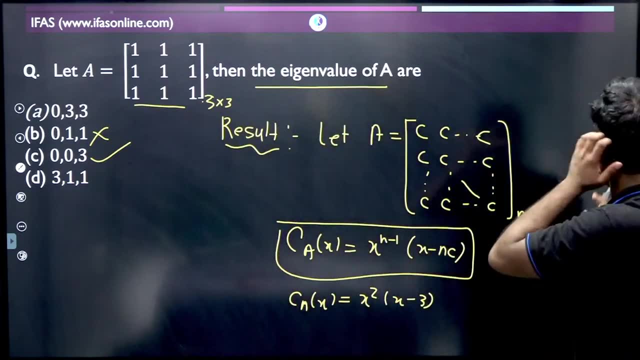 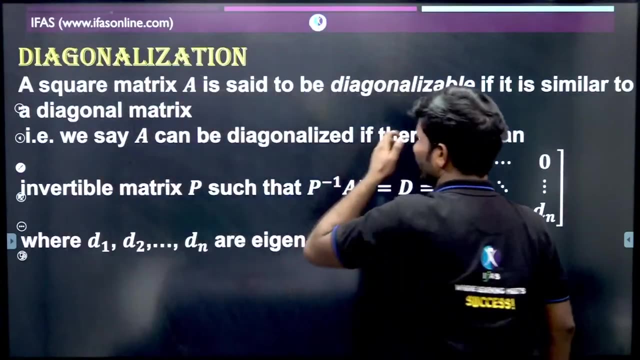 So what you have to do is first of all select simple questions and correct it. Okay, Anu Yadav, Sheetal Again, let's go ahead. Some of our silent students who don't speak on time? Okay, now the diagnosis has come. 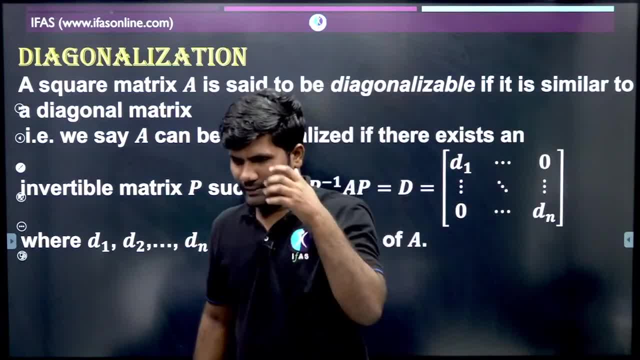 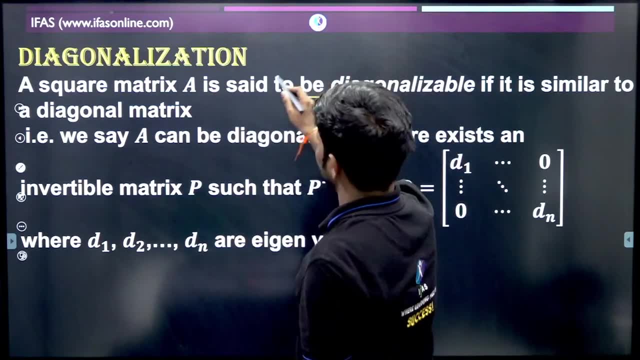 Once. tell you the definition of diagnosis, Okay, Or go straight to the question: Tell me what do you want? So any matrix we call a square matrix A as diagonalizable only when it is similar to a diagonal matrix. 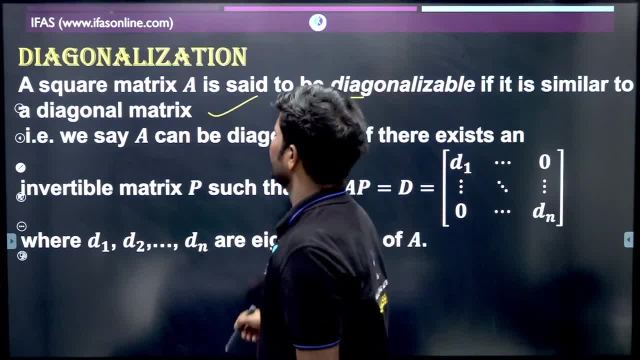 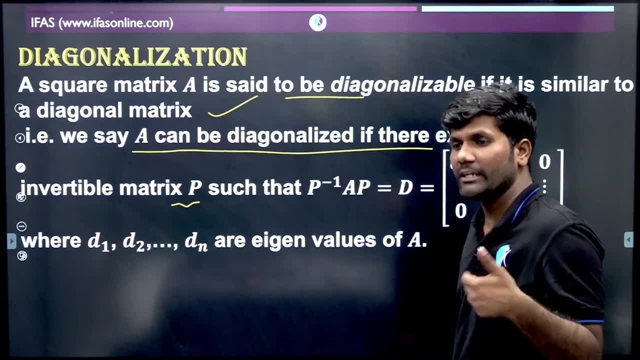 Means some row operation has been done to bring it to a diagonal matrix, And in other words we call any matrix as diagonalizable only when we get an invertible matrix. What kind of matrix, Invertible P which satisfies this condition? where P inverse A P is found in diagonal matrix equal. 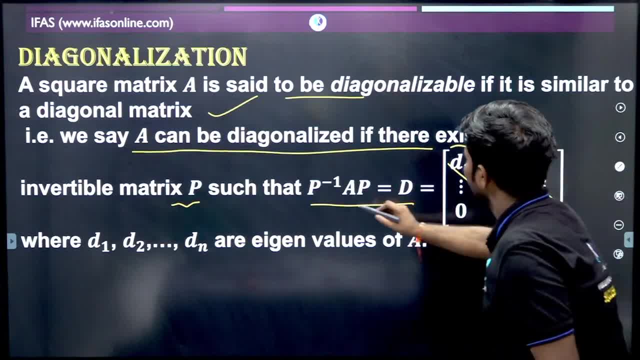 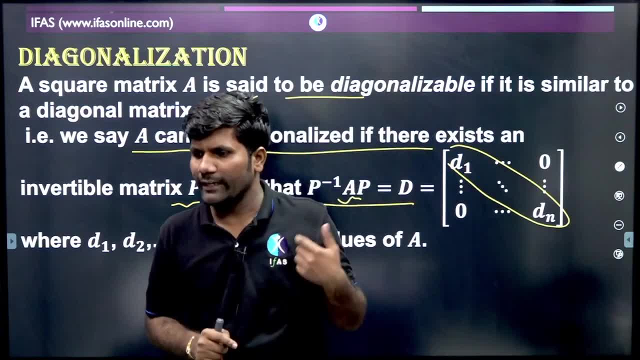 So in this way diagonal matrix is found. So in this way this D1, D2, Dn are one matrix with a eigenvalues. Okay, Now, it won't be easy to do this again and again, So for that there are some results and properties. 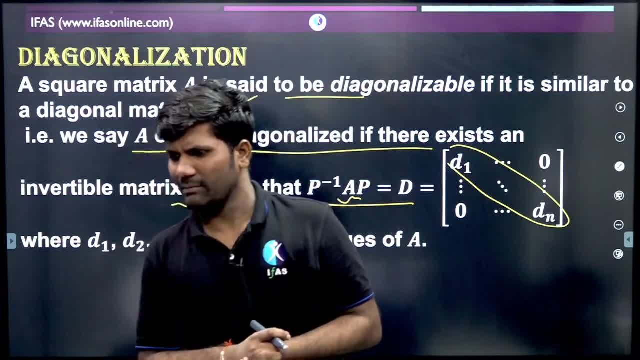 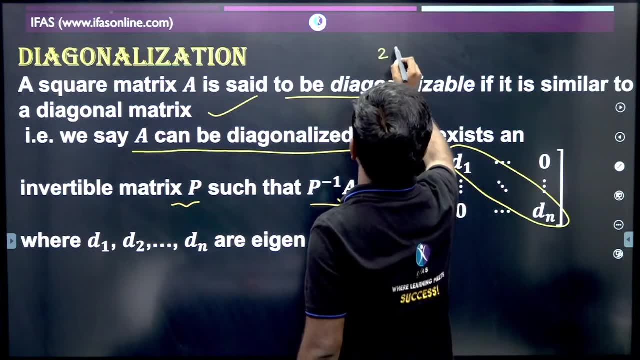 Lalit Kapawa. Sir, how to find the last two digits of power number Do model of 100.. To find last two digits. like any number is given, 20 raised to suppose 30 is given, It is said to find last two digits. 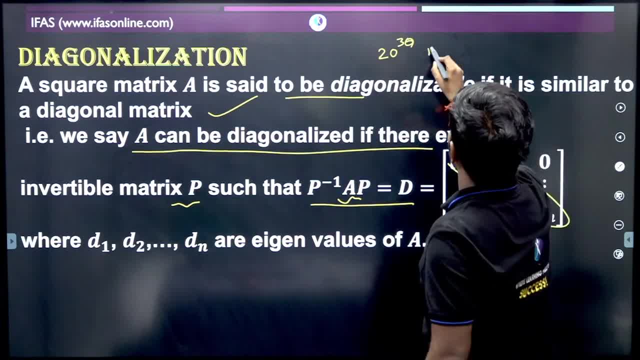 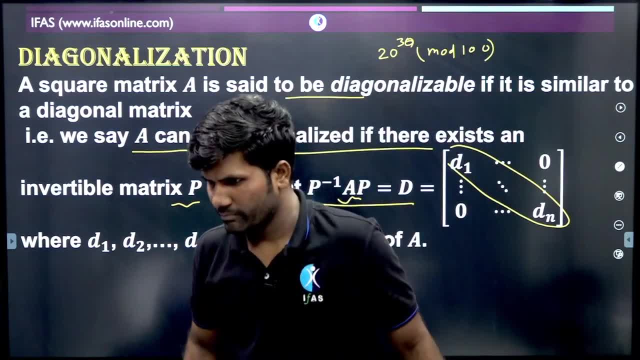 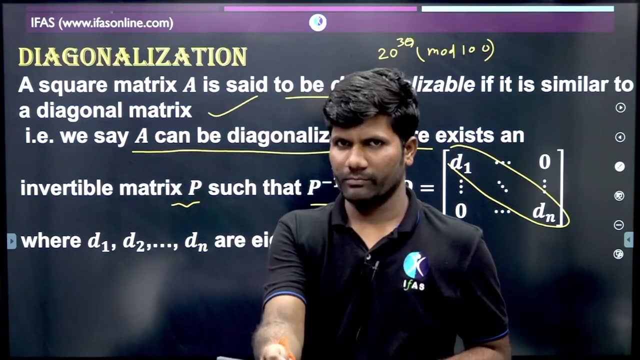 Then what to do? then what you have to do is modulo 100 here. modulo 100 and perform the operation and you will get Lalita Power. Sujata Net's online batch is starting from 23rd, after 3 days, and offline is starting from 1st October. 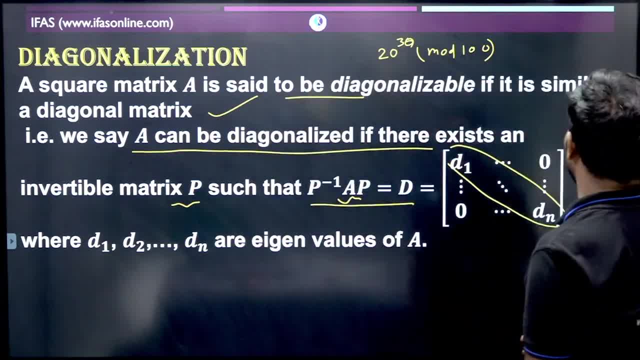 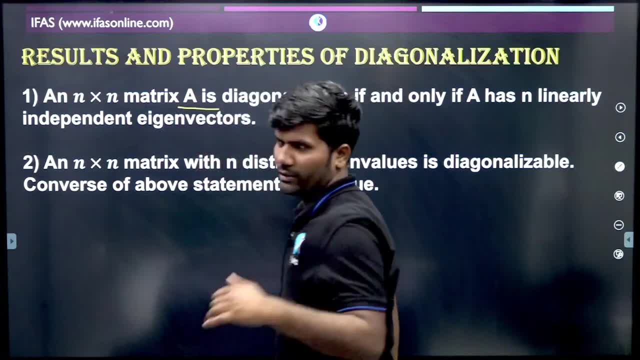 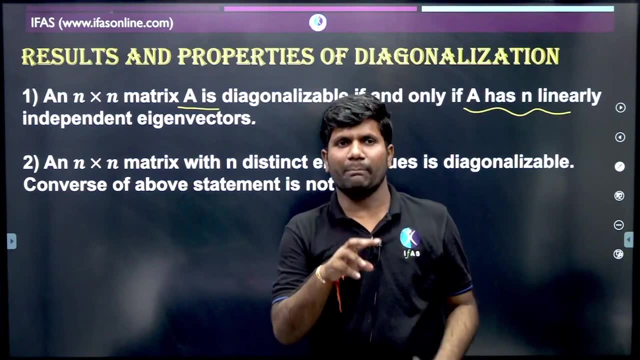 absolutely zero matrix is diagnisable. now let me tell you some results. any matrix will be diagnisable only if matrix n cross n. matrix is diagnisable if, and only if, it has n linearly independent eigenvectors. if any matrix has n linearly independent eigenvalues. 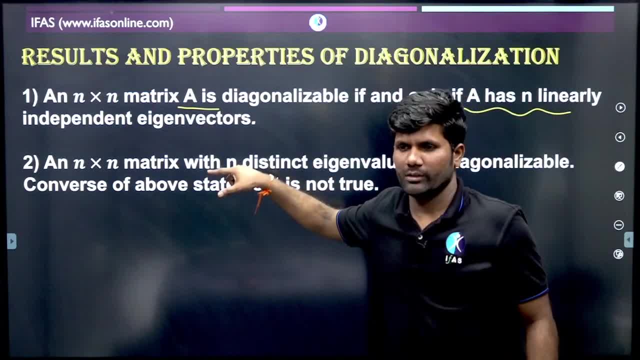 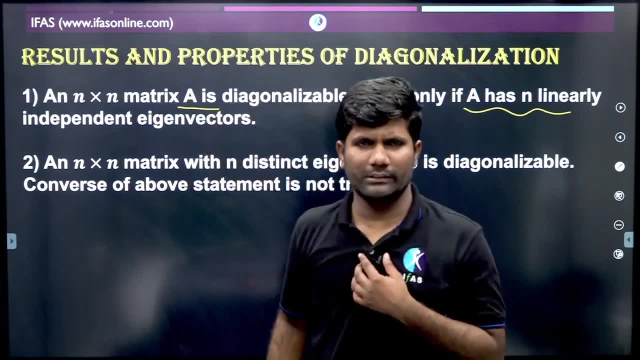 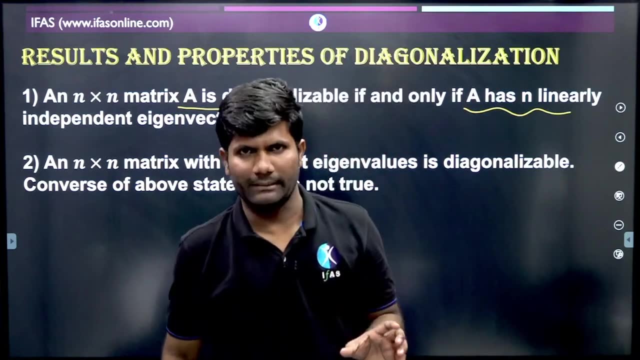 then it will be diagnisable. it is necessary and sufficient. condition means both direct part and converse are true, Anu. remember online batch is starting from 23rd, see. once you are given the link, our team will provide you the number in the comment section. rest of the details you can take from there. 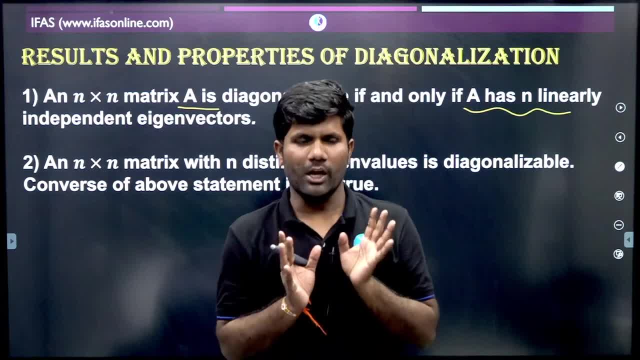 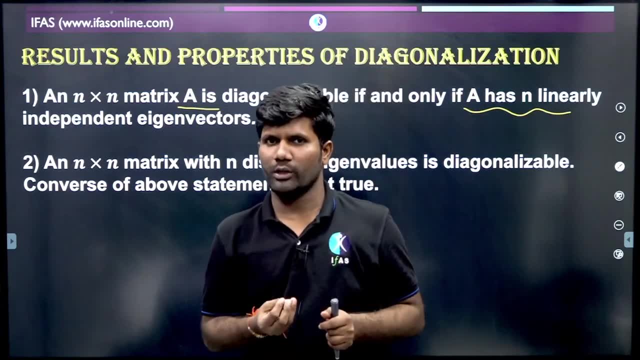 online batch is starting from 23rd to 3 days. so the special thing about this online batch is: if you have any doubt, then what will you do? you can type and ask. if you want to ask through audio or through video, all three facilities are available. 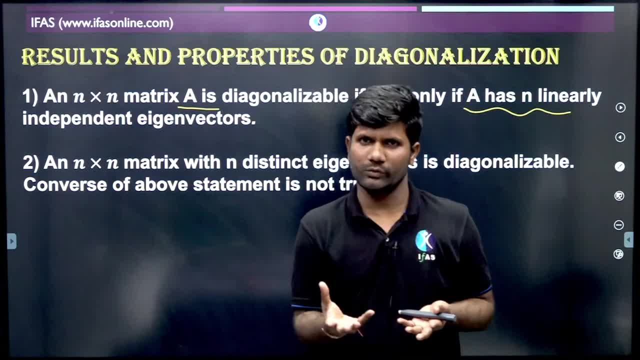 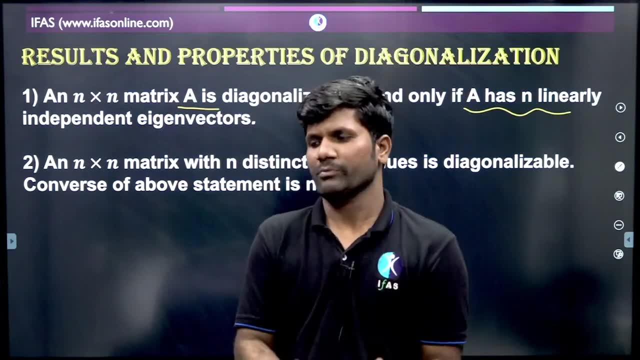 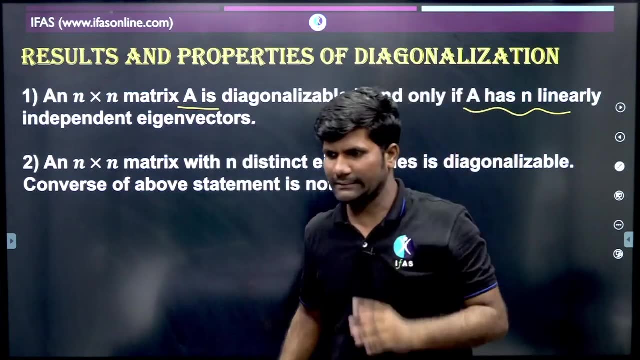 along with that. DPP means after every lecture you will get practice questions, Sunday test and teacher hand out. you will get all the things in a proper way, in a systematic way, as per the rules. is it clear? so our online batch is starting from 23rd. 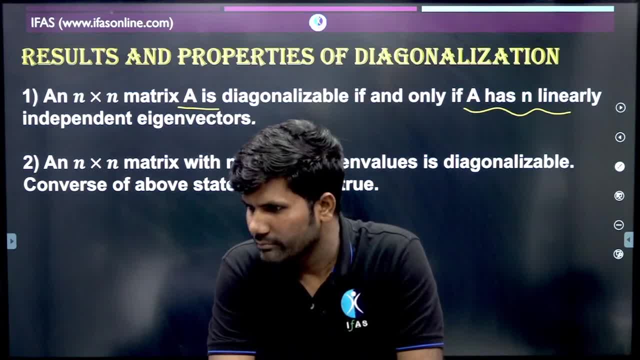 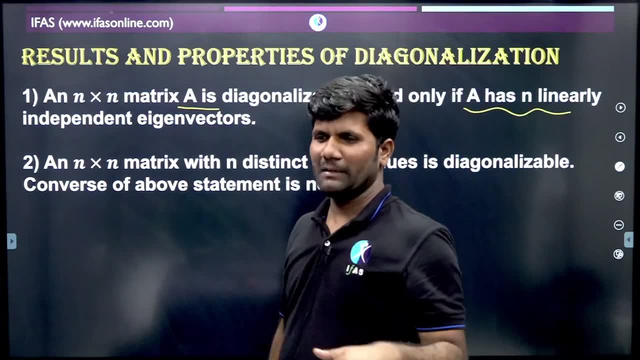 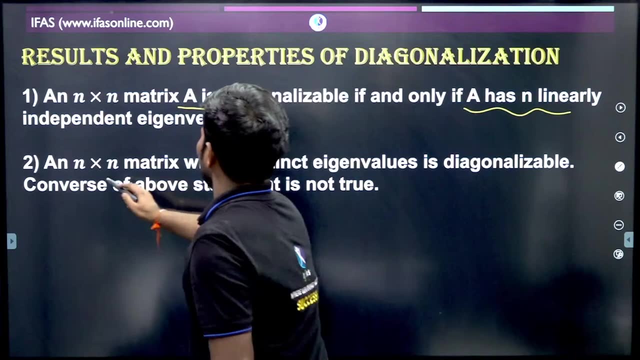 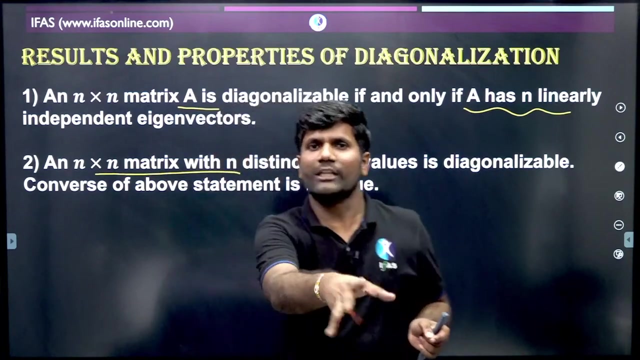 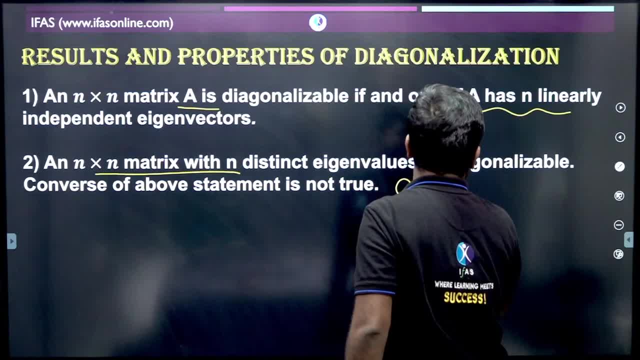 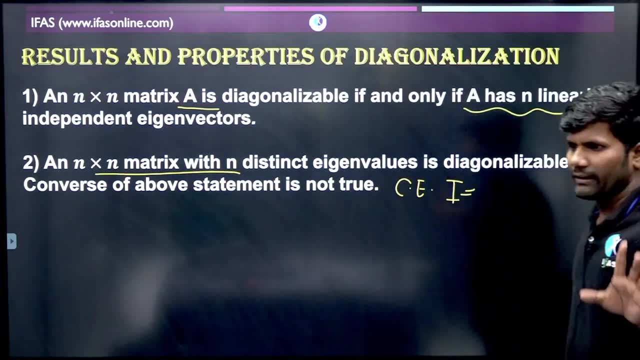 converse is not true. for counter example, take identity matrix. identity matrix, all eigenvalues are one. then also, it is diagonalizable. it is not distinct. okay, it is clear till here. now let's come to the next slide. there are some results and properties. we come by telling it is diagonalizable. 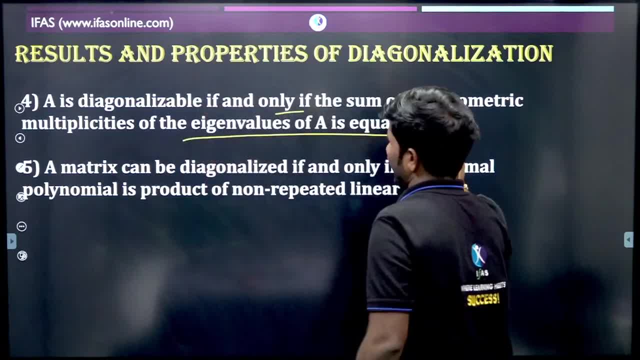 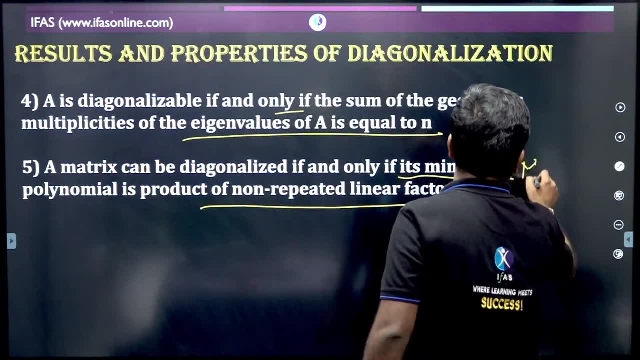 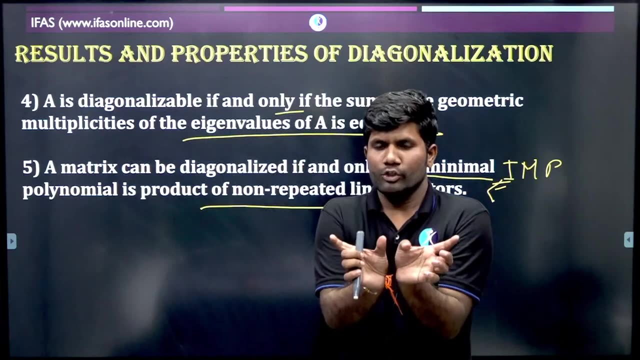 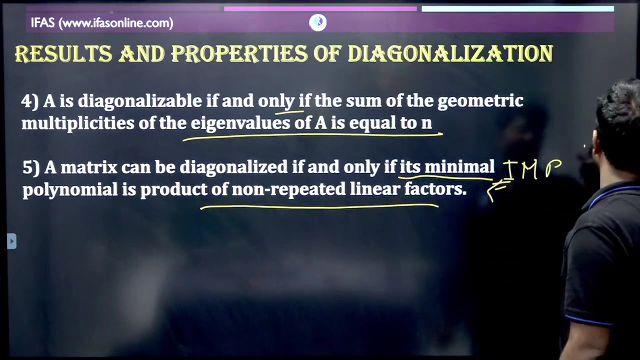 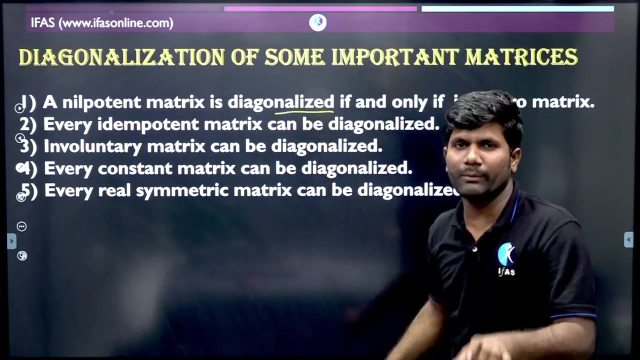 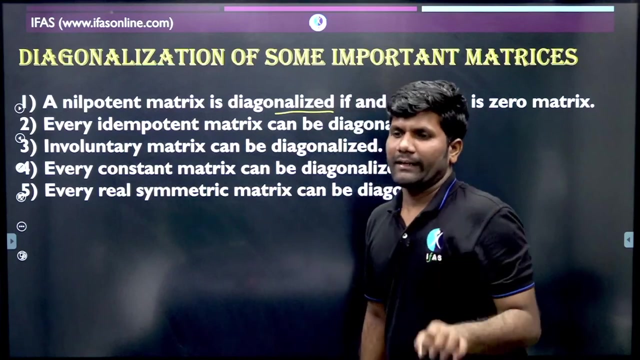 if, and only if, sum of the geometric multiplicity of eigenvalues equals to n, a matrix is diagonalizable. if our minimal polynomial is product of non-reputed linear factor, is NILPOTENT MATRIX NEVER DIAGNOLIZABLE. NILPOTENT MATRIX IS DIAGNOLIZABLE. 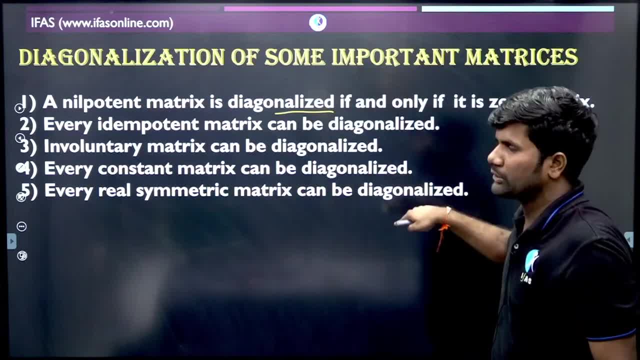 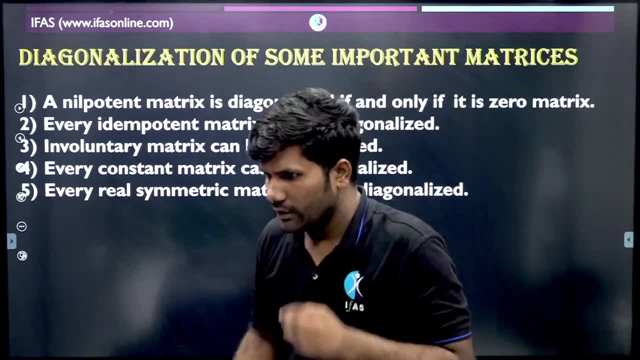 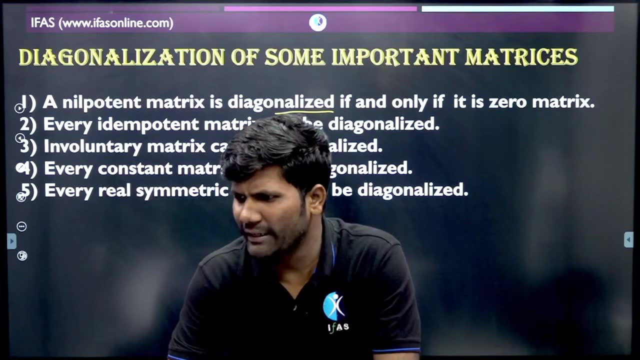 IF, AND ONLY IF, IT IS A ZERO MATRIX. from here i can say that ZERO MATRIX IS ALSO DIAGNOLIZABLE, which is TRUE sujata. call me once, see me. as far as i know- i think it will be till 7- you call me once. i am not confirmed. 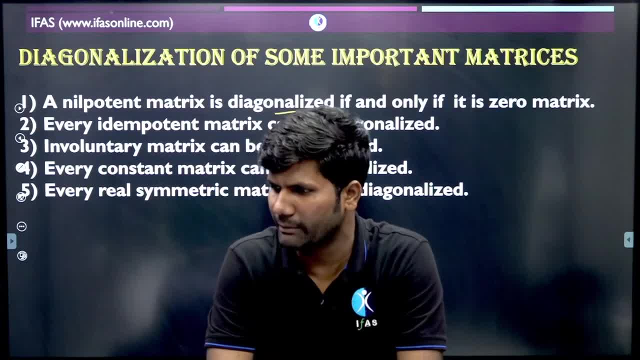 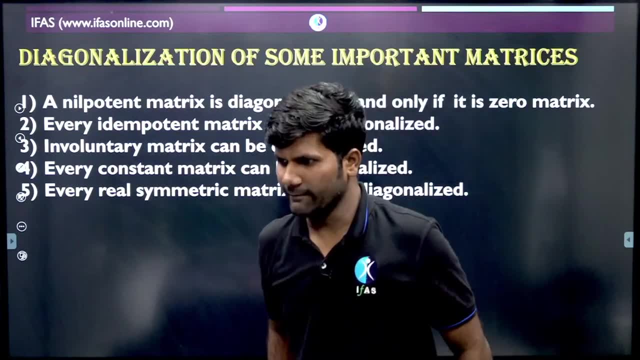 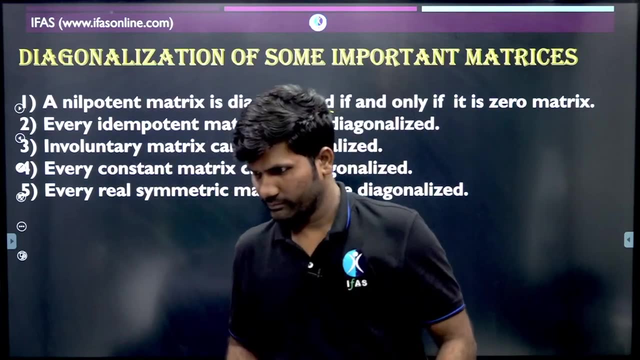 see, i have given you the number from both the numbers. call me on the first number. if it is not 7, then call me. otherwise, talk to me tomorrow after 10. you will get the rest of the details from there. arvind for you also, sujata. 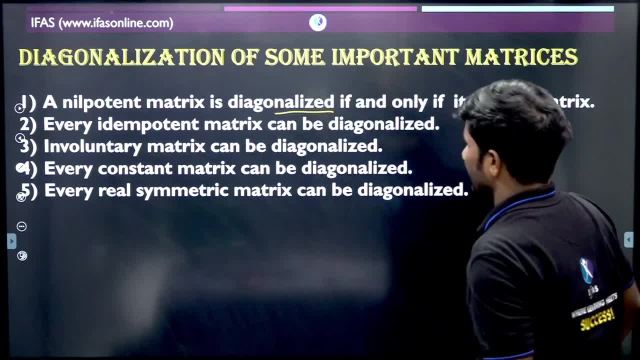 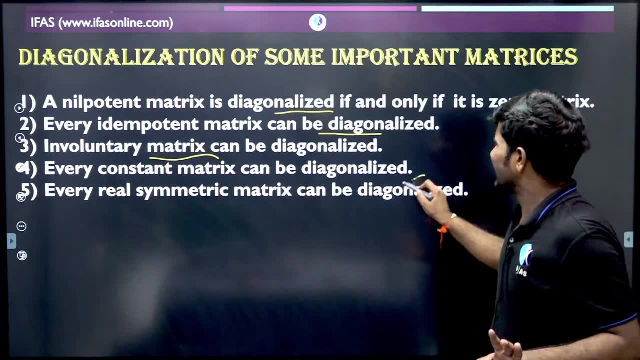 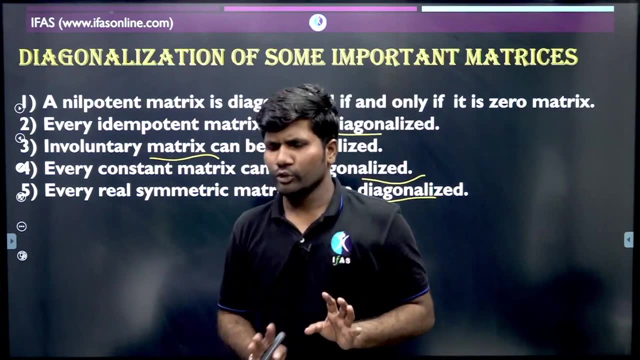 arvind. you both can do this. ok, now what is here? every idempotent matrix is always diagonalizable. rotary matrix is always diagonalizable. constant matrix is always diagonalizable. real symmetric matrix is also diagonalizable. if you know so many results, then on the basis of that. 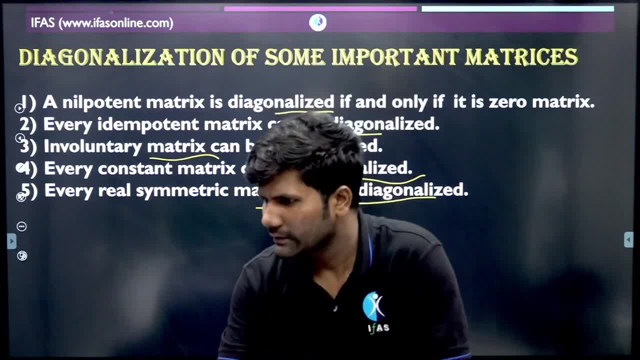 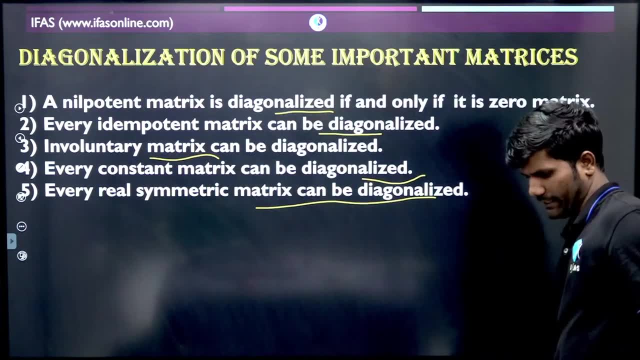 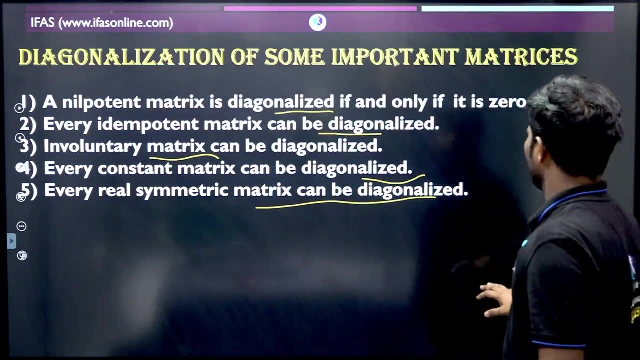 all the problems, diagonalizable. almost all the questions. you will do 99% ok. where it was not uploaded, we will do it ok. let's come to the next slide. i hope till here you will be clear. now we have seen the results. let's see the applications. 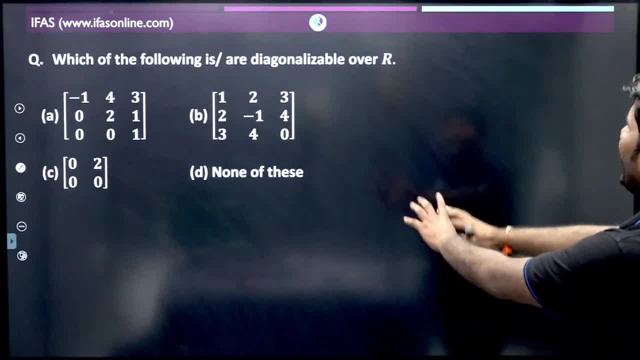 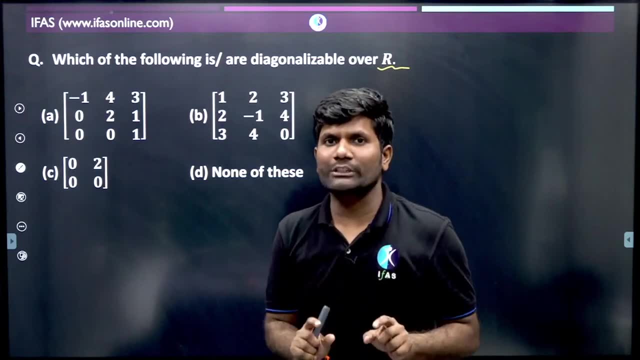 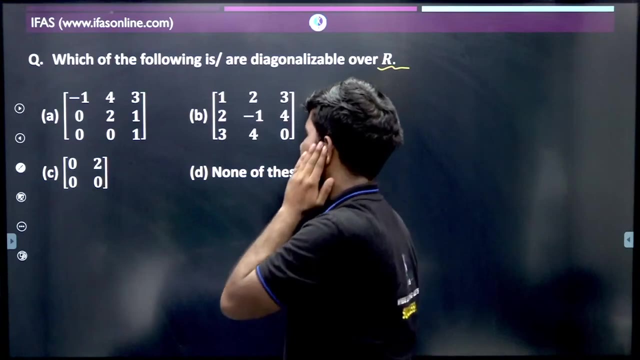 ok, which of the following is, or are, diagonalizable over R? so matrix is said to be diagonalizable over R. when it is diagonalizable and where all the eigenvalues go in the real number. ok, so keep this in mind. now solve: is it diagonalizable or not? 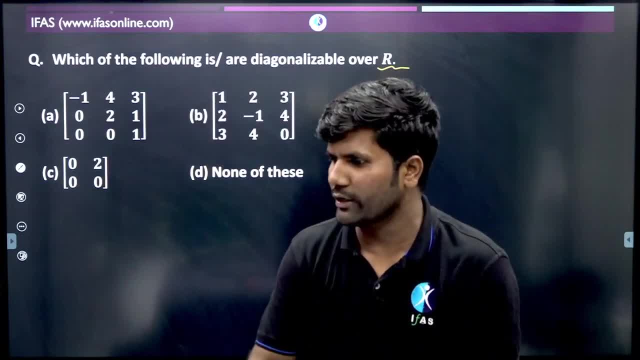 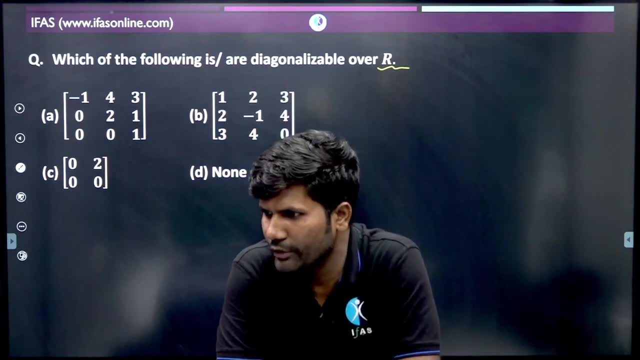 quickly solve which option will be correct. bhakti nagpal lalitha pawar dilip sujata bharshali. ab kareem panu yadav lalitha pawar pallappal. tell me the truth. 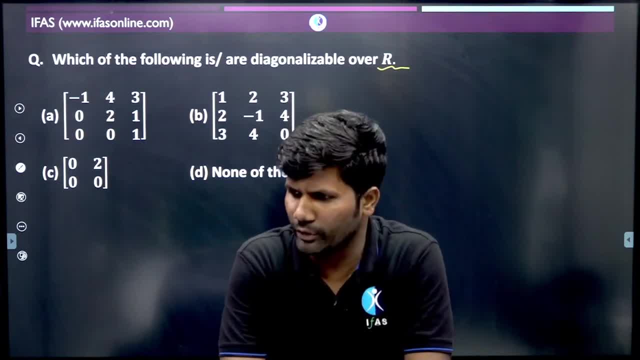 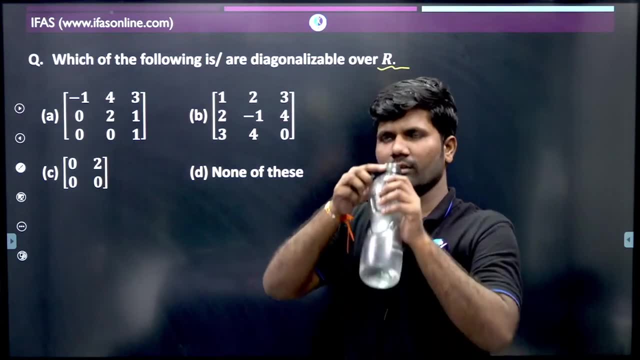 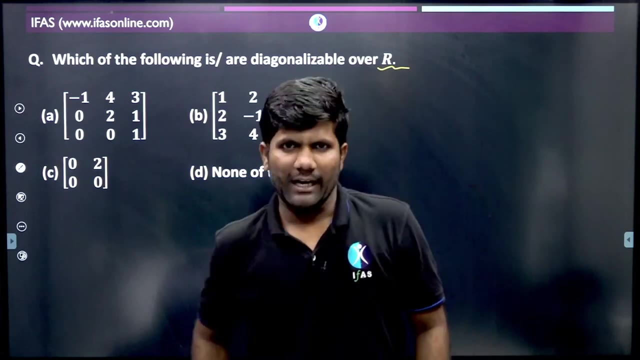 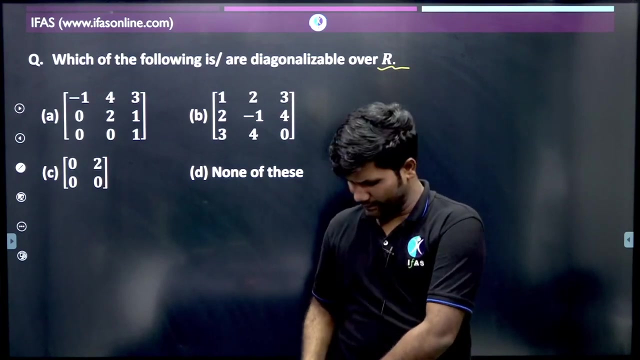 if you prepare for net, then the set is done automatically. there is no effort for that. ok, now in the general category, i think 52 to 53 to 54% cut off, which can be done easily. ok, very good. bharti lalitha very good. 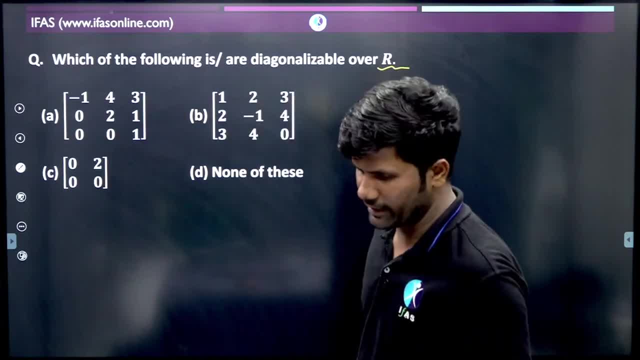 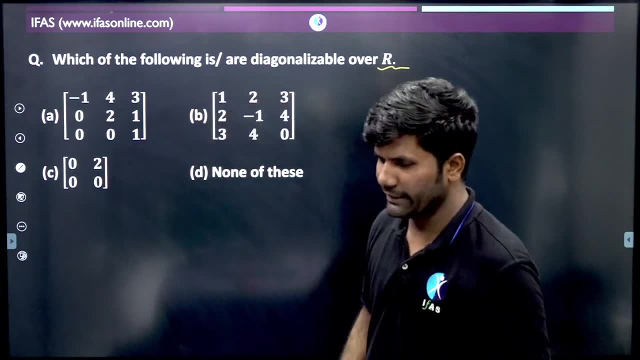 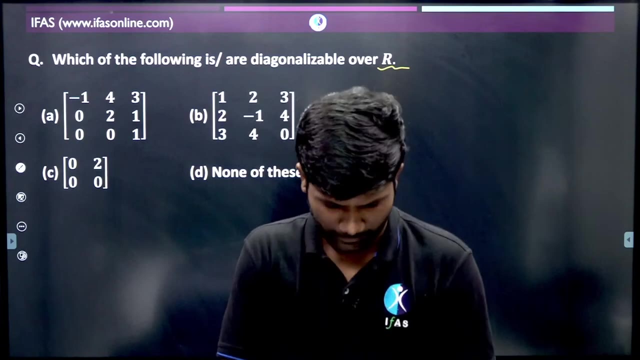 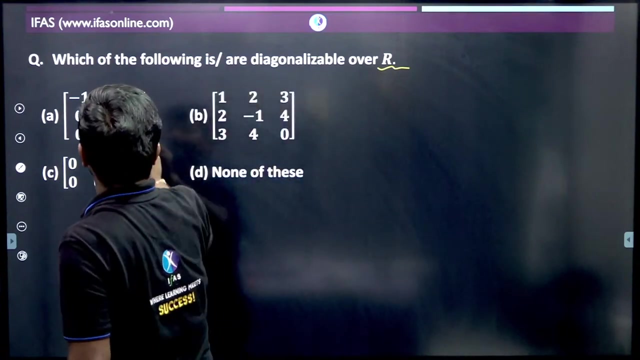 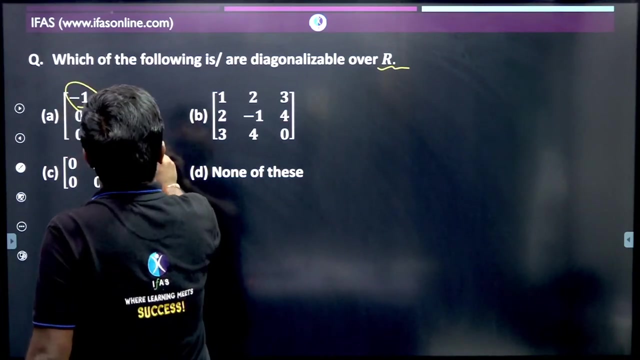 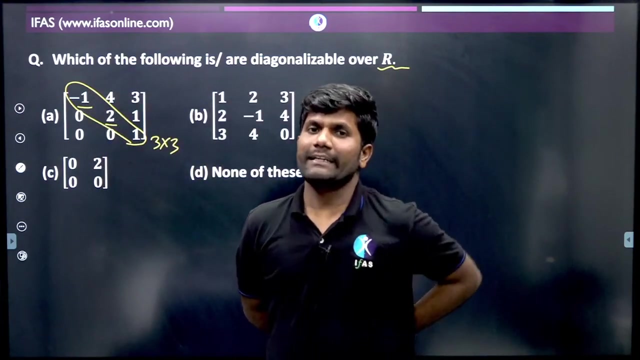 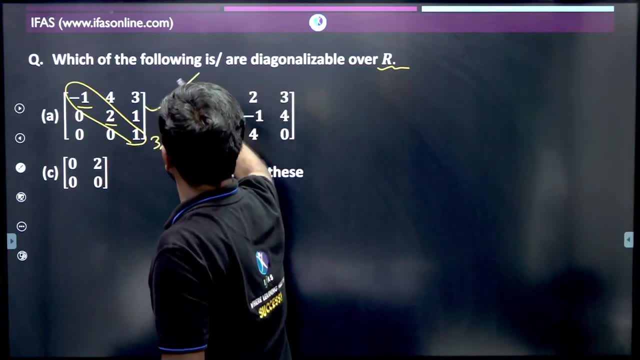 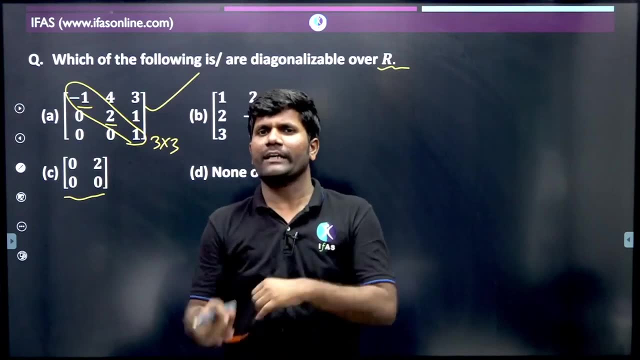 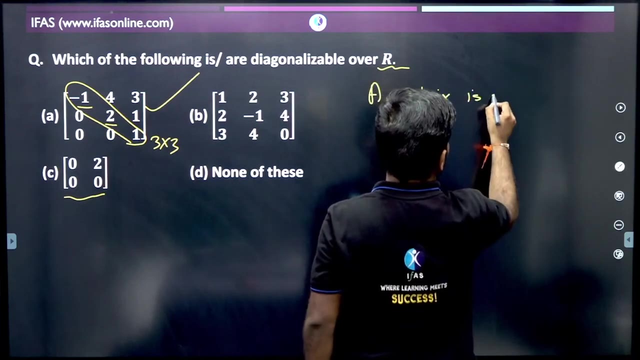 so here we are asked which diagonalizable a is correct? and option b, option b? along with this, there is a result. what does the result say? a matrix is nilpotent if, and only if, all its eigenvalues are zero. a matrix: a matrix is nilpotent, any matrix nilpotent- square matrix. 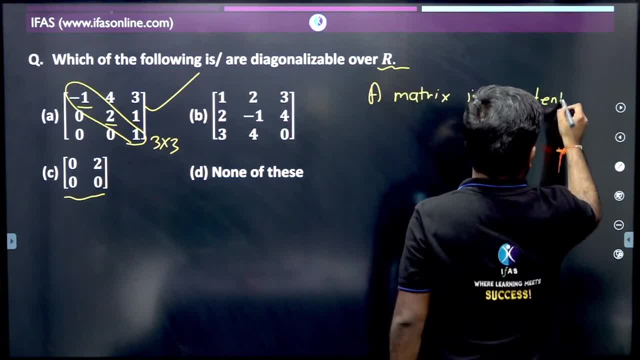 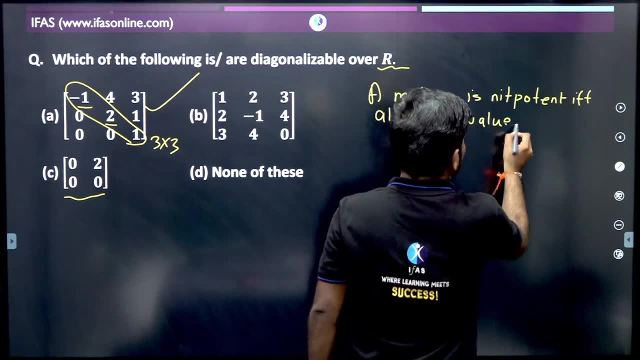 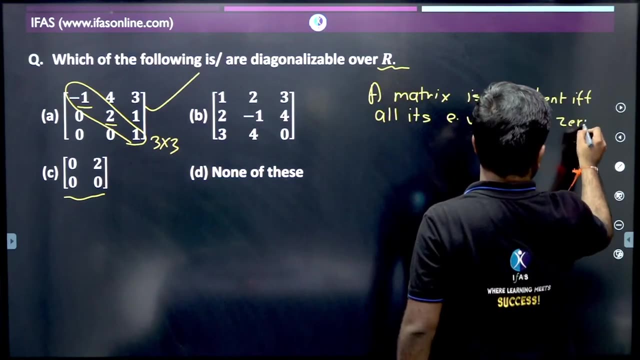 a matrix is nilpotent if, and only if, all its eigenvalues are zero. all its eigenvalues are zero. if such a matrix is given, all its eigenvalues are zero and matrix is nilpotent, okay, eigenvalues are zero, so use this result. what kind of matrix is this? a is nilpotent. 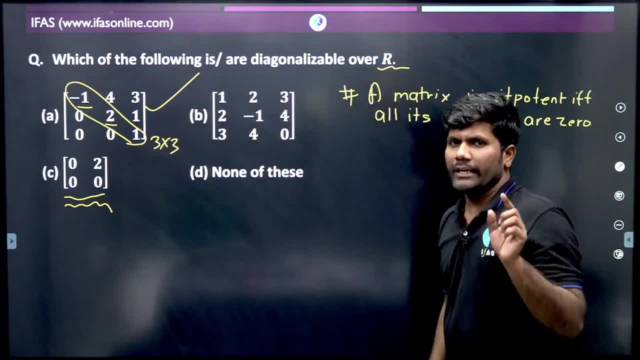 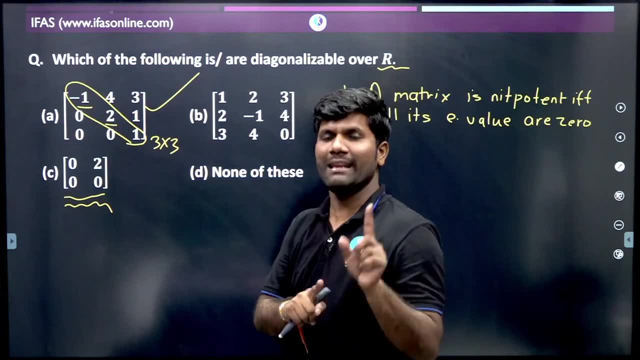 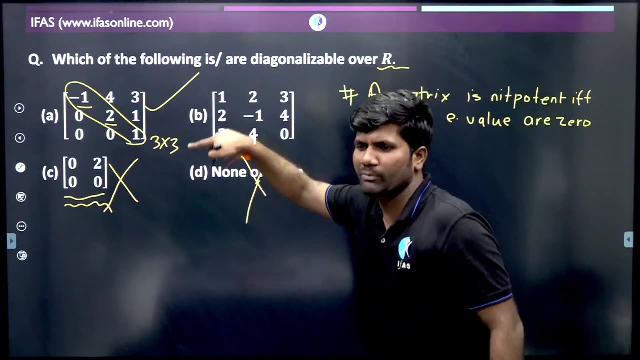 matrix, and we saw last result: that a nilpotent matrix is diagonalizable if, and only if, it is zero matrix. non-zero, nilpotent matrix is never diagonalizable. it means that option c is incorrect. option d is also incorrect. now let's come to option b. now tell me what. 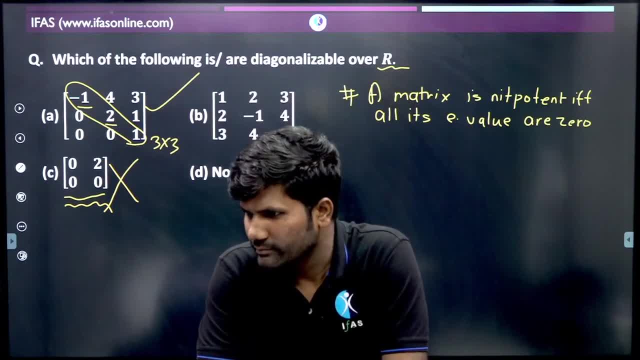 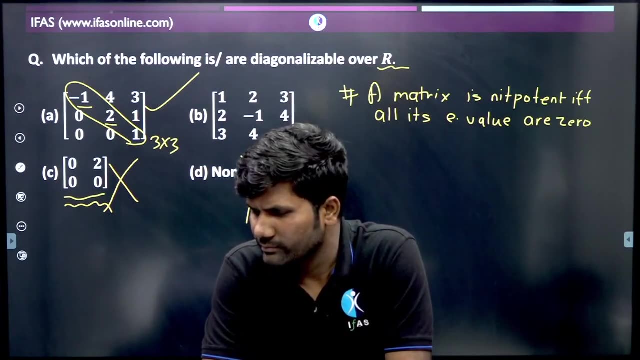 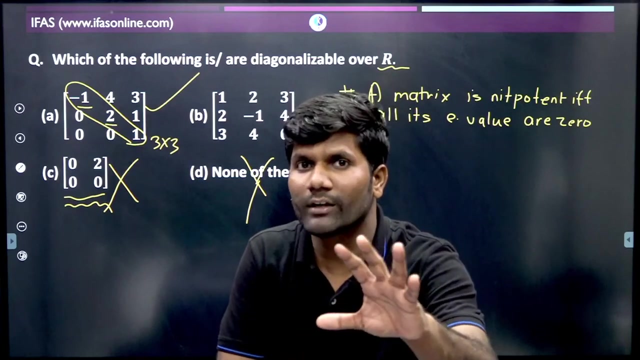 can you say about option b? absolutely very good. mayuri sujata is saying that i was preparing for pjt exam so paper is cancelled. which pjt sujata is explaining now. if, and only if, you give the matrix a nilpotent, it will be diagonalizable. 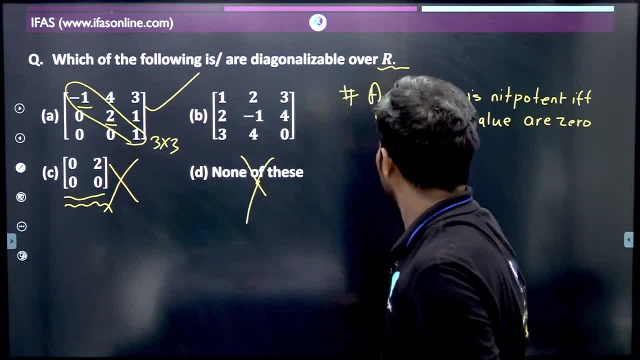 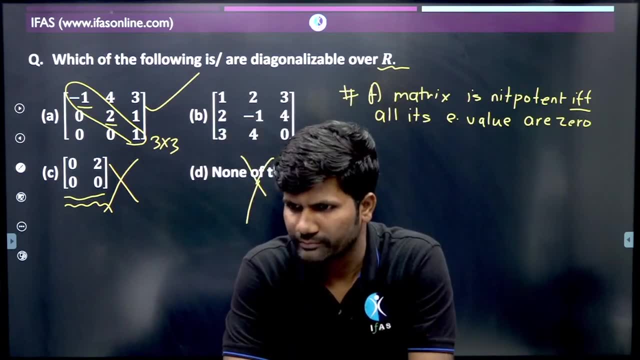 even if it is completely zero in a non-zero, nilpotent matrix, it will be not diagonalizable. okay, which abharti. which if and only if, yes, if and only if is there in the matrix. listen here, okay, yes, yes, absolutely. if any matrix is given, it will have all the eigenvalues. 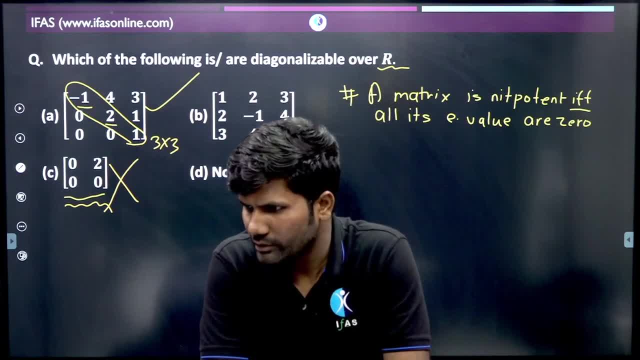 are zero, then it will be nilpotent. if it is nilpotent, then all eigenvalues will be zero. if, and only if, abharti right sujata, what was he telling you? which pjt sujata is explaining this? you see, this is the problem with nilpotent matrix. like the matrix is wrong, the matrix. 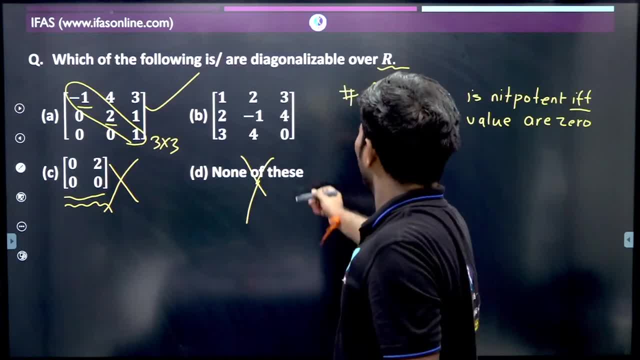 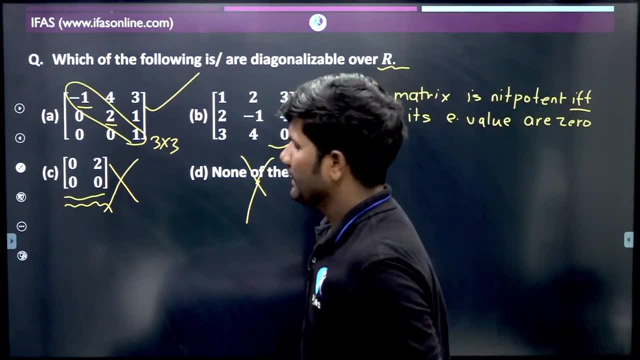 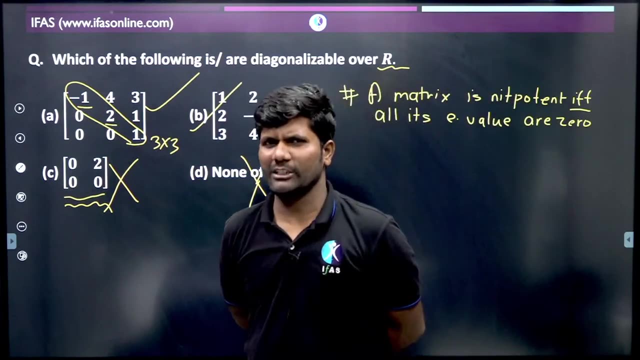 and if you see, this is symmetric matrix and there are real entries, so real symmetric matrix is always diagonalizable. this means option b is also correct. so here a and b are correct. but keep in mind, not net, not in Maharashtra state. msq does not come, mcq comes. only one option is correct. okay, but 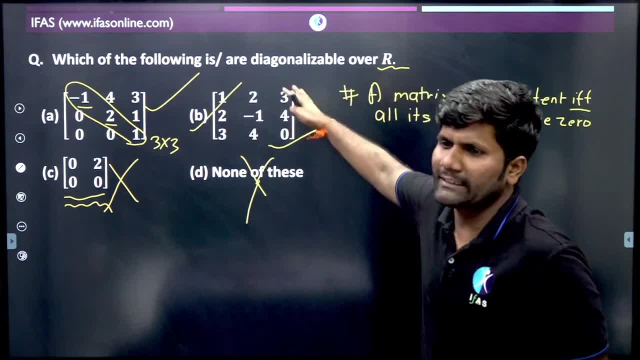 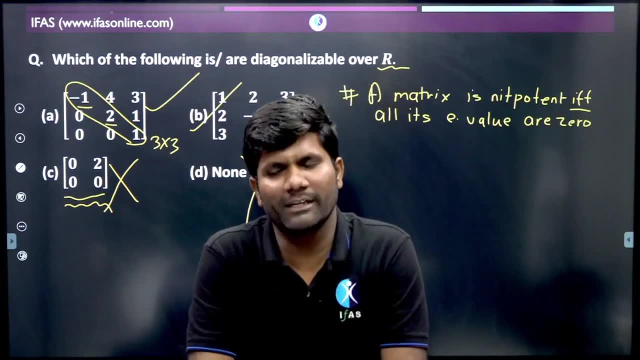 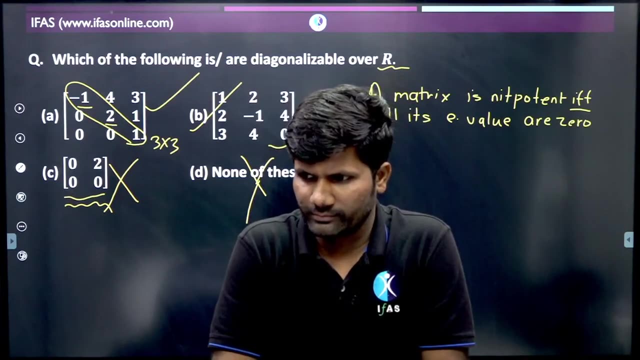 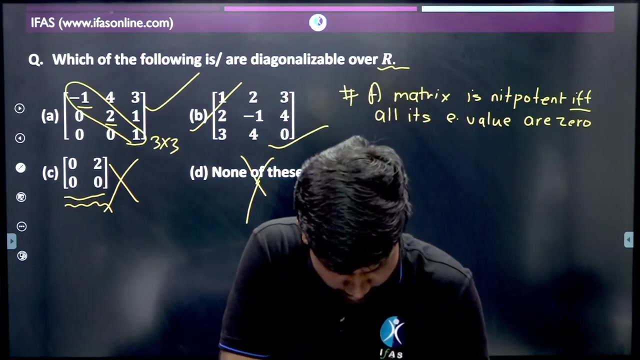 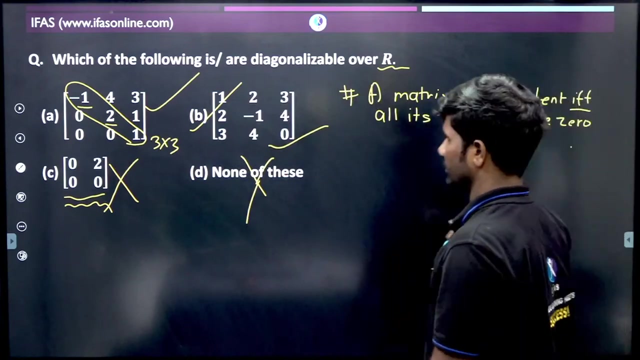 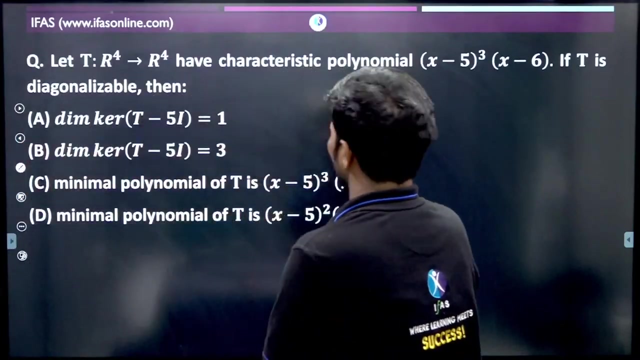 practice you guys. okay, all the students are clear till here. once you tell me let me go to the next slide, have you understood? all the students are clear. okay, remember, let's go to the next slide now. tell me what will happen. leti, for example. leti, for example. 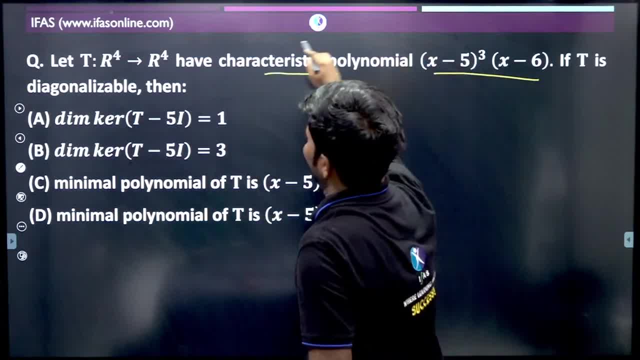 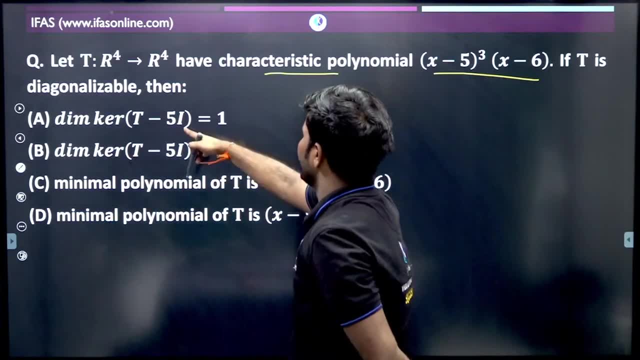 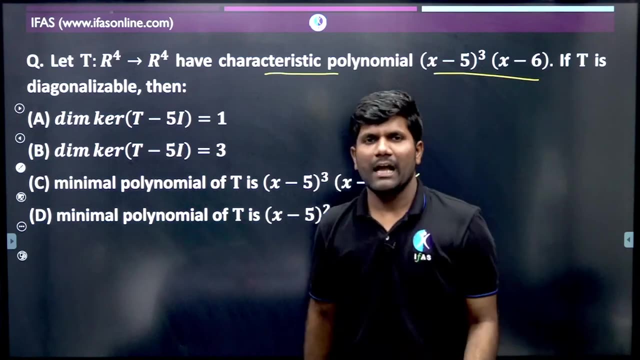 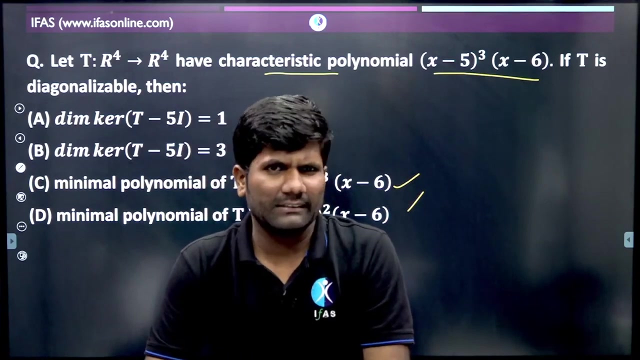 leti. for example, dimension of kernel t minus five is equal to one. dimension of kernel t minus five is equal to three minimal polynomial. Now you have to tell me which of these options will be correct. Chuleshwar Patel. CSIR NET exam. I think most of the chances will be in December. 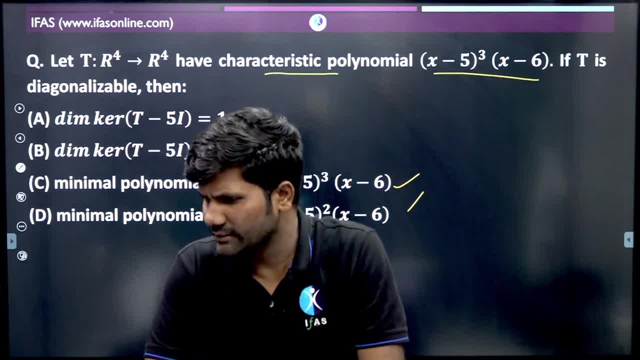 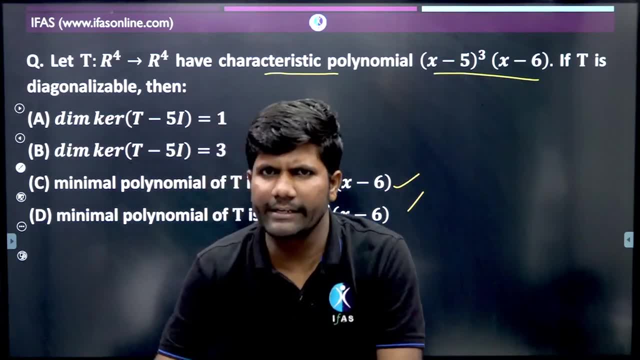 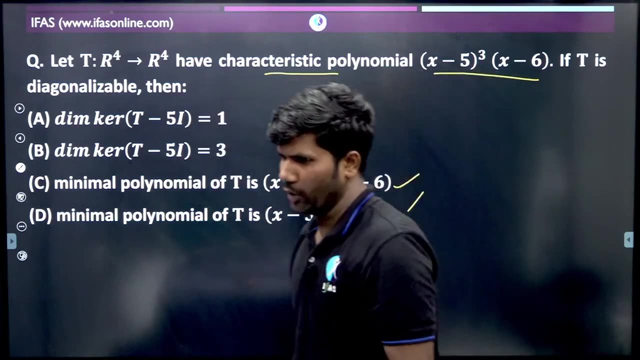 The form has not come yet. Most of the chances are there, Sachin, which exam has been cancelled? Maharashtra State has not been cancelled. It will be on time. It is not cancelled. How did you do, Nikita? You did it very quickly. 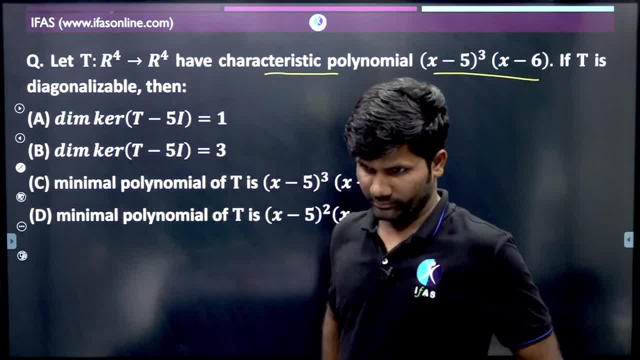 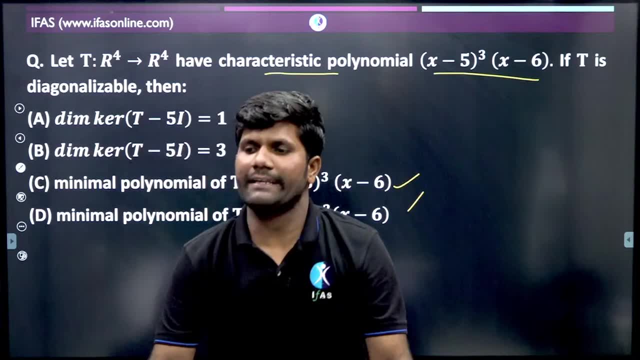 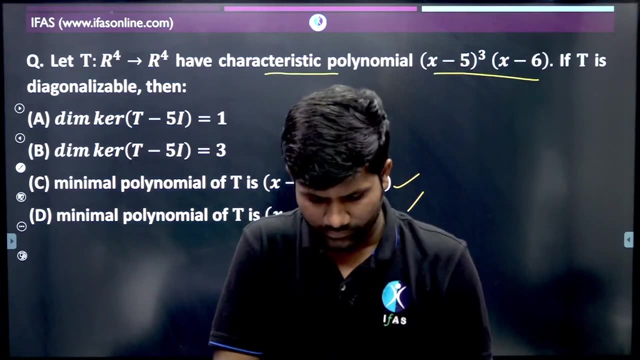 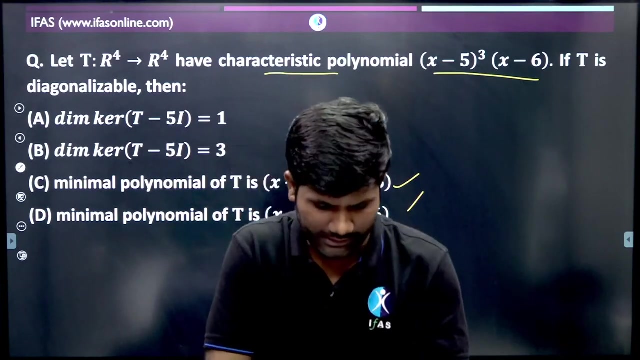 How did you do it? Yes, Dilip Vagmode B is asking: How did you do it? Tell me once I know how you did it. All students tell me how did you solve it. Sachin, tell me, are you ready or not? 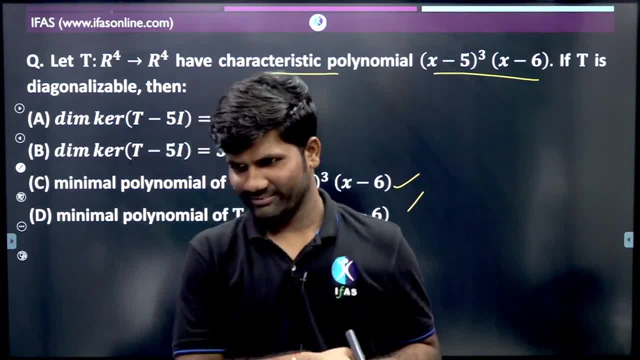 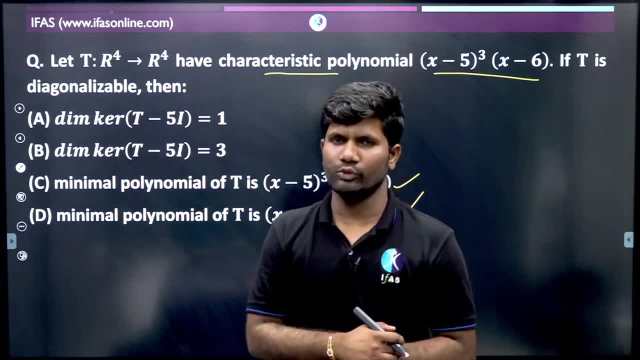 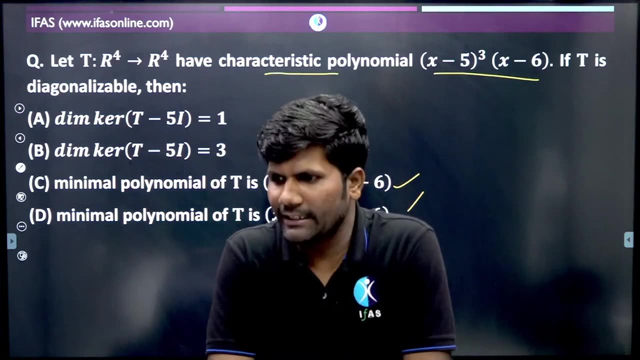 Sujata is asking: Don't take so much tension for the state. Keep the basic things clear. Don't do wrong to those who are coming. 99% of the chances will be there. Okay, If you are preparing for NET. 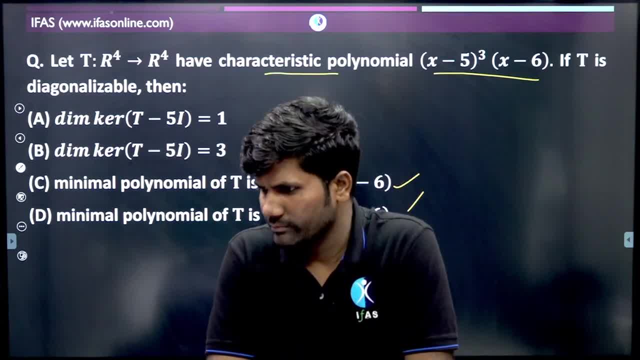 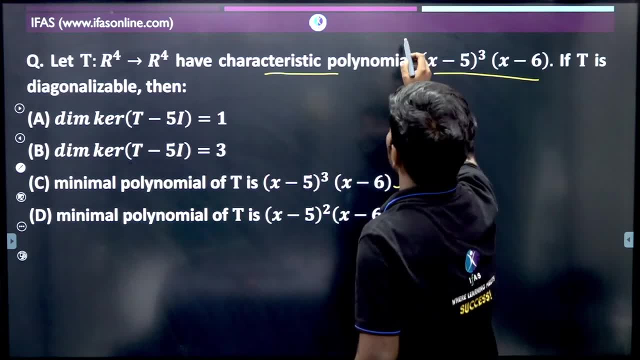 then Maharashtra State will be done easily. Okay, AMH request to GM. Okay, Tell me once, what have you given me? T from R4 to R4, characteristic polynomial AST T of X. And what is this? It is diagonalizable. 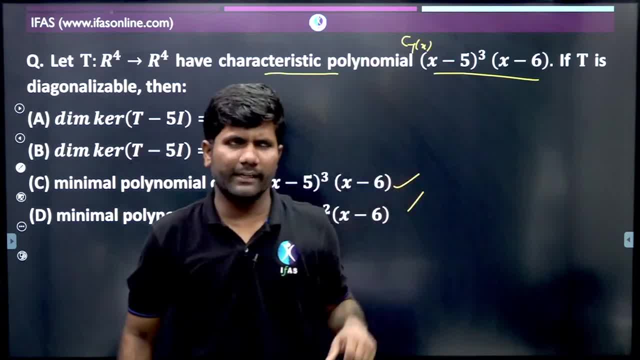 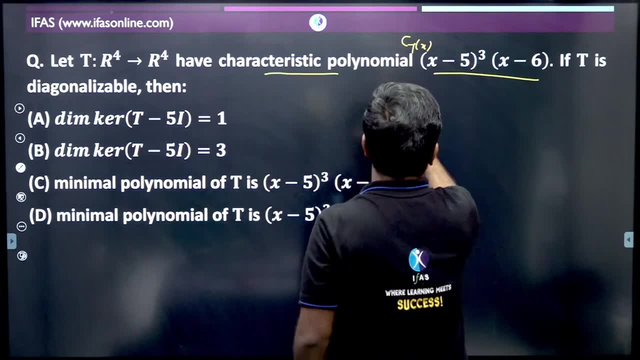 So we have done a result. You must remember what I said in the last slide: A matrix is diagonalizable if, and only if, its minimal polynomial is a product of non-repeated linear factor. What will be its minimal polynomial? Minimal polynomial is a product of. 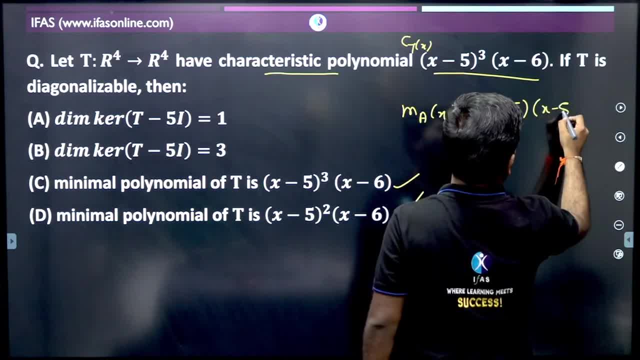 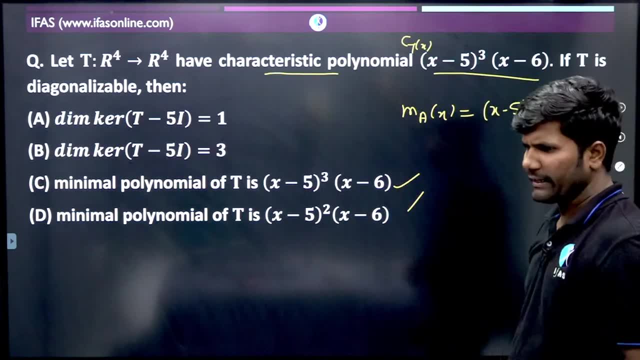 non-repeated linear factor. So this is the minimal polynomial. So this is the minimal polynomial. If it is a minimal polynomial, you have to do Jordan block further. If you write it in Jordan block, then look here: Phi is a block of minimal polynomial size. 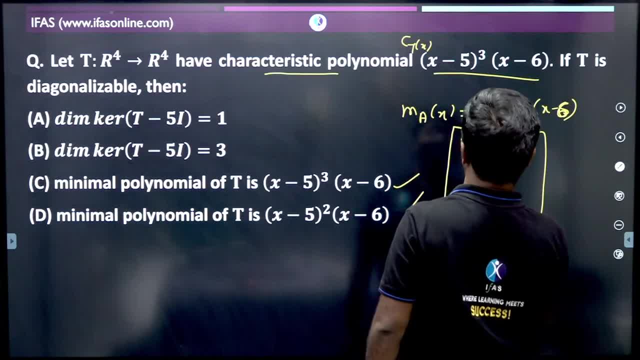 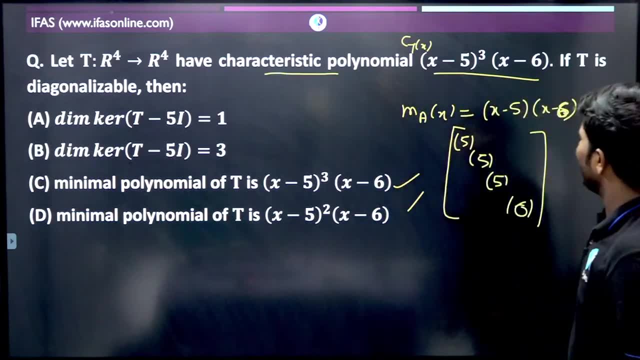 Phi is a block of minimal polynomial size Phi and 6. This type of block will be made here. Okay, See, these will be blocks. Let me tell you once: In minimal polynomial, the block for any number is its geometric multiplicity. 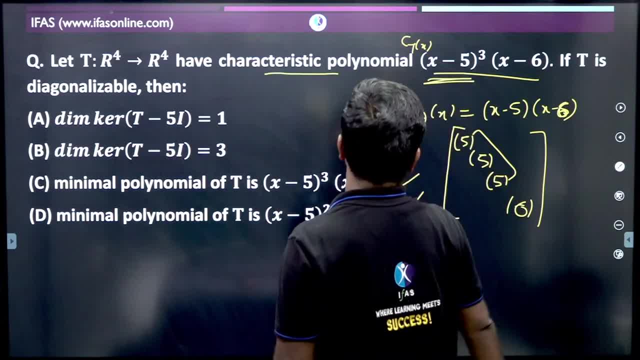 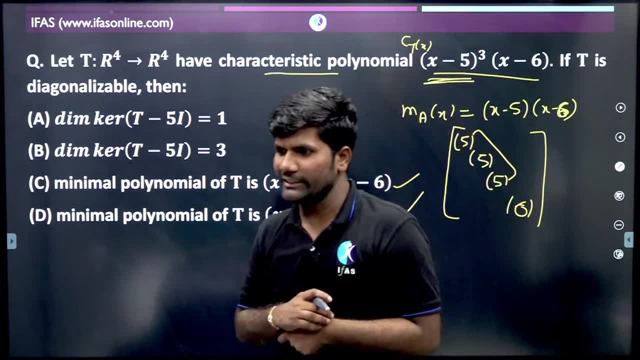 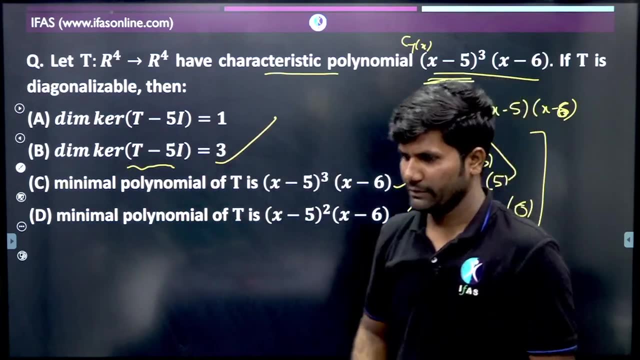 It means. what is its geometric multiplicity? What will be its geometric multiplicity? It will have geometric multiplicity 3.. And getting geometric multiplicity 3 means dimension. Dimension of kernel is 5 minus lambda is equal to 3.. So this option will be correct. 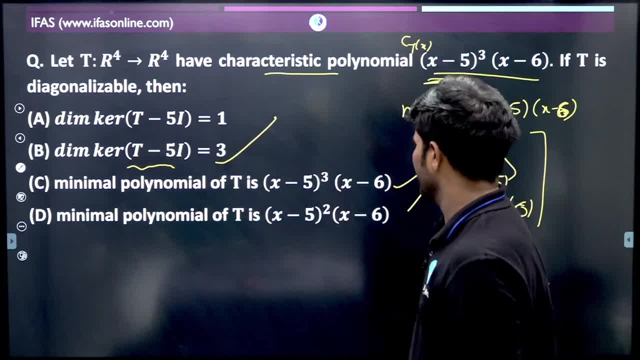 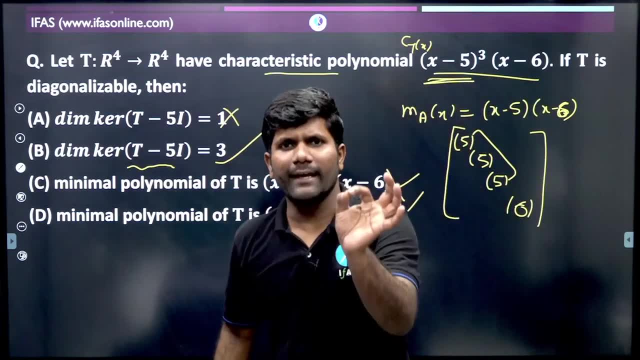 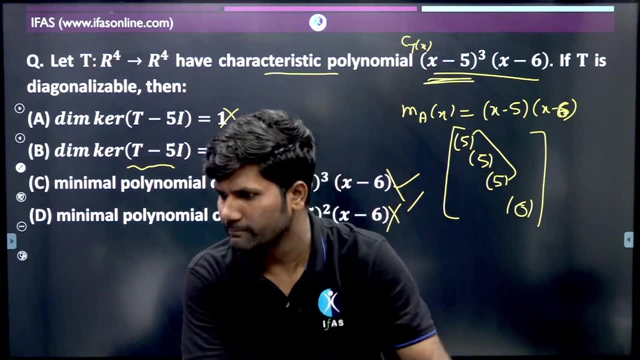 Okay, All students. it is clear. Minimal polynomial will be A. A option is finished, So here option B will be correct. Is it clear to everyone? Tell me once. If you have any doubts you can ask. Okay, Okay. 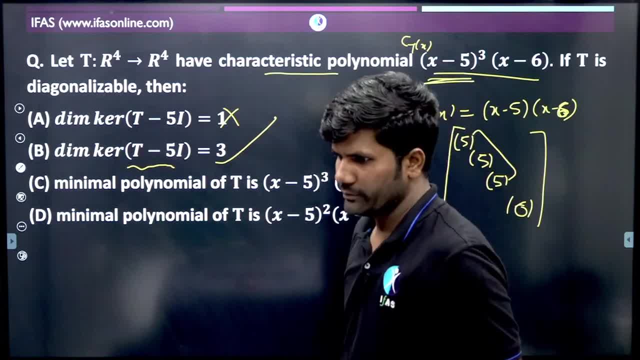 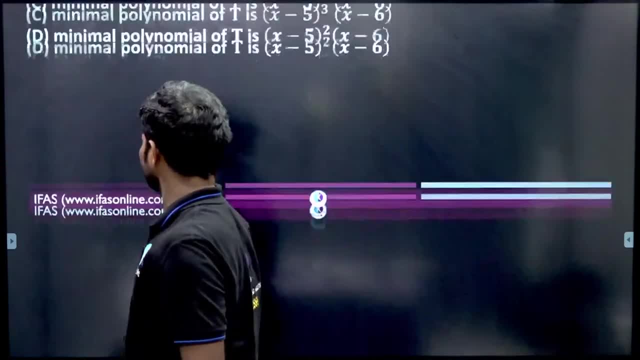 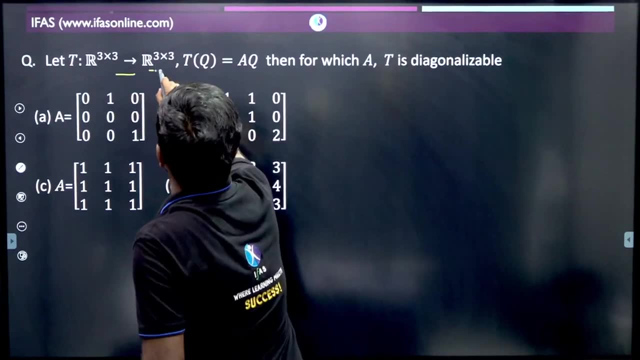 All students have given correct answers. Okay, Let's come to the next slide. So there are some more questions that are waiting for you. Now. we have to tell here that T from R3 to here is a map. T of Q, Then for which A? 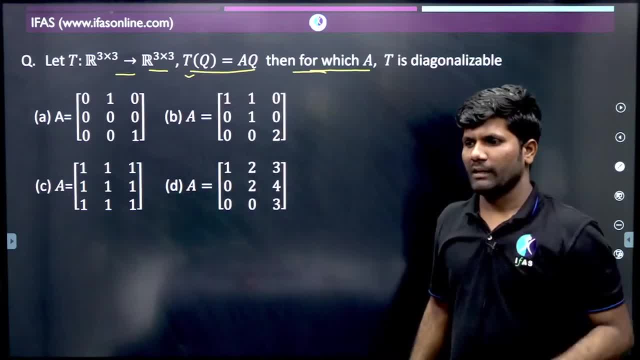 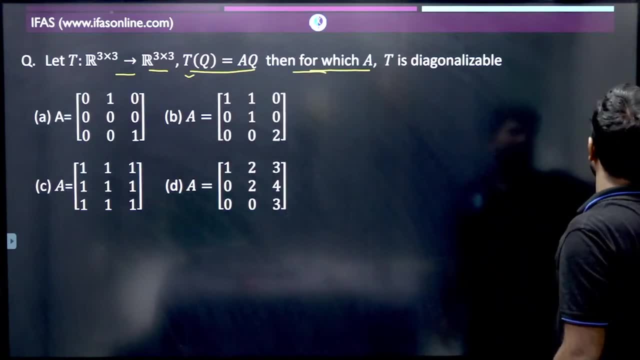 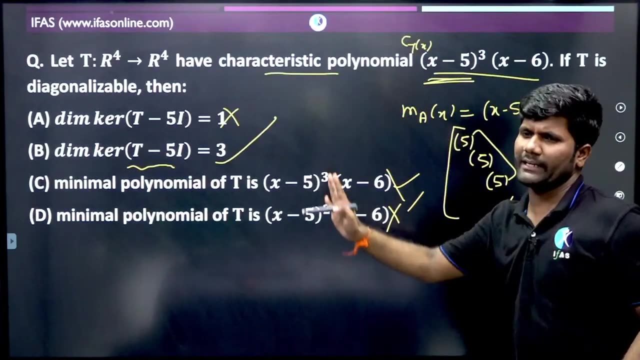 Now, for which value of A will T be diagonalizable? Now tell me which answer will be correct. So we had done one more question of this type. Bharati says, repeat it. Bharati actually tells: you See, in matrix, T is diagonalizable. 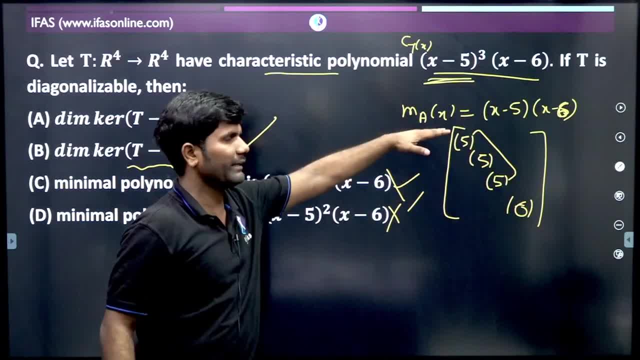 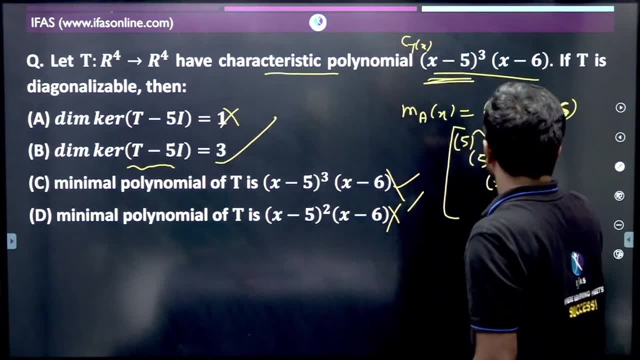 Means minimal polynomial is non-repeated. Minimal polynomial will be a product of non-repeated linear factor. So actually I used Jordan block in this. I used Jordan canonical form. Now see in minimal polynomial: how much is phi? The power of phi is 1.. 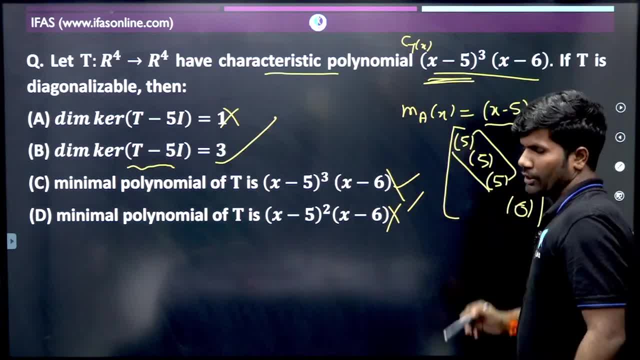 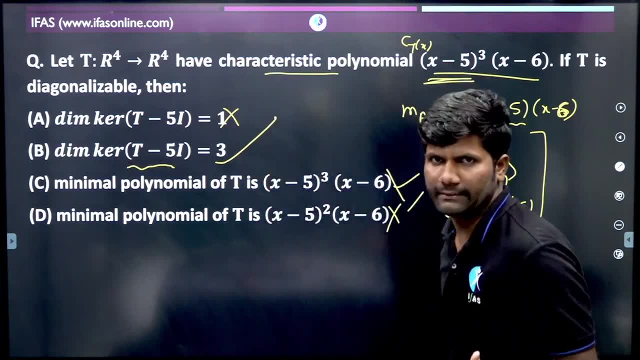 If phi is made in Jordan block then it will be 1 cross 1 block, So it has 3 blocks. So in any Jordan canonical form for any eigenvalue, blocks are made as much as its geometric multiplicity is. So it has 3 blocks for 5.. 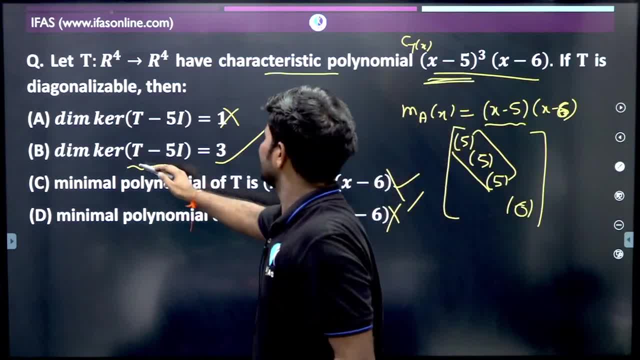 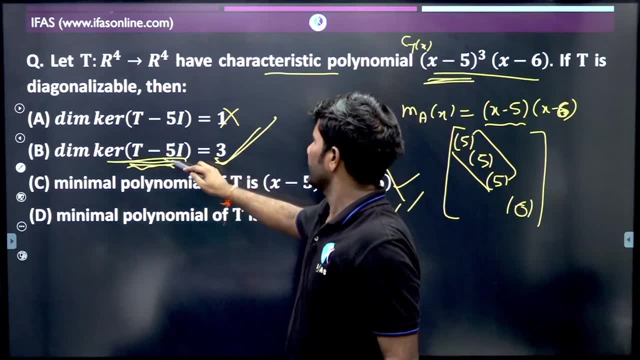 Means for lambda equals to 5,. its geometric multiplicity is 3.. And its dimension, which is called E lambda. its dimension is called geometric multiplicity. Means for lambda equals to 5, we will get 3 geometric multiplicity. 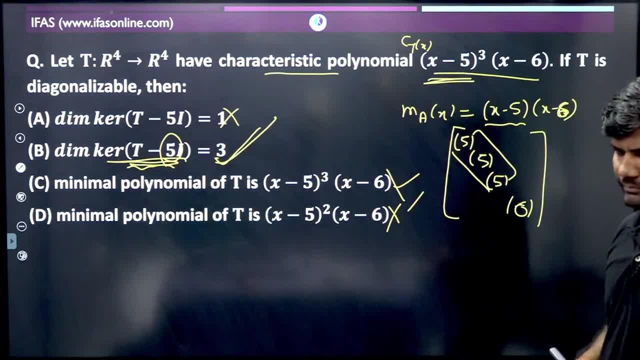 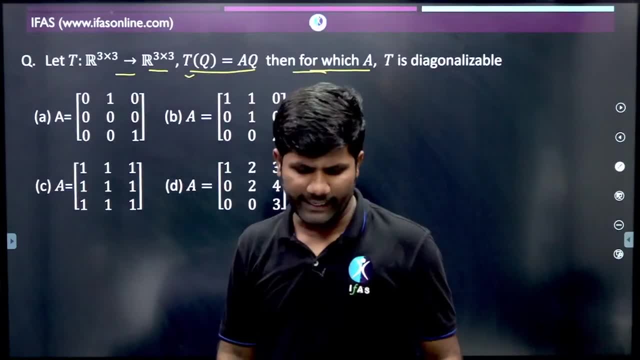 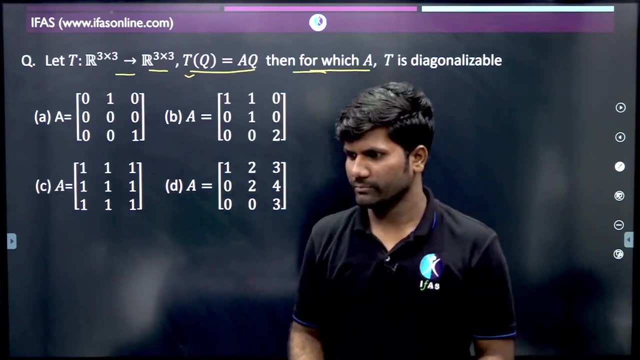 This is what we have done here. Bharati Nakpal. Let's come to the next slide. Solve this question now and tell us what is the correct answer. So all the students solve it quickly and tell us what is the correct answer for this question. 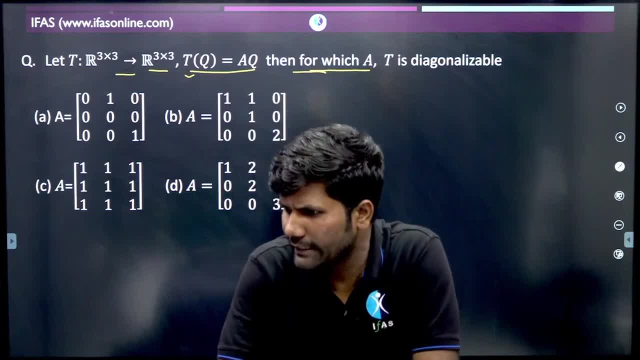 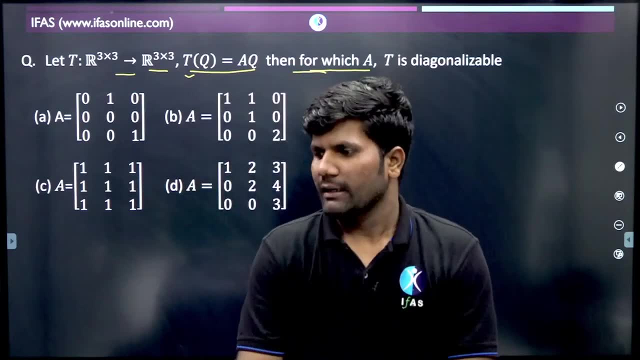 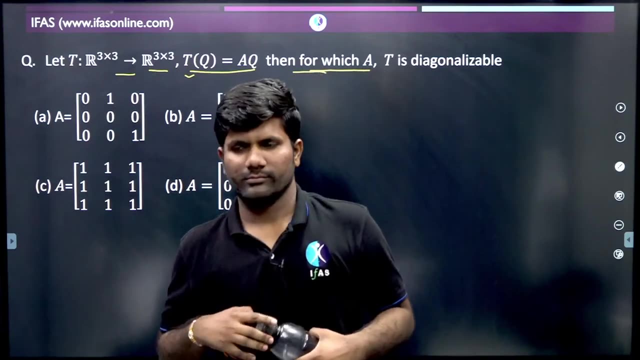 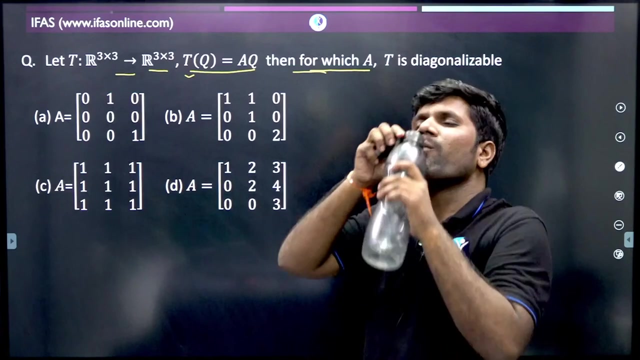 Tell me once. we will get only one answer For A, A, B, Karim. It will be 1.. Ok, Rest of the students. what is the answer? No one gave the rest. Forget the rest. Dili is saying it will be D. 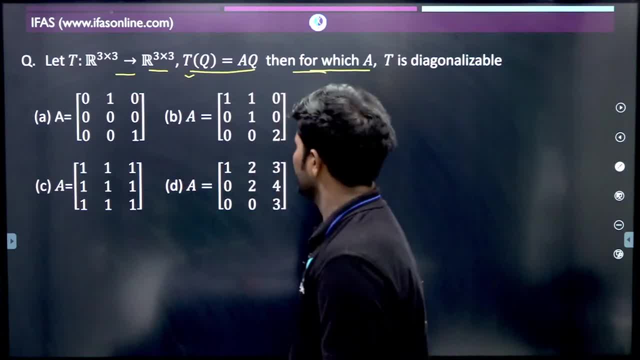 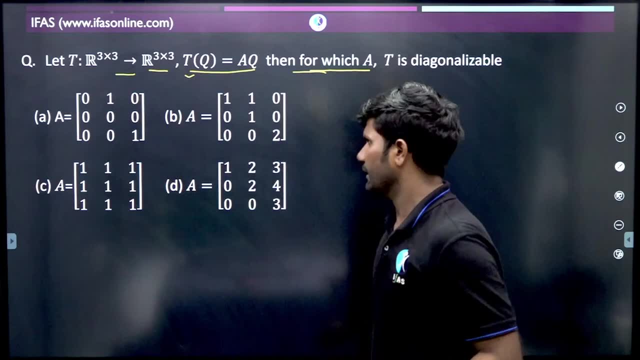 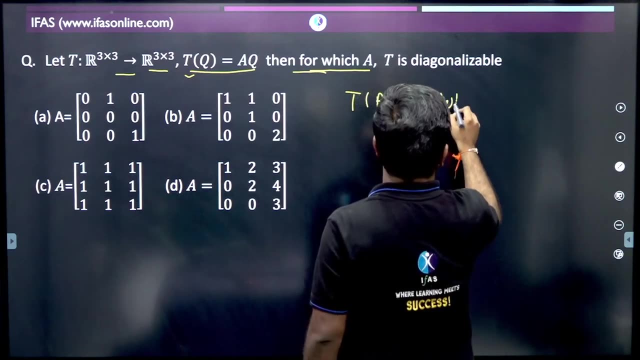 Ok, Tell me once For B A, B, Karim, It is 1.. Ok. Rest of the students. we will get only one answer. Dili is saying it will be D. Ok, Rest of the students. 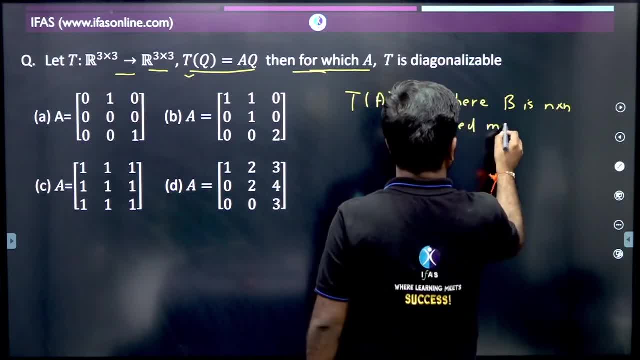 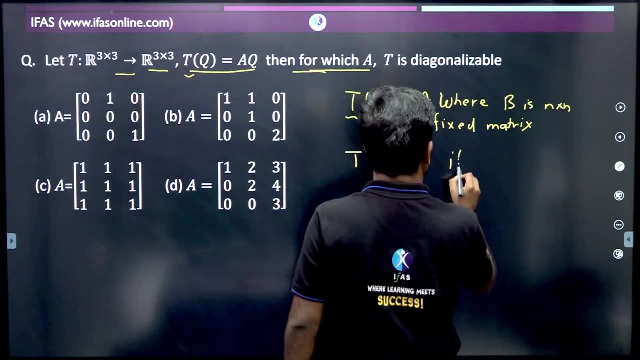 we will get only one answer. Dili is saying it will be D Ok. Rest of the students. we will get only one answer. Dili is saying it will be D Ok. Rest of the students. we will get only one answer. 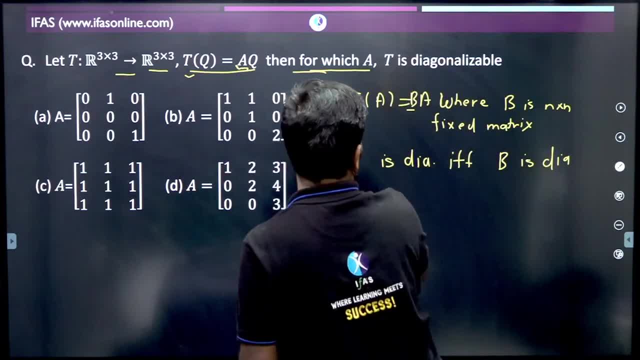 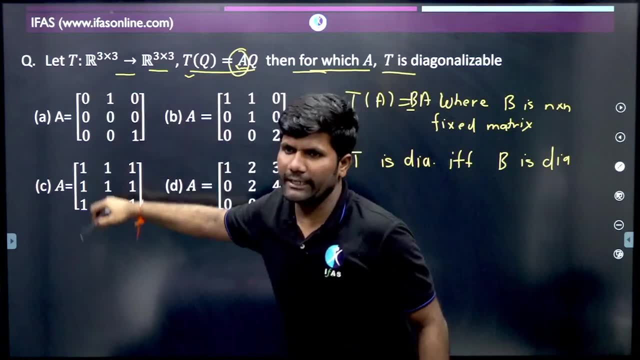 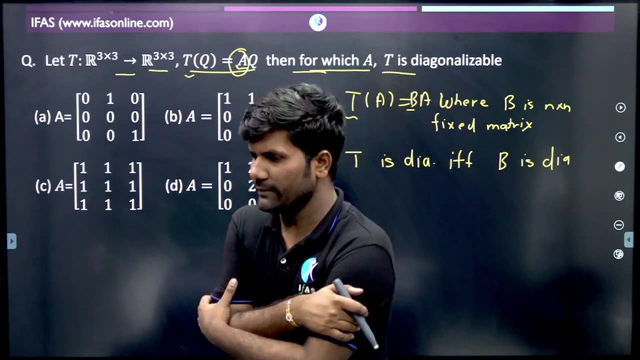 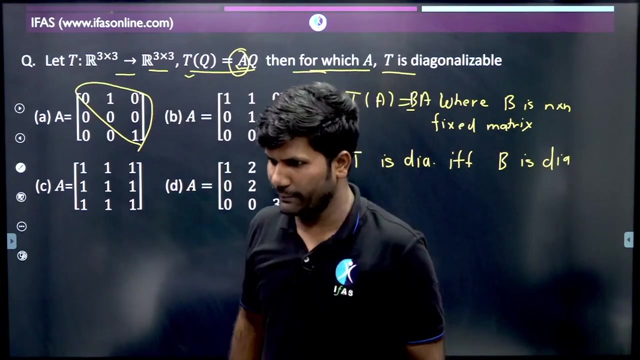 Dili. For R, it will be D. What is the answer? Rest of the students? we already got it. Yeah, for R, it will be D. idiot, Is your answer correct? what is the Truth? It is triangulisable. that's why it is diagonalisable. 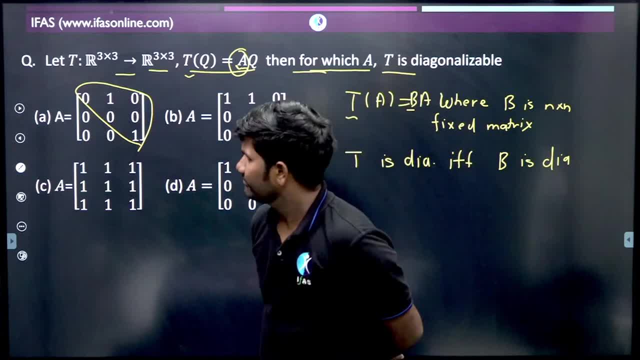 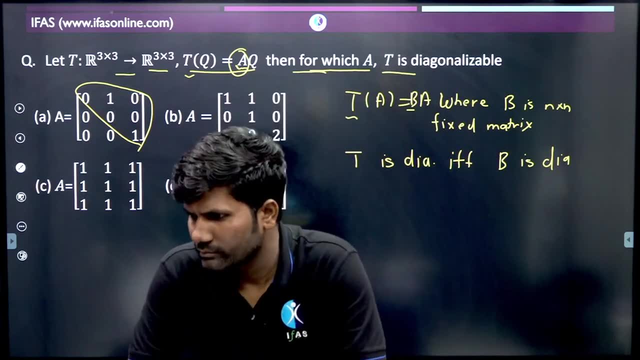 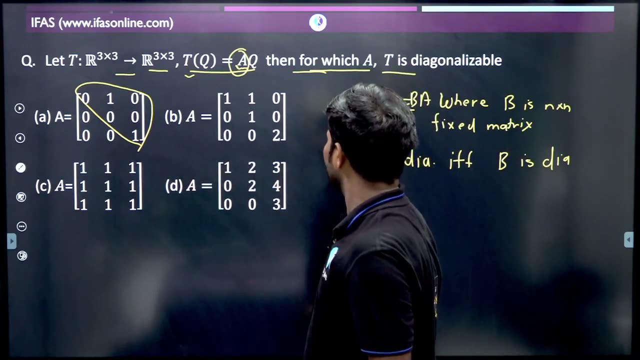 Is A diagonalisable or not? What can you say about option A? Is it diagonalisable? Absolutely, Bharti. Is A diagonalisable or not? Look is B or not. D is diagonalisable and constant matrix is also diagonalisable. C and D are. 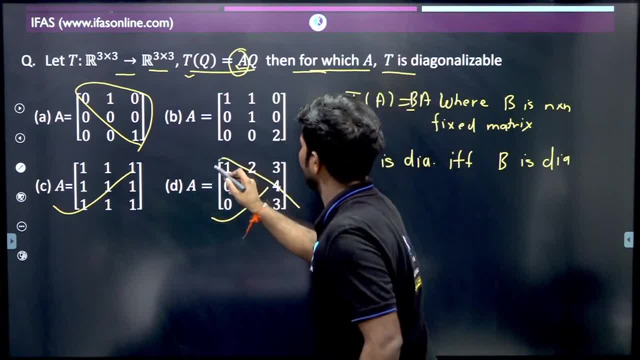 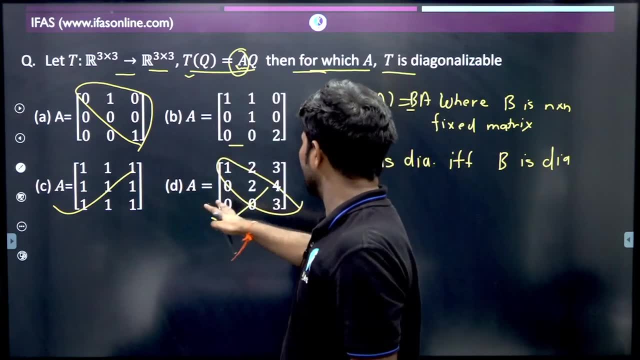 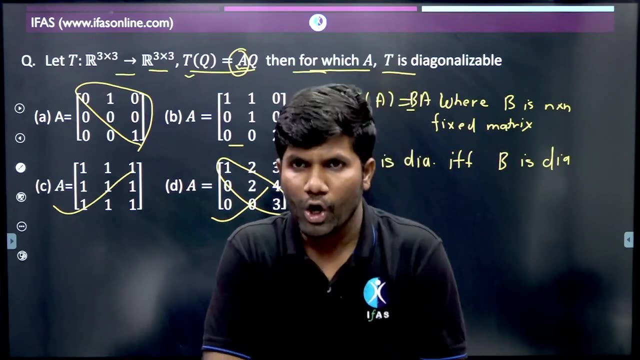 Look: constant matrix is diagonalisable. It has n distinct eigenvalues. These are also diagonalisable. Now we have to check these two. Is it diagonalisable or not? Means option C and D is correct. But what can we say about option A and B? So quickly solve it and tell us. 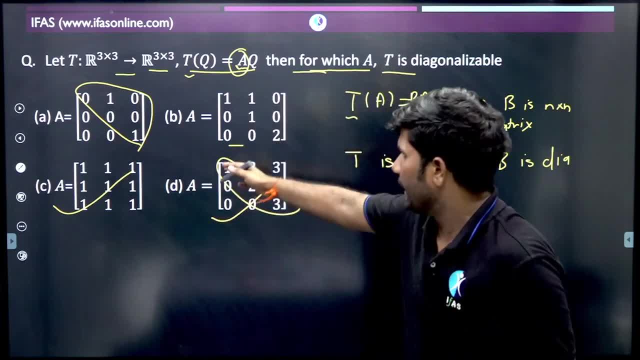 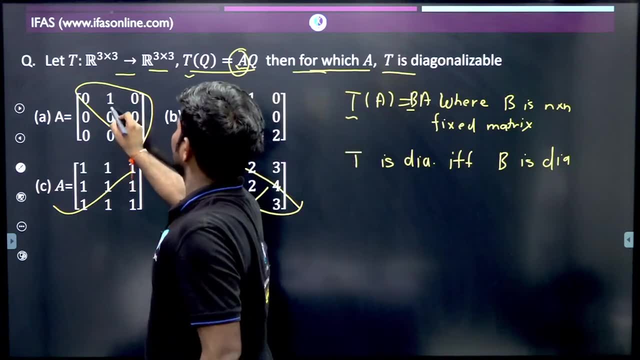 What can you say about option A and B? Is A diagonalisable? What do you think? Now check it. Now check its geometric multiplicity of zero. If you get 2, then it is algebraic 2. If you get 2, then it is diagonalisable. 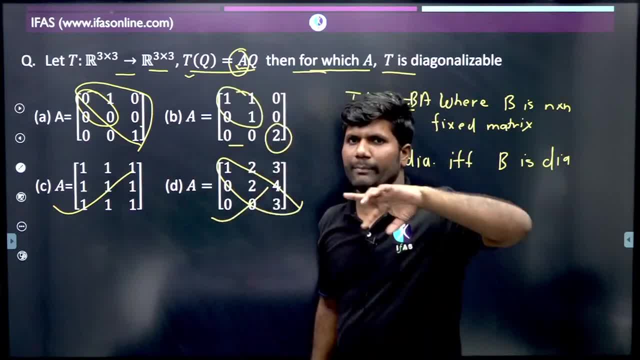 Now check the geometric multiplicity of 1. If you get 2, then it is algebraic 2. If you get 2, then it is diagonalisable. If you get 2, then it is diagonalisable. You have to check A and B. 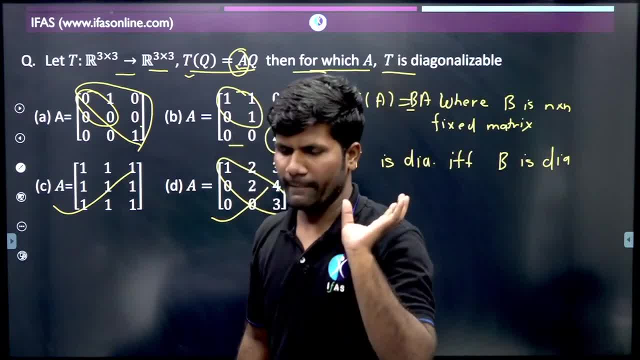 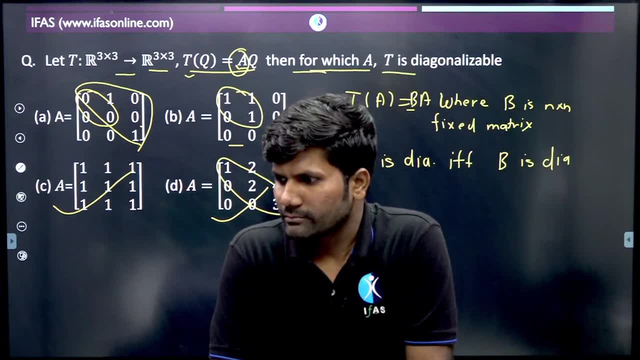 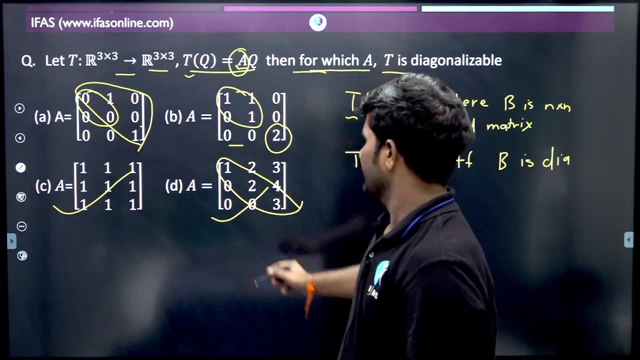 I have given you a hint. It is clear to everyone. If anyone has any doubt, you can ask All students. It is very impotent. It is not nilpotent. It has eigen value of 1. Matterち is nilpotent. All eigen values are 0. 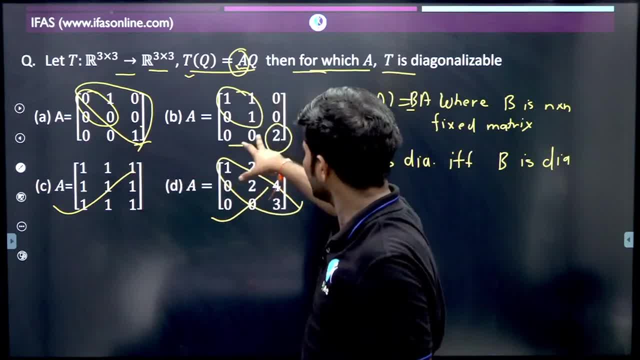 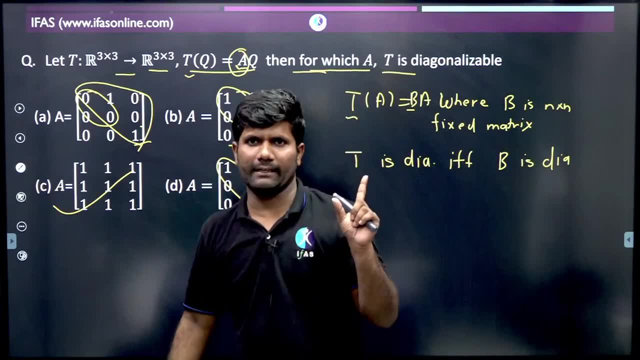 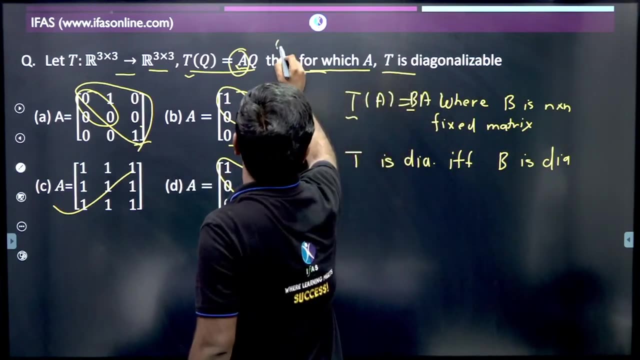 Ok, If there is 1's geometric multiplicity 2, Then it will be diagonalisable. Monica, You have to check option A and B. See here. Algebraic multiplicity of 1 is indeed 1. Very often, geometric multiplicity is Always less than or equal to. 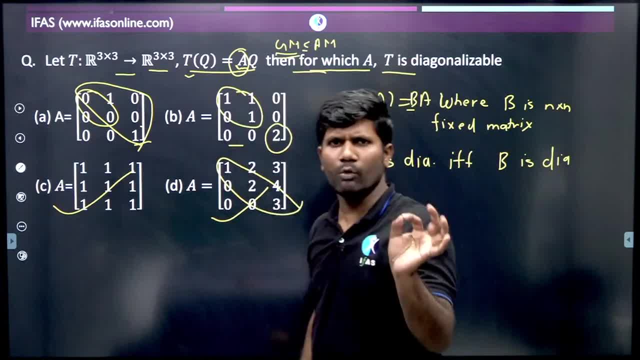 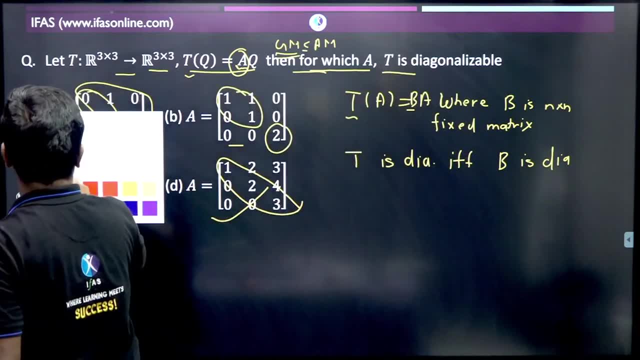 Algebraic multiplicity And geometric multiplicity is based onischen and equationalistGs. always 1 will be, at least now its algebraic multiplicity is 1, so it means geometric multiplicity will be 1. just to check who comes: 0 comes. 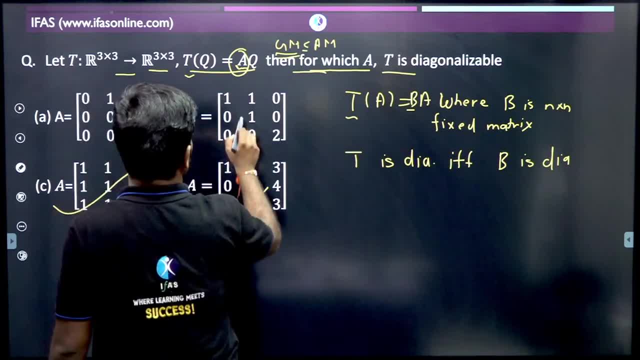 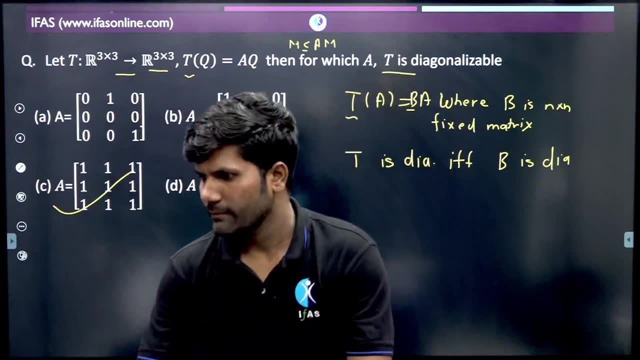 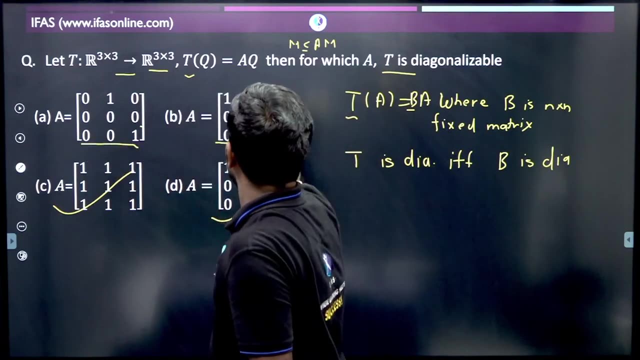 so here check 0 and here check 1 and tell what will be the correct answer. ok, is everyone clear? now I leave it on you. come on, bharati dilip. you have to check if A is diagonalizable, if option B is diagonalizable. 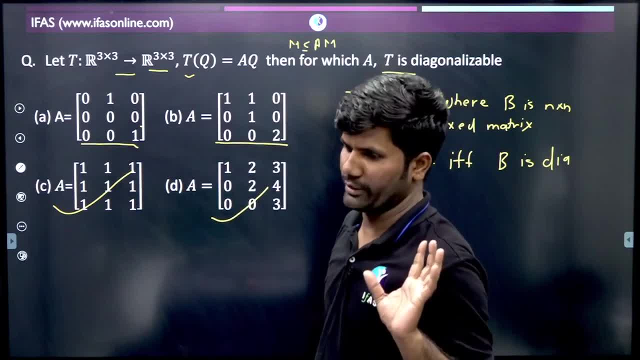 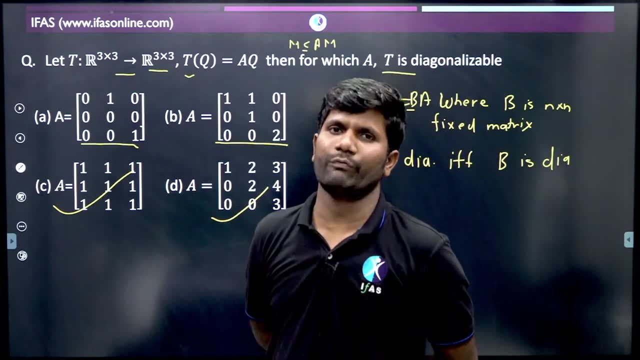 then A will also be correct. if A is not diagonalizable, then A will not be ok. you have to check this. what is the hint? A is same as G. check it. A matrix is directly diagonalizable if A is same as G for each eigenvalue. 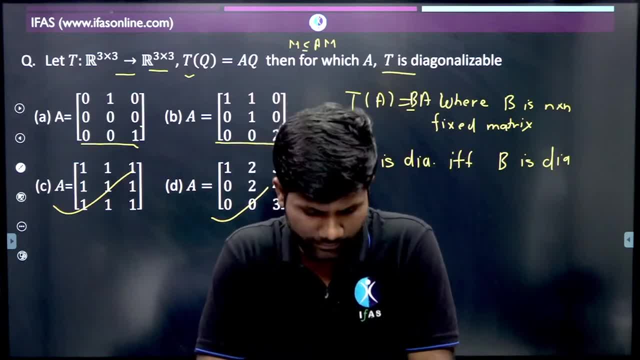 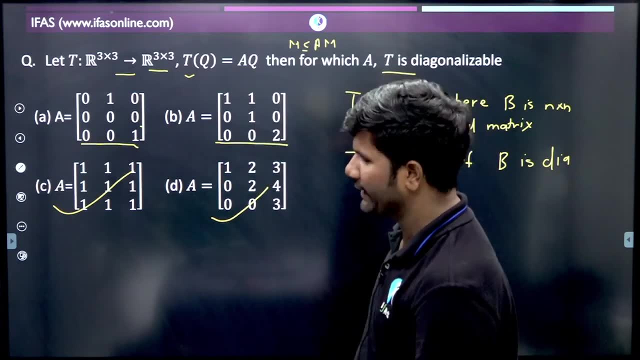 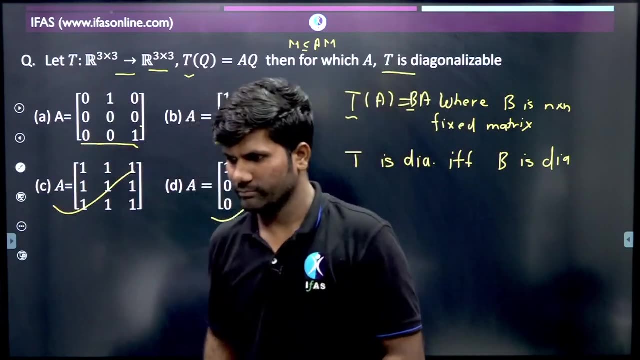 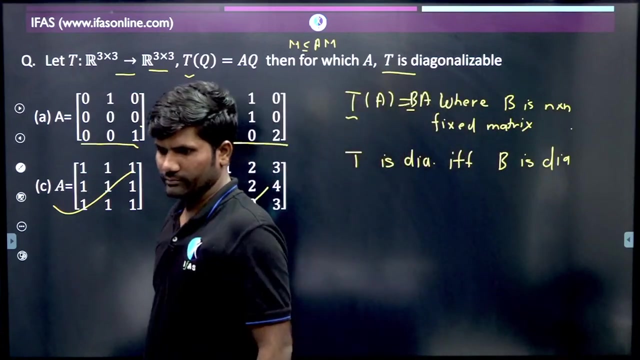 ok, is everyone clear? come on next. 0 has geometric multiplicity 1. if dilip 0 has geometric multiplicity 1, then it will not be diagonalizable. dilip, ok, you can mark it as it is now come on next slide. ok, bharati says A and B are not diagonalizable. 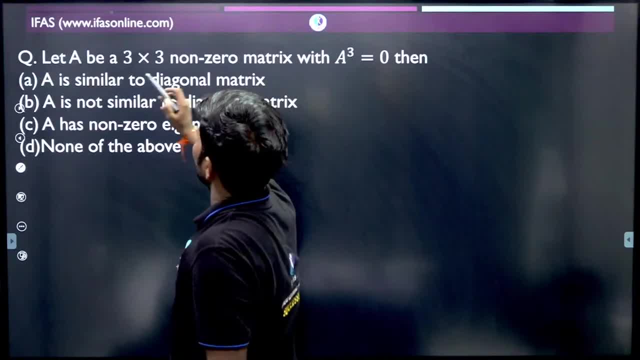 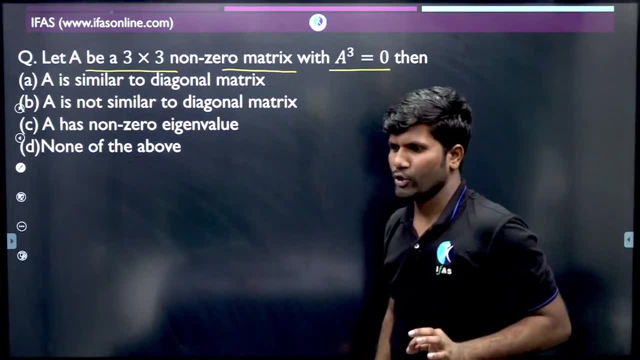 so you have to check and decide. ok, here we have given A, B are 3 cross 3 non-zero matrix and A cube is equal to 0. then now we have to select the correct one. so quickly solve it and tell what is it? Bharsali, what did we say? 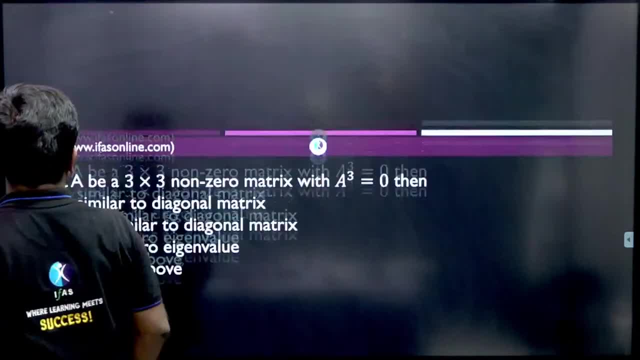 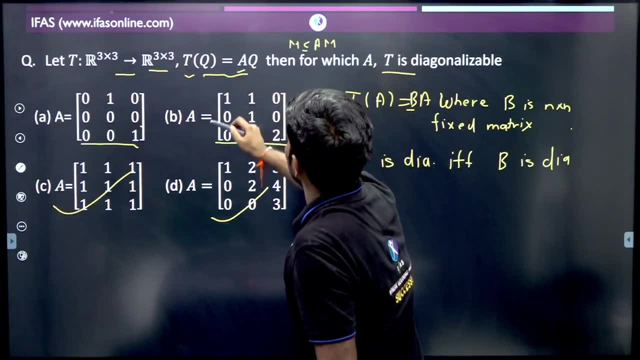 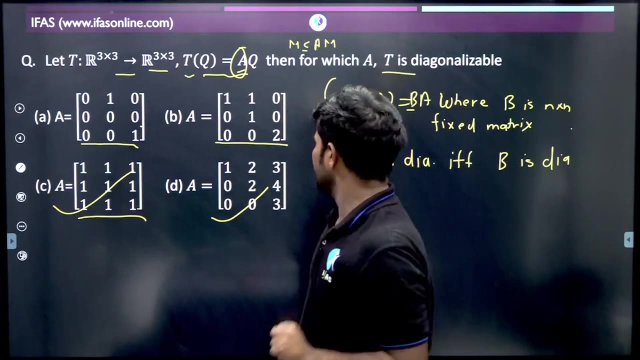 come on, let's tell Bharsali. once you do it, Bharsali, I said: look now, A will be diagonalizable only when A is diagonalizable because we have used this result here. ok, now, in this case, constant matrix is always diagonalizable. it has 3 distinct eigenvalues. 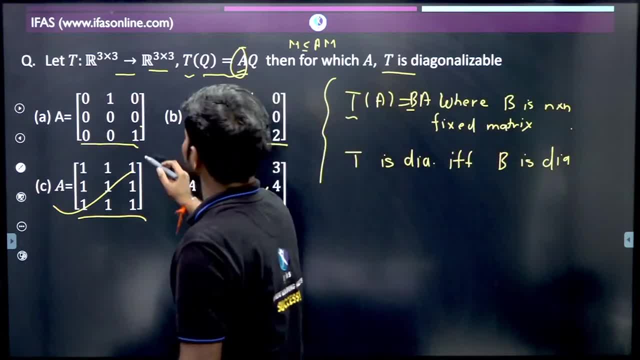 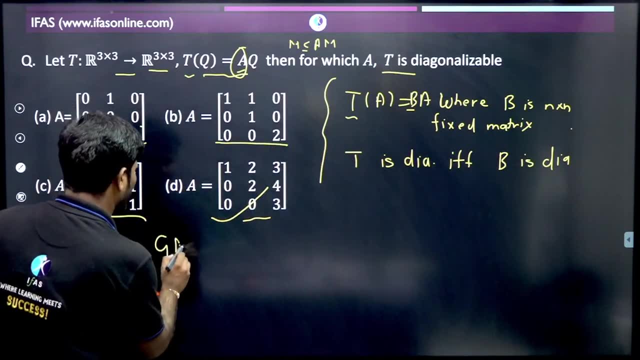 A is also diagonalizable. it means C and D are correct. now comes A and B. and how do we decide A and B? so we have a result. what does a result say? any matrix is diagonalizable only when, when, for every eigenvalue lambda, its algebraic multiplicity is equal to. 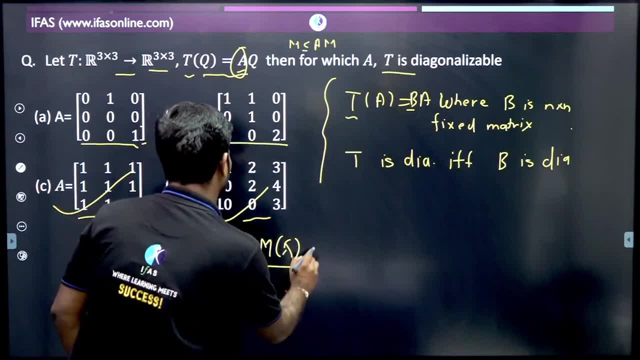 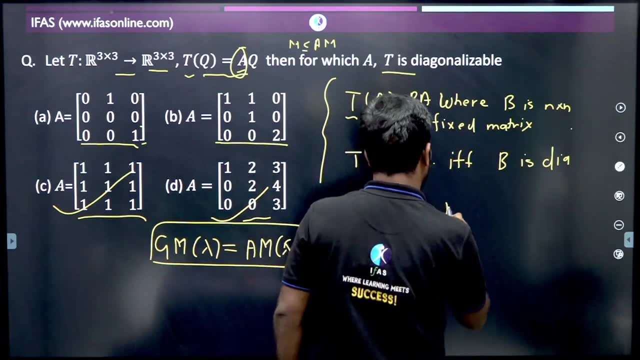 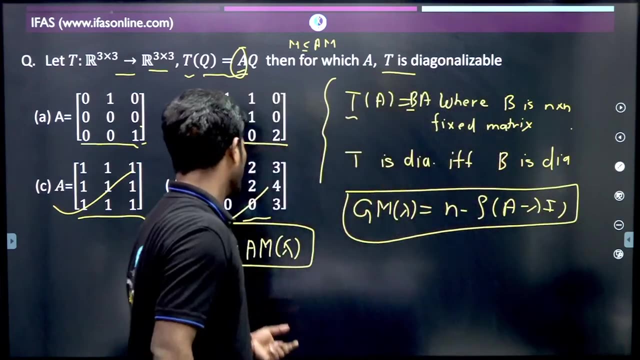 the geometric multiplicity. ok, use this result and you can decide. now comes the matter: how to find geometric multiplicity. so geometric multiplicity for lambda is equal to n minus rank of A minus lambda I. so what can you get from here? you can get geometric multiplicity. 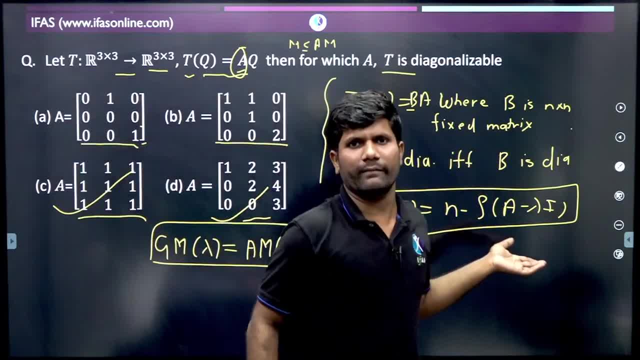 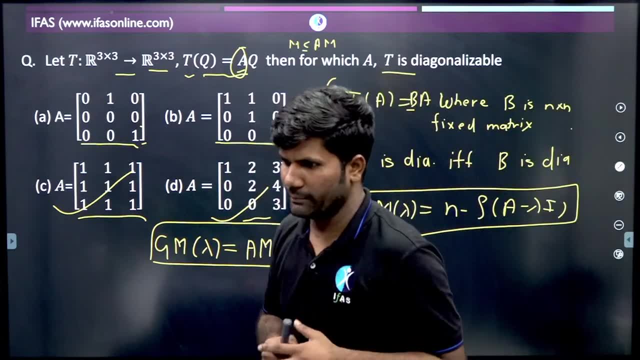 here: if the order of the matrix is n cross n, then in that case keep the value of n here. if it is 3 cross 3, then keep 3, 3 minus rank of A minus lambda R. ok, you just have to check that, Barsali. 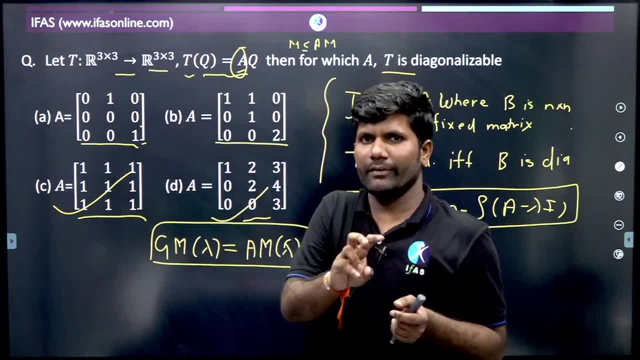 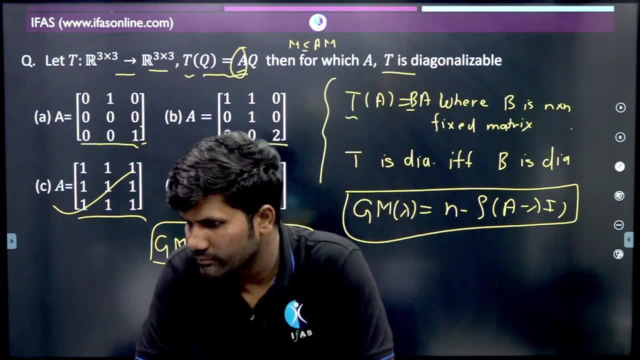 that eigenvalues, geometric multiplicity. for every eigenvalue, algebraic multiplicity, geometric multiplicity is equal or not. if it is equal, then it is diagonalizable, if not, then it is not. ok. done, Barsali, it has been repeated. did you understand? ok, what did you do? 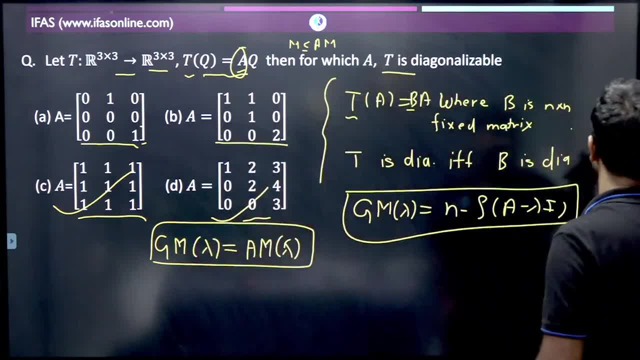 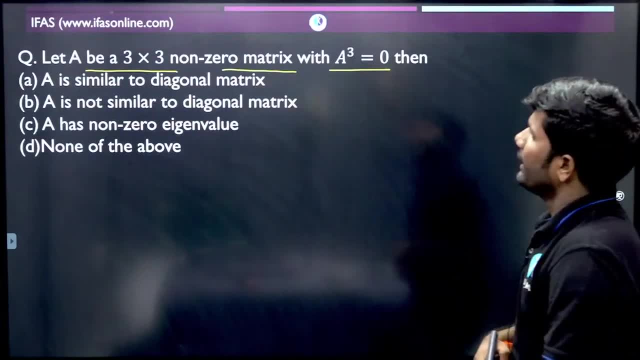 you deleted the comment. ok, you did B. ok, let's come to the next slide. now here we have to tell which one will be correct. what is given here? A, B, this is 3, cross, 3, non zero matrix. and what is A cube? it is zero. 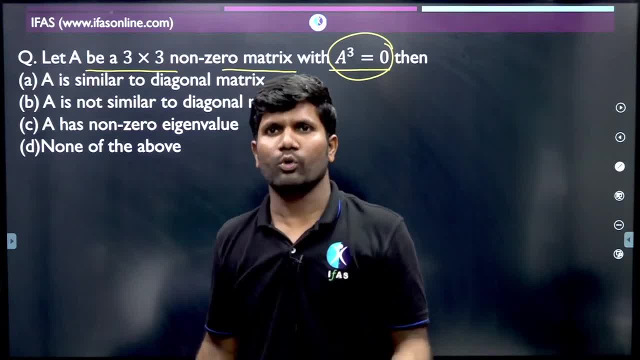 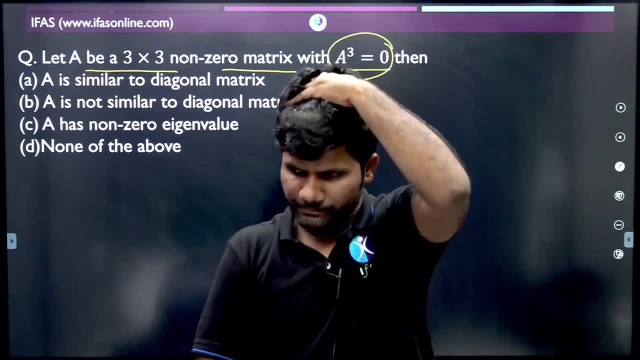 what is the meaning of A cube being zero? what do you think if A cube is zero, what will be the meaning of this? tell me what will be the meaning of A cube being zero. A, B, Kareem, Anshul, Chaudhary, Barsali, Dilip. 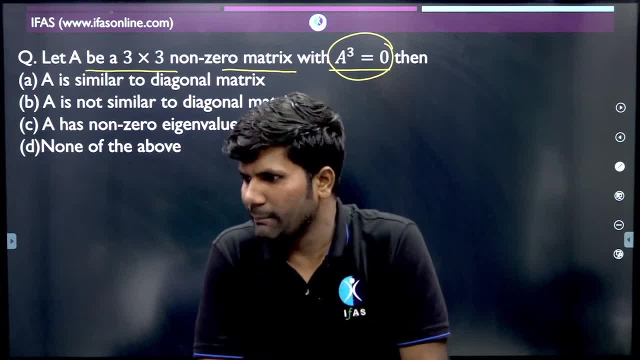 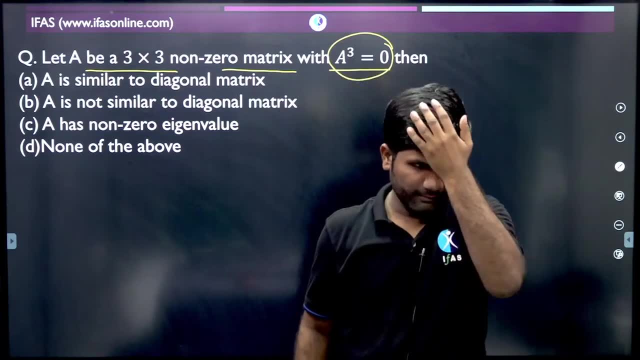 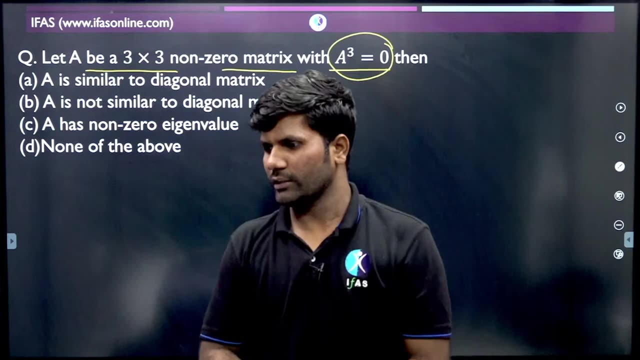 Lalitha, Pratik, Sheetal, Shyama, Monika, A, B, Kareem, what do you think? tell me Bharati Nagpal is saying B and C? ok, come on, Barsali is clear. ok, come on. now tell me. what kind of matrix is this? 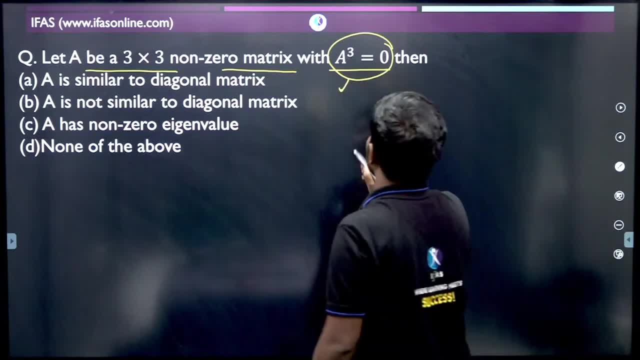 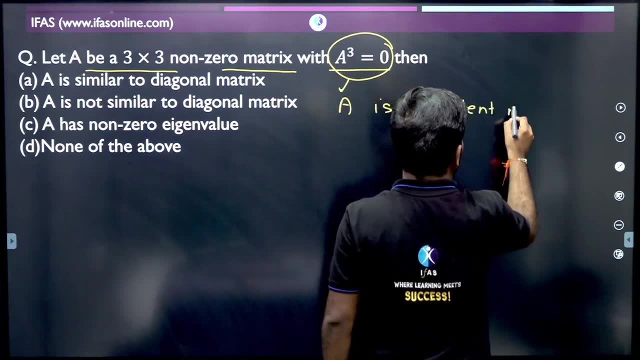 A cube is equal to zero. it means that A is nilpotent matrix. so what can we say here? A is nilpotent matrix. what is this? it is nilpotent matrix. but observe one thing carefully: what 3 cross 3? non zero nilpotent matrix. 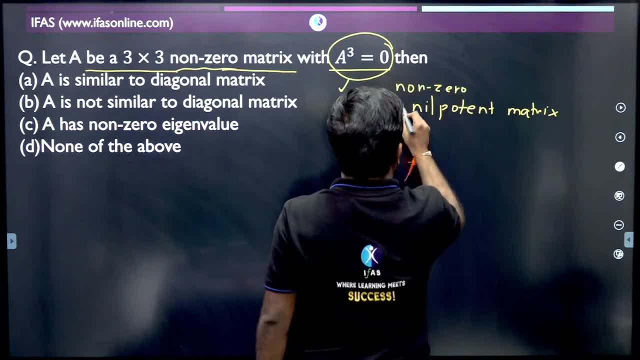 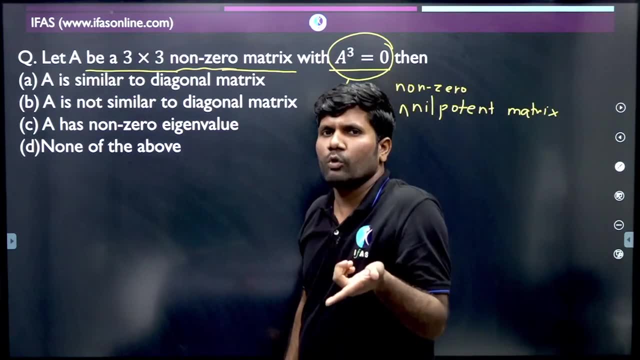 it means that analyzes non zero nilpotent matrix. if it is non zero nilpotent matrix, then what we saw- any nilpotent matrix will be diagonizable only if it is zero. but but what is this non zero matrix? it means it won't be. 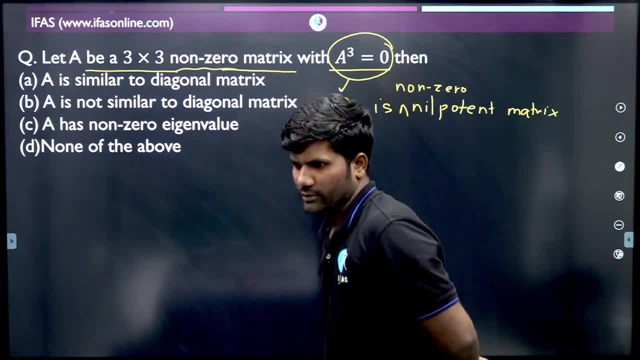 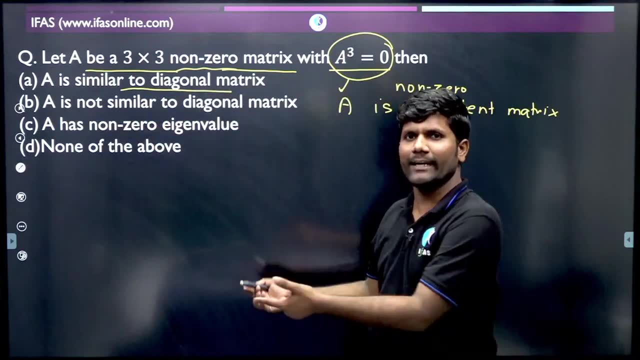 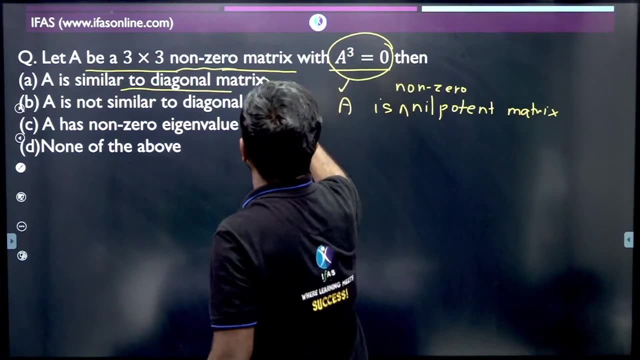 diagonalizable right, is it clear? so what is here is similar to diagonal matrix. it means that A is diagonalizable, which is incorrect. why? because A is non zero nilpotent matrix and non zero nilpotent matrix is never diagonalizable. so first option is incorrect. option b is, given that a is not a diagonal matrix, similar. 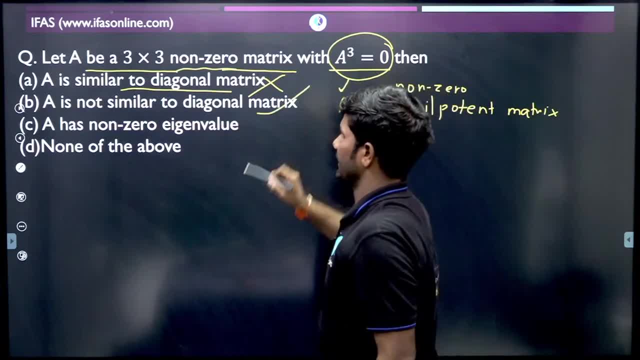 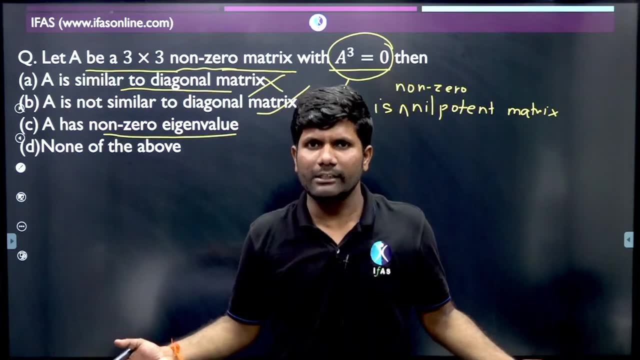 to that. it means that a is not diagonalizable. this means a is correct. after that, what is said here? a has non-zero eigenvalues. tell me once: a matrix is nilpotent matrix if, and only if, all its eigenvalues are zero. but here what is being said? that it is nilpotent matrix and its eigenvalues are zero. 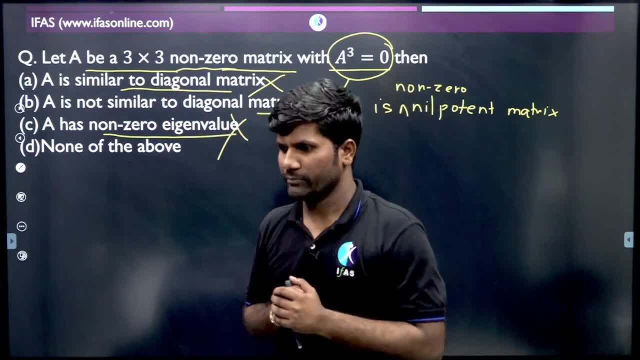 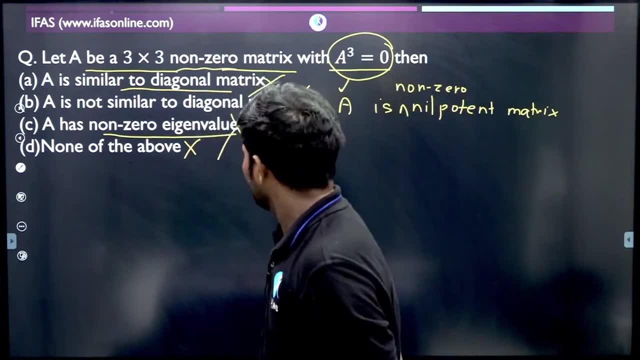 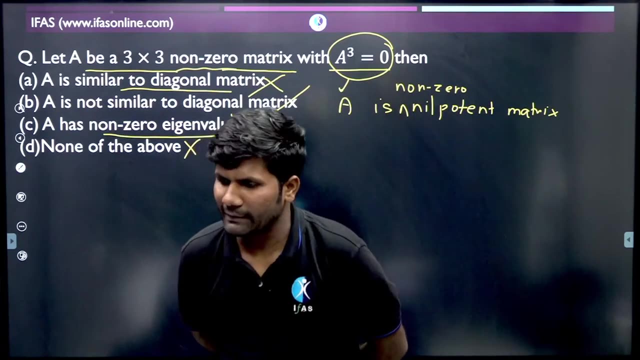 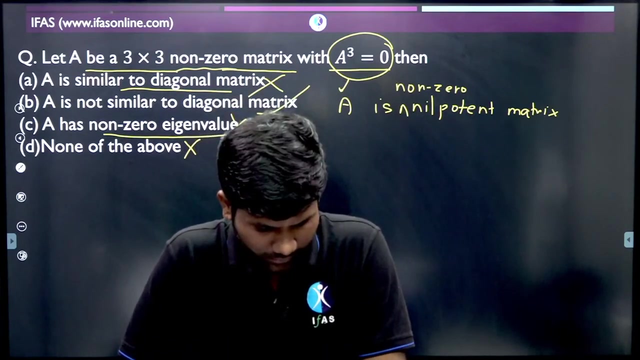 which is a very big wrong thing. so last option is incorrect. this means that what will be correct here, b will be correct. tell me one thing, chuleshwar patel. how did you tell me c? how did you tell chuleshwar that it will be c? how did you do that? you got the correct answer, c. 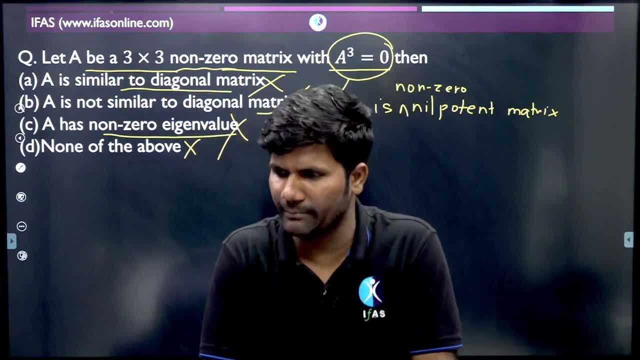 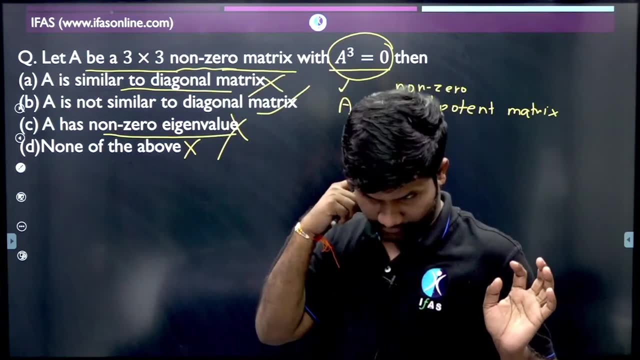 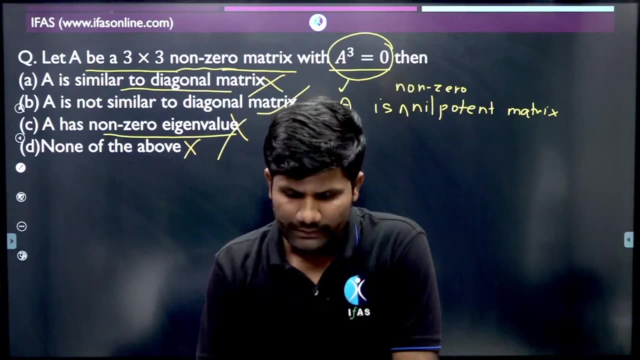 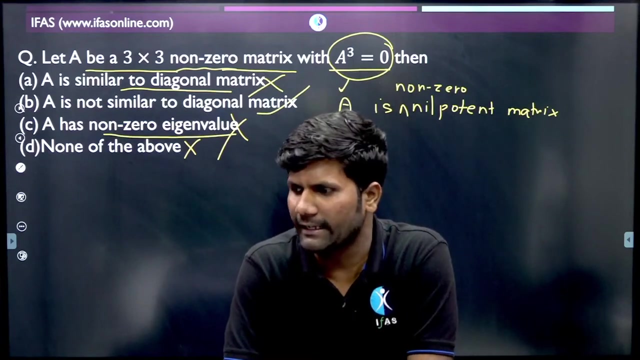 bharati is also saying, bharsali is also saying: ganesh thackeray is also very good. and anyone else has any doubt? is it clear? all the students are clear. see, a comment has been made on the side of ifs math. if you want more such live sessions, 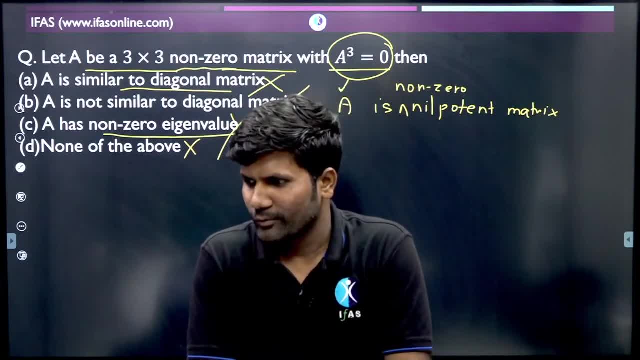 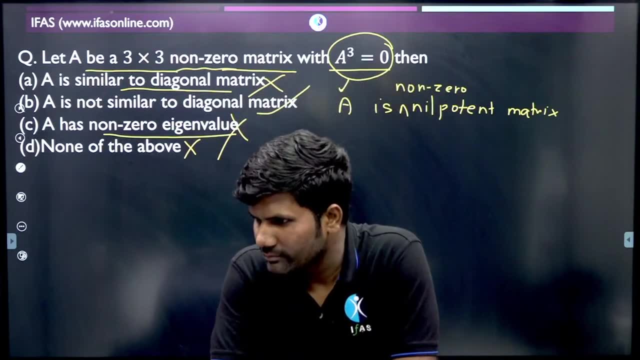 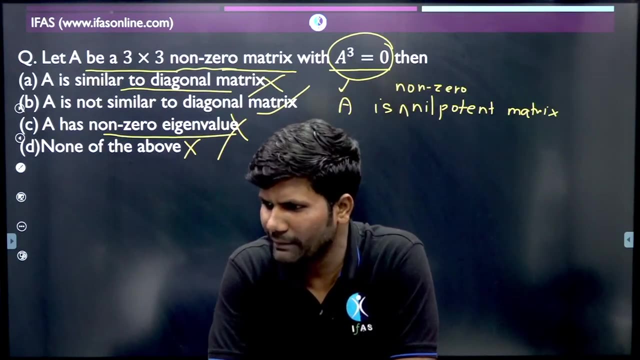 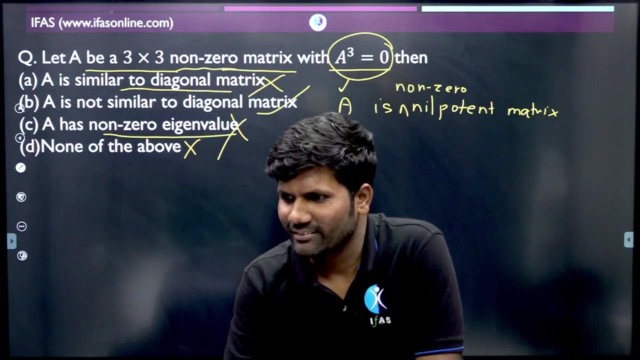 then first of all, like see in the comment, want more live session? hit the like button. okay, lalitha pavar, which one is yours? please upload my pyq. which one, lalitha, when did you do? yes, lalitha, tell me once, when did you do pyq which we? 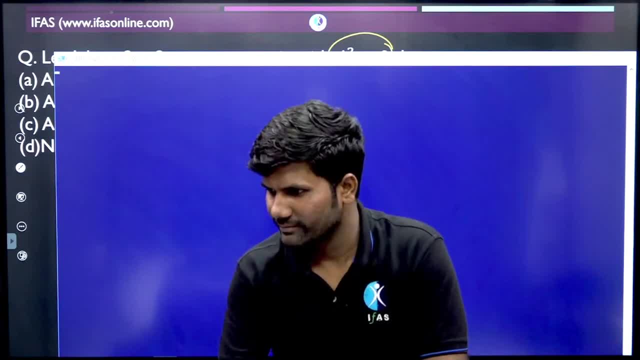 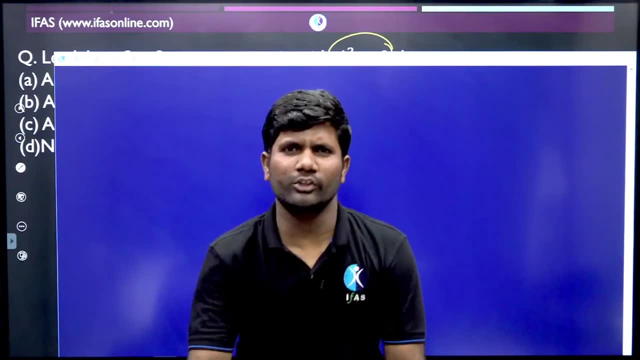 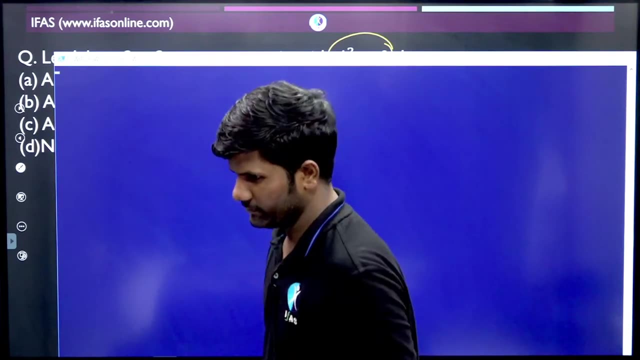 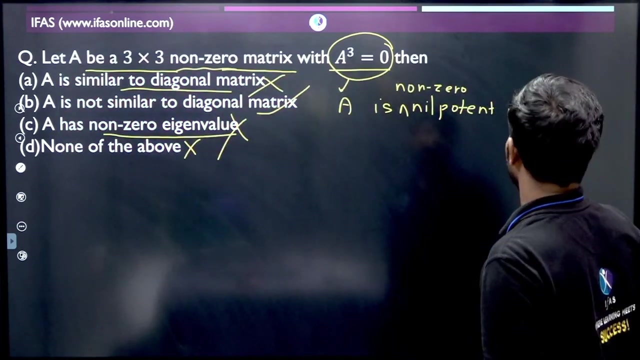 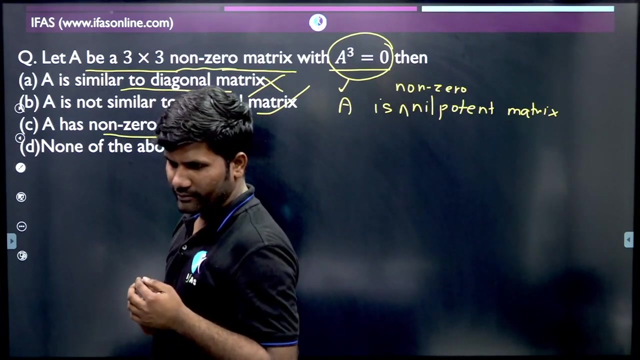 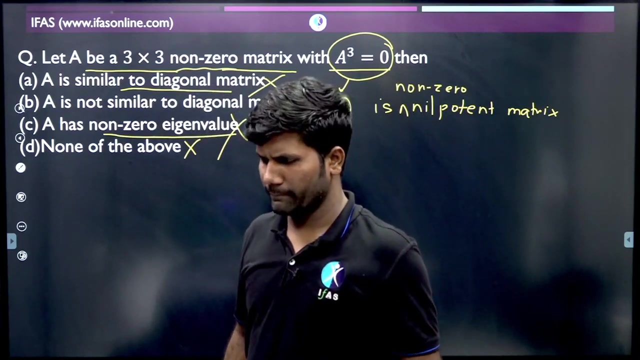 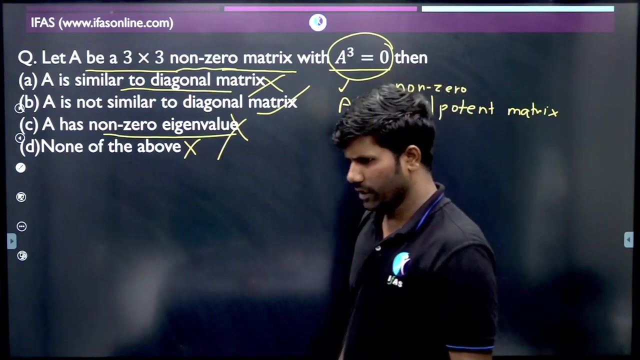 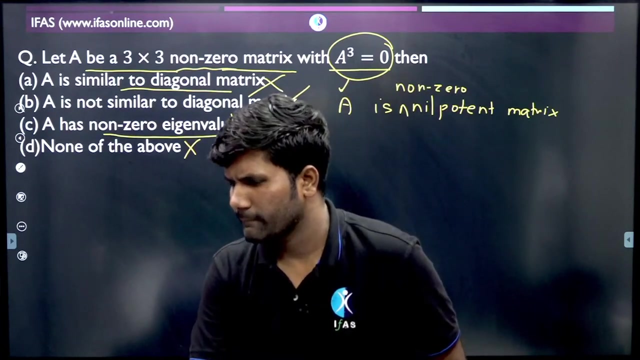 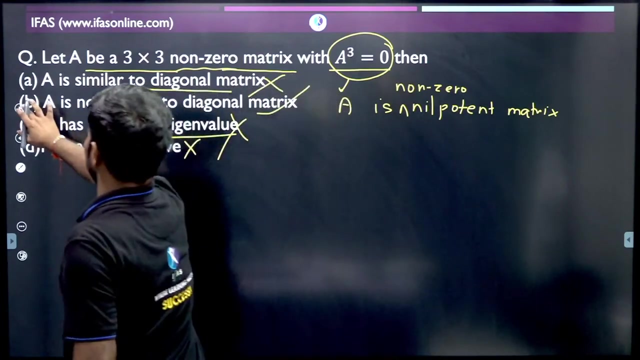 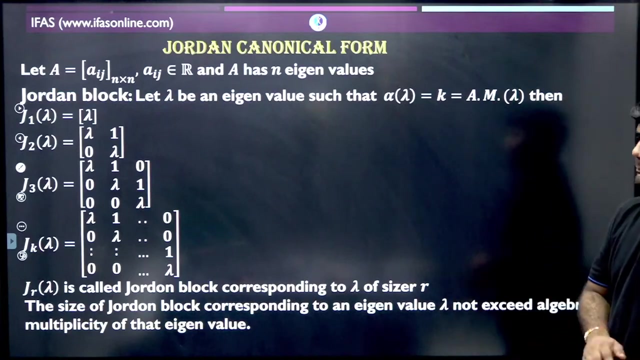 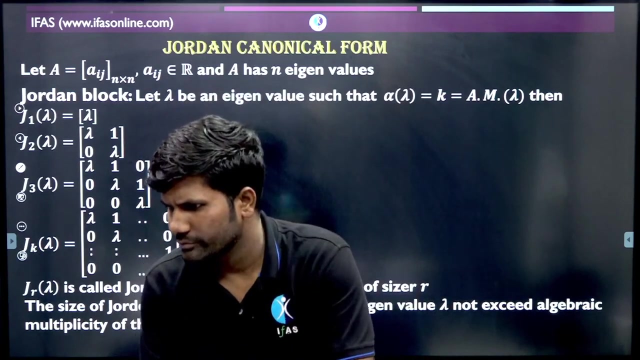 did not upload. yes, lalitha, ok, so let's see, let's start from here. let's try to solve the question directly, without theory. yes, we solve on the Jordan canonical form. yes, we do. let's go, let's do the theory or come to the direct question. 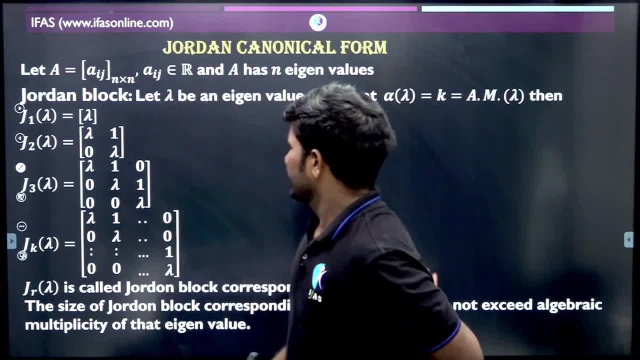 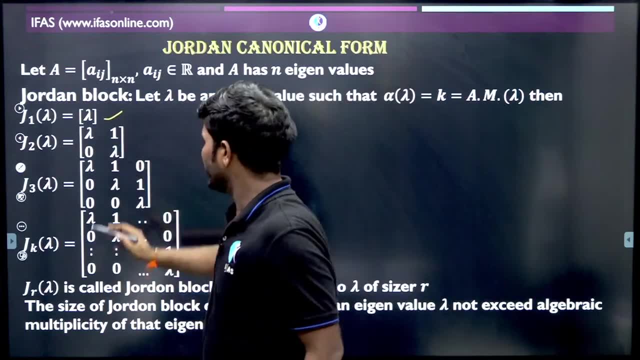 yes, tell me. the question is here to solve. look what we do in the jordan canonical form. we write in the Jordan block. if an eigenvalue is repeated once, then we write it this way. if it repeats twice, then we write the eigenvalue in diagonal and on that we write one here. 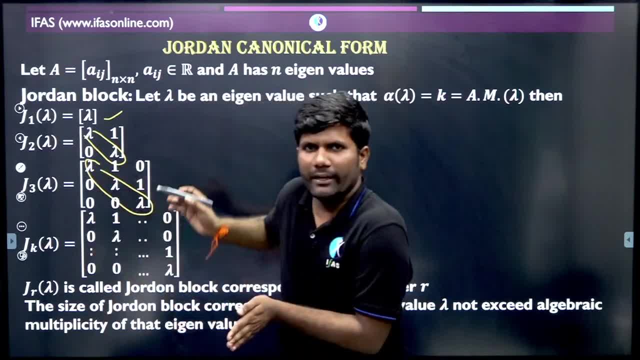 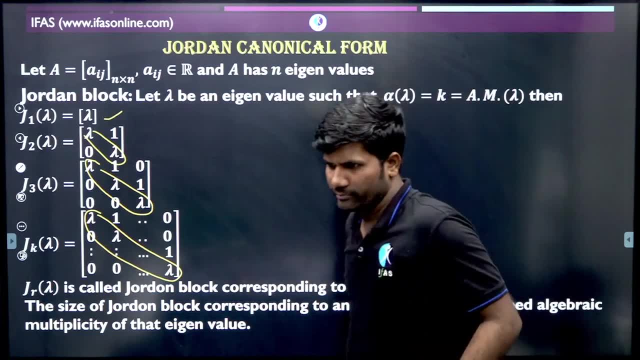 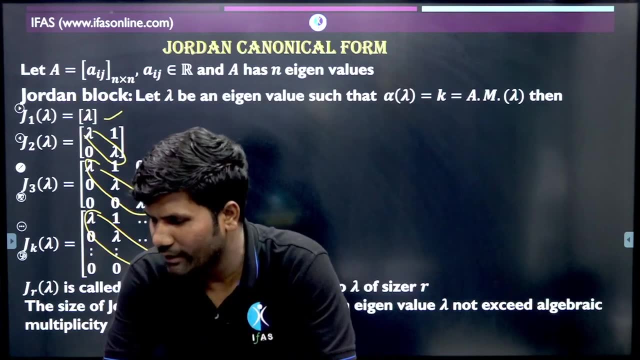 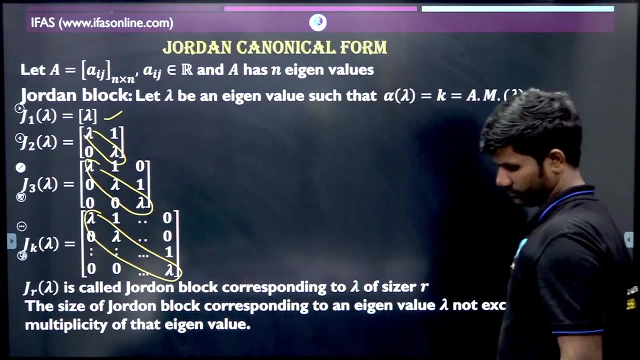 it happened three times, so I wrote it in diagonal and on that diagonal, the one that goes above. same way, we write n times this way and write 1,1,1,1 on the diagonal above it. no download will happen. let's move ahead. we are given tools for conversion. 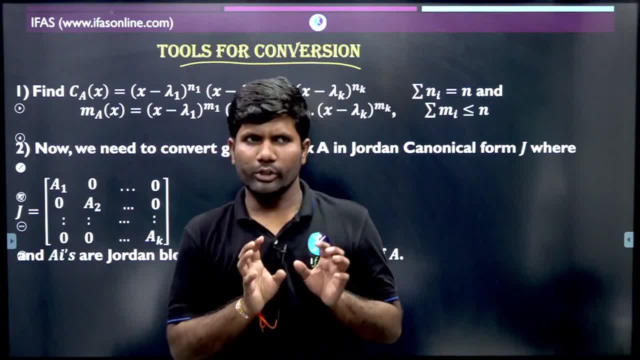 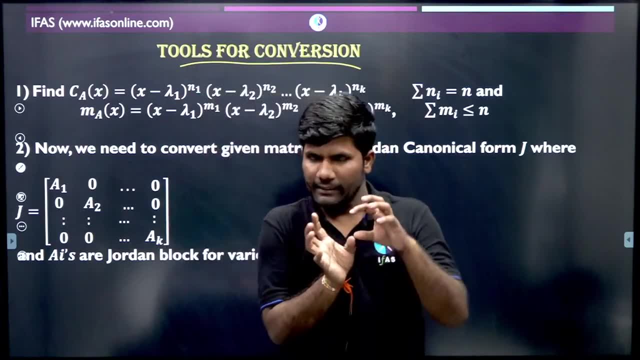 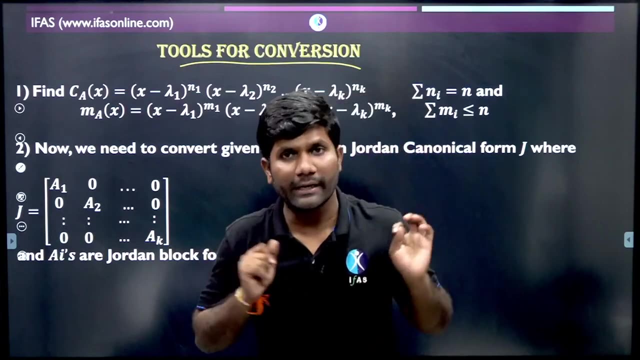 we diagonalize a matrix because when a complicated matrix comes in diagonal form, when a complicated matrix appears in the form of diagonal, then it is easy to find its eigenvalues, eigenvectors, triads, ranks, determinants. but all the matrices are not diagonalizable. 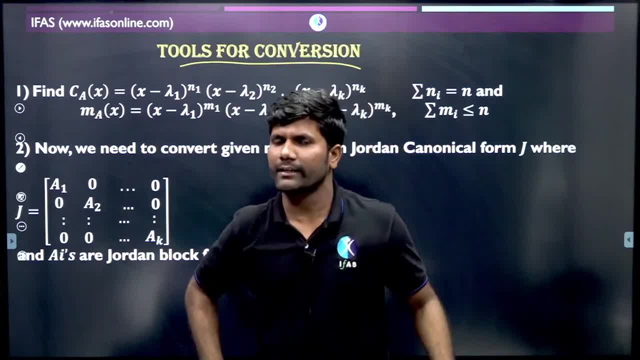 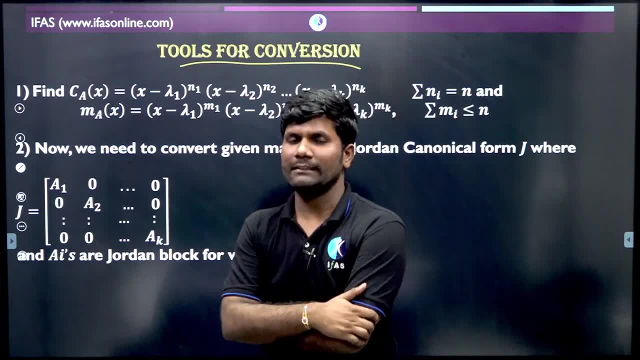 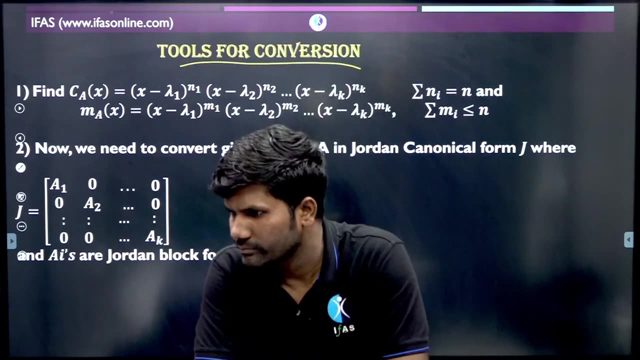 now we know that if the matrix is not diagonalizable, then how to find its property? so in that case we have a big tool which is called JST form, Jordan Canonical Form. so in that case, we do Jordan Canonical Form, we do awareness, we will do awareness. 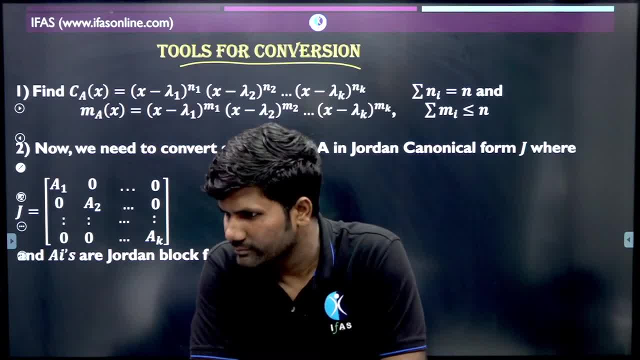 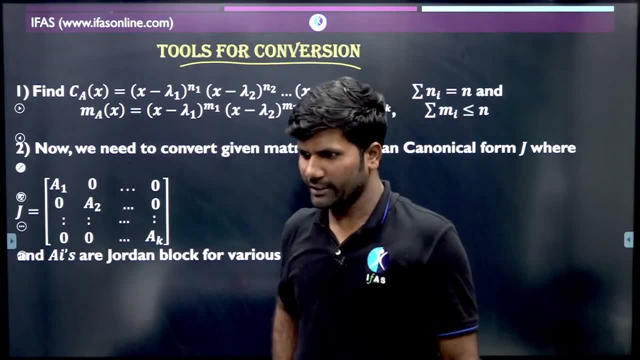 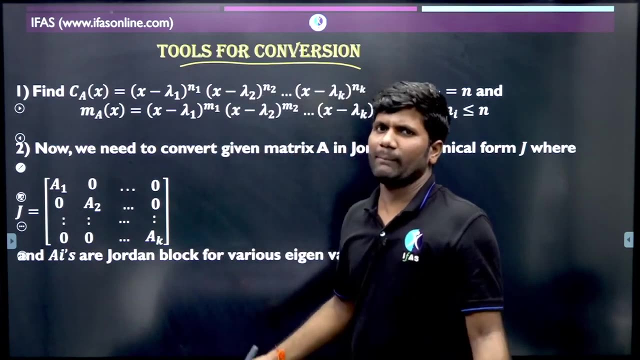 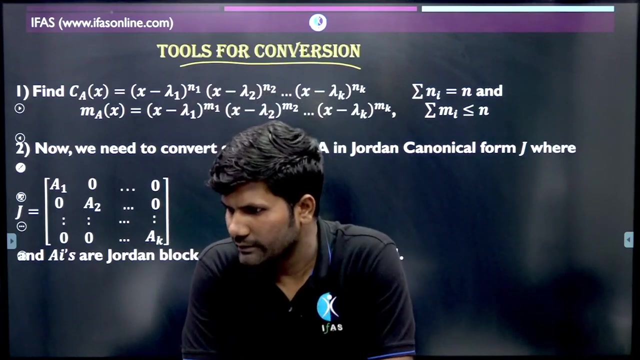 yes, Mayuri, tomorrow will be Upside Algebra. similarly, tomorrow will be session of Upside Algebra, if I am correct now. this whole week will be successful because it is Maharashtra state exam. so we want you to revise all these things once. ok, see for you. Maharashtra state test series has also come. 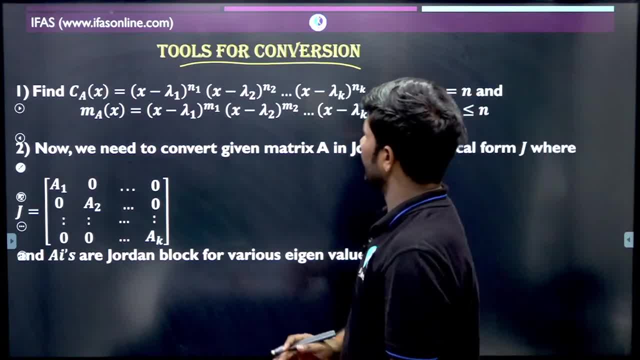 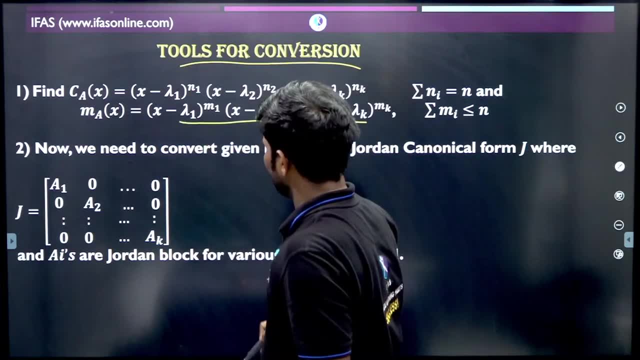 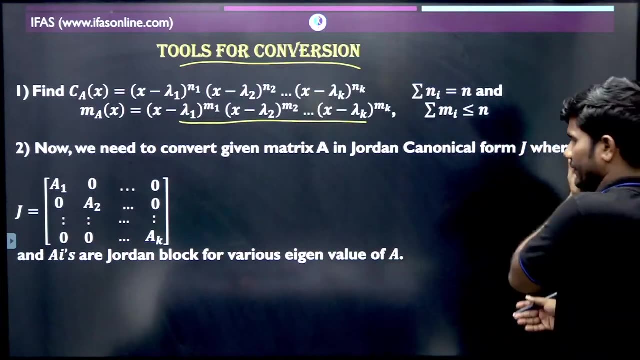 let's move ahead. in that case, what we do? first, find the characteristic polynomial, find the minimal polynomial of the matrix. now, minimal polynomial will be something like this: ok, after that, what you have to do, you have to convert it into Jordan Canonical Form. now it comes to how we will convert. 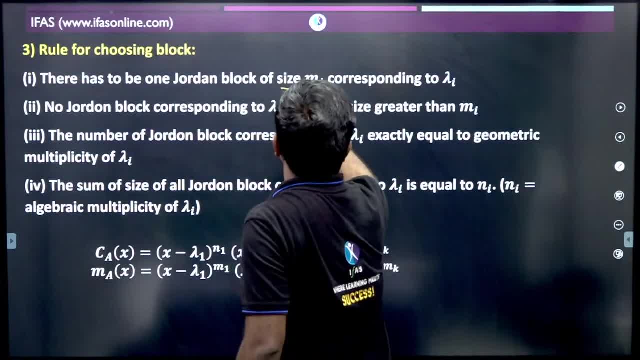 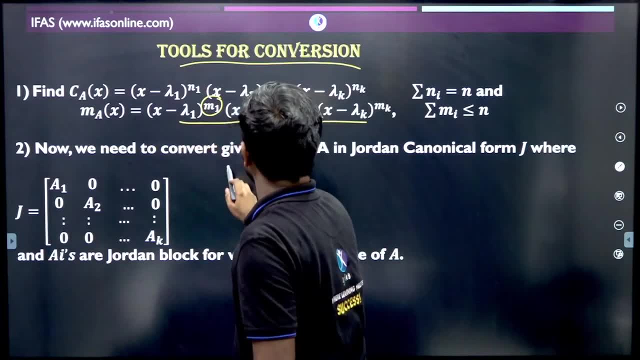 so what I do to convert. now, whatever the power of the minimal polynomial, see what is the power of the minimal polynomial if it is M1. so here the block which you will make for lambda 1. its size should not be more than M1. either M1 will be maximum or less than that. 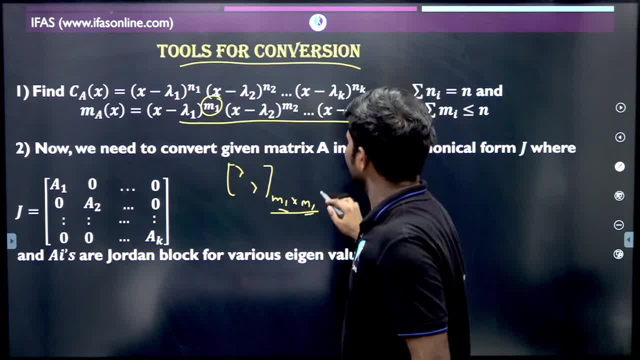 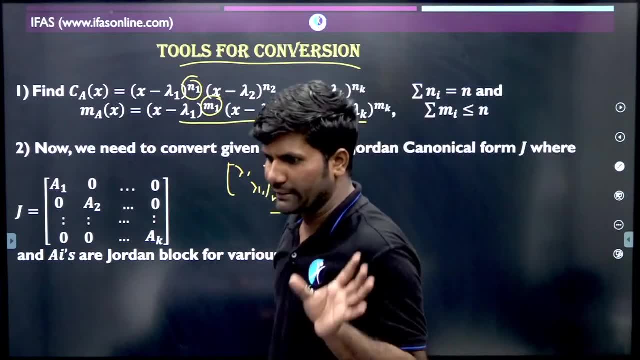 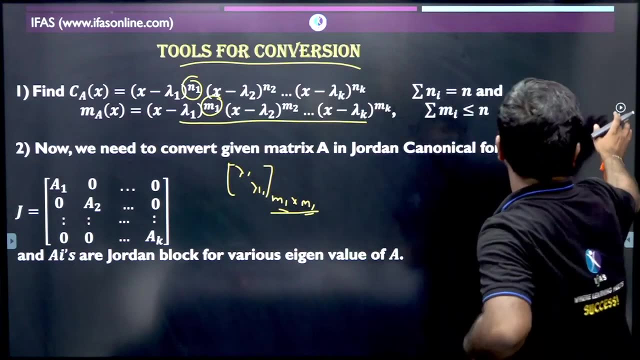 keep this in mind and to do the whole sum for the block which will be made for lambda 1, to do the sum, you should get N1 for every eigen value. you have to do this process. you have to repeat it. ok, clear now. after that, now it comes to. 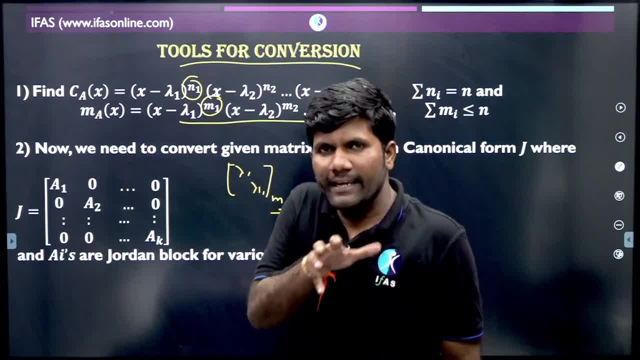 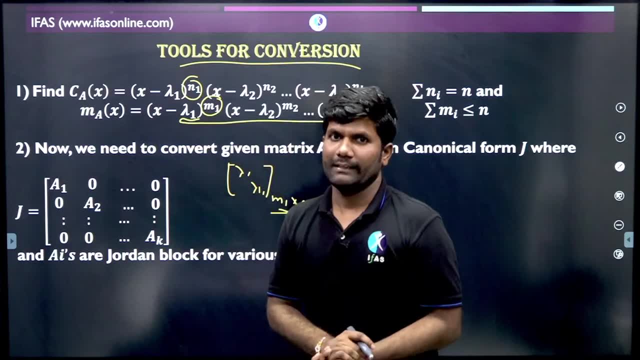 how many blocks are made for any eigen value, so only those blocks are made. like for lambda 1, I think, how many blocks are made, so only those blocks will be made. as much as its geometric multiplicity or the number of linearly independent eigenvectors. 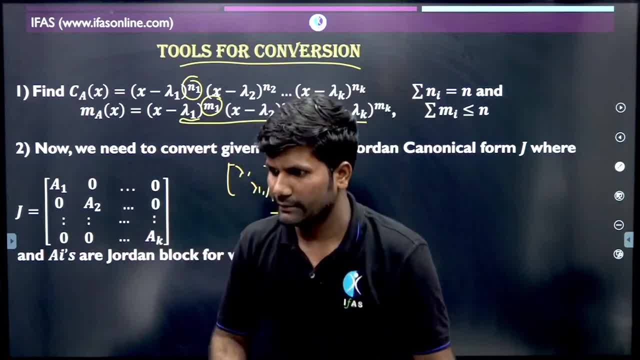 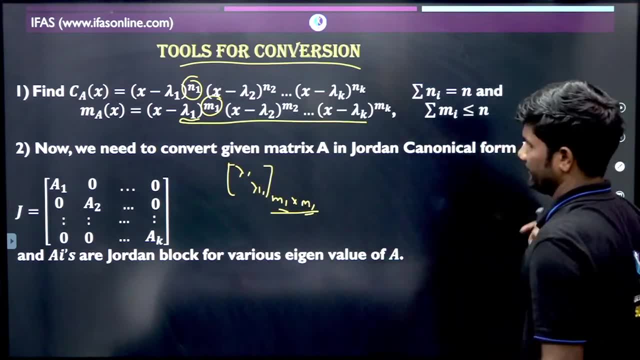 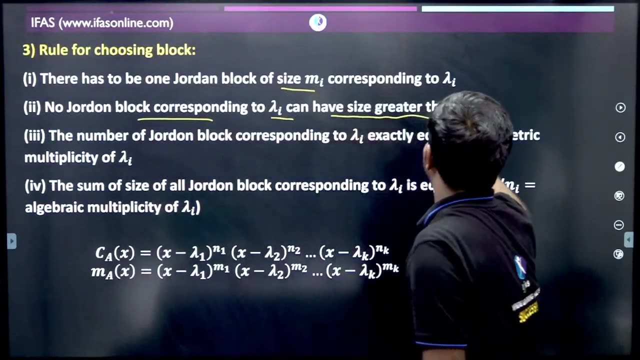 as much as its Jordan blocks are made ok, clear. thank you, noob entertainment. thank you so much. let's go now. let's talk further. now what is here? number of Jordan blocks corresponding to lambda. i have a size greater than can have a size no Jordan block. 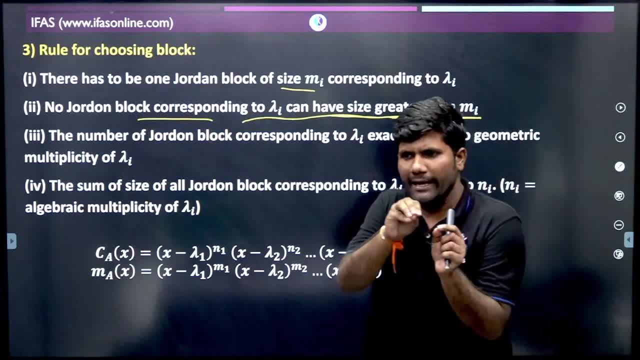 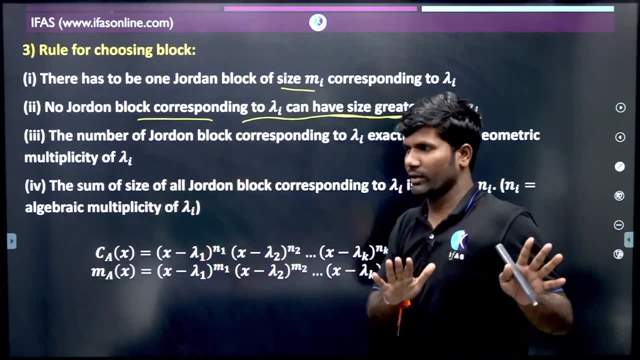 corresponding to lambda i has a size greater than M. i means if, for any eigen value, if you are making a block which will have the power of minimal polynomial, no matrix can be bigger than that. it will be smaller than that, ok, third, what it says: the number of Jordan blocks corresponding to lambda i. 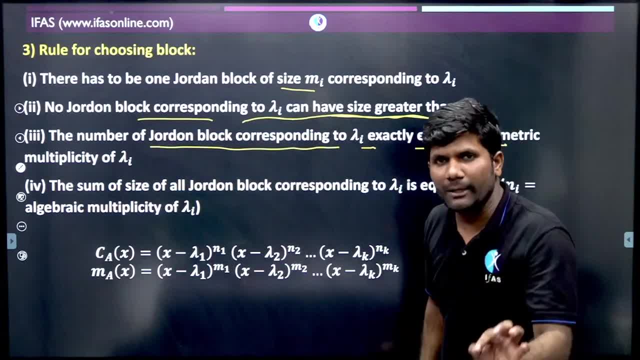 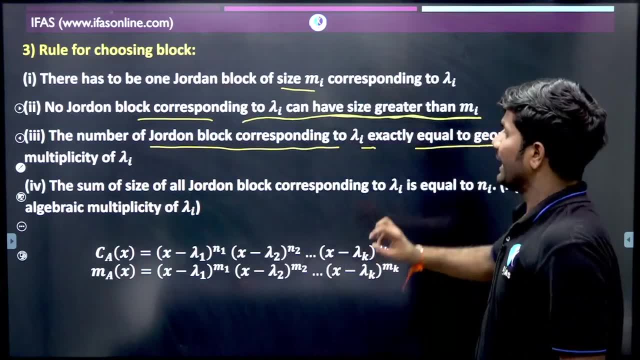 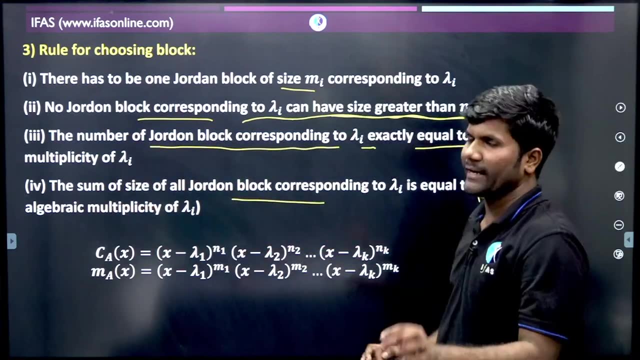 exactly equals to the geometric multiplicity. any eigen value for lambda now it comes to how many blocks are made. so as much as its geometric multiplicity is exactly that many blocks are made, and every block when you add its order, how much will you get? you will get n i. 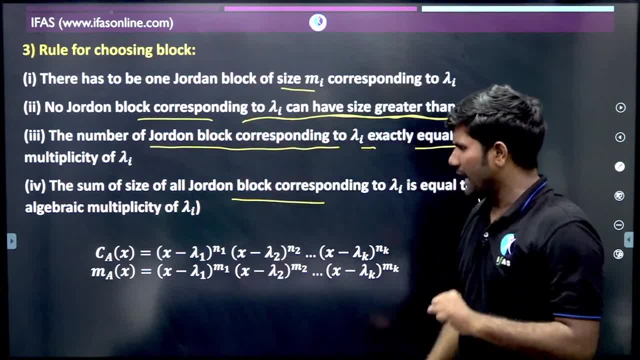 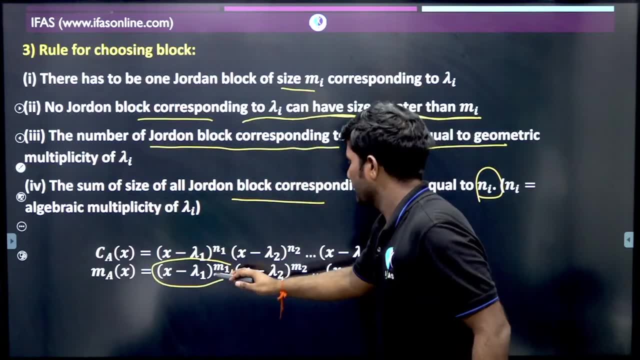 means the power of minimal characteristic polynomial. so here, ok, see this. for this, for lambda 1, how many blocks will be made, the size of this block. how much will be the size of this block? maximum will be m1. and how many blocks will be made, how much will be its geometric multiplicity. 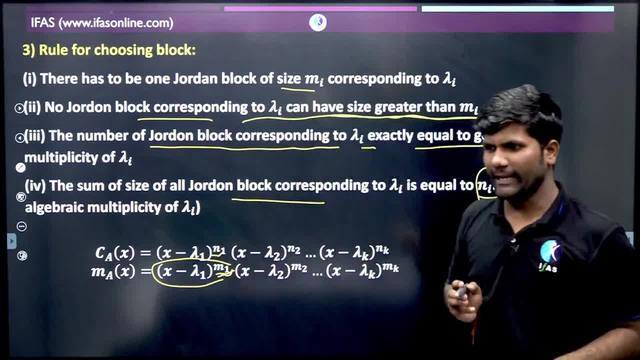 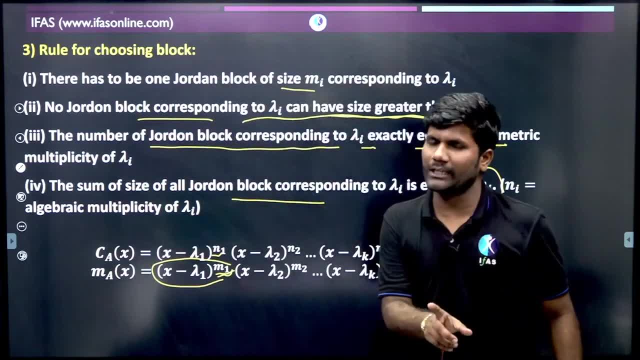 and if you add the order of all the blocks then you should get n1. ok, if you keep this much in mind, then you can easily convert in Jordan canonical form. so any matrix we convert in Jordan canonical form so that we can easily know its property, because then 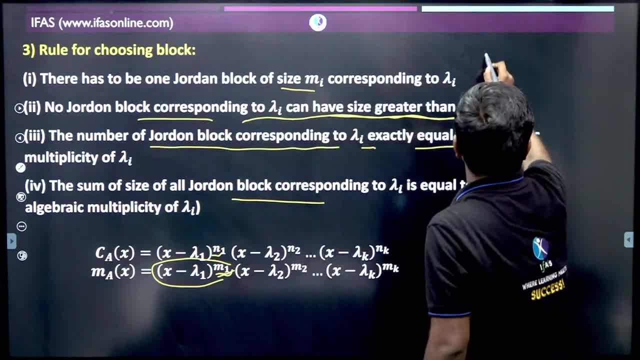 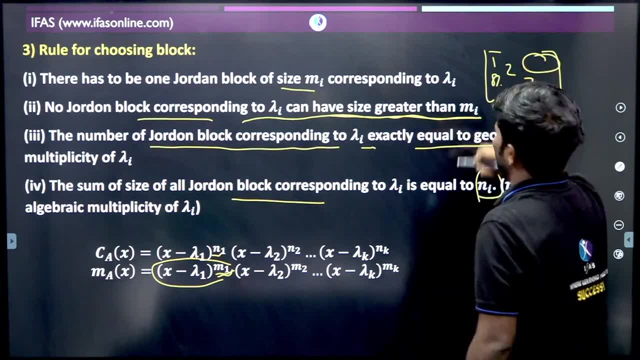 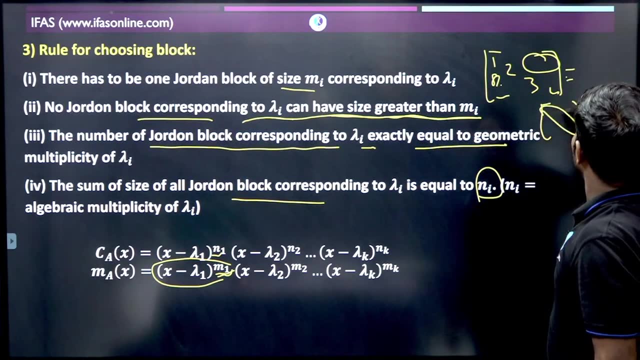 it comes in the form of block. now tell me once. I will give you a matrix like 1, 2, 3, 4, 5, 6, 7, 8, 9, 10, 11, 12, 13, 14, 15, 16, 17. 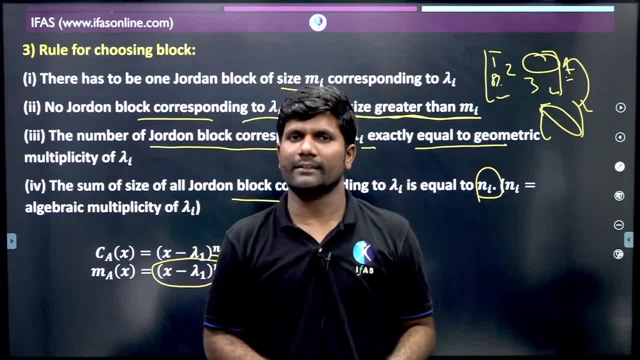 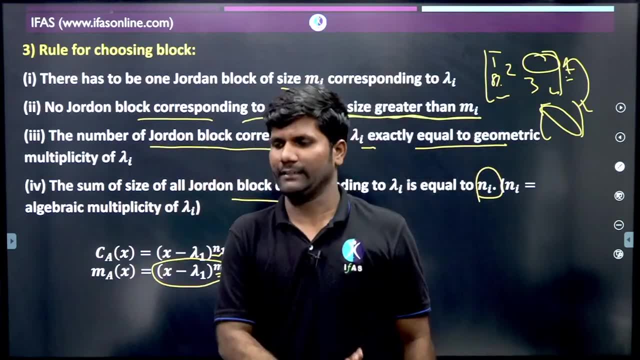 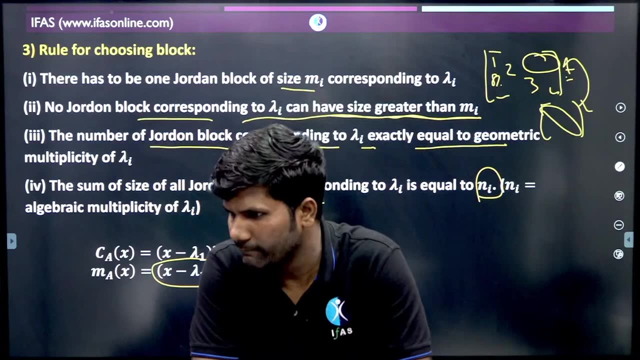 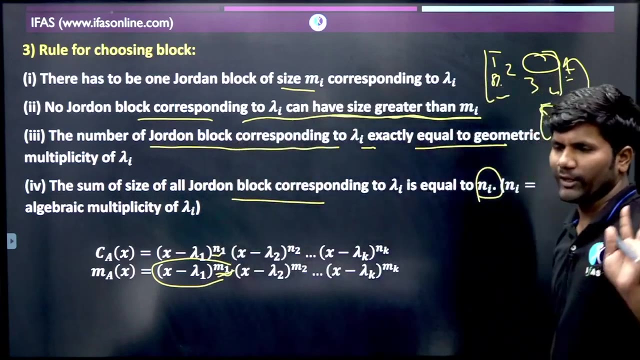 18, 19, 20, 21, 22, 23, 24, 25, 26, 27, 28, 29, 30, 31, 32, 33, 34, 35, 36, 37, 38, 39, 40, 41, 42, 43. 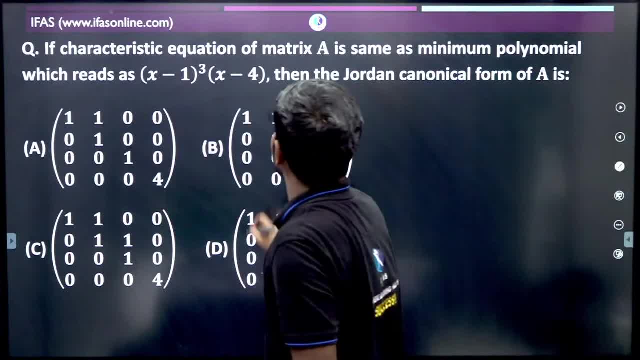 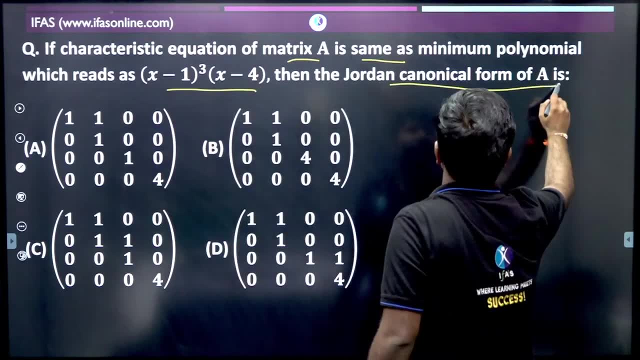 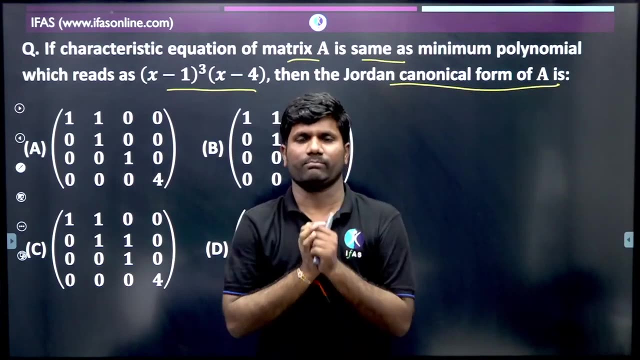 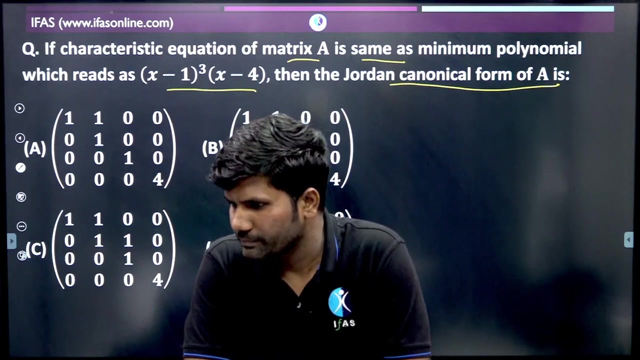 44, 45, 46, 47, 48, 49, 50, 51, 52, 53, 54, 55, 56, 57, 58, 59, 60, 61, 62, 63, 63, 63, 64, 65, 67, 68. 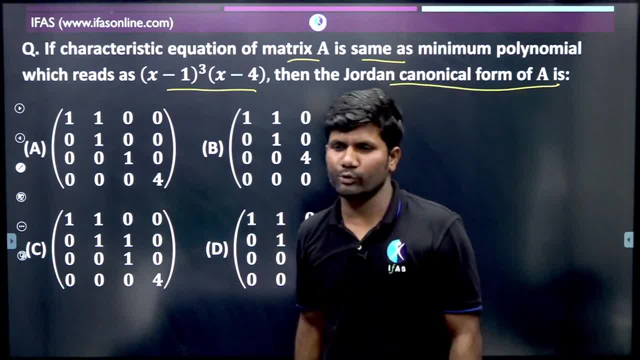 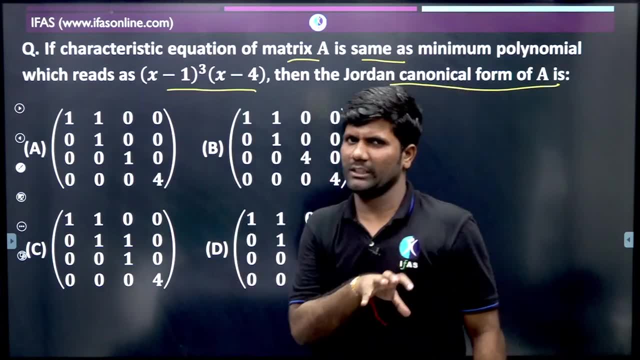 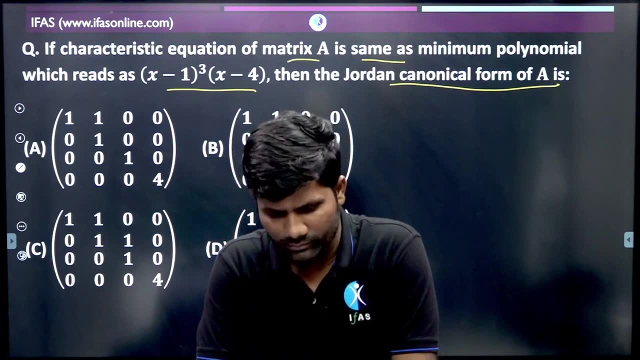 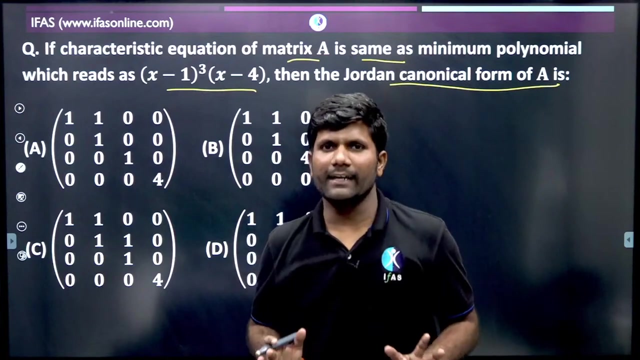 69, 69, 70, 71, 72, 73, 74, 75, 76, 77, 78, 79, 80, 81, 82, 83, 83, 84, 85, 86, 87, 88, 89, 90, 90, 91. 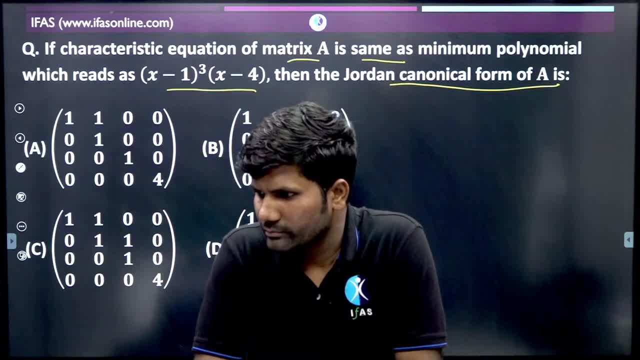 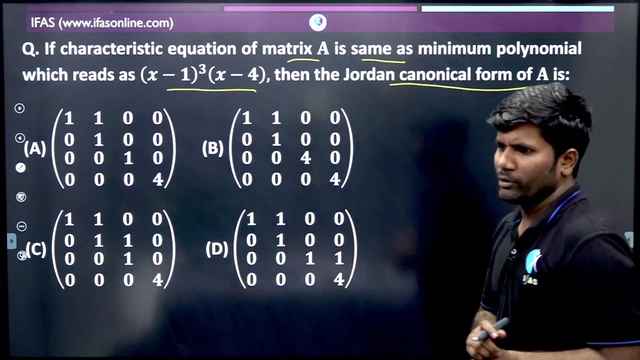 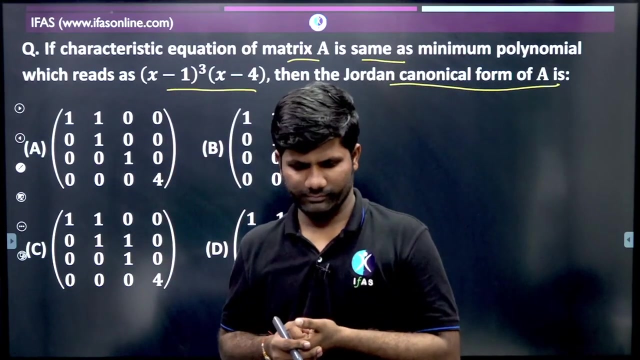 92, 93, 93, 94, 95, 96, 97, 98, 99, 100, 100, 10, 11, 12, 13, 14, 15, 16, 17, 18, 19, 20, 22, 23, 24, 25. 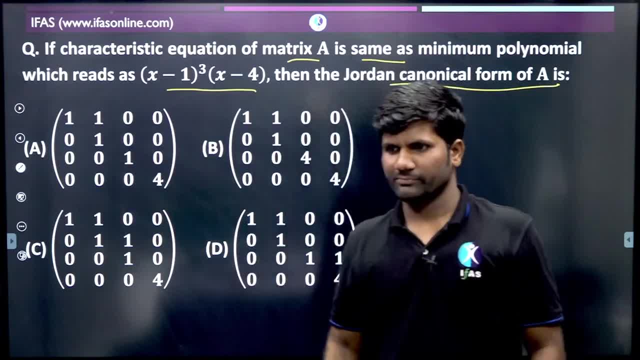 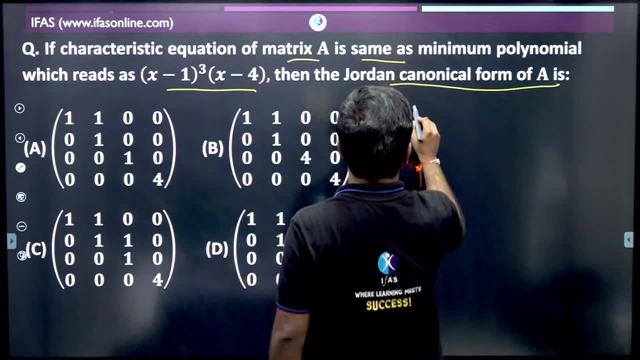 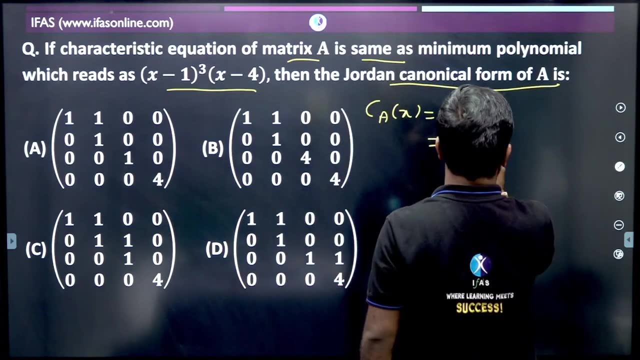 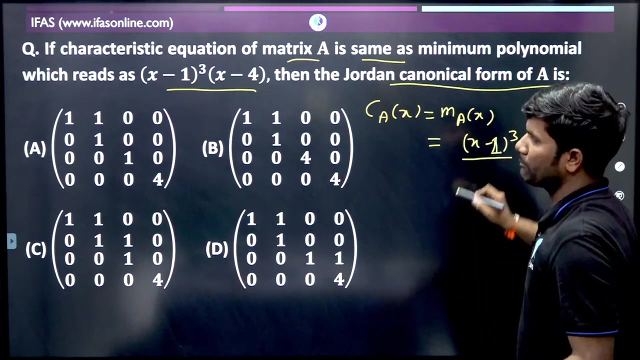 26, 27, 26, 27, 28, 29, 30, 31, 32, 33, 34, 35, 36, 37, 38, 39, 40, 41, 42, 43, 44, 45, 46, 47, 48, 49. 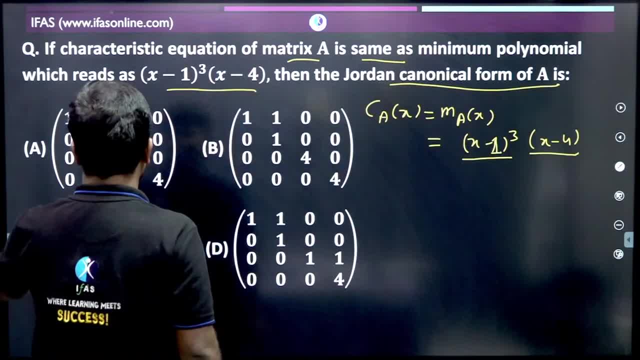 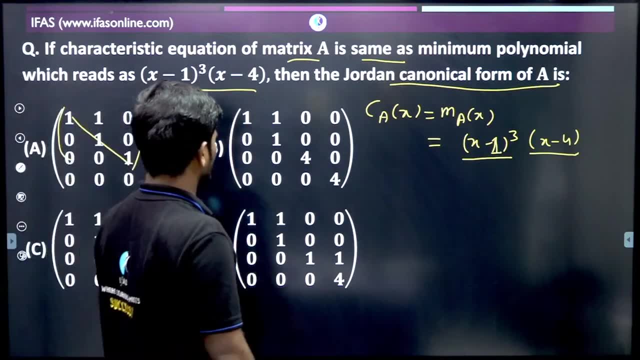 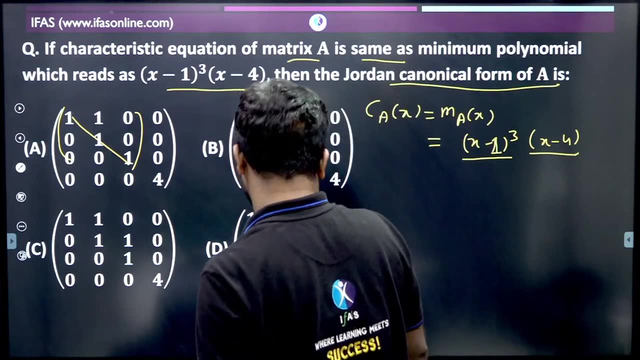 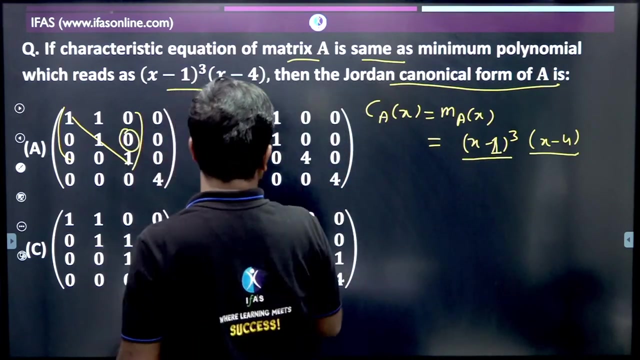 49, 50, 51, 52, 53, 52, 53, 54, 55, 56, 57, 58, 59, 60, 61, 62, 63, 64, 65, 66, 67, 68, 69, 69, 70, 71. 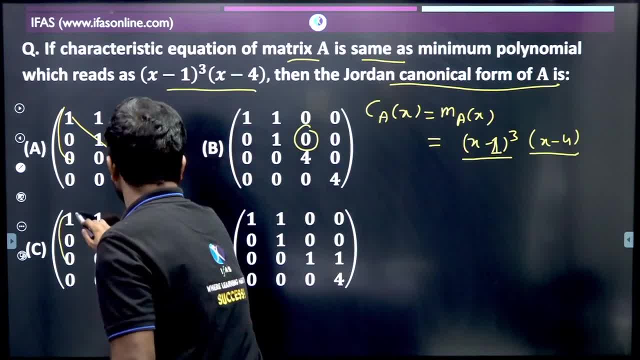 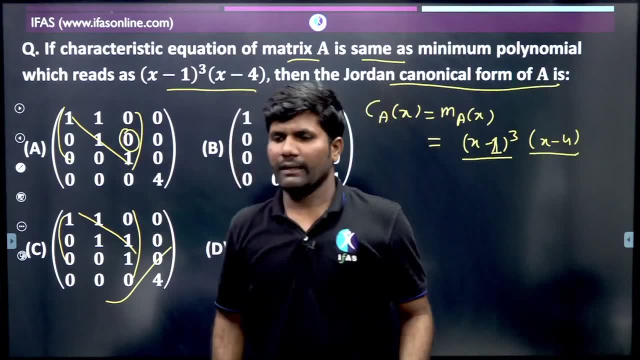 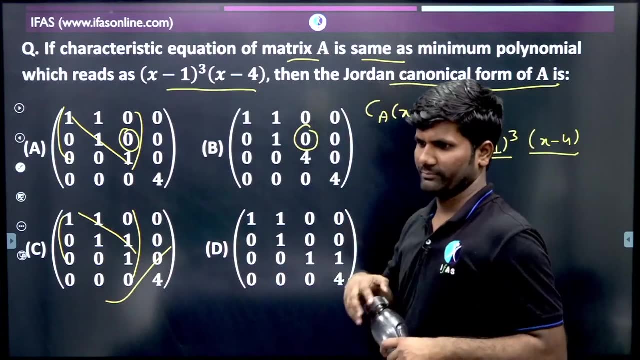 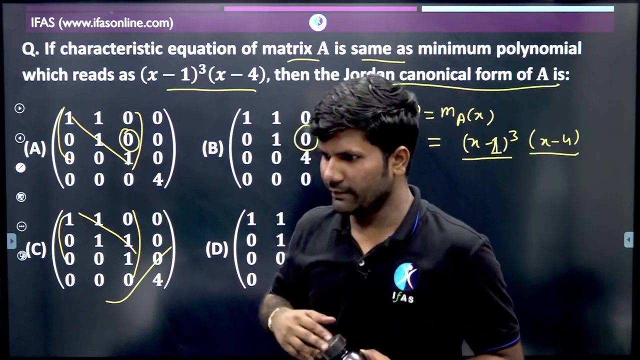 72, 73, 73, 74, 75, 76, 76, 77, 78, 78, 79, 79, 80, 81, 82, 83, 84, 85, 86, 87, 88, 89, 90, 91, 92, 93. 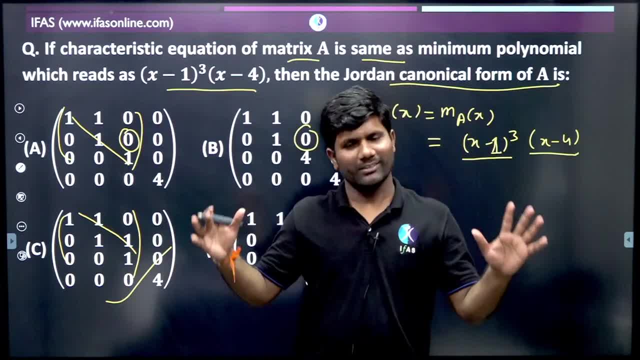 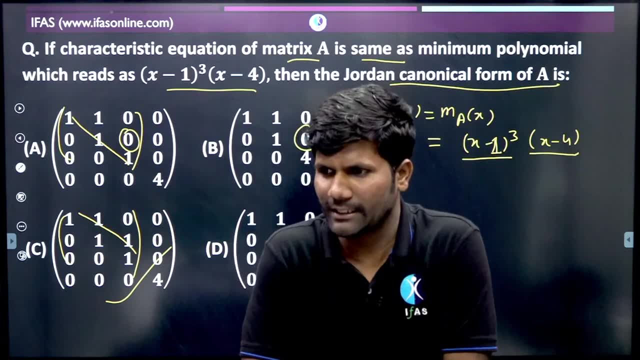 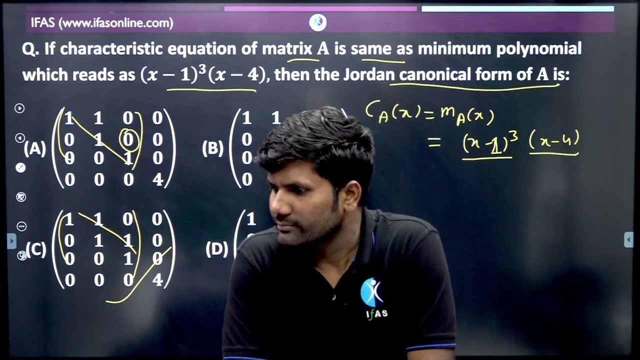 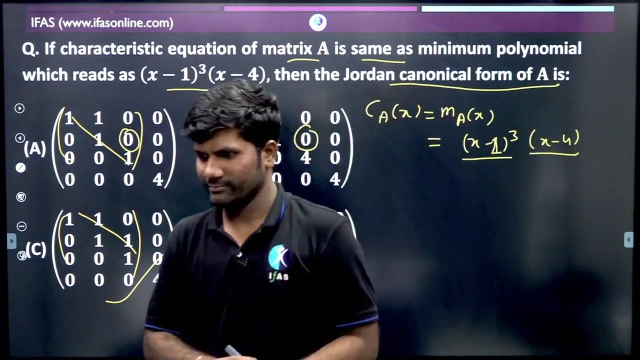 94, 95, 96, 97, 97, 98, 99, 100, 100, 100, 100, 100, 100, 100 15, 10, 11, 12, 13, 14, 15, 16, 17, 18, 19, 20. 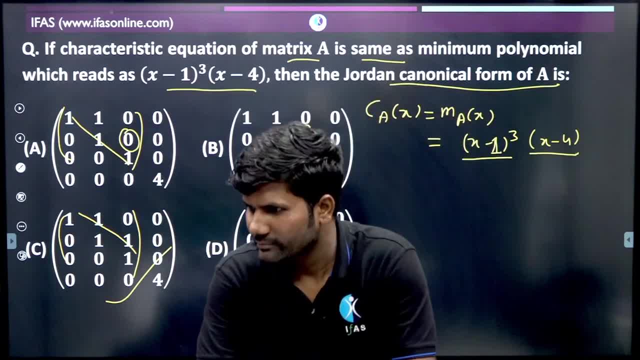 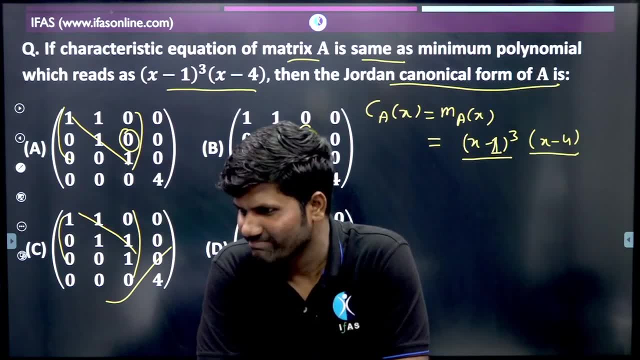 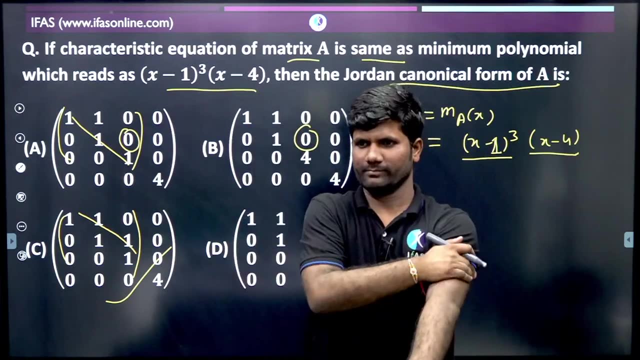 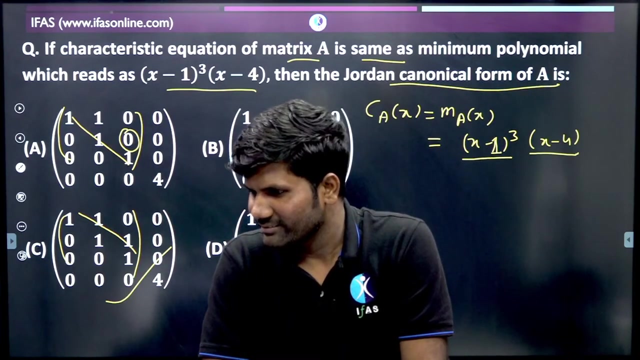 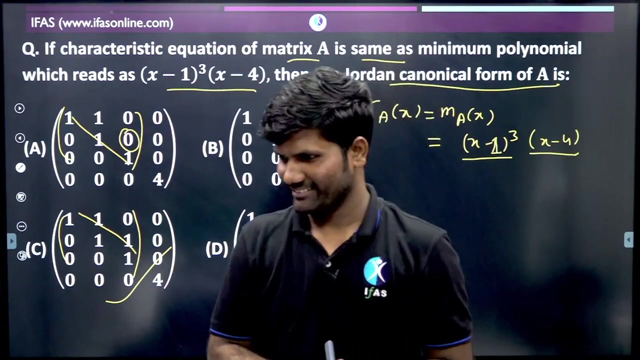 21, 22, 23, 24, 25, 26, 27, 28, 29, 30, 30, 31, 32, 33, 34, 35, 36. Thank you, ABKarim. you guys are good, that's why the teaching is looking good here, okay. 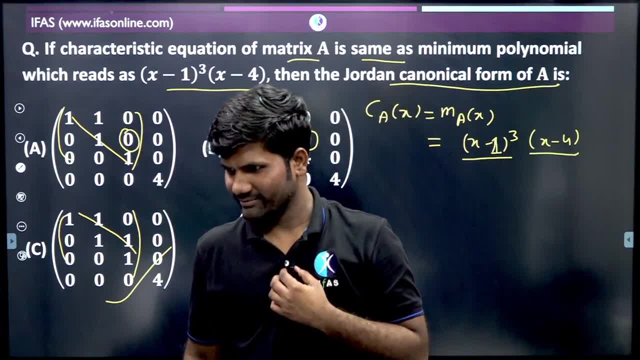 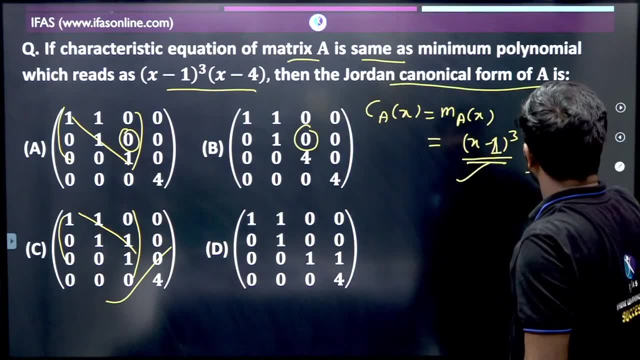 Shall we go? Tell me once, Sandesh, what is the short trick of this? Now, tell me. this is the minimal polynomial that is given, that is, one block will be made of this, one will be made of this, and there is no short trick in this. this is clearly. 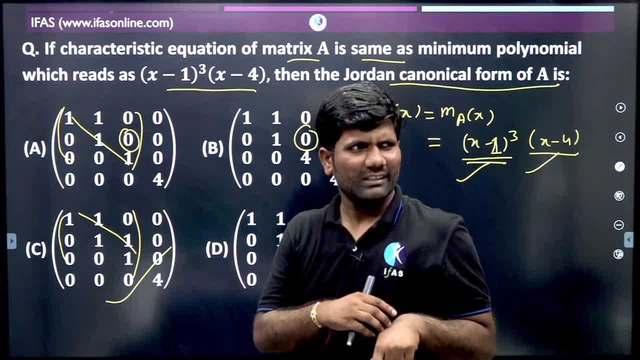 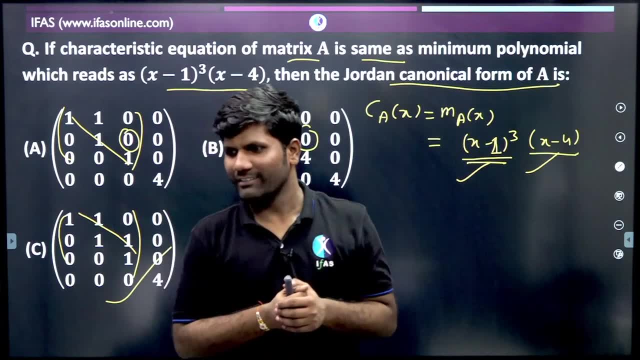 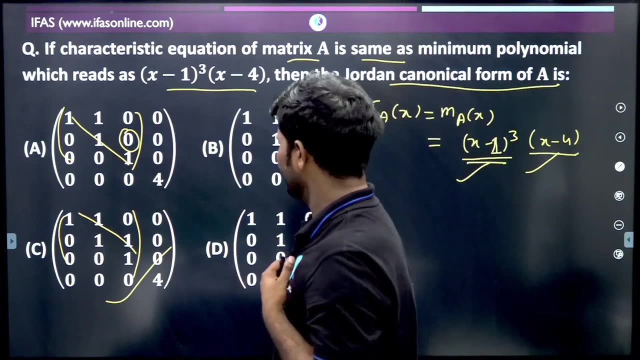 visible Sandesh Thackeray. Sandesh, are you an offline batch? Thank you, Sachin Kedar. Vesnavi Ingole is saying that it will be C. very good, Vesnavi, you are a little late, okay. 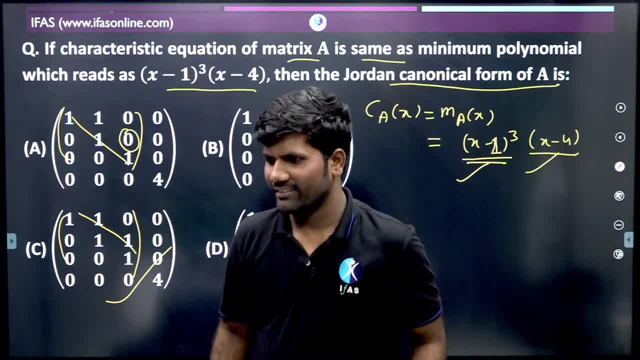 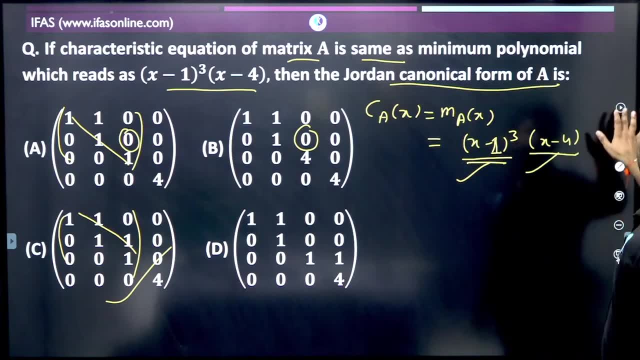 Along with time. if you have to remove the video, then a lot happens, right? Okay, come on, let's come to the next slide. Okay, So I have given one more question: what is the real matrix of A? 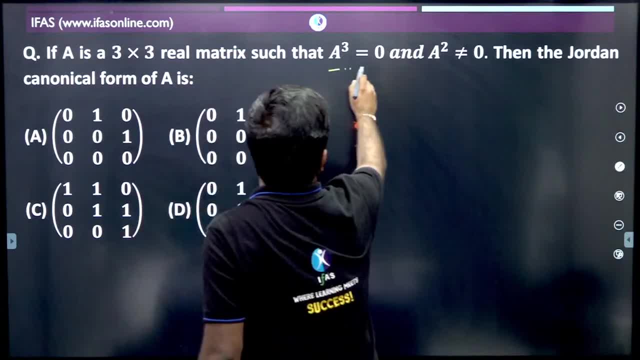 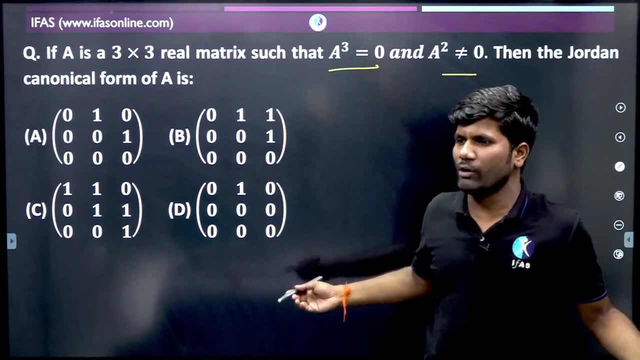 What is the real matrix of A? Now, here, what is given is a three cross three real matrix, such that A cube is equal to zero and a square is not equal to zero. Then the Jordan canonical form of A. Now tell me what is the correct answer to this. 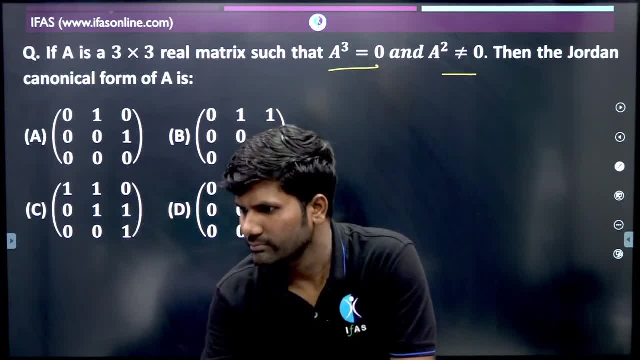 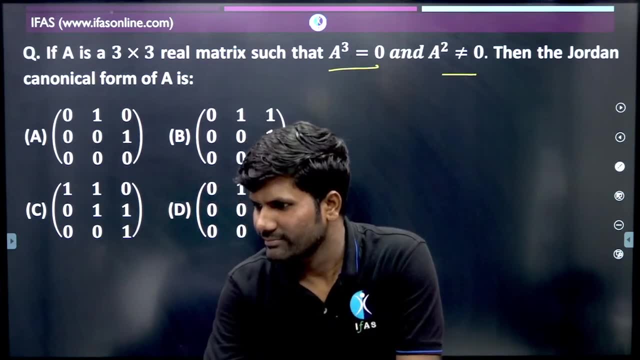 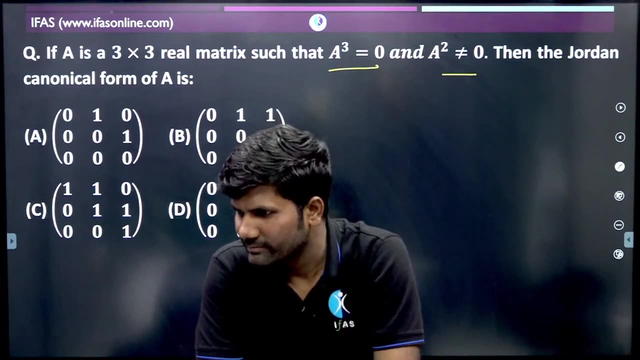 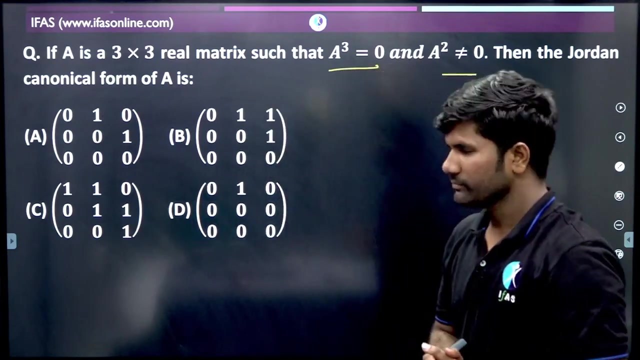 Sorry students, Tell me what will be its answer. Sorry students. So if your doubts are cleared, then do the exam properly and pass it this time. okay, Here see what is given to us. A is 3 cross 3 matrix, such that A cube is 0.. 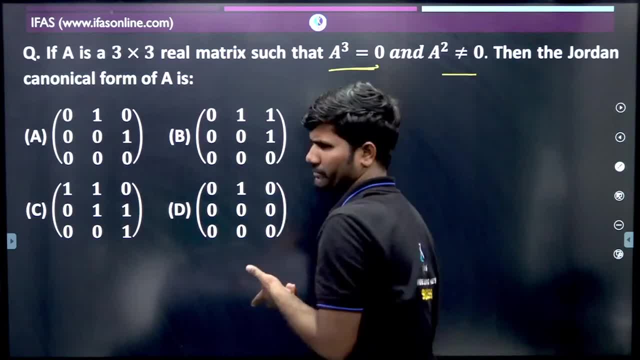 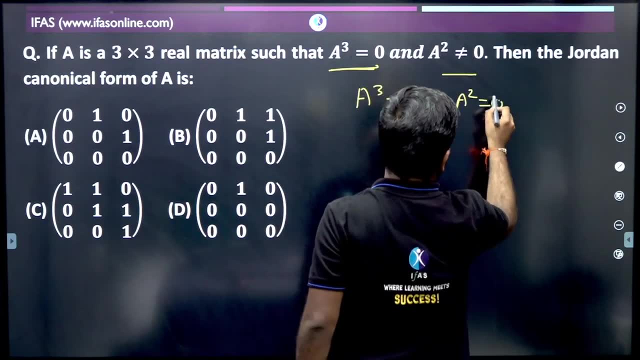 Now, A cube is 0, but A square is not equal to 0.. What will this mean? A cube is 0 and A square is not equal to 0.. If A square is not equal to 0,, what will this mean? 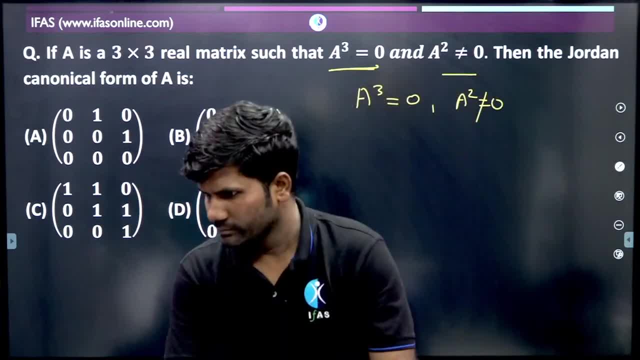 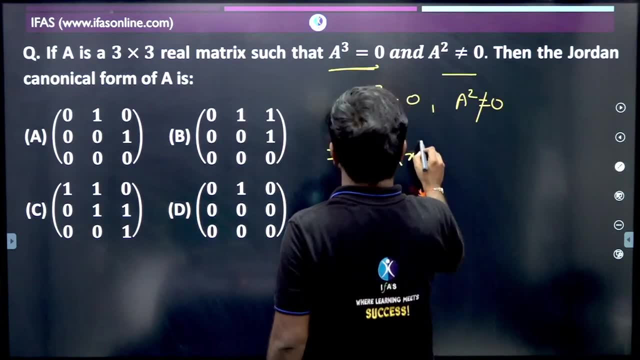 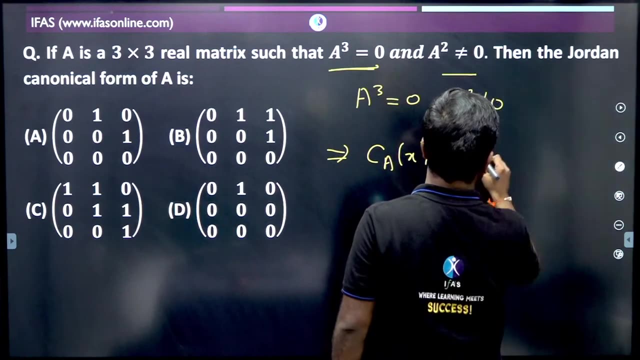 What will be its minimal polynomial? If A, this means its characteristic polynomial will be A cube. A cube means we are talking about X cube here. okay, But here X square is not equal to 0, A square is not equal to 0.. 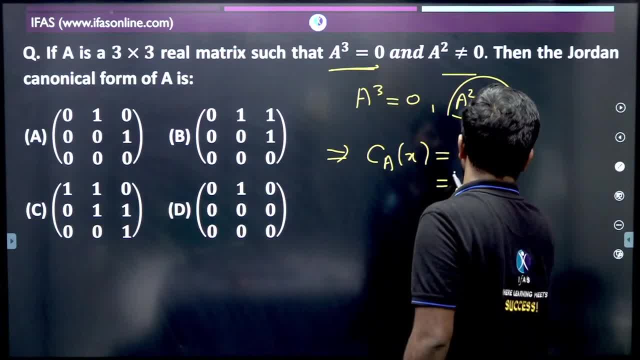 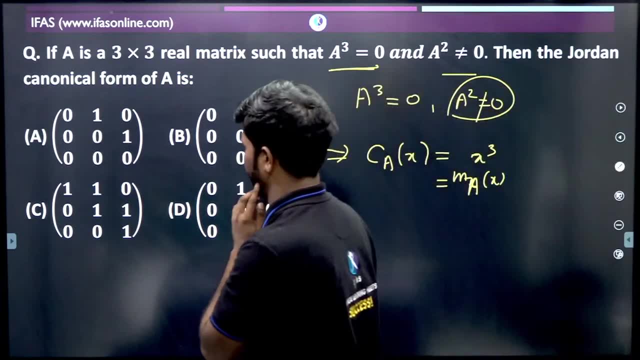 This means, its minimal polynomial will also be X cube. So what will be M, A, X, B? It will be X cube only. So here characteristic polynomial and minimal polynomial are both same. So here characteristic polynomial and minimal polynomial are both same. 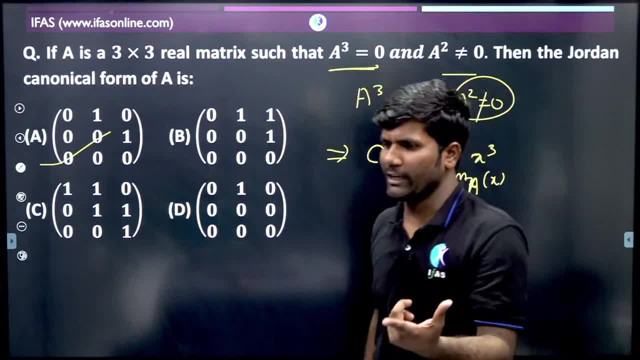 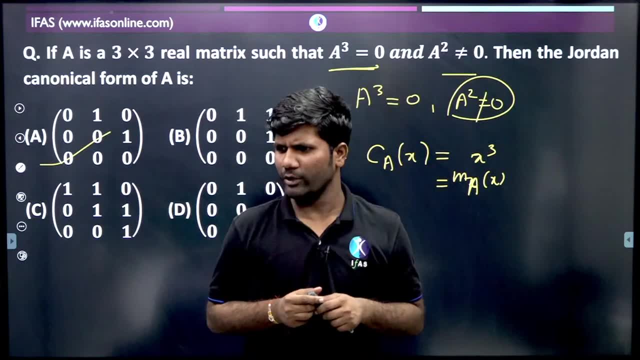 So correct answer will be the same. So here option is B. Pooja, Souraj, Shuleshwar, Vaishnavi Sachein, These three Bloom have given allство. Sheetal, Jamdade, Prateek, Nikita Aanchal Chowdhury. 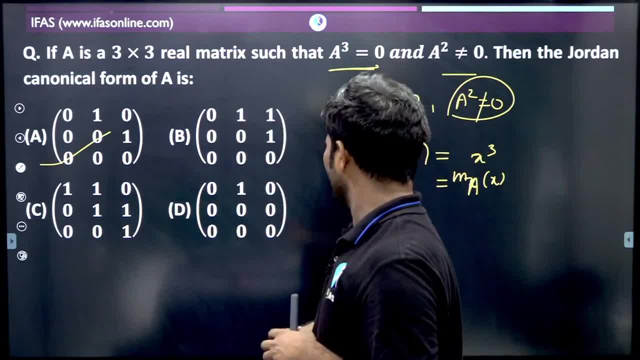 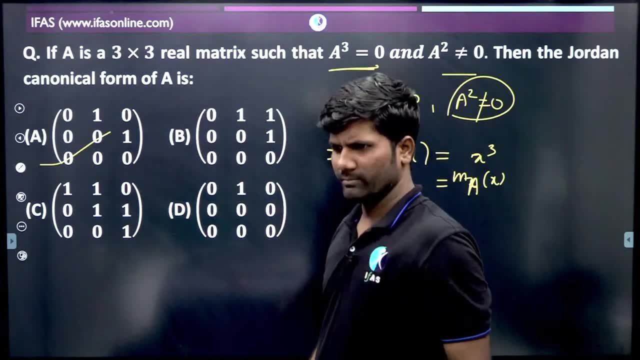 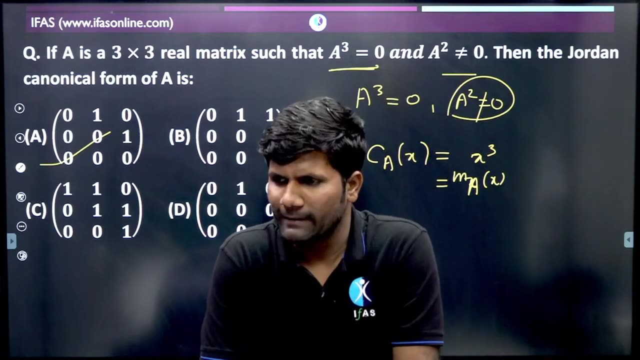 Almost all have given correct answer. Why D? Who has said D NOB Entertainment D not See it's not 1HP. Ok, Yes, it will be A. Is it clear to everyone? Let's move on to the next slide. 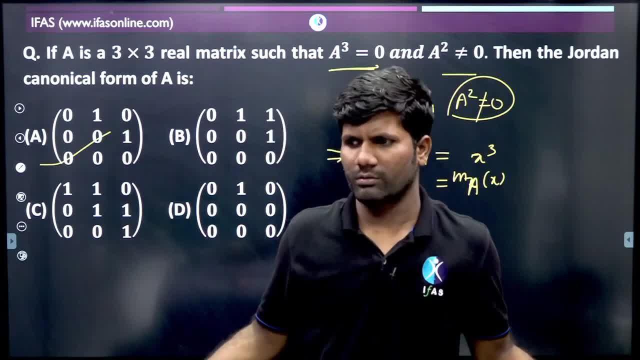 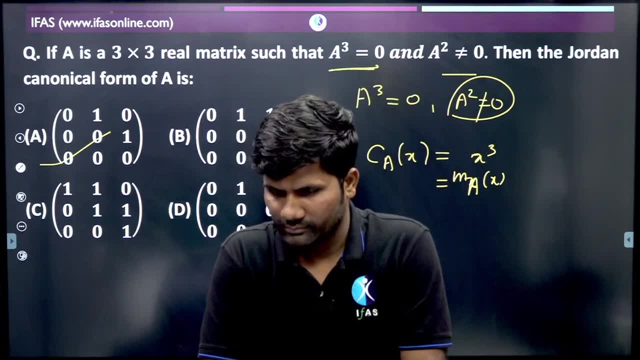 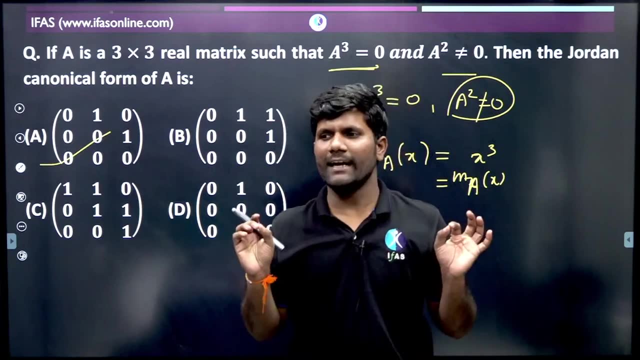 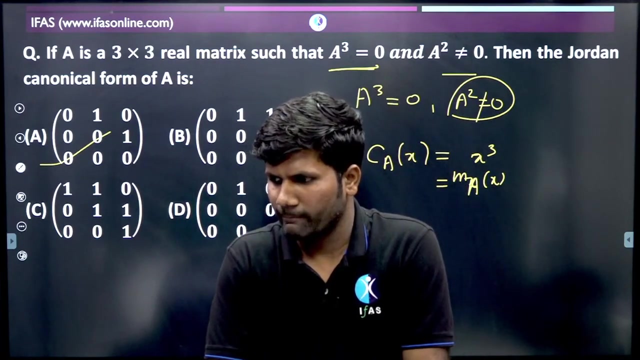 Why did I choose Q Lalitha? Tell me Confirm. Tell me Confirm. What is your doubt? Why are you not Confirmed? Is it clear to everyone? What is your doubt? Tomorrow will be the group theory at this time at 5 o'clock. 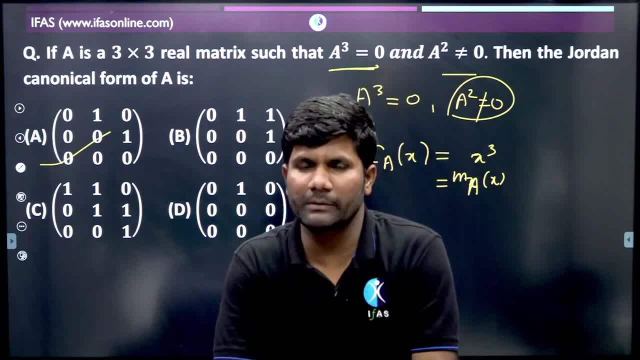 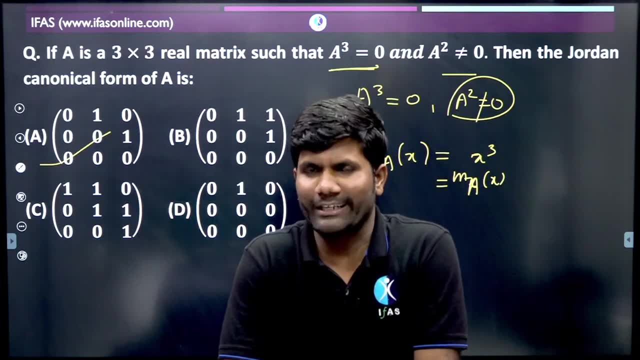 And if you want to practice questions, then from 8 o'clock it will run on our second channel. There will also be a 3 hour session Today. we will stay at Manohar, sir, it will be real, But there will be questions of DU. 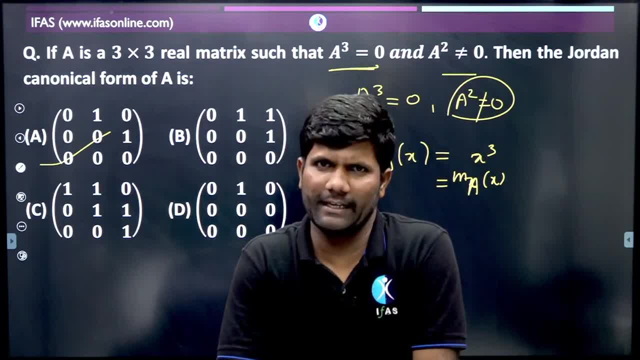 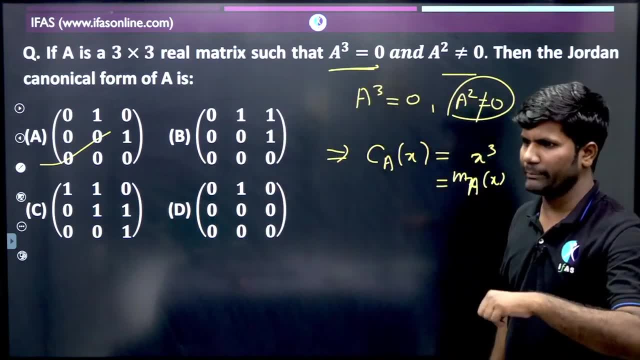 So the questions of DU are almost similar to your exam. So you can come there and do it, No problem, it is entertainment. You can come there and practice questions. at 8 o'clock the session will start, Sir. what to repeat for this? 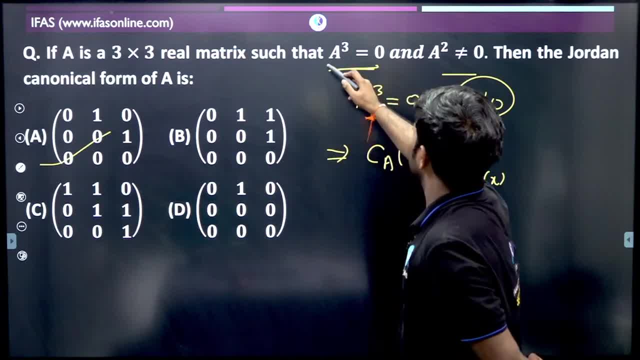 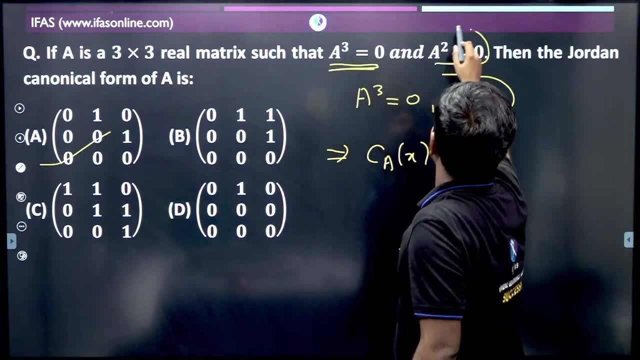 Sir, we were telling you here what is given to us: a cube is equal to 0.. If a cube is 0, it means it is a nilpotent matrix. But what is said here, a square is not equal to 0.. 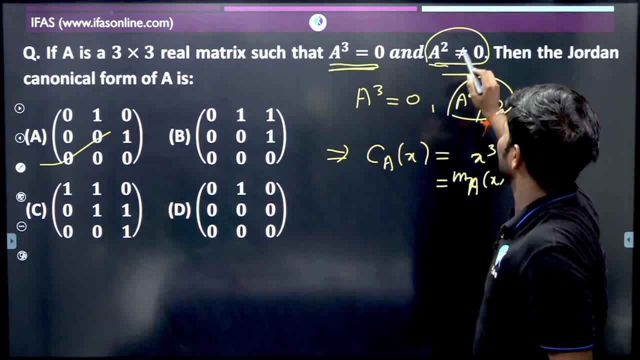 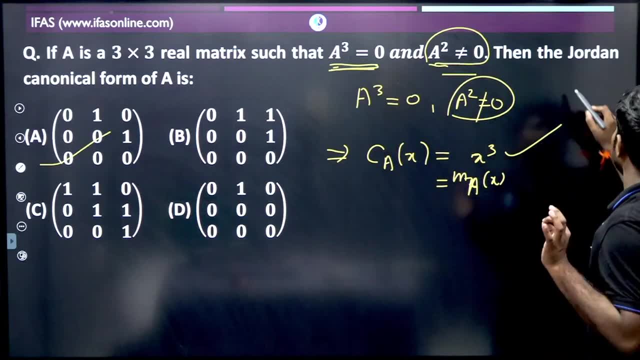 If a square is not equal to 0, then its minimal polynomial can not be x square. Its characteristic polynomial is 3 cross, 3 matrix and a cube is 0.. Now the minimal polynomial will be x Or it will be x cube. 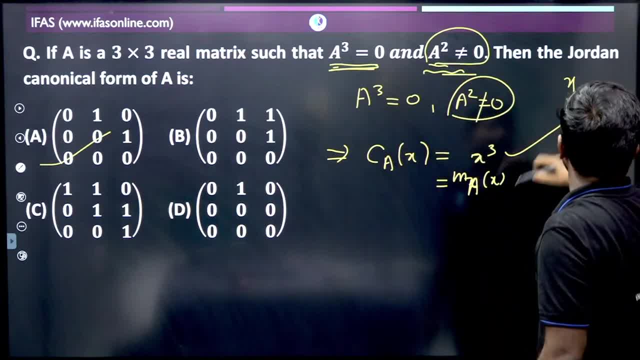 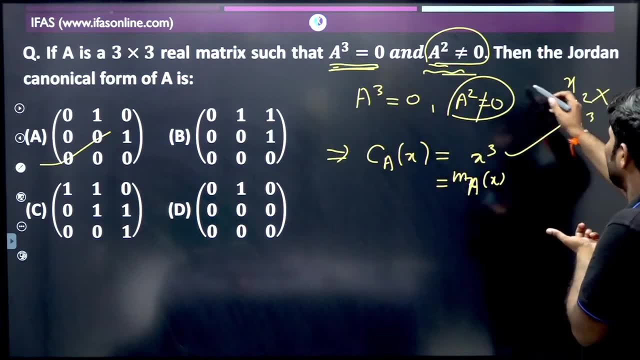 But here it is clearly given that a square is not 0.. It means it is not a minimal polynomial. Now the question is: will it be x? If it was x, then x square would also be 0.. It means a square. 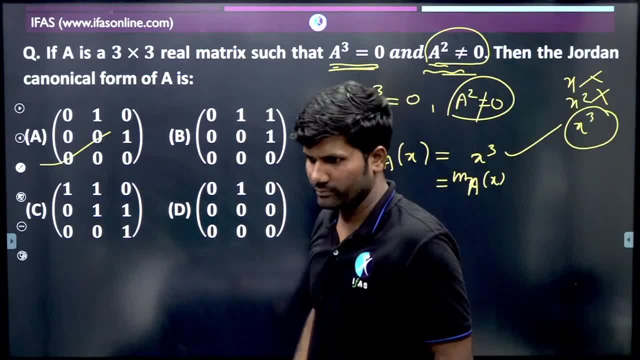 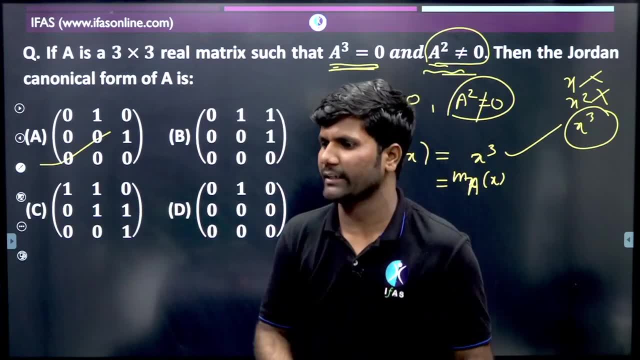 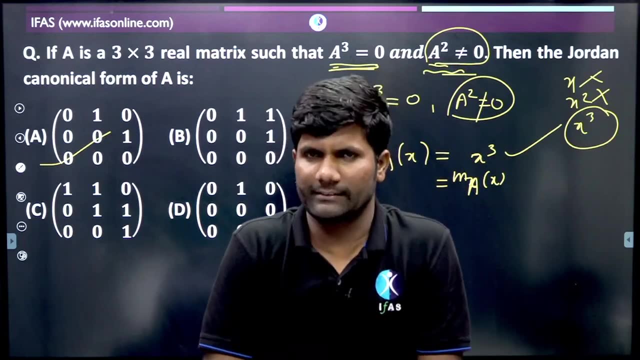 It means it is not even a, So this will be the minimal polynomial. Remember the name of the channel is iitjam mask. If our team is listening, then provide the link of iitjam channel in the comments. Remember the name of the channel is: 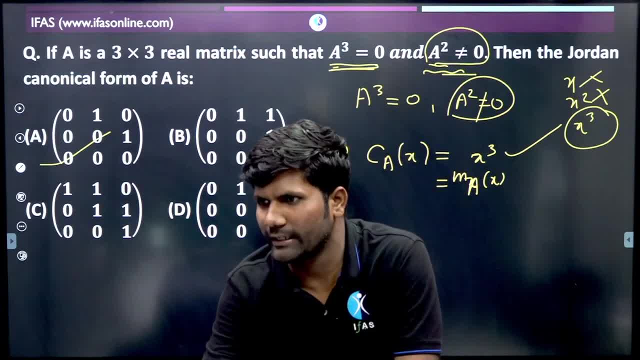 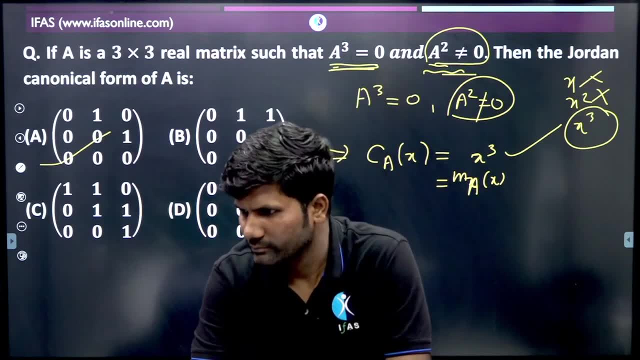 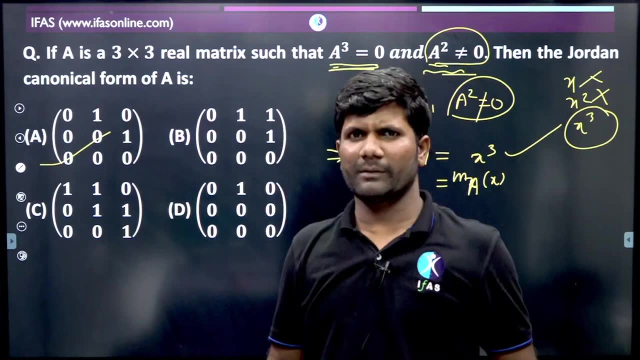 iitjam mask. It is a high channel of IFS, I have told you So maybe we will provide you the link of that channel in the comments. Remember it is happening on that channel from 8 o'clock, So this whole week is on that channel. 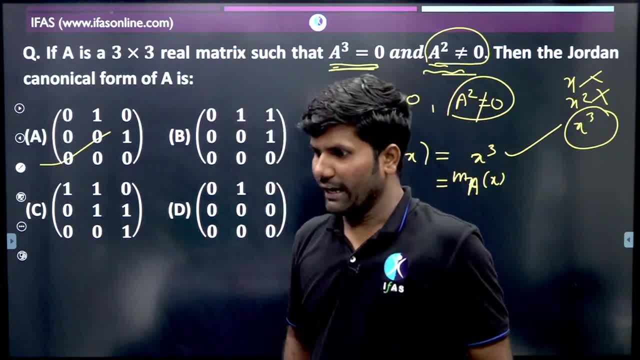 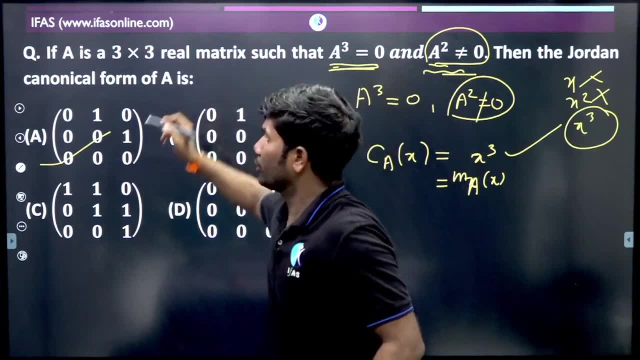 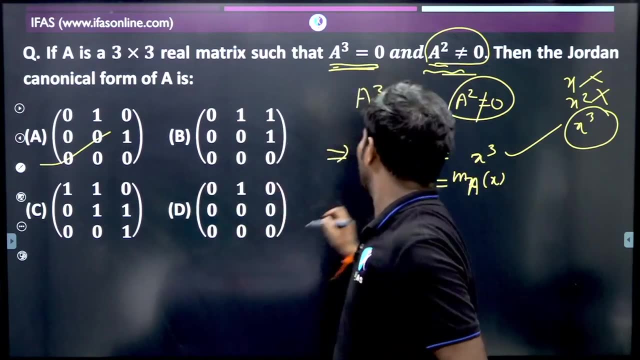 and on both channels. One is at 5 o'clock, one is at 8 o'clock. In that case, anything could have happened. It means here nothing was said about a, whether it is non-zero or not, a could have been 0,. 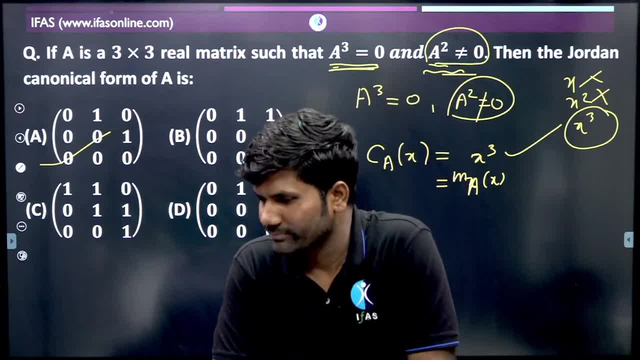 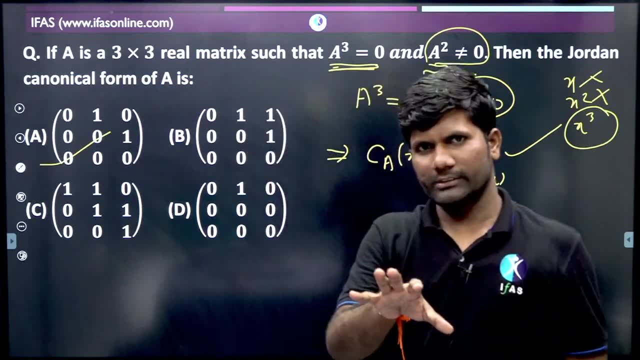 a square could have been 0.. Now we can't tell you for sure. For this we have given a condition here. If this had not happened, then there would have been some other answer. Yes, Dilip. okay, Shall we go ahead? 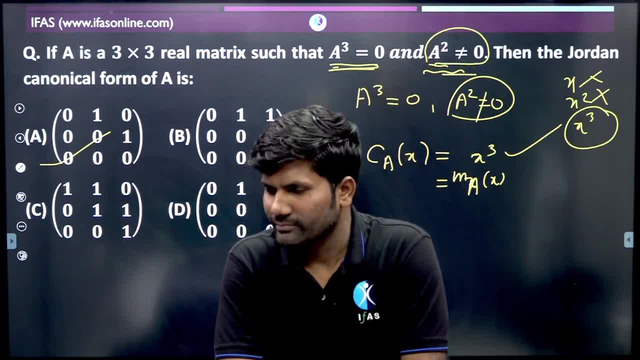 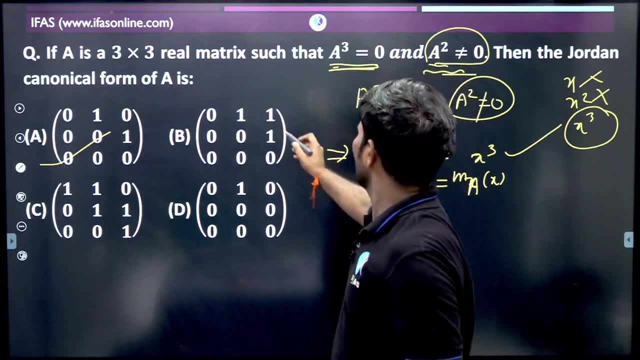 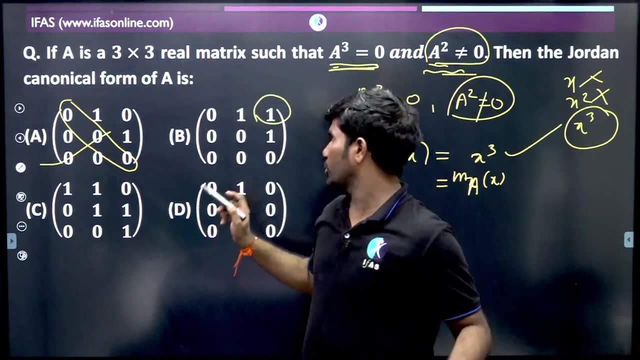 All of you Now tell me a and b may be correct. No, no, this will not happen. See, there is a 1 above this. this will not happen, See. only the diagonal has an eigenvalue and above that there is a 1 on the diagonal. 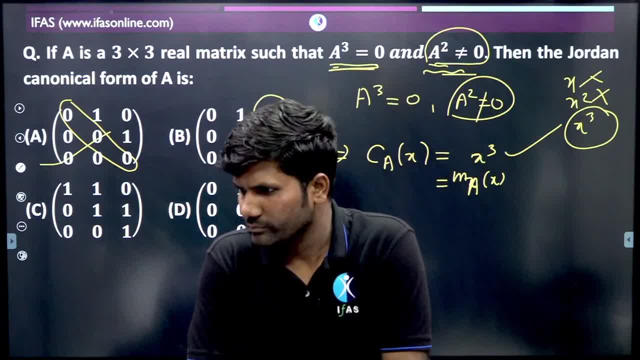 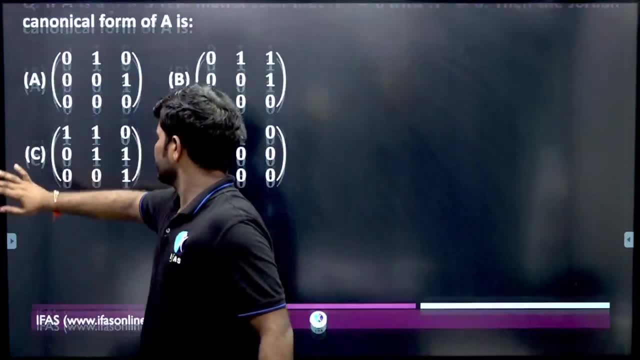 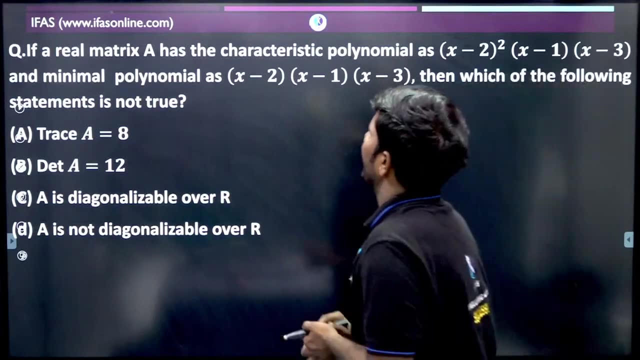 The rest is 0.. There is a 1 above this. this will not happen. a, b, karim. okay, Let's come to the next slide. Let's go ahead. We have a question here too. If a is a real matrix, 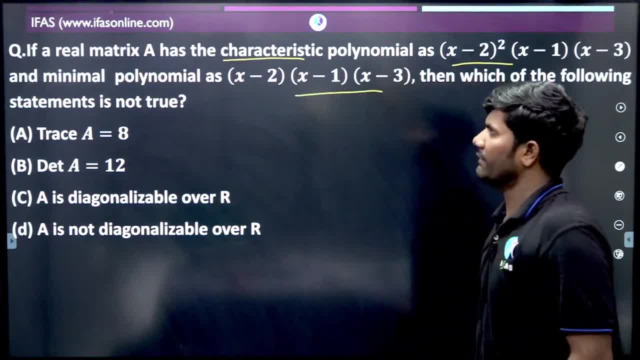 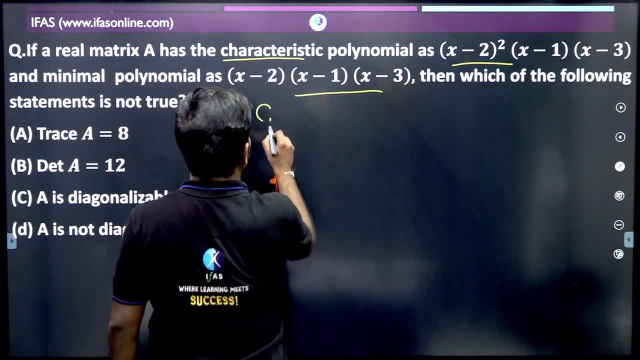 has a characteristic polynomial, this and minimal polynomial. is this then, which of the following statement is not true? Now we have given characteristic polynomial and minimal polynomial. we have to tell which option is not true. So cx is, given that characteristic polynomial is x-2 square. 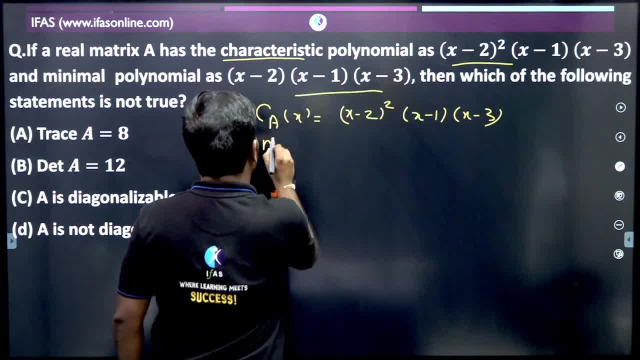 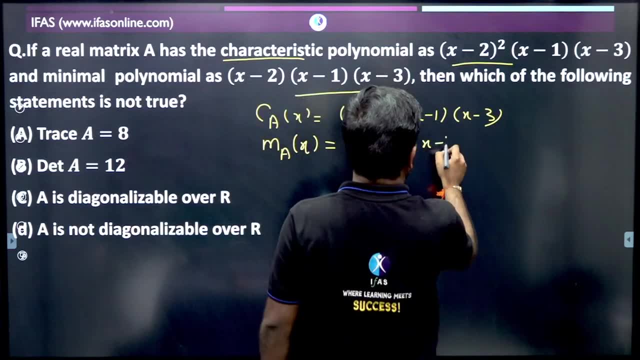 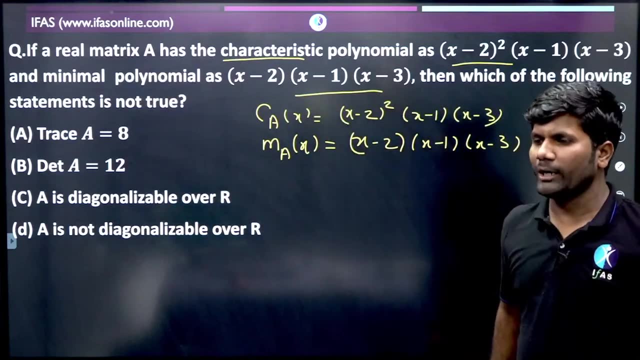 x-1, x-3.. What is given to us Minimal polynomial is given to us x-2, x-1, x-3.. Now we have to tell you what is the correct answer. So quickly solve all the students. 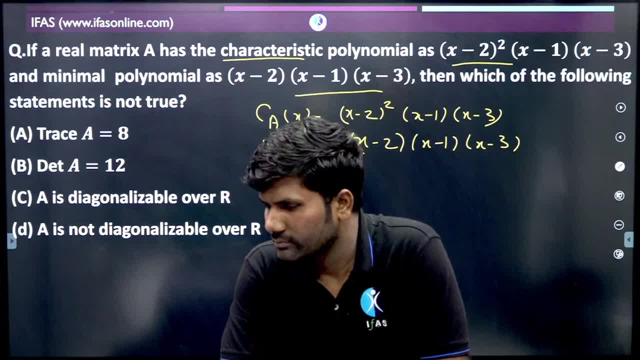 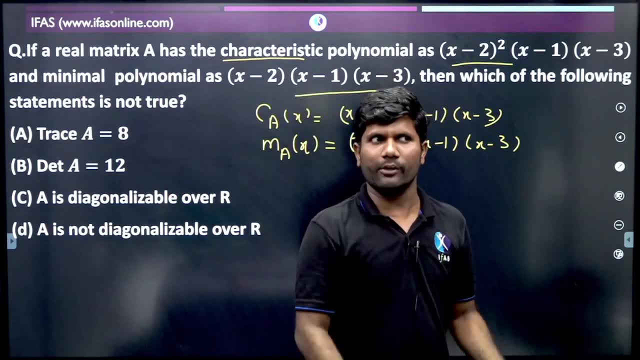 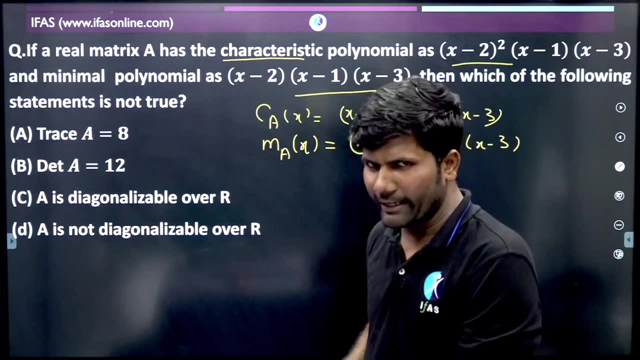 and tell what is the correct answer here. Tell me See, in the comment section our team has provided a link. So if you click there, you will go to our official website and you will get the question practice there. Just copy the link. 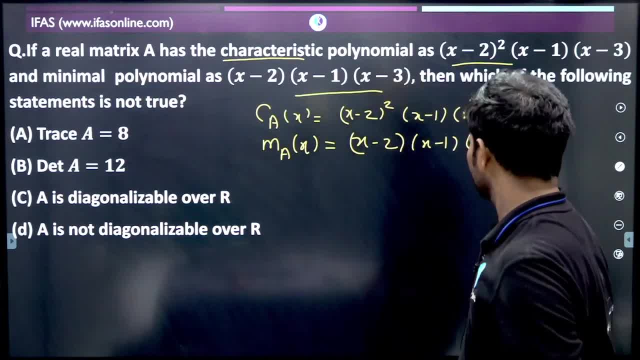 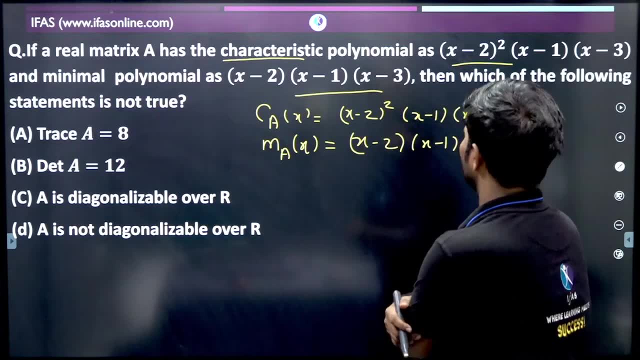 and go after the lecture. Now what was the first one? Trash of a is 8.. Trash is the sum of eigenvalues. So what are the eigenvalues? 2, 2, 1, 3.. Now add them. 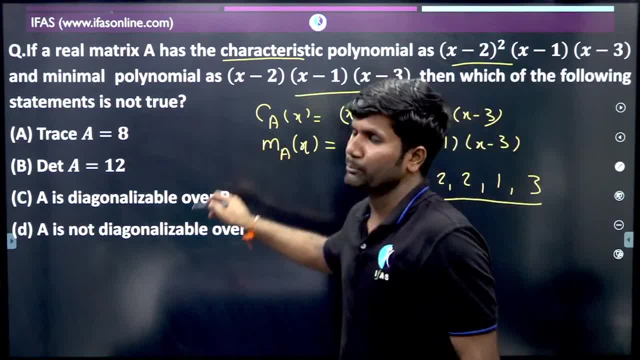 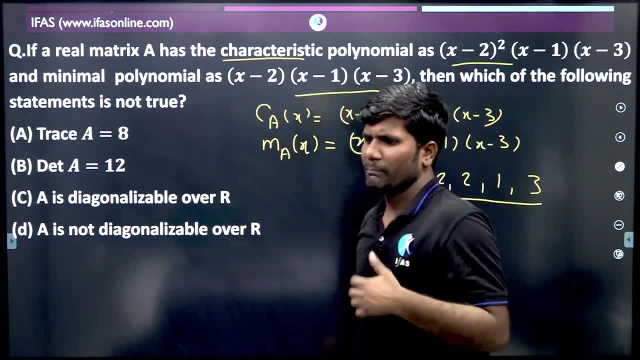 See how much will it be. It will be 8.. So trash is 8.. Which of the following statement is not true? This is true, But we have to select incorrect. Which of the following statement is not true: 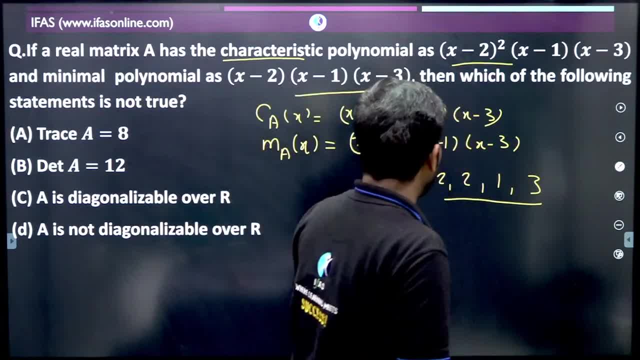 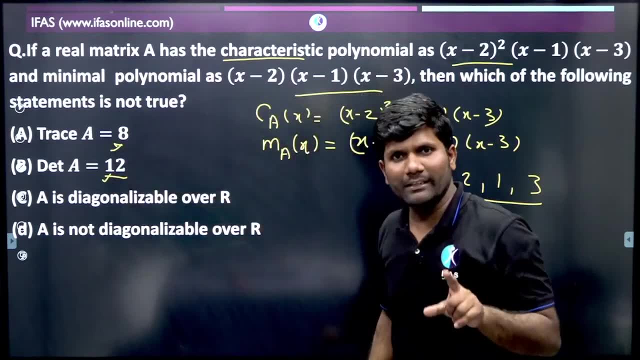 After that, what is option B? Determinant of a is 12. Now you will multiply them. Product of eigenvalues is same as determinant. It means that its determinant is also 12.. This is also correct, But we have to select false statement. 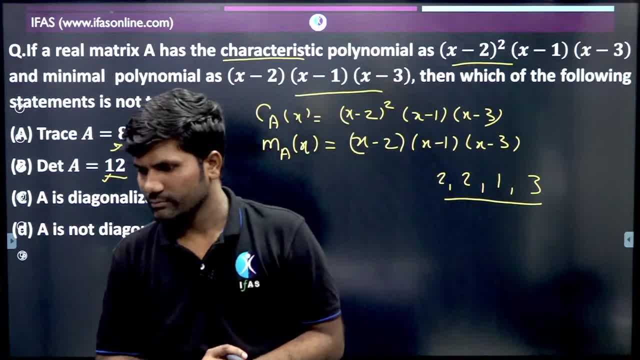 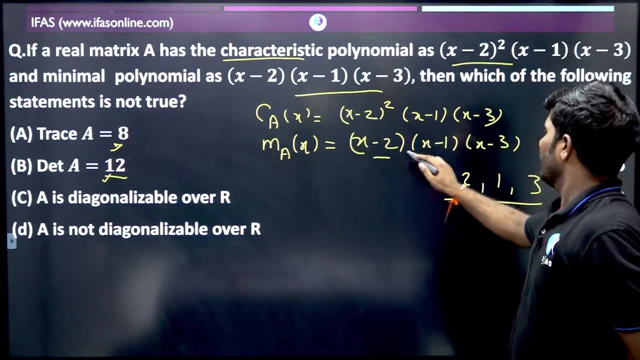 So we cannot say a and b are correct, Absolutely Bharti. Now if you see here, a is diagonalizable over r. What are all the eigenvalues of a? They are real number. And what is minimal polynomial? 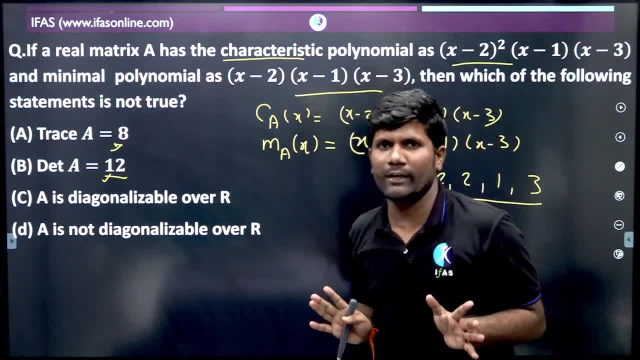 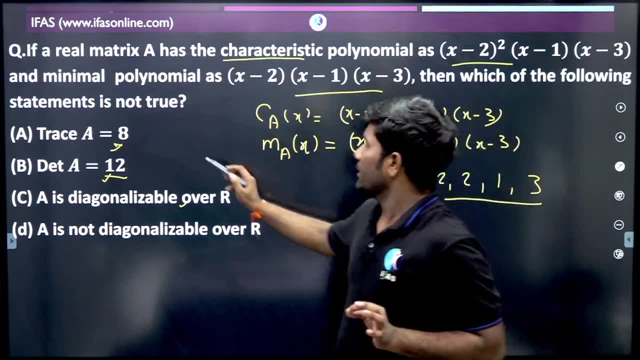 Product of non-repeated linear factor. It means that this matrix is diagonalizable. So here option C is also correct. We have to select incorrect, So we will not select this also. Keep this in mind during the exam Here, not true. 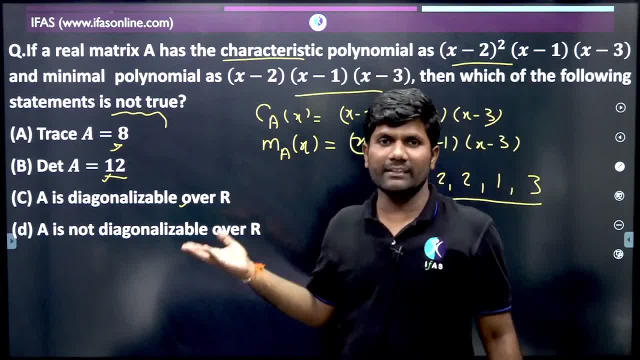 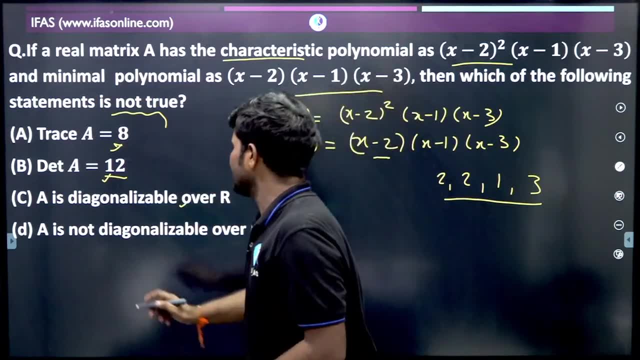 Here, many people make mistakes. If you do not read the question carefully, then which of the following is incorrect? Which of the following is or are false? But what you do? You quickly select anything. It is diagonalizable over r. 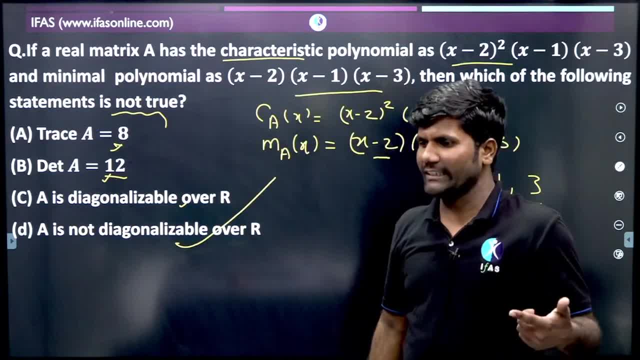 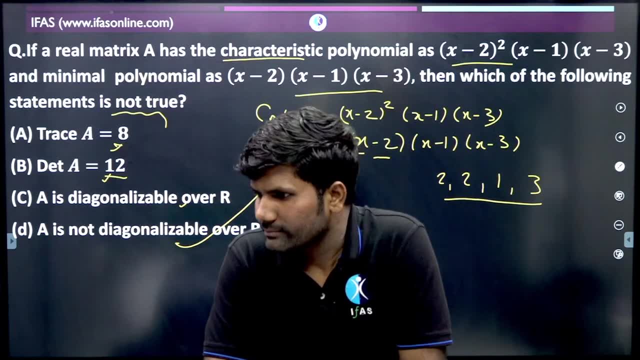 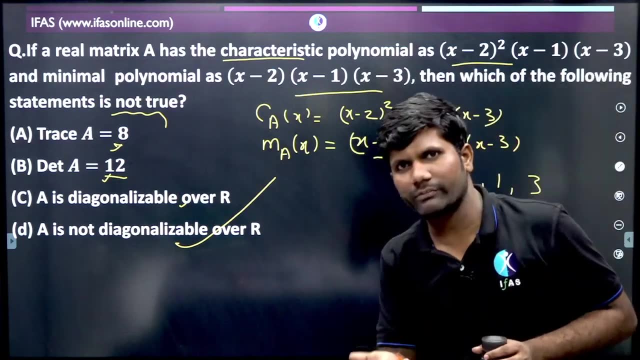 Which is incorrect. It means that this is correct According to the question. So here option D is correct. Yes, it is not true. No, entertainment, It is diagonalizable. Why? Because minimal polynomial is product of non-repeated linear factor. 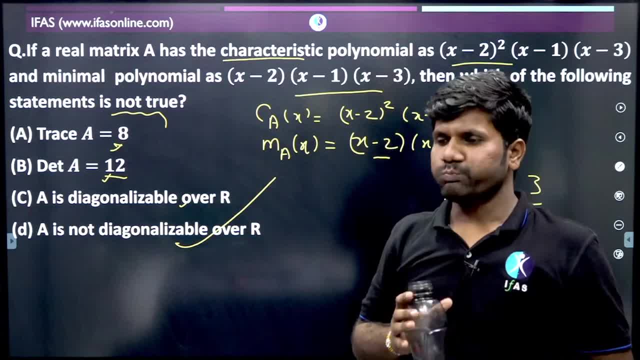 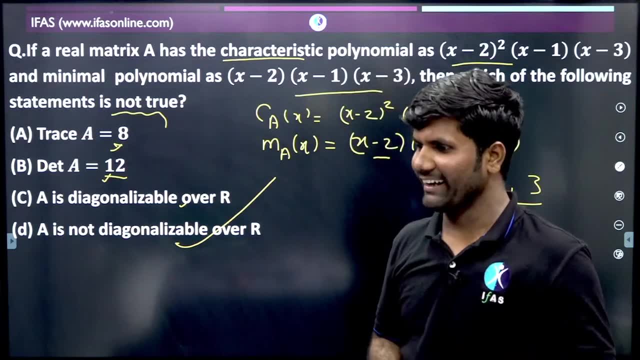 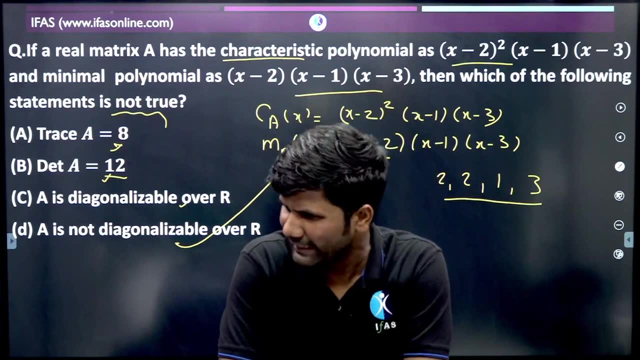 Sakshi. what happened? Did you not understand? What is the matter? Tell me, what did you not understand? Look at Vaishnavi. he understood. He said: yes, Ok, I am late Saturday. I am late Saturday. 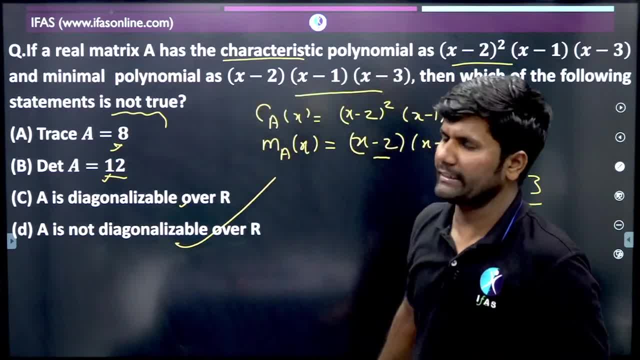 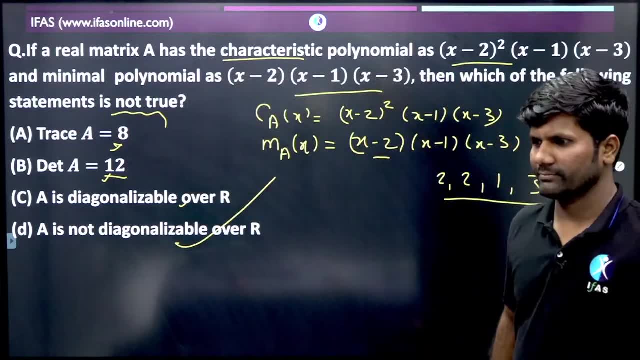 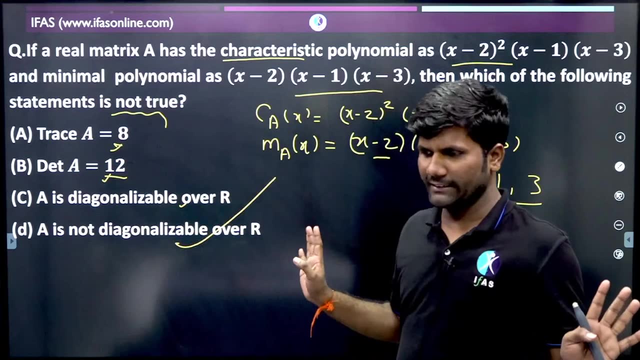 Ok, Ok, D is correct. Everyone understood, No doubt. Let us move ahead. You tell me once, All students tell me once: Ok, Now we can move ahead. Anshal is telling D. Very good, Anshal. 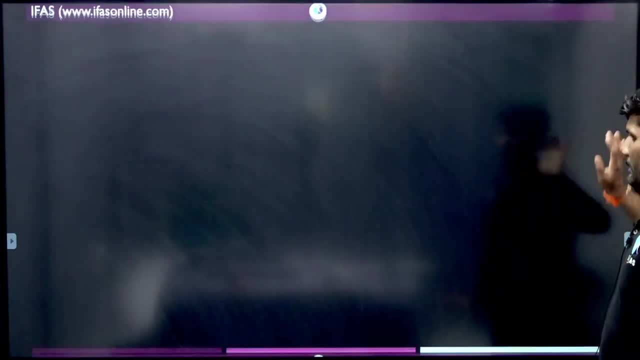 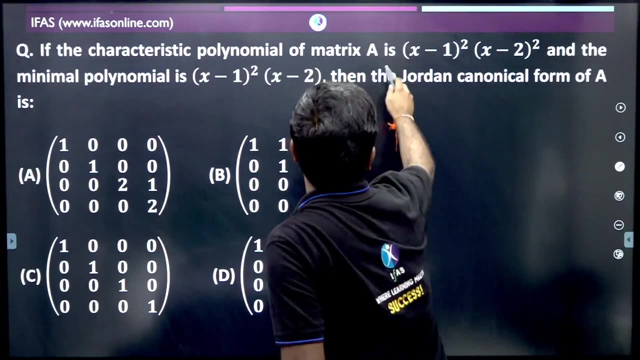 Ok, Let us come to the next slide. Let us see if there is a question or not. We have to see, Do this. There is one more question. If the characteristic polynomial of the matrix is this and minimal polynomial is this, then the Jordan. 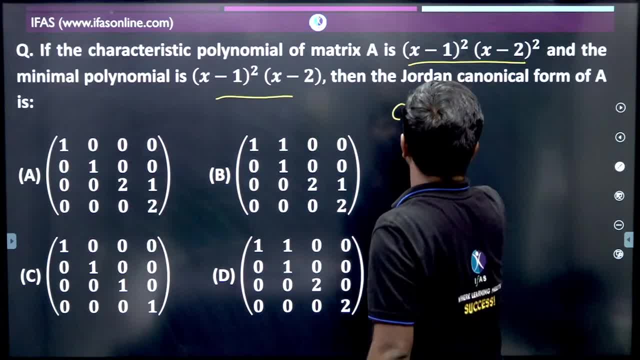 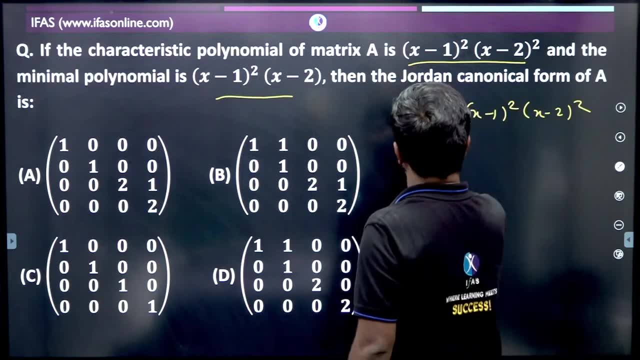 I think. has it been repeated? No, no, It is not repeated. What is characteristic polynomial? It is x-1 square, x-2 square and minimal polynomial is given that What is a minimal polynomial? Minimal polynomial is given to us. 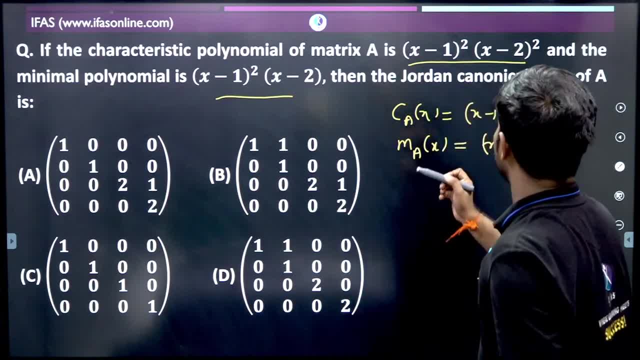 x-1 square and x-2.. Now tell me what will be the Jordan canonical form of this. Look, the size of the minimal polynomial is 2.. Here also, it is 2. Means a block will be made where 1,1 will be there. 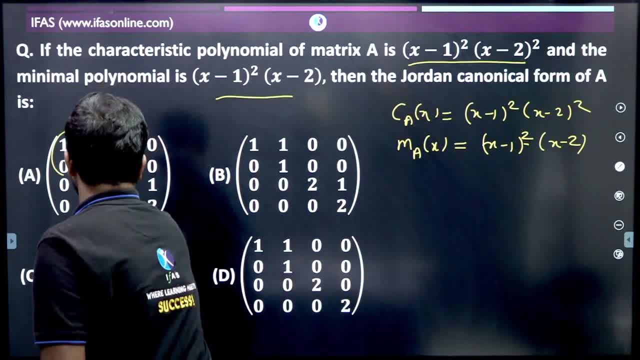 If 1 should come above 1,, which is not there, then it is over. If 1 should come above 1,, which is not there, then it is over. If 1 should come above 1,, which is not there, then it is over. 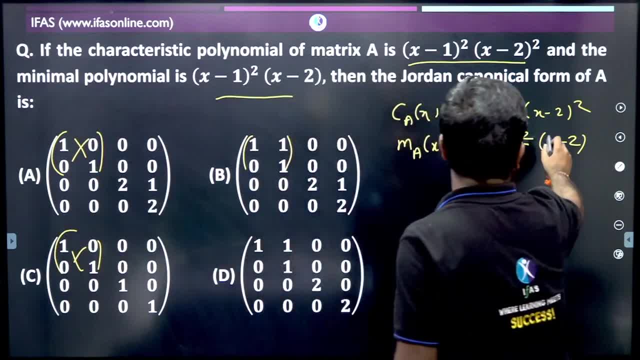 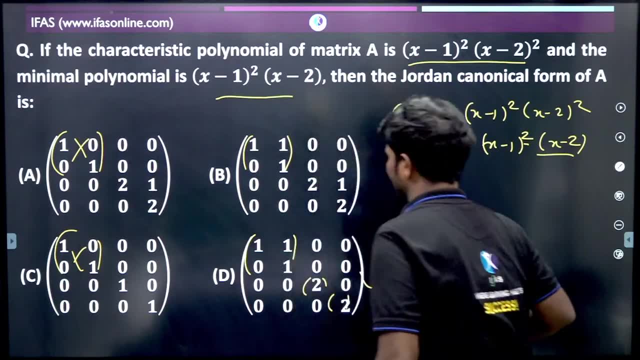 Here 1 came above 1.. A block is done. 2 should be made separate for 2.. Because the degree of minimal polynomial is 1.. 2 should be made separate here. It means that option D will be correct. 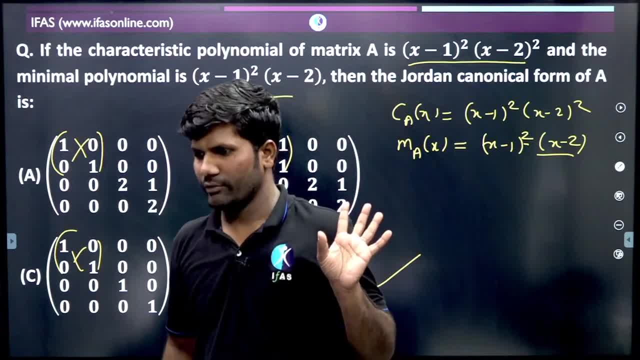 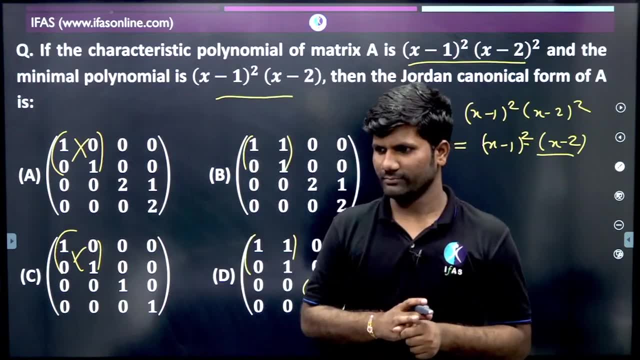 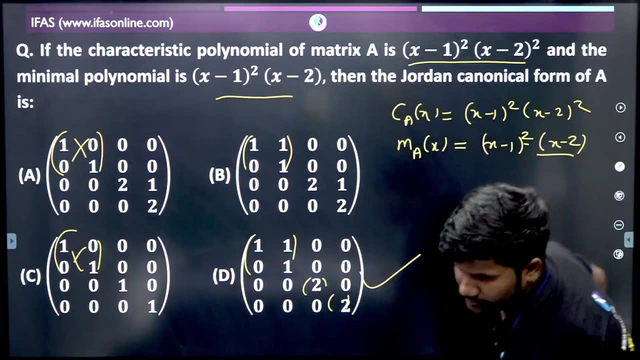 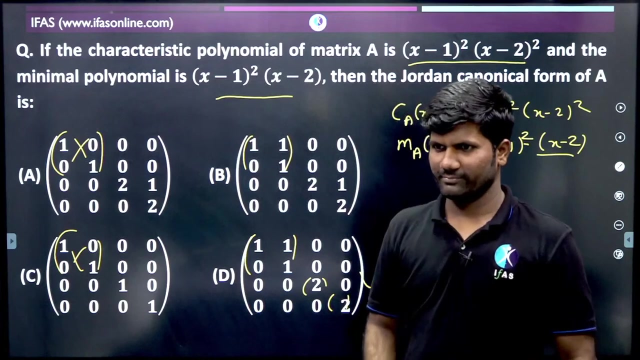 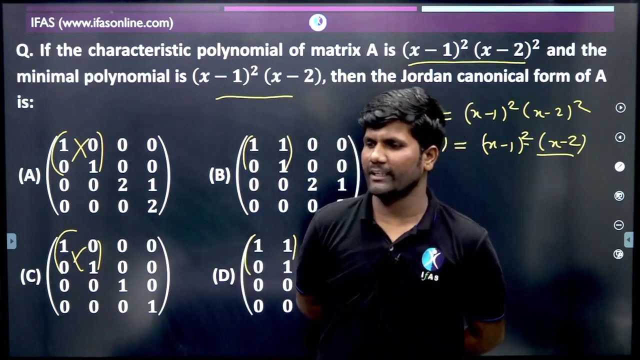 Is it clear to all students. Very good, Almost everyone has given the correct answer. D will be correct here. Okay, Come on. Did you like it? Come on, Tell me once. Very good, Your answers all are correct, Chuleshwar. 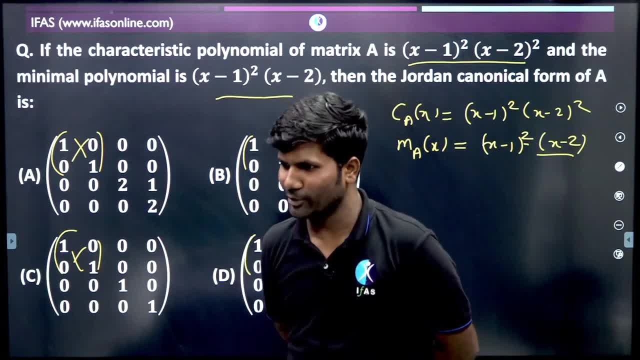 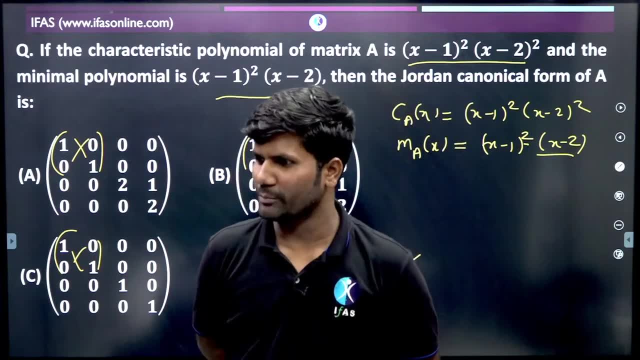 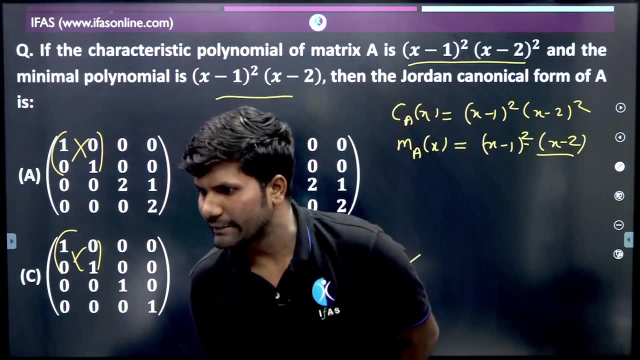 Chuleshwar, Gupta, Gopta, Jyotika, Satchina, shorts, Bharati, Lalita magazines believed be same. For the rest, explain accordingly. see how much power it has. in its minimal polynomial it is 1, so all the blocks that will be made for 2. 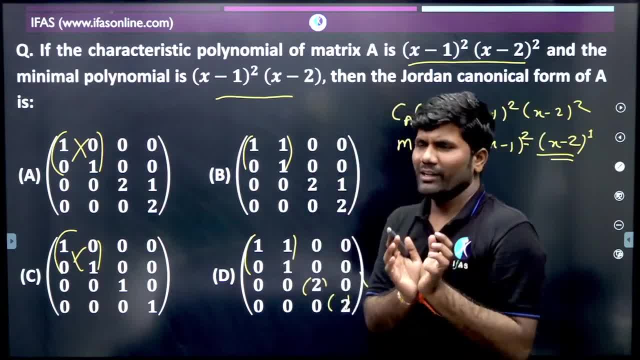 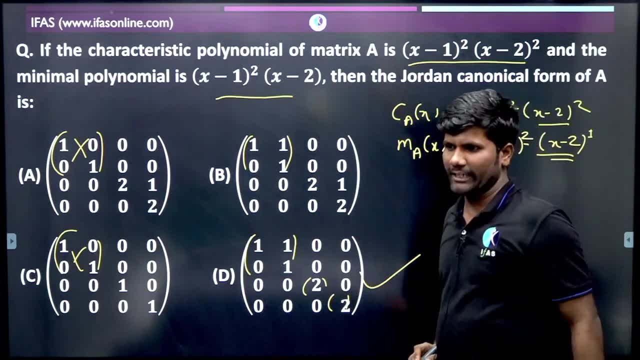 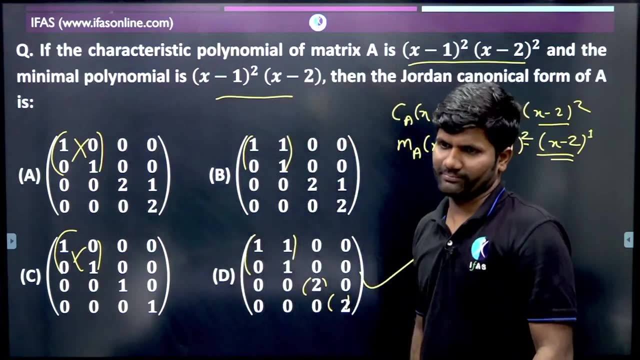 its size will be more than 1 or less than 1, and here the total is 2, power is 2. characteristic polynomial means 2 blocks of 1 cross 1 will be made, which is made here. ok, Thank you, Bharti. all the students are clear. 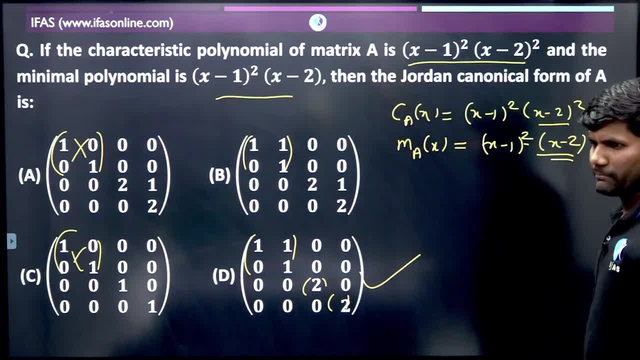 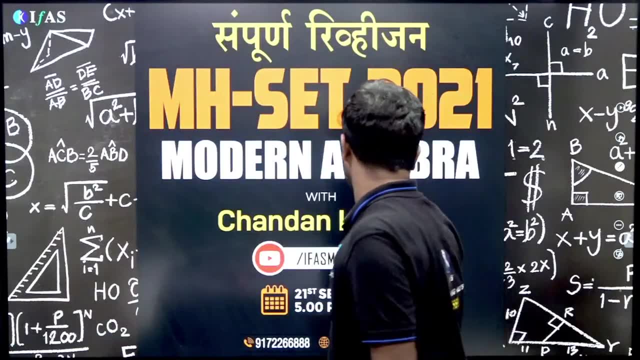 ok, next slide. if there are any questions, then we will do it. ok, I also don't remember whether there is a question or not. ok, now there is no question. so tomorrow there will be modern algebra, or you can say upside algebra. Chandan sir will join with you. 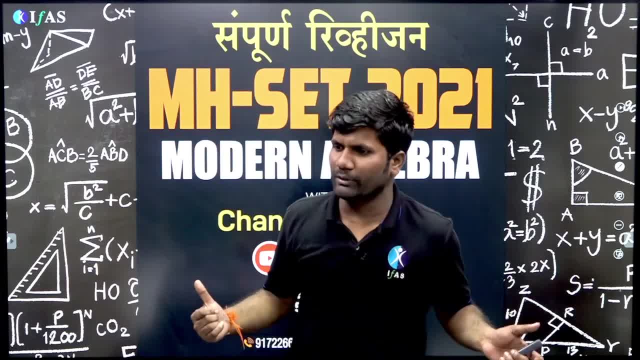 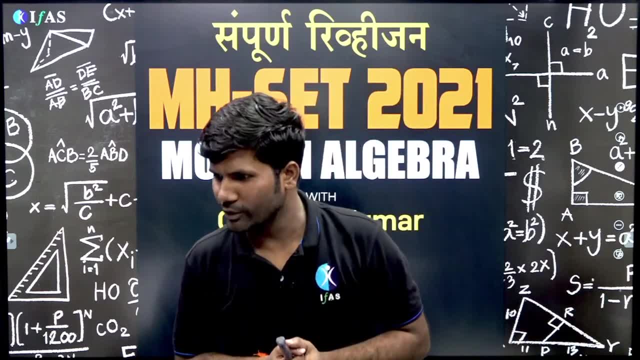 time will be same. 5 pm channel will be same. you just have to join with them. revise your group theory and ring theory. ok, Thank you, Anu. so let's hope that today's session you must have enjoyed so once, if you haven't liked it yet.